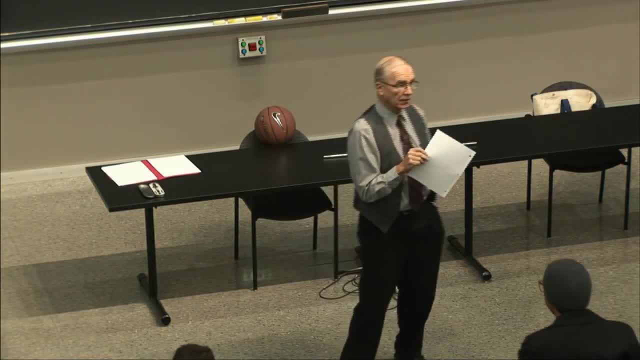 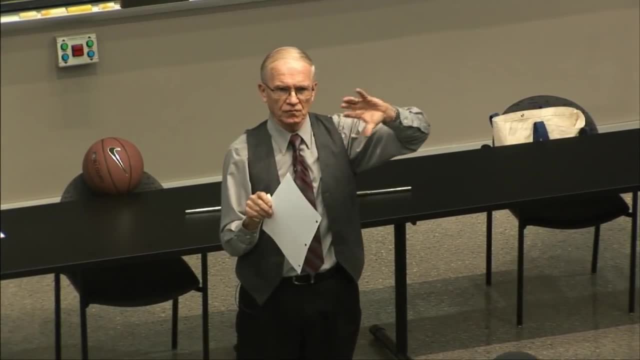 It's about 10 pages long And I highly recommend you read them. They're not somehow up with the notes associated with lecture notes. They're tiny. I'm going to weigh down at the bottom So you have to scroll all the way down in the Stellar website. 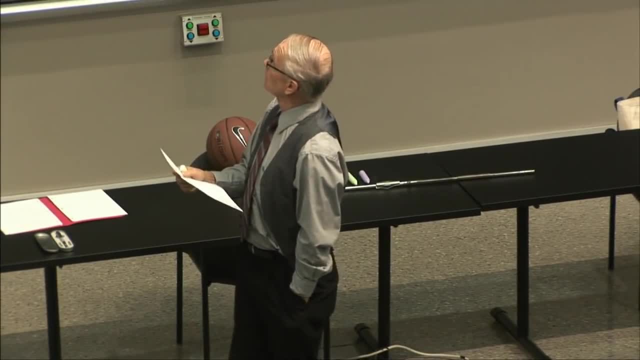 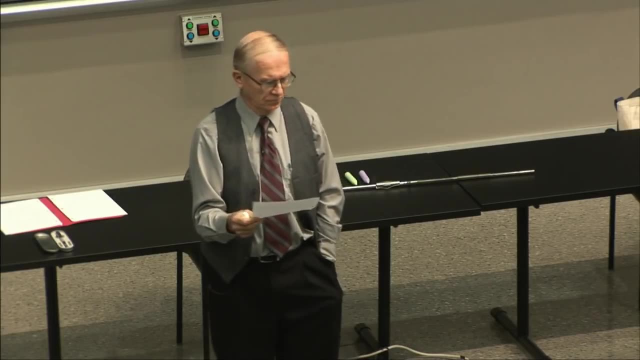 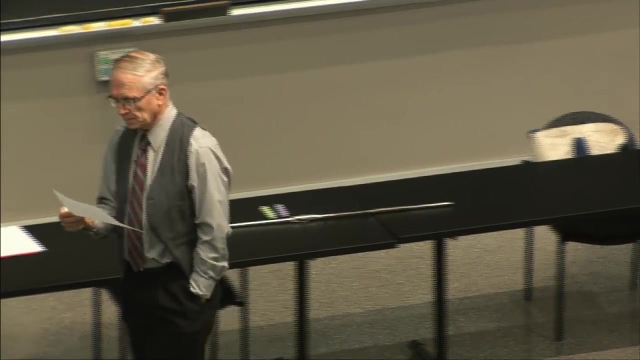 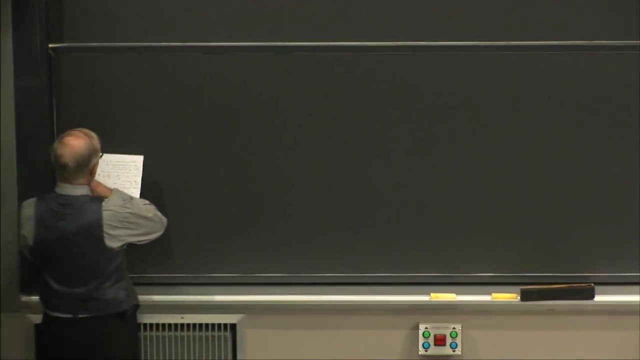 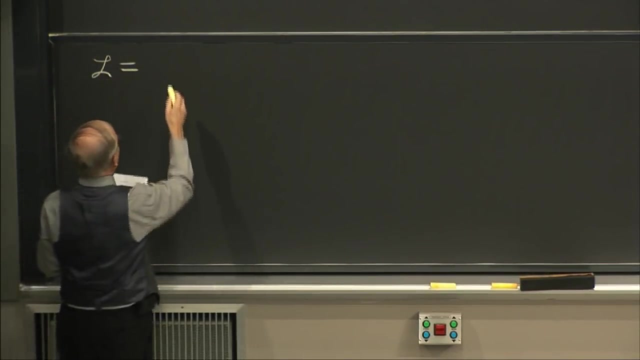 to find them. Our second quiz is November 8.. That's a week from next Tuesday. Pretty much same format as the first one. OK, so let's talk about how to use Lagrange equations. So I defined what's called the Lagrangian last time. 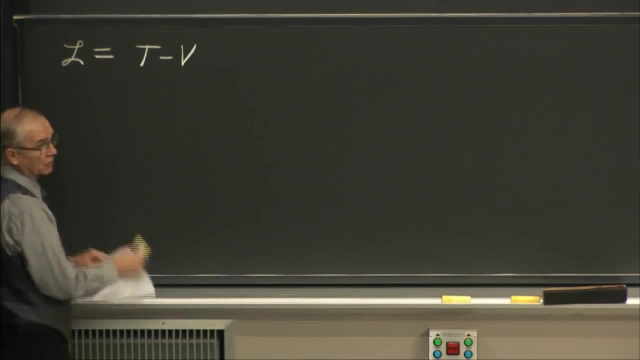 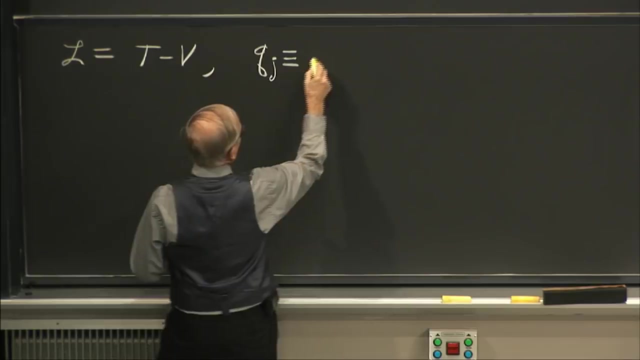 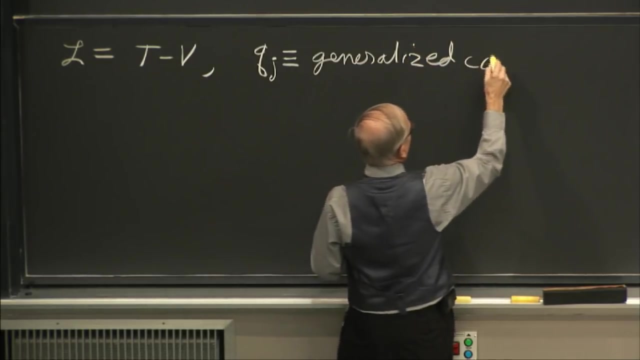 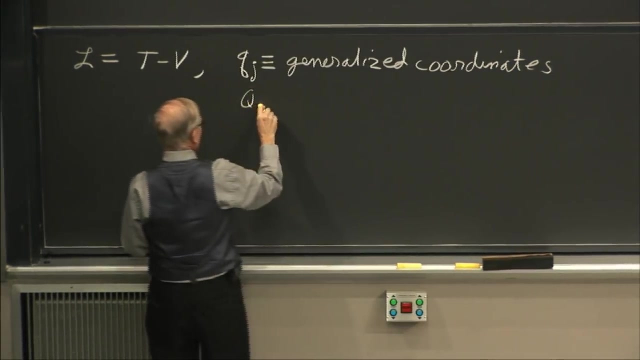 t minus v, the kinetic energy minus the potential energy of the entire system, total kinetic and total potential energy expressions. Then we have some quantities, qj's. These are defined as the generalized forces, Generalized coordinates, I should say, And the capital Q sub j's are the generalized forces. 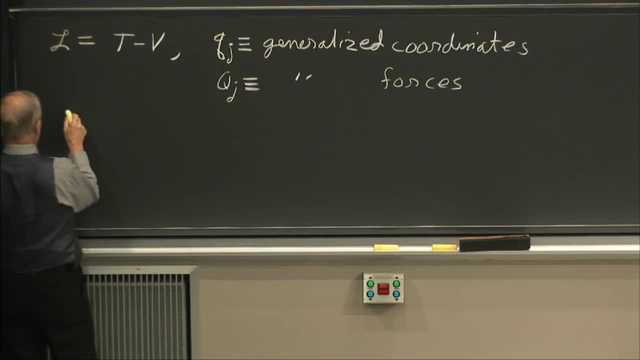 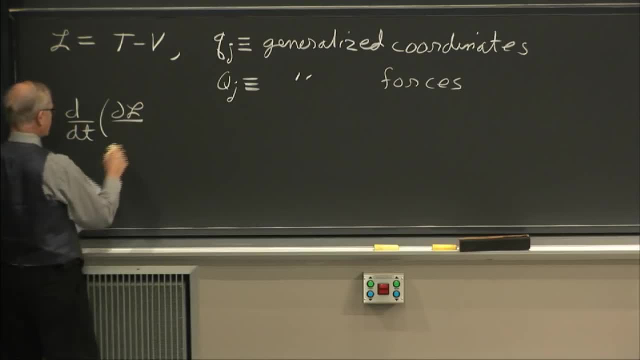 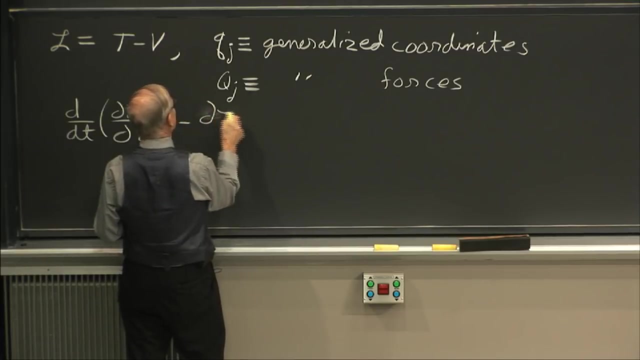 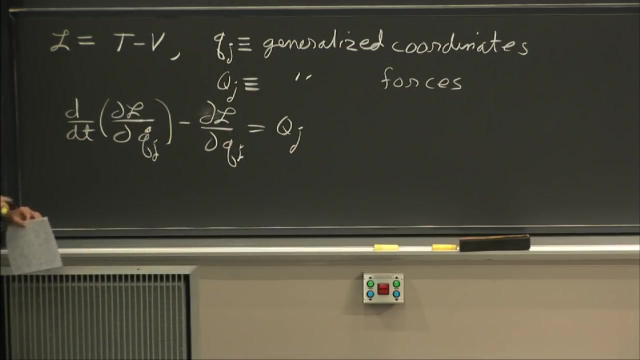 t equals 1.. t equals 1.. of the partial of L with respect to the qj dots the velocities, minus the partial derivative of L with respect to the generalized displacements equals the generalized forces And for a typical system you'll have a number. 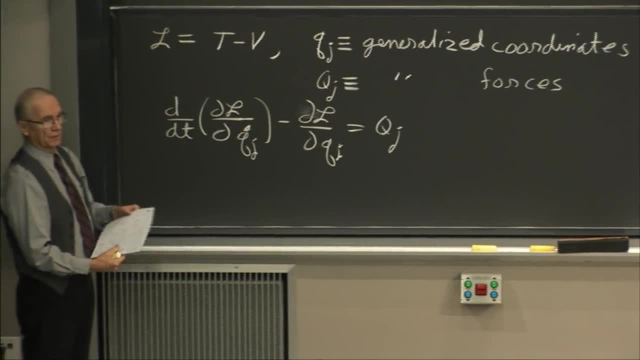 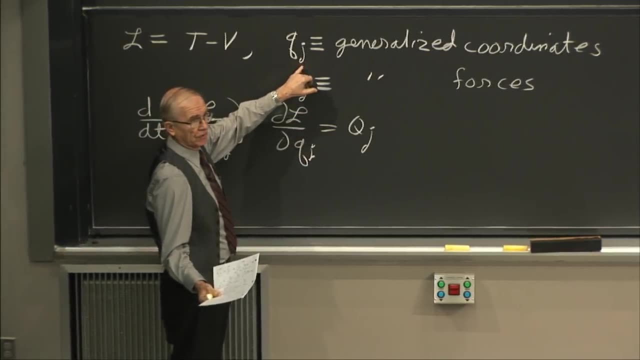 of degrees of freedom, like say 3.. And if you have three degrees of freedom, you need three equations of motion, And so the j's will go from 1 to 3 in that case. So the j's here refer to an indice. 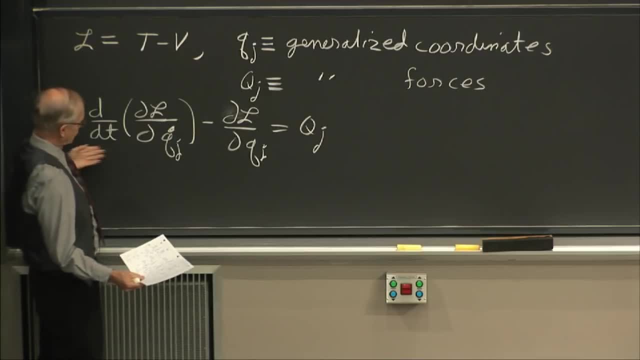 that gives you the number of equations that you need. So you do this calculation for coordinate 1, again for coordinate 2, again for coordinate 3, and you get then three equations of motion. OK, So this is a little obscure. 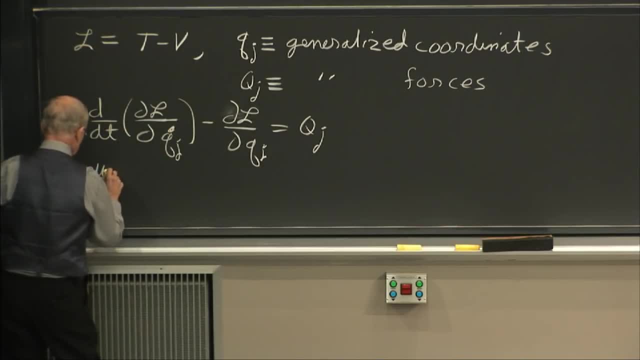 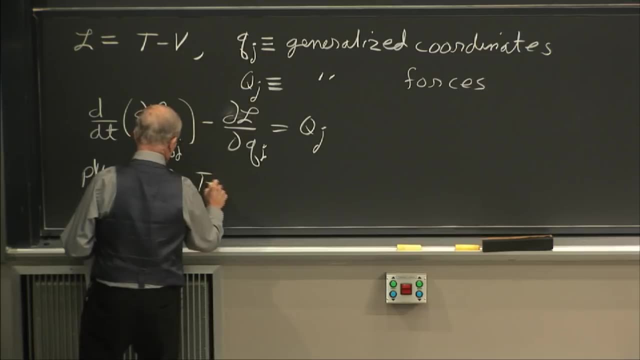 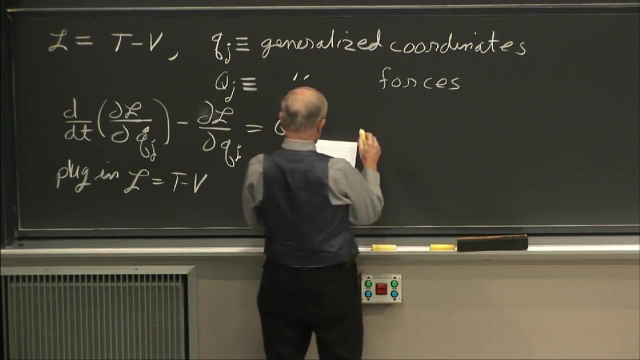 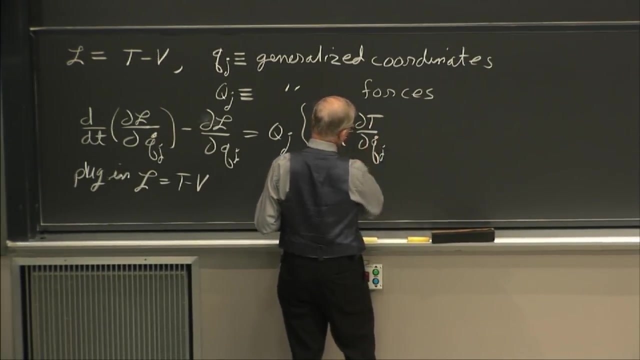 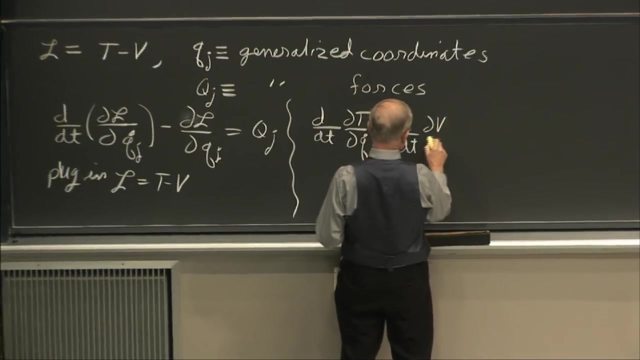 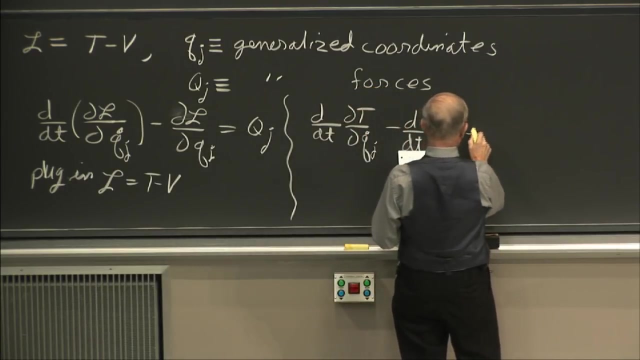 I like to let's just plug in for L equals t minus v And just put it in here and see what happens. You get d by dt of The partial of t with respect to qj dot minus d by dt of the partial of v with respect to qj dot plus. 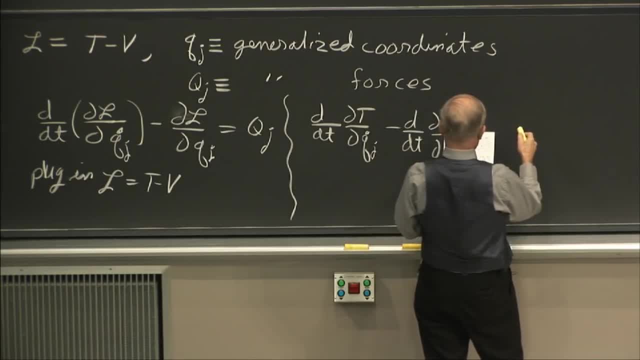 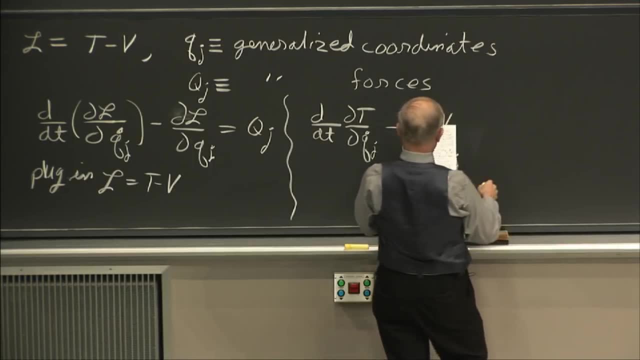 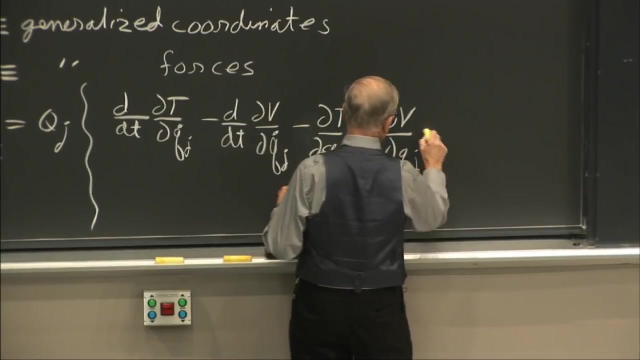 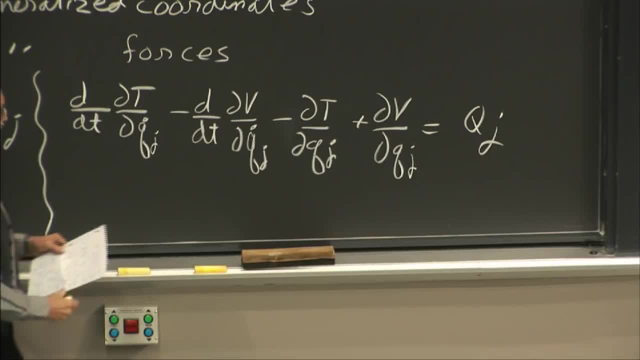 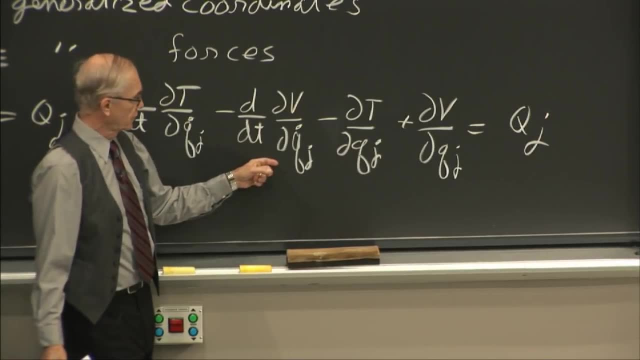 equals capital Q, Aj's. Now, when we first talked about potential energy a few days ago, we said that for mechanical systems, function of time, or anybody remember velocity? So if the potential energy is not a function of time or velocity, what will happen to this term? 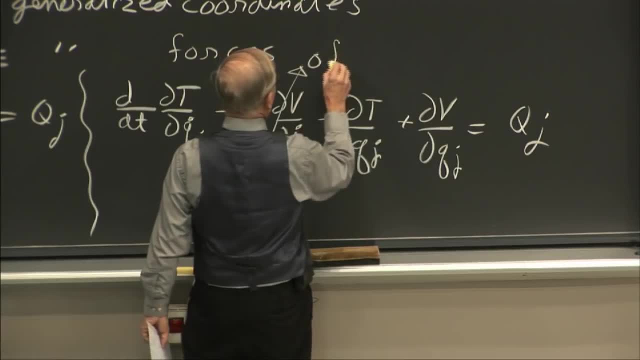 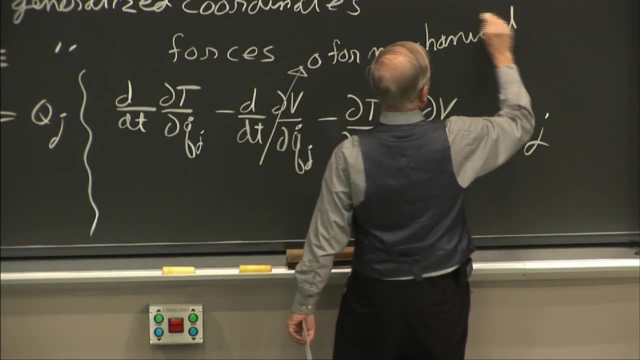 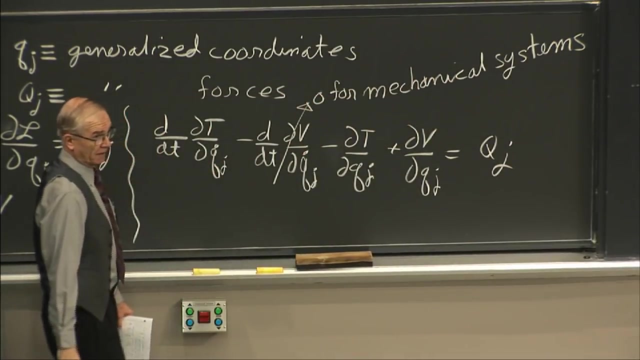 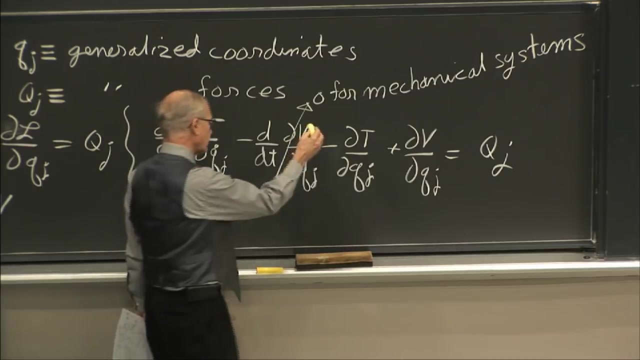 This goes away. So this is 0 for mechanical systems. If you start getting into electrons moving in magnetic fields, then you start having potential energies involving velocities, But for mechanical systems this term's 0. And I think the bookkeeping. so this: 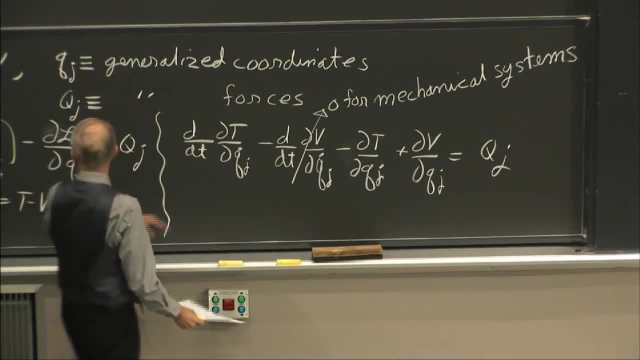 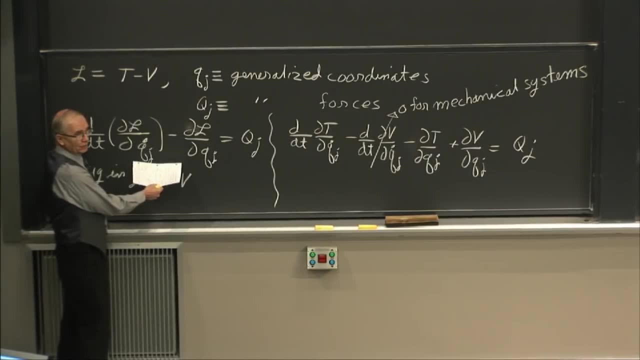 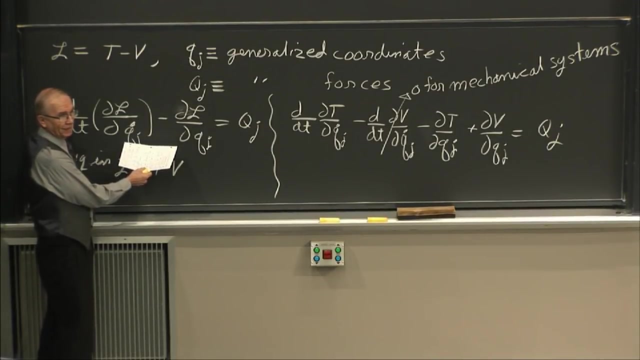 is the form of Lagrange equations that I write down when I'm doing problems. I don't write this. Mathematicians like elegance And this comes down to this, this beautifully elegant, simple-looking formula, But I'm an engineer And I like it to be efficient and practically useful. 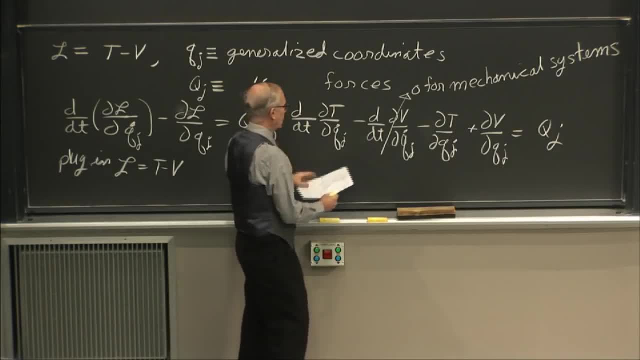 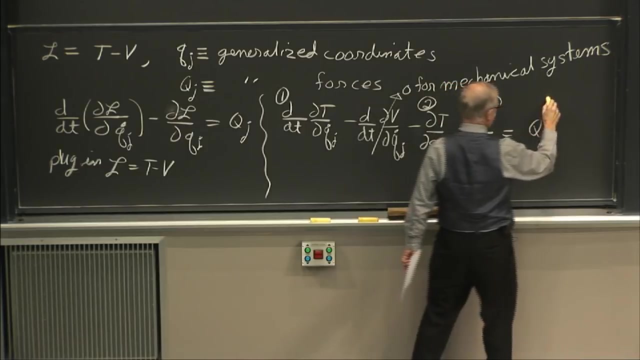 This is the practically useful form of Lagrange equations, So you just use what you need: Kinetic energy here, kinetic energy there, potential energy there, And I number these. There's a lot of bookkeeping in Lagrange, So I call it term 1, term 2, term 3, and term 4.. 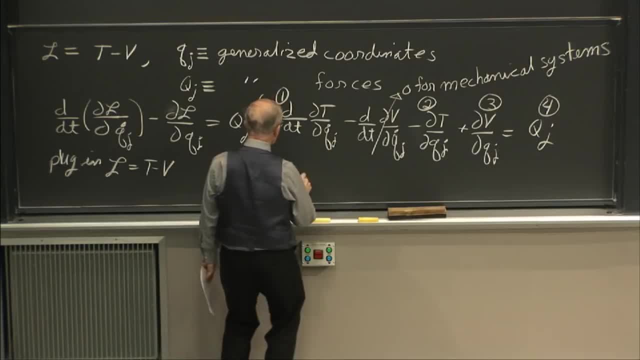 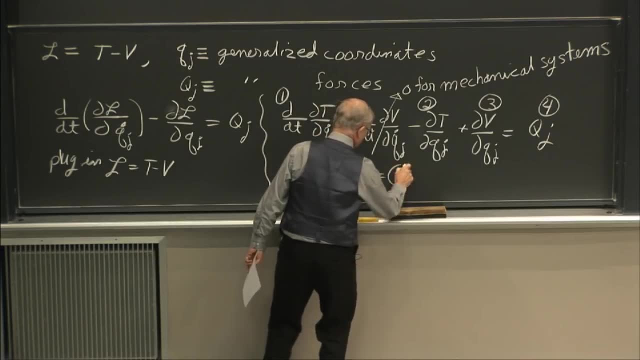 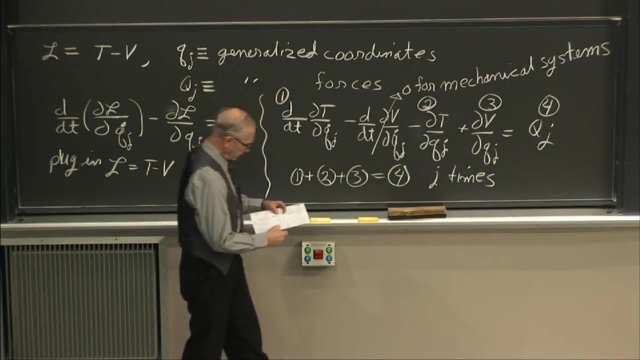 Because you have to grind through this quite a few times, And so when you do, basically you take 1, the results of 1, plus 2, plus 3, equals 4.. And you do that j times to get the equations you're after. 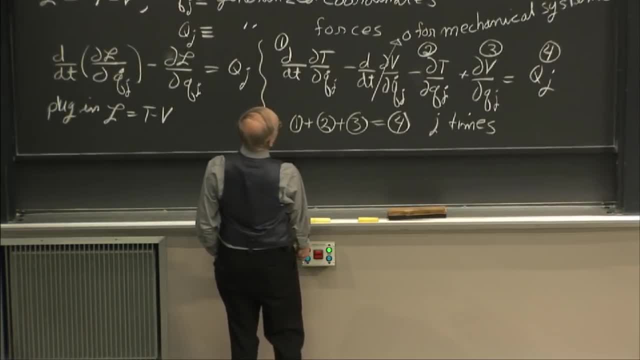 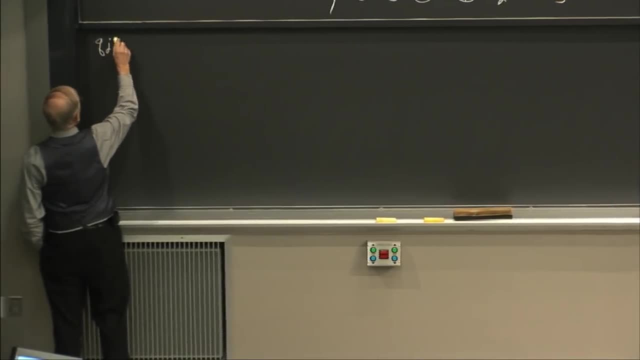 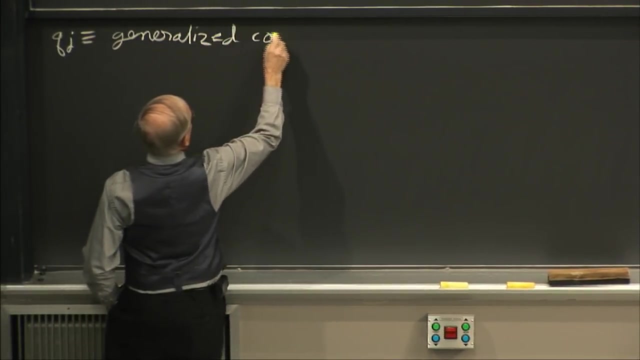 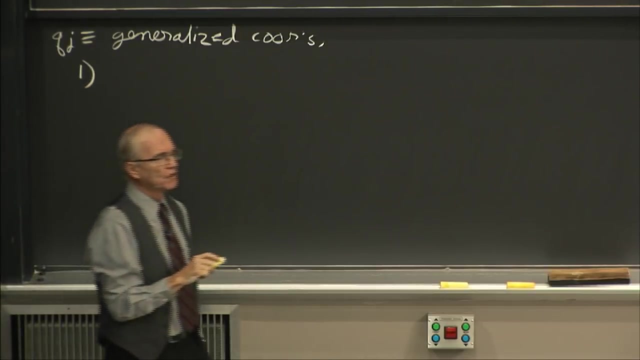 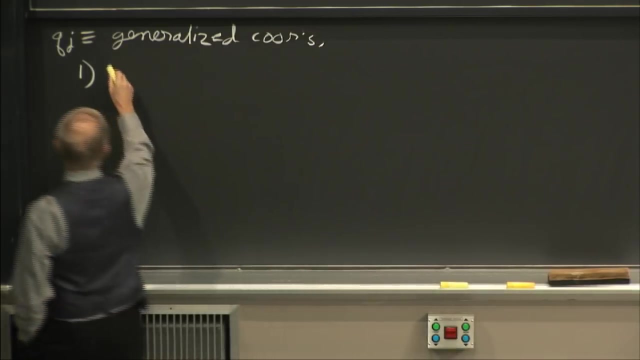 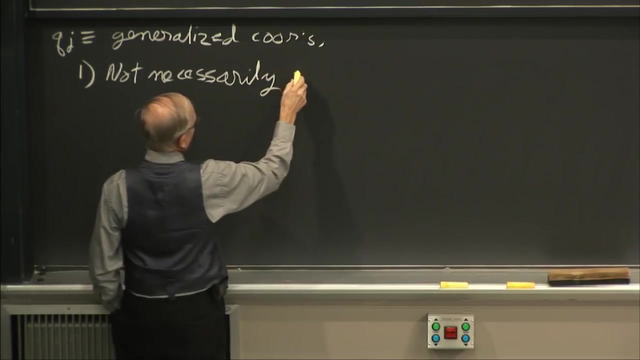 So now we need to talk a little bit about what we mean by generalized coordinates qj. What's this word generalized mean? Generalized just means it doesn't have to be Cartesian, Not necessarily Cartesian As in x, y, z. 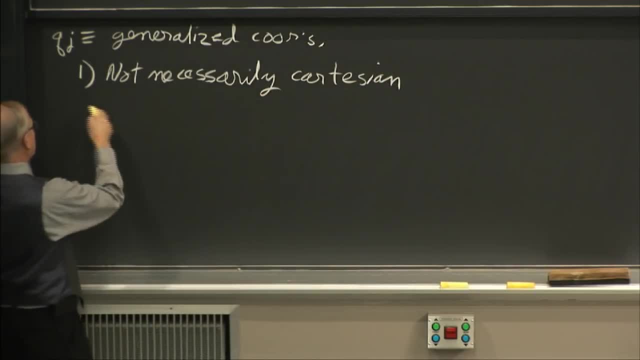 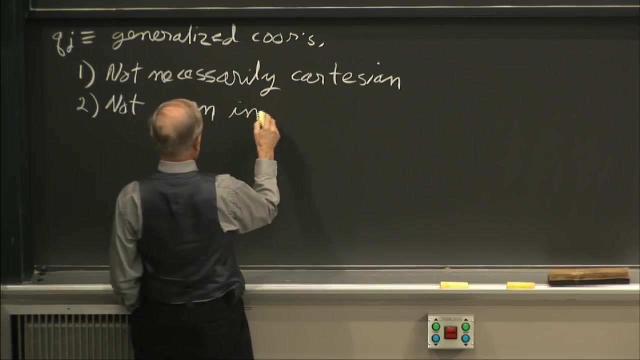 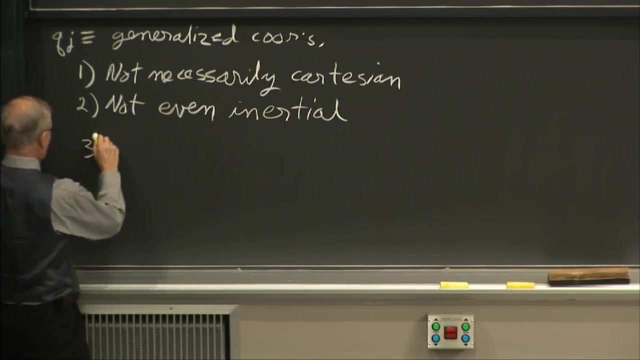 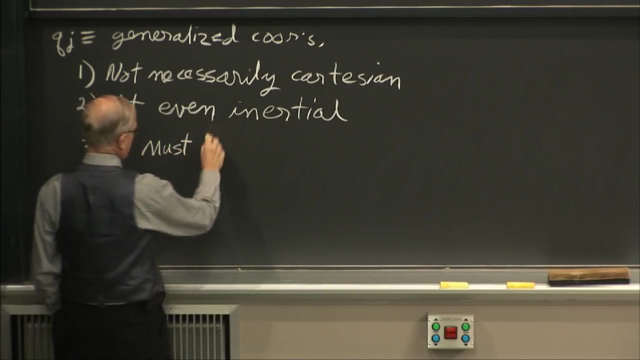 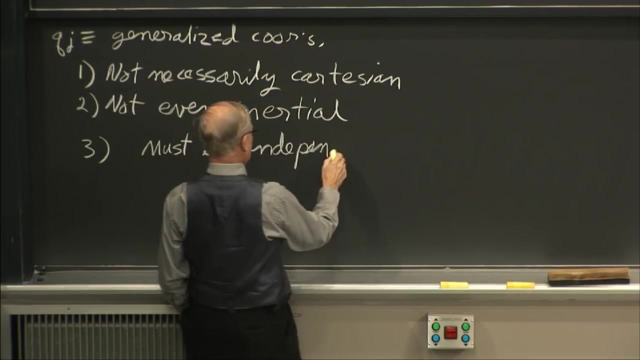 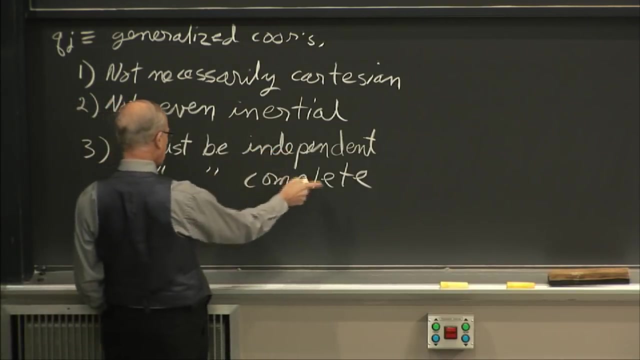 You have a lot of liberty in how you choose coordinates, Not necessarily Cartesian, Not even inertial. They do have to satisfy certain requirements. The coordinates, they must be what we call independent, They must be complete, And so they must be independent and complete. 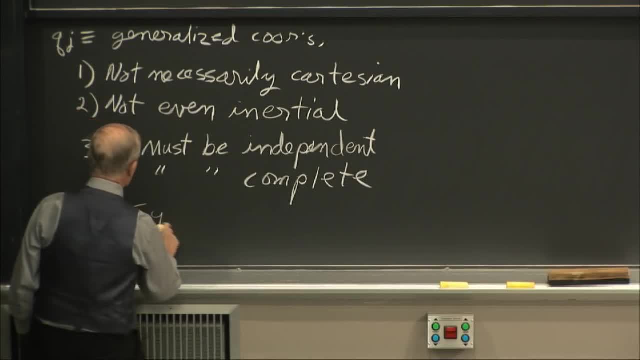 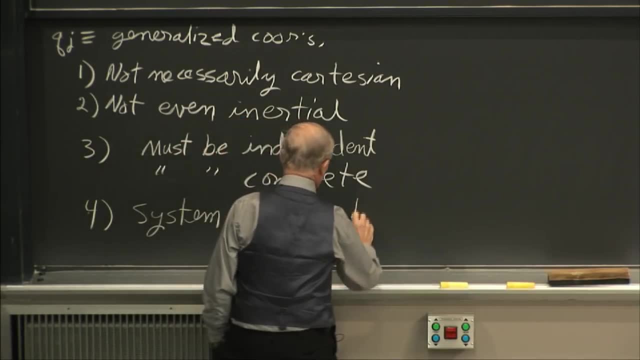 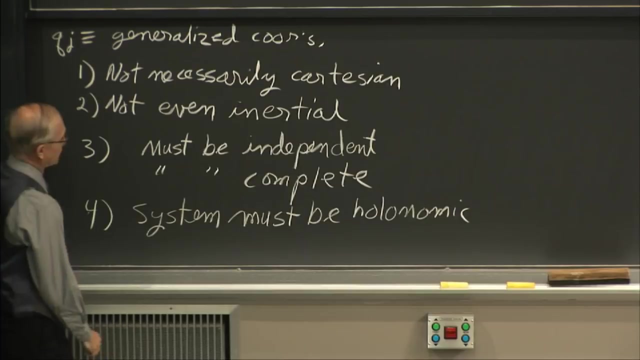 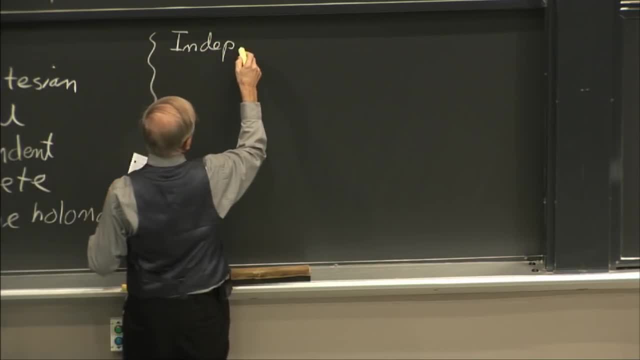 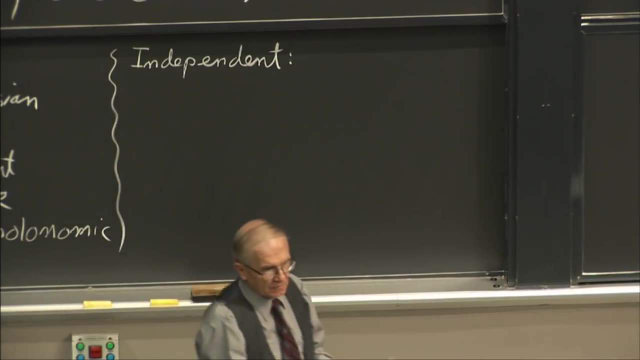 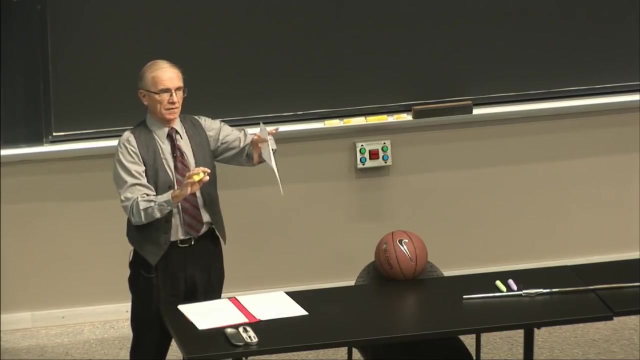 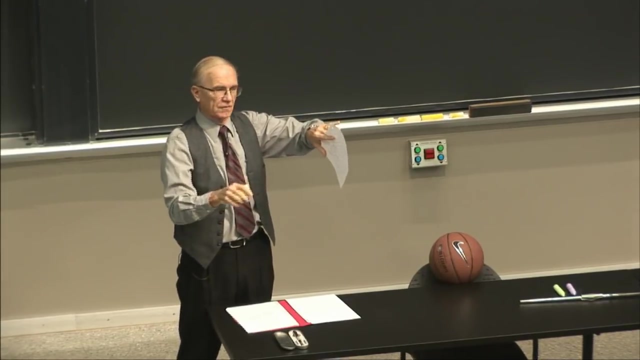 So what this means? It has to be belongs, It has to be independent. So what do we mean by independent? So if you have a multiple degree of freedom system and you fix all but one of the coordinates, a system can't move in all but one of its coordinates. 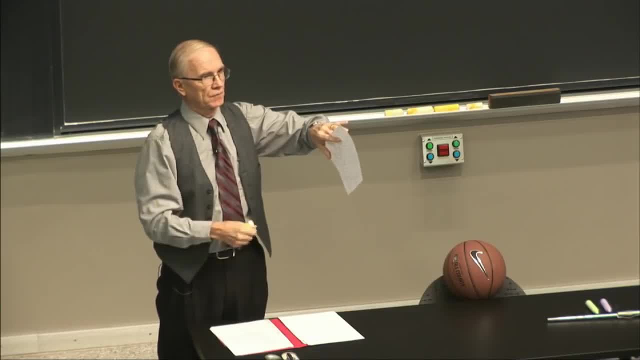 That last degree of freedom still has to have a complete range of motion. They have to have the complete rule, the range of motion. So if you have a multiple degree of freedom, So if you have a double pendulum and you grab the first mass, 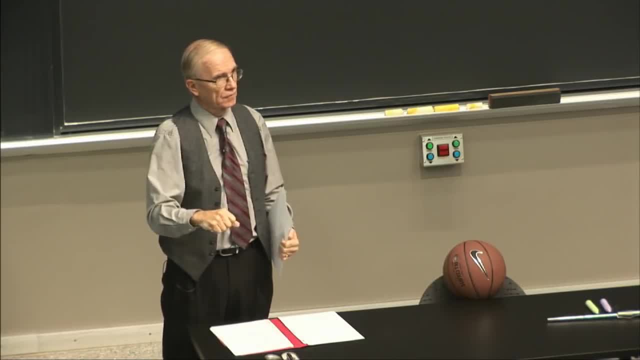 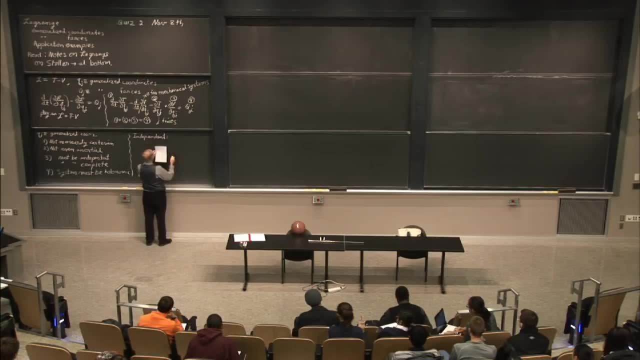 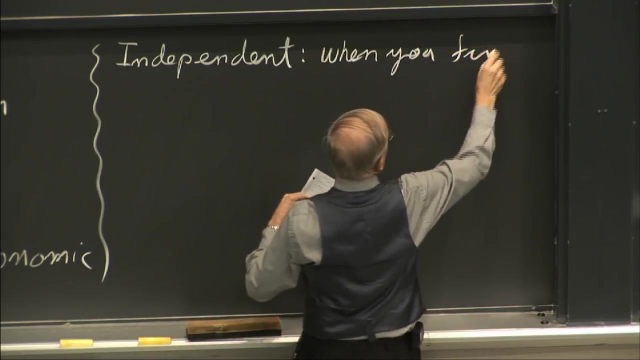 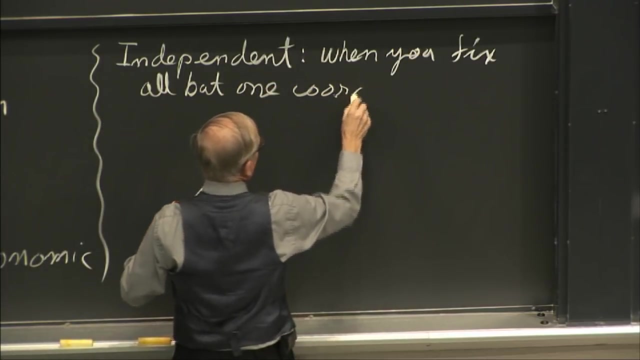 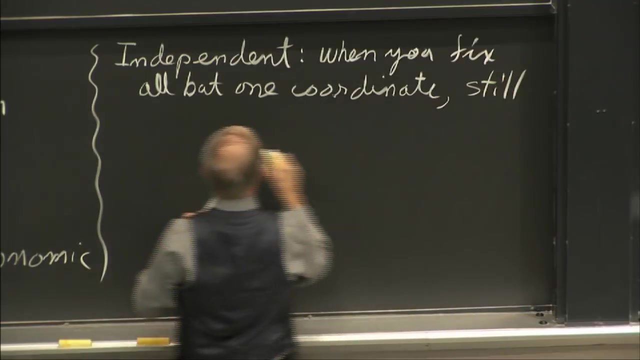 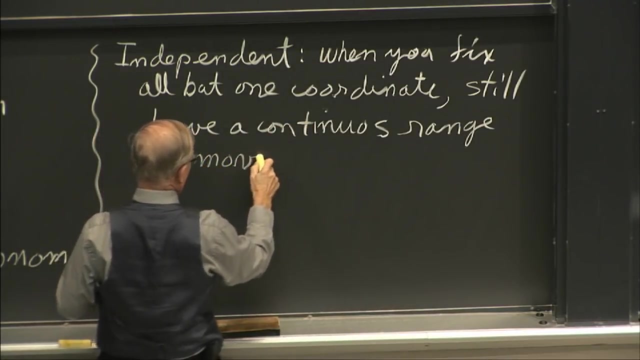 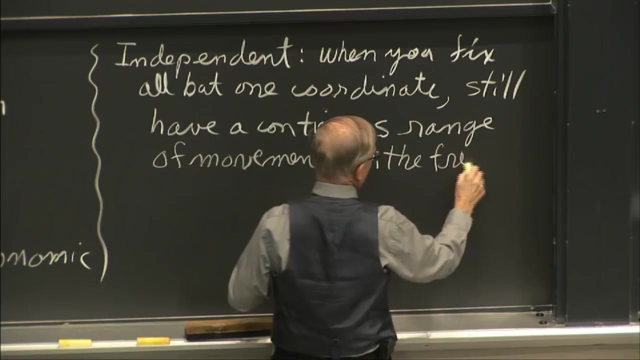 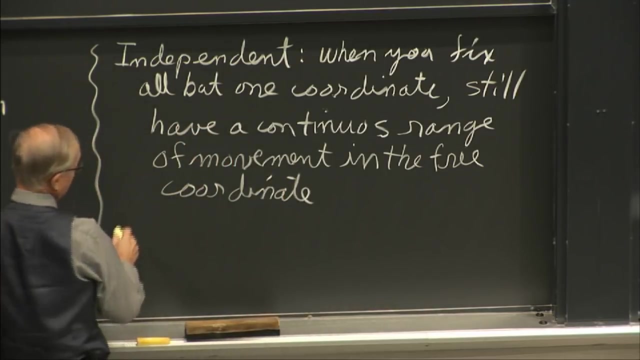 the second mass can still move. It takes two angles to define your double pendulum So independent. when you fix all but one coordinate, Still have a continuous range of movement, essentially in the free coordinate. And that's independence. And we'll do this by example mostly. 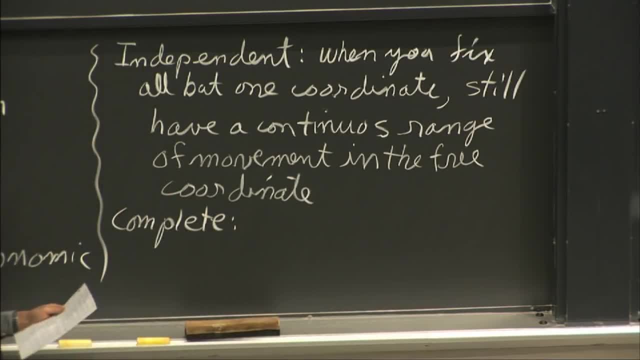 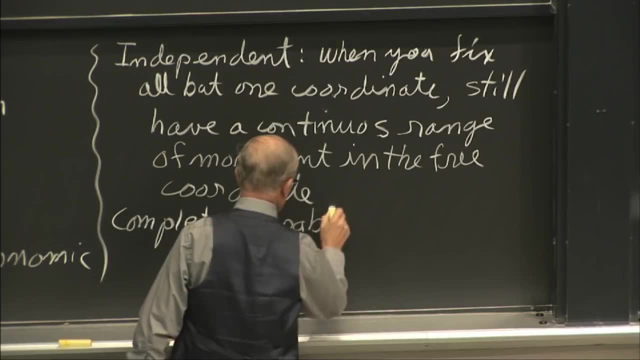 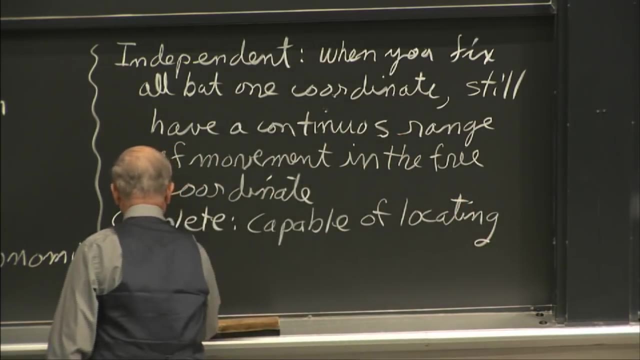 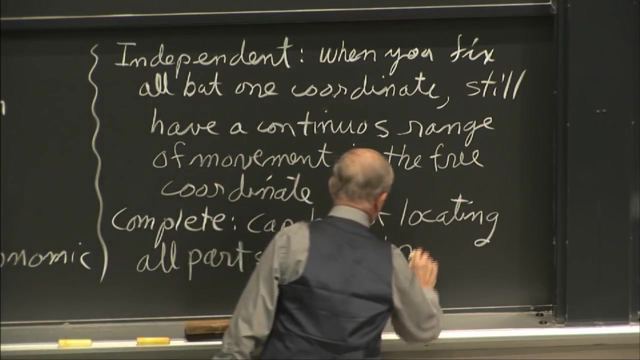 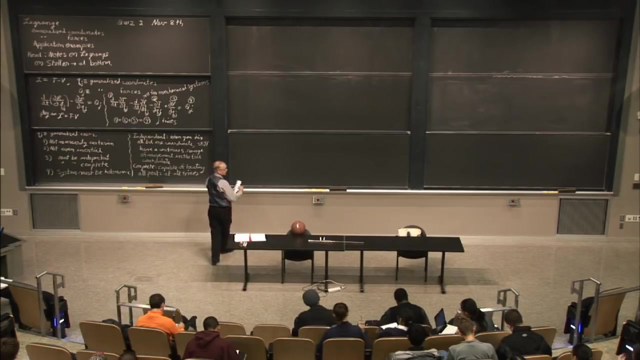 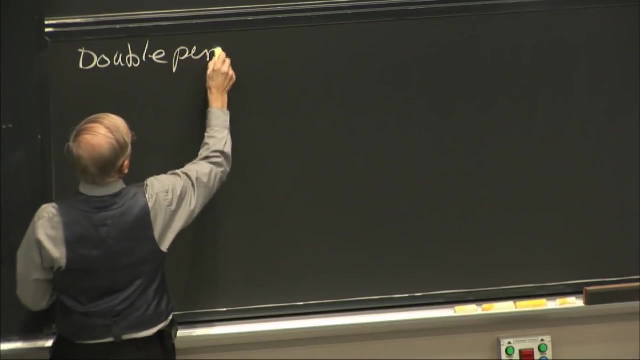 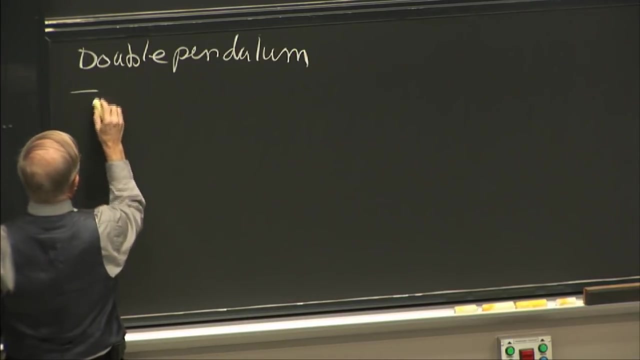 And complete really means it's capable of locating all parts of the system at all times. So let's think about it. Let's look at the system here: Double pendulum: It's a simple one, just made out of two particles and strings. 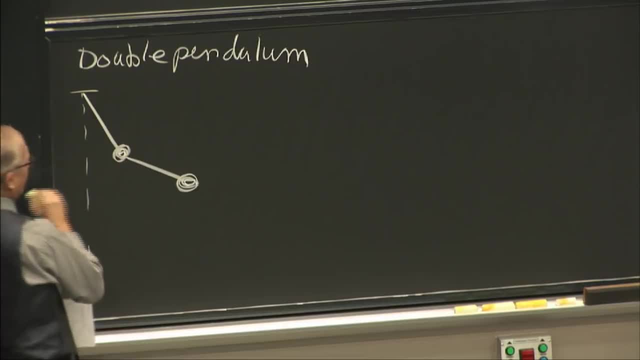 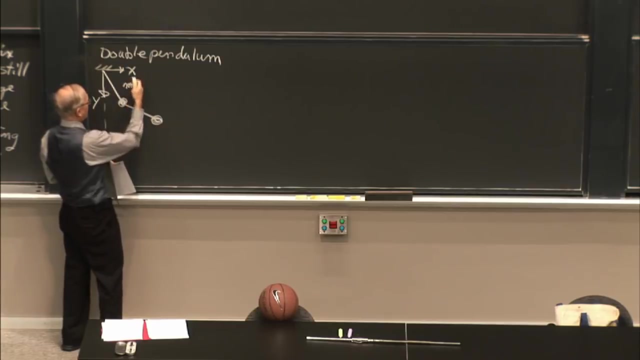 I didn't bring one today And I need to pick some coordinates to describe this And we'll put this in a. we'll use some Cartesian coordinates here, say an x and a y, And here's particle One And I can choose to describe this system xy coordinates. 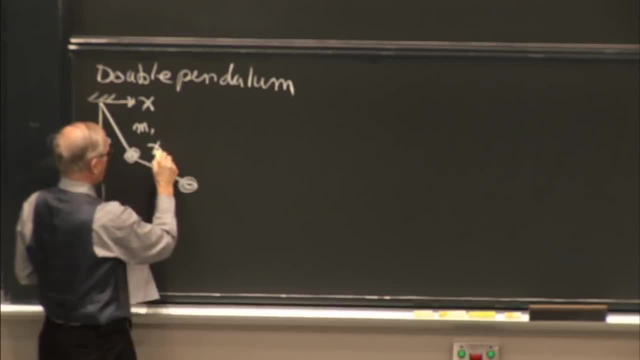 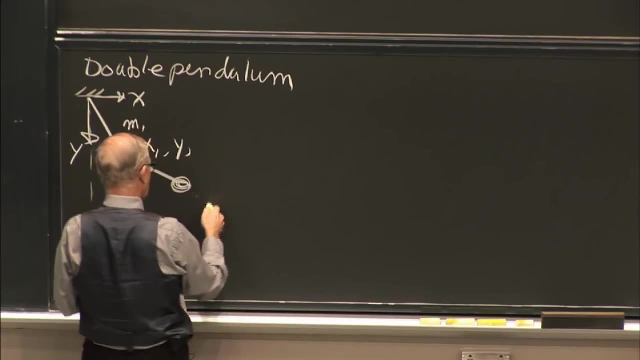 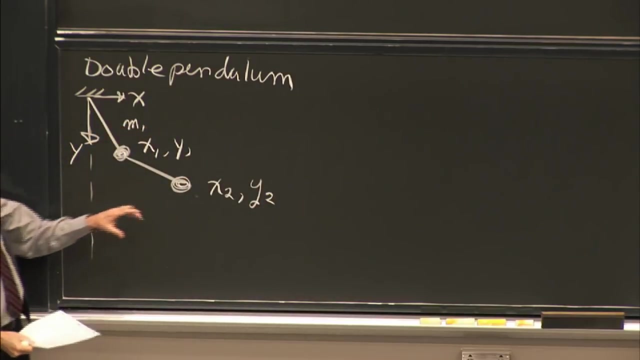 And I'll specify the location of the system with coordinates x1 and y1, two values to specify the location of that, And down here I'm going to pick two more values, x2 and y2, to describe the. so these are: x1 is a different coordinate. 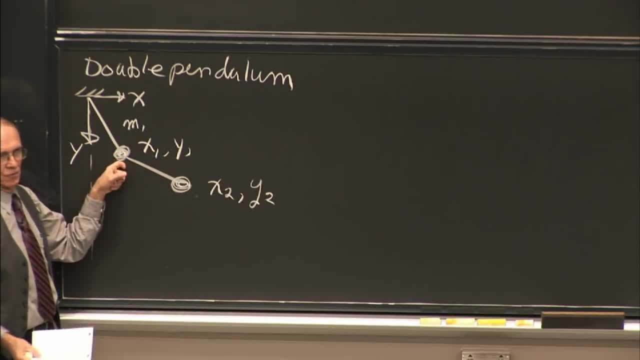 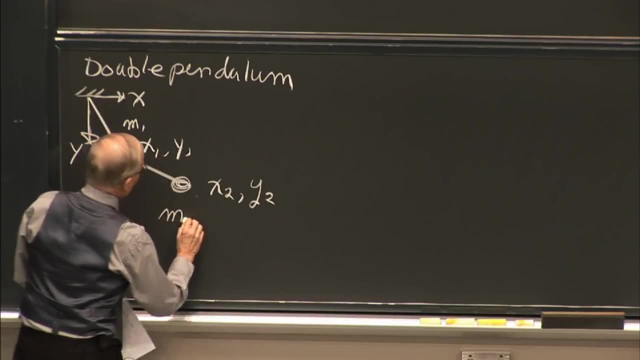 from x2.. x1 is the x position, x2 is the x position of particle one. x2 is the x position of particle two, y1 and y2.. So how many coordinates do I have to describe this system? How many have I used? 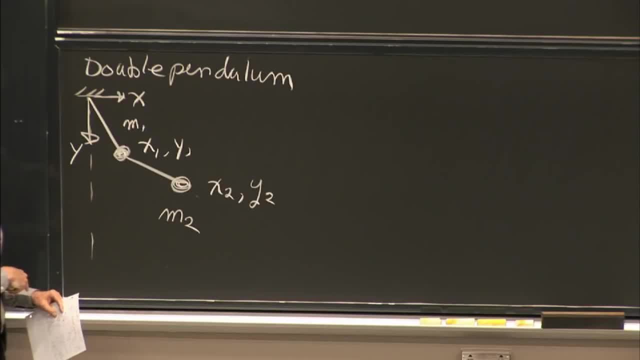 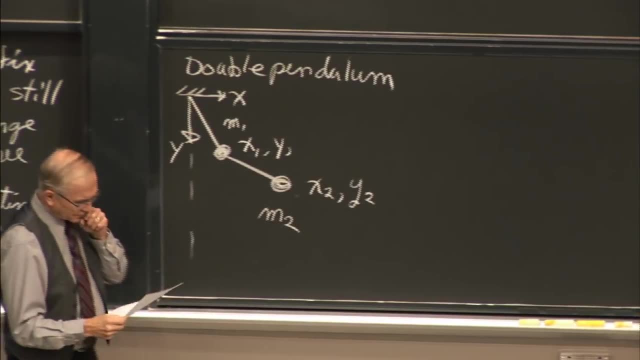 Four right. How many degrees of freedom do you think this problem has? Two right, So there's something already a little out of whack here. OK, But the point is, These Aren't independent, you'll find. You just do a test. 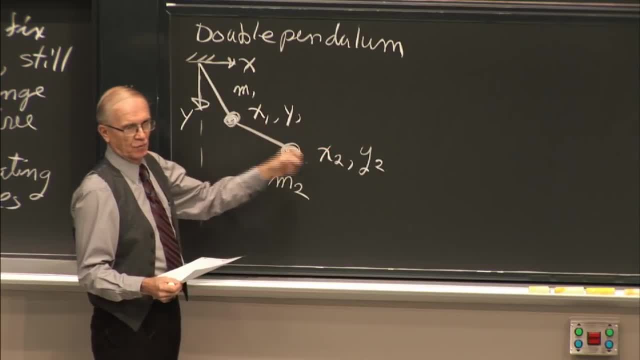 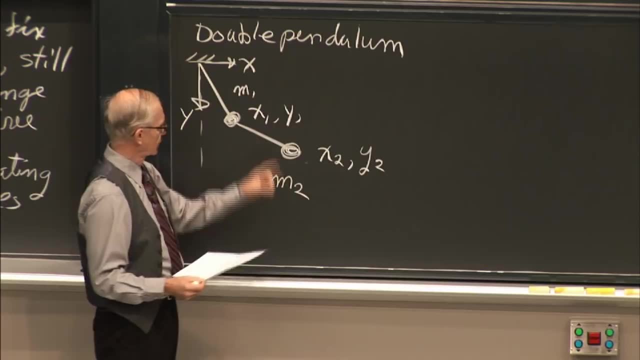 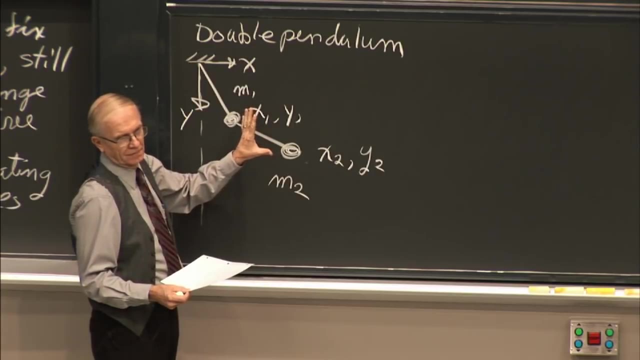 You'll find that these aren't independent. If I fix x1 and x2, the system doesn't move right. I say this has got to be one and this has got to be three. This system is now frozen. So this system of core coordinates. 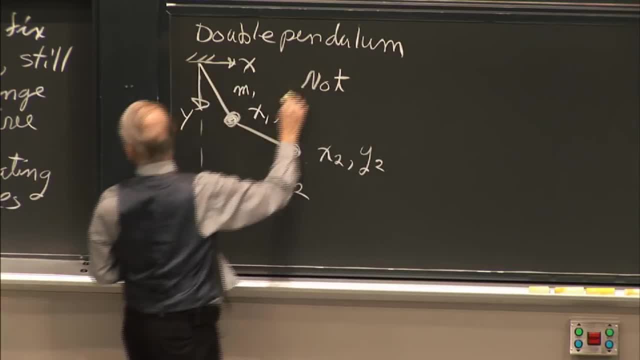 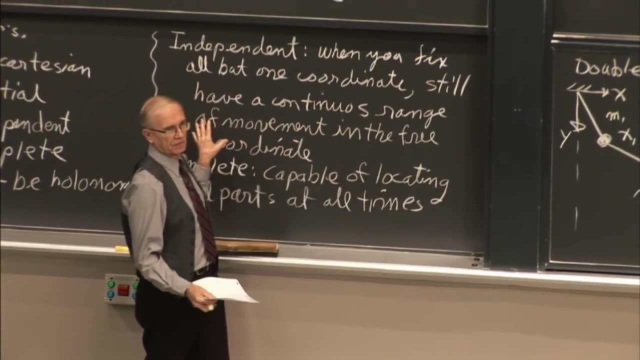 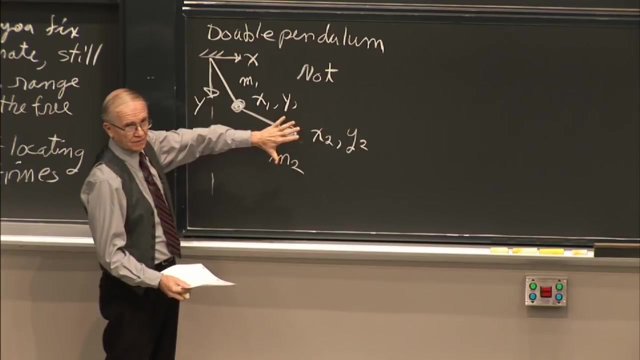 is not independent. What do we say Independent? Independent When you fix All But one coordinate is still have continuous range of movement. of the final one, I can fix only just two of these and I've frozen the system. I don't even have to go to the extent of fixing three. 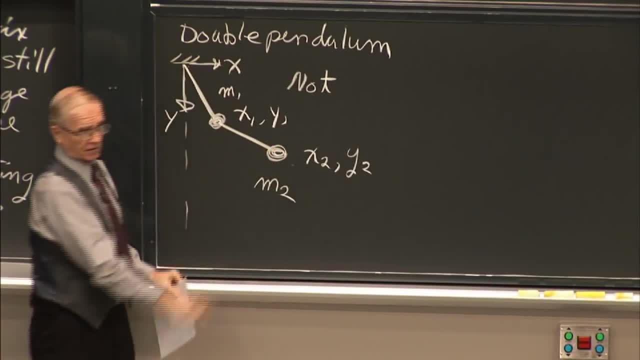 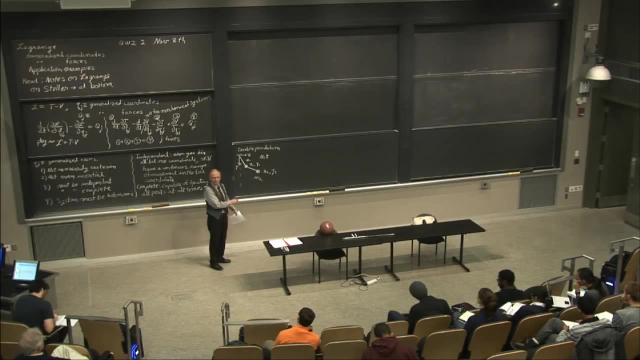 I'm assuming the strings are of fixed length. You can't change the string length. OK, So this is not a very good choice of coordinates And we had a hint that it might not be, because it's more than we ought to use. 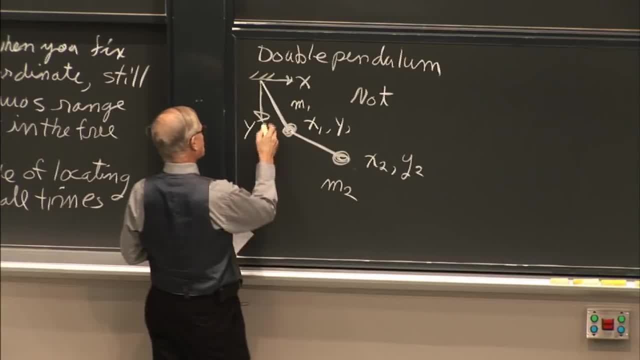 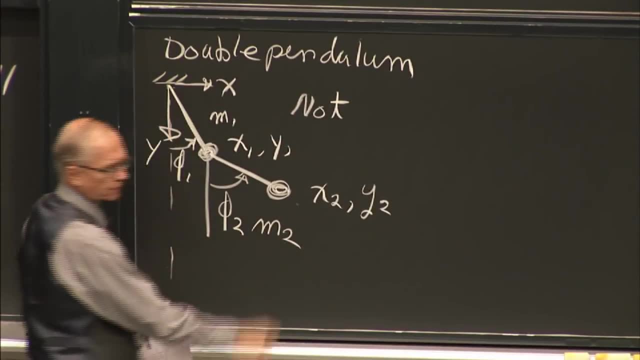 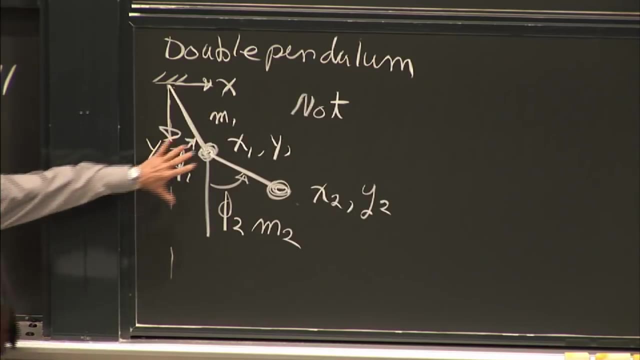 We only really need two, OK, And then if we choose these angles, phi 1 and phi 2, let's do the test with that- Are those independent? So those are the coordinates of the system. If you fix phi 1, is there still free and continuous movement? 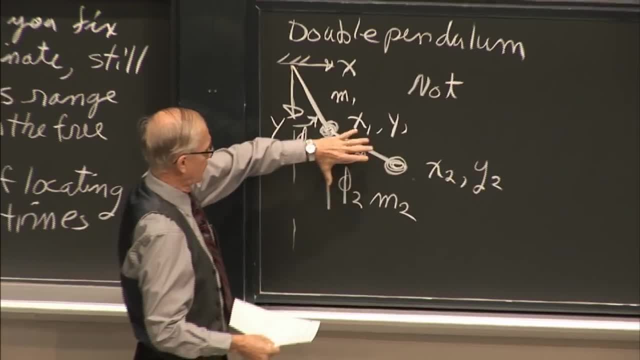 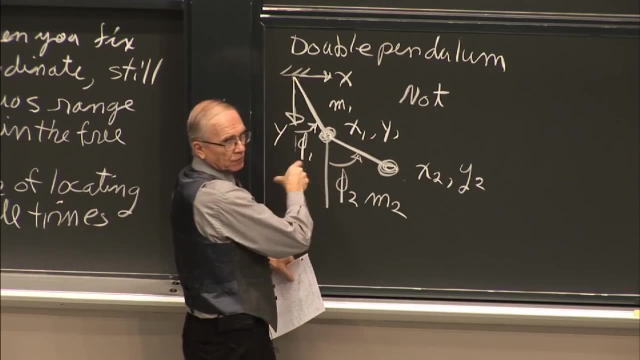 of phi 2 of the system. Sure, And if you fix phi 2, it means you can require this angle. stay rigid like that And move phi 1,. well, the whole system will still move. So phi 1 and phi 2.. 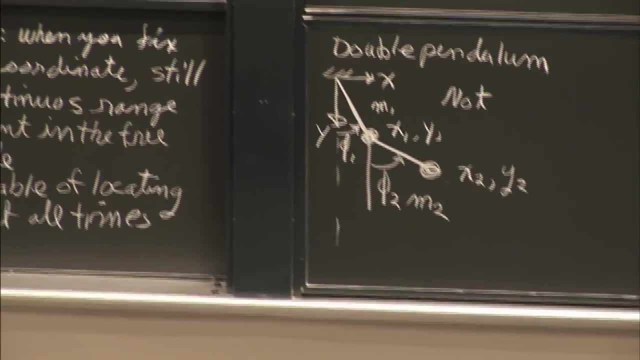 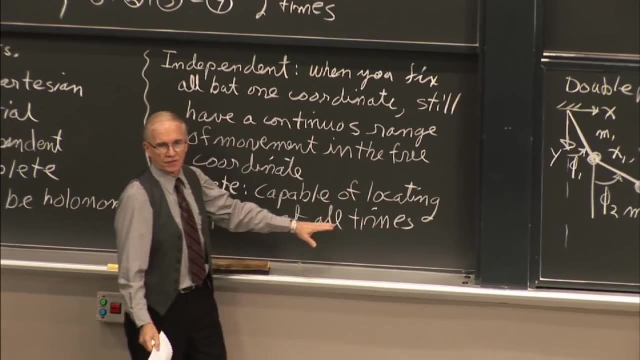 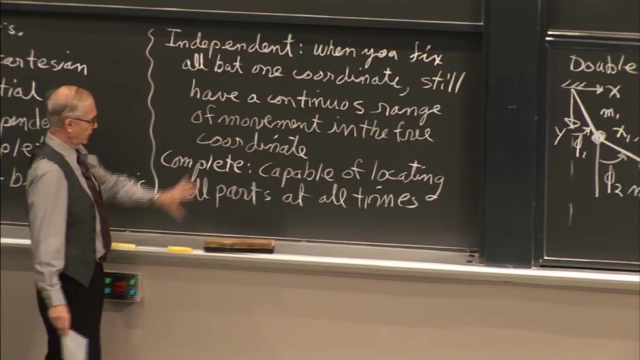 And phi 2 are a system which satisfies the independence requirement- Complete. They're both systems that are complete. They're both capable of locating all points at all times. But only the pair phi 1 and phi 2 in this example are both independent and complete. 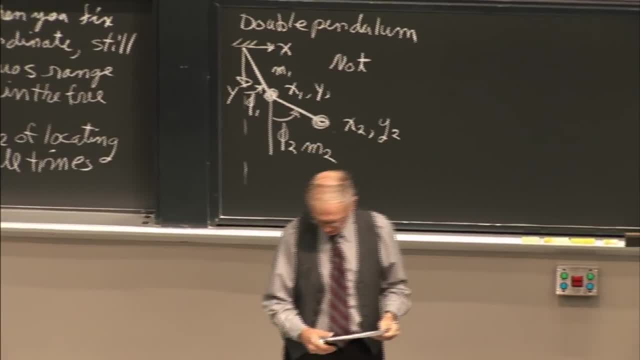 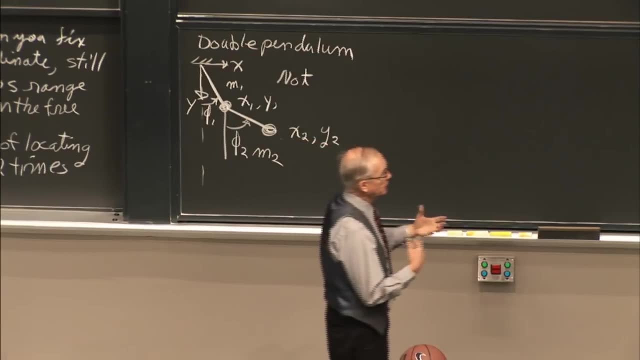 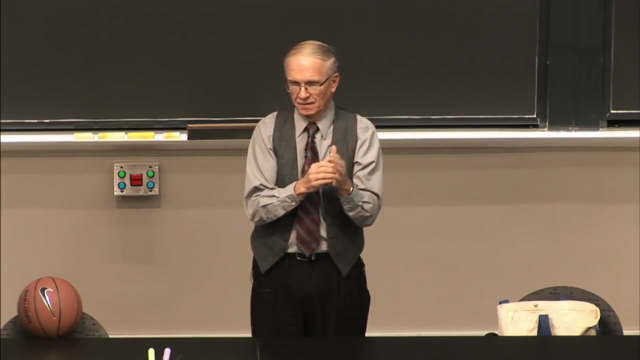 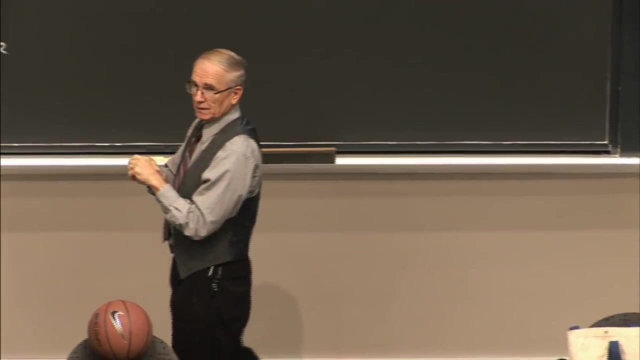 Now the third requirement is this thing called holonomic. Holonomicity, And what it means to be holonomic is that the system, the number of degrees of freedom required, is equal to the number of coordinates required to completely describe the motion. Now, most of the time, every example, 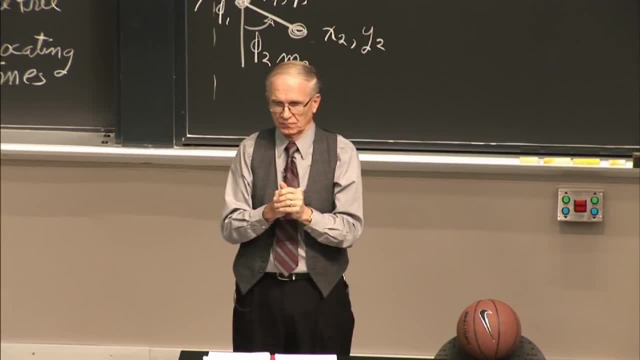 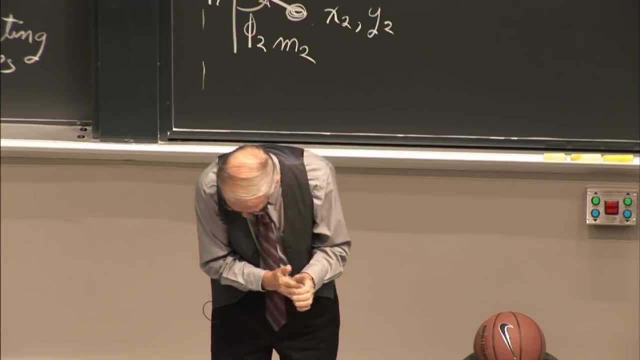 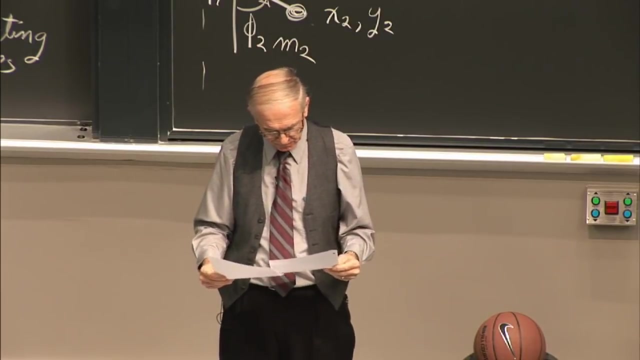 we've ever done so far in this class satisfies that We pick phi 1 and phi 2. And that's all the coordinates that we need to completely describe the motion. Let me see if I can figure out a counterexample. I didn't write down this definition. 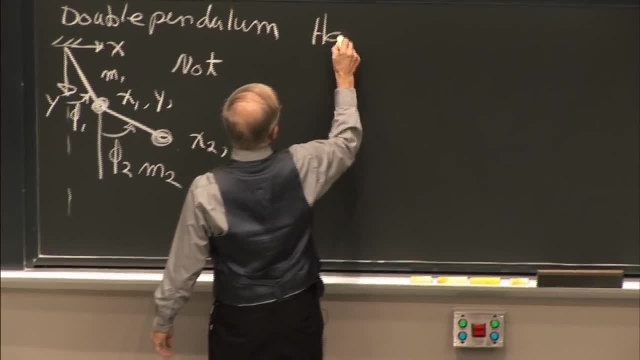 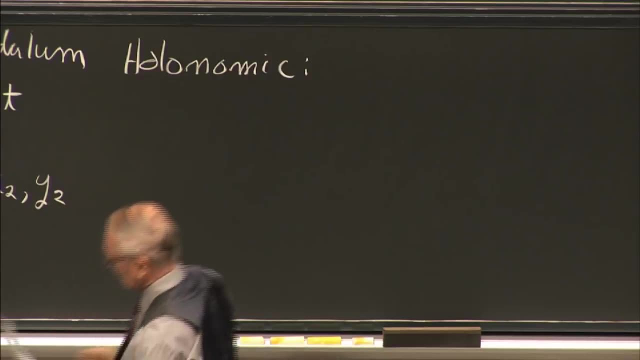 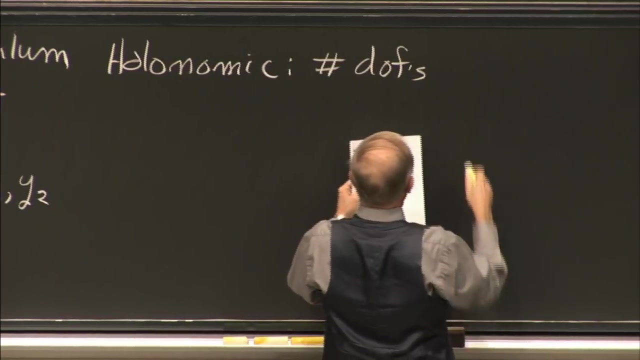 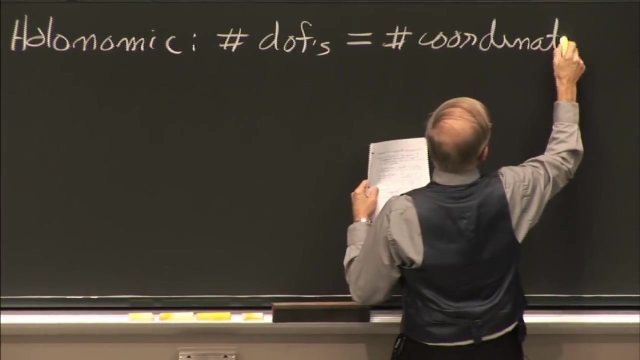 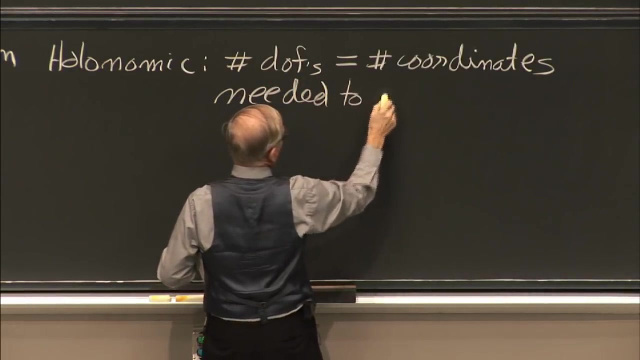 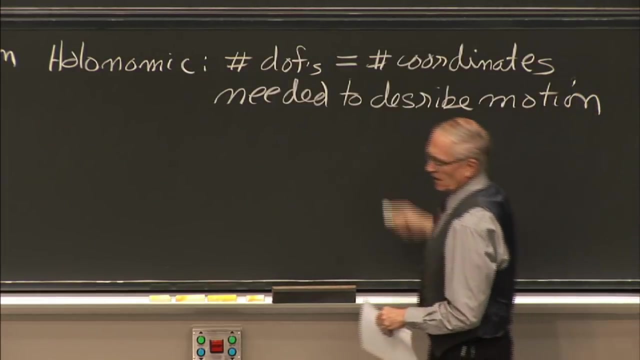 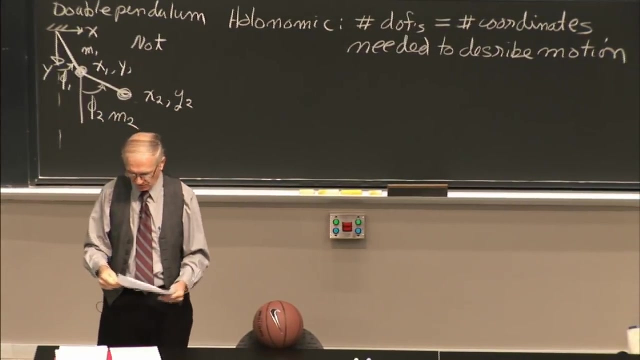 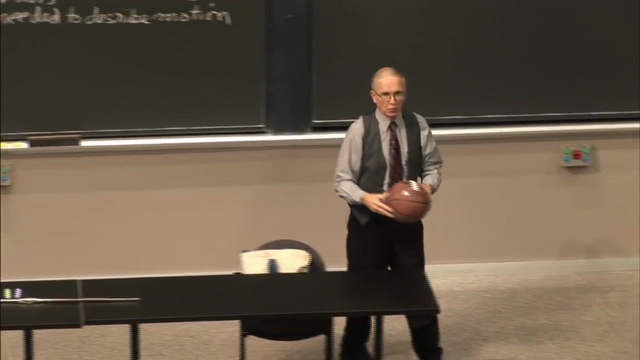 So holonomic? And if the answer to this question is no, you cannot use Lagrange equations. OK, OK, OK, OK, OK. So let's see if I can show you an example of a system in which you need more coordinates than you have degrees of freedom. 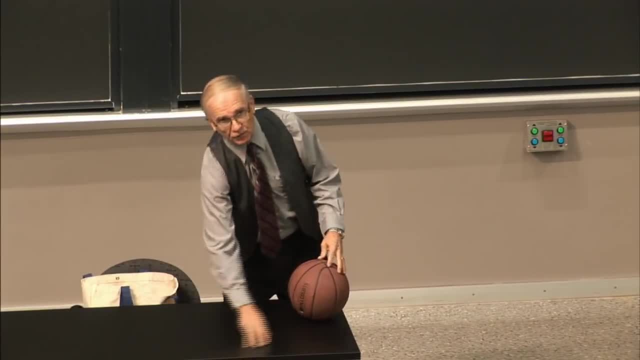 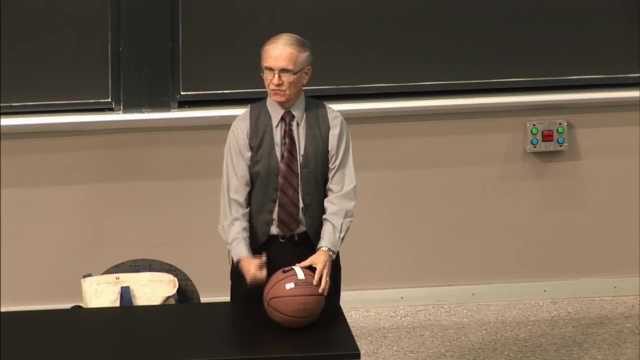 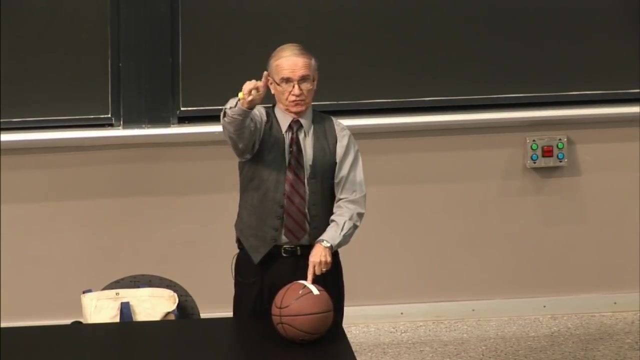 I've got a ball. This is an xy-plane And I'm not going to allow it to translate in z And I'm not going to allow it to rotate about the z-axis. OK, So those are two constraints, right? So this is one rigid body. 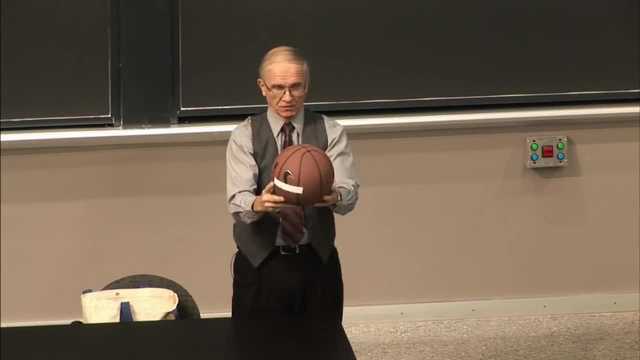 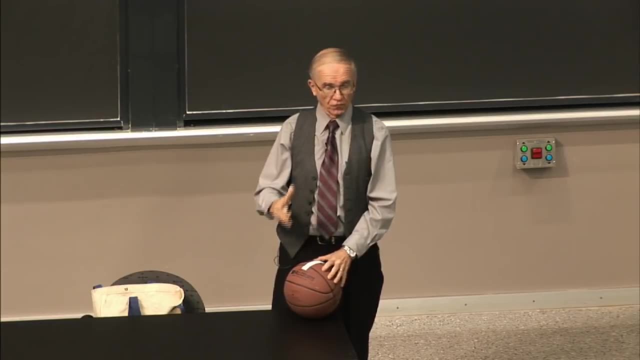 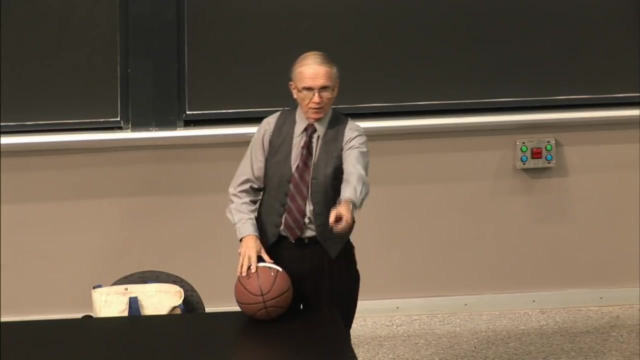 In general. how many degrees of freedom does it have? Six, OK, I'm going to constrain it. So no z-motion Five, No z-rotation Four. It's not going to allow it to slip. This is x and that's y. 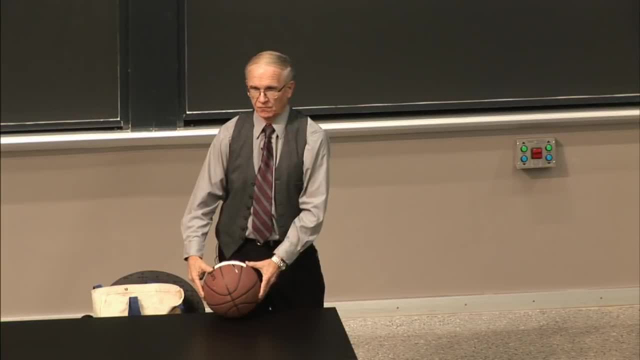 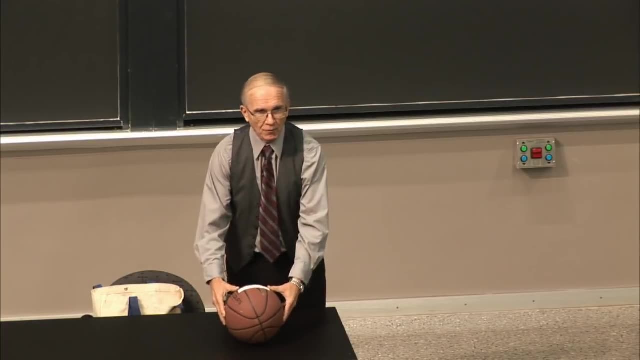 I'm not going to allow it to slip in the x. So now I've got another, That's one. Now I'm down to three And I'm not going to allow it to slip in the y Two. So by our calculus of how many degrees of freedom you need, 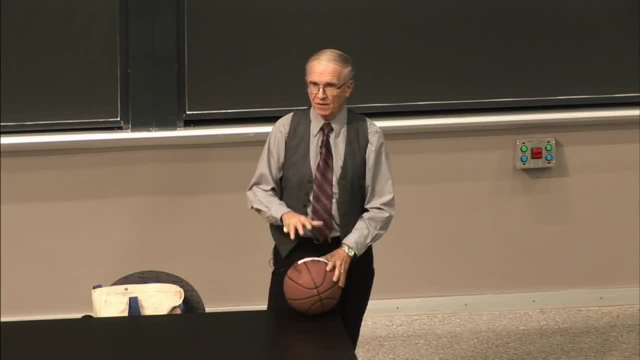 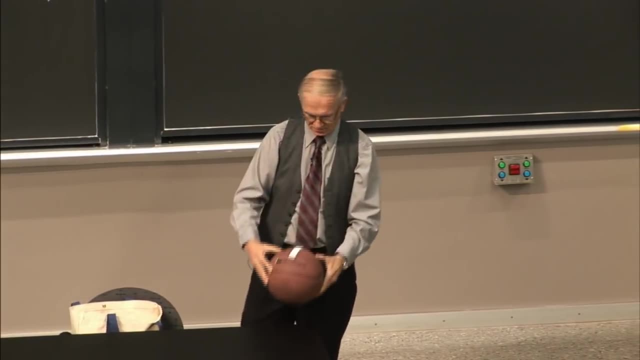 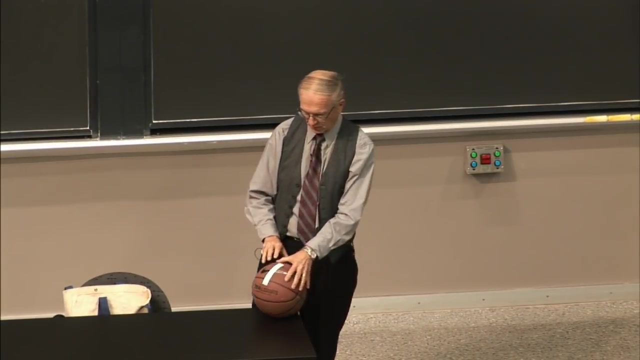 we're down to two, We should be able to completely describe the motion of this system with two coordinates. OK, So I've got this piece of tape on the top And it's pointing diagonally that way And I'm going to roll this ball. 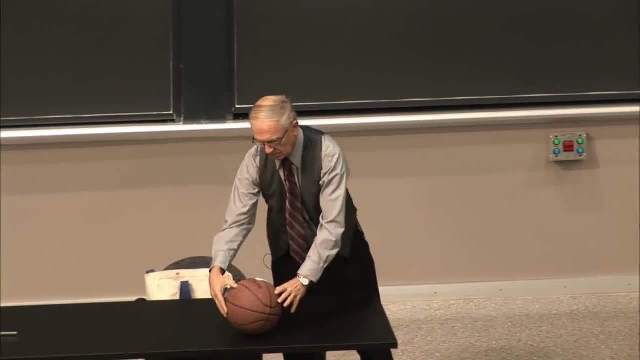 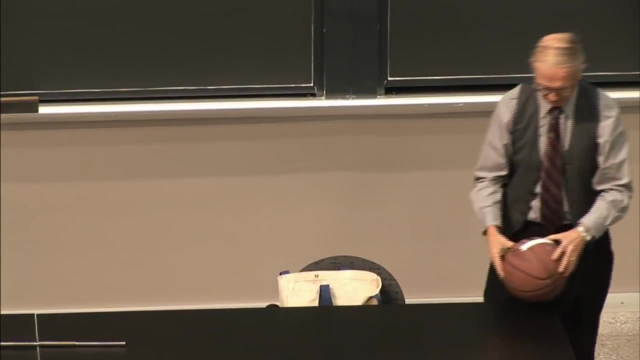 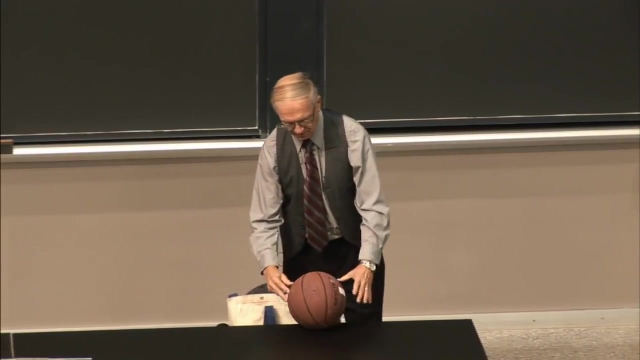 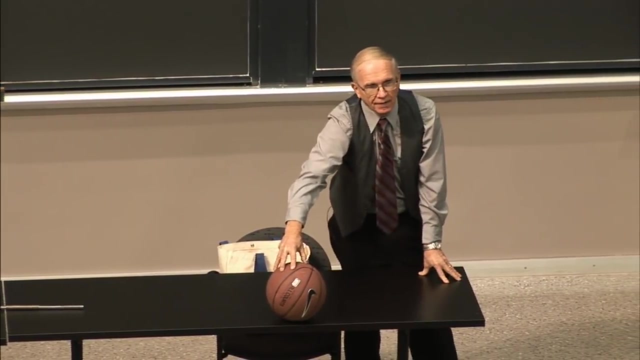 OK, Like this until it shows up again. So it's right on top, just the way it started. OK, Now let's start off the same way again. I'm going to roll first this way, and then I'm going to roll this way to the same place. 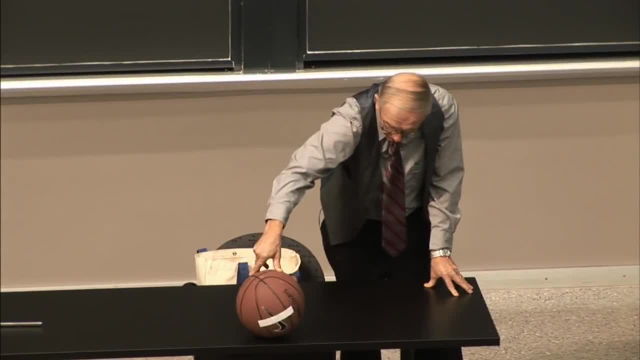 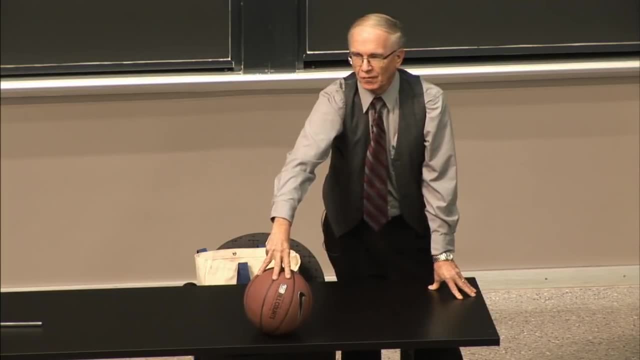 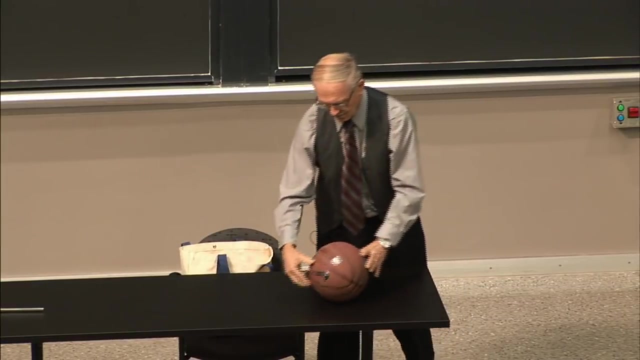 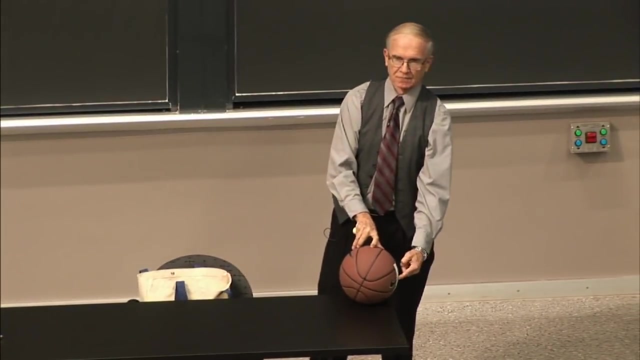 Where's the stripe? It's in the back. So I've gone to the same position, But I've ended up with the ball not in the same orientation as it was. I went by two different paths And the ball comes out over here. 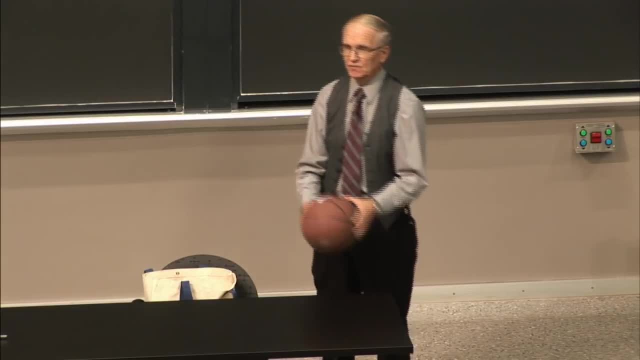 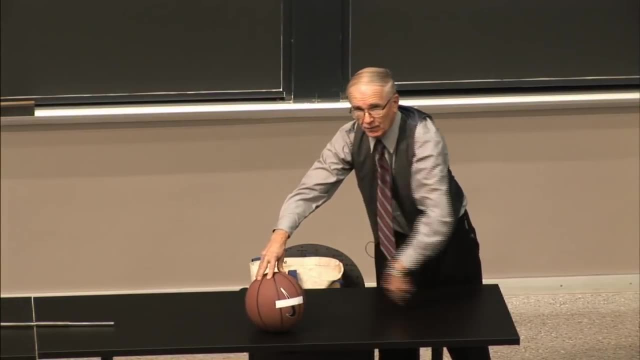 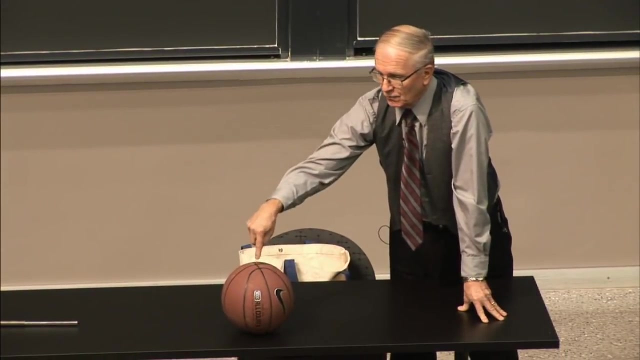 rather than up there where it started. OK, So this system to actually describe where the ball is at any place out here, having gotten there by running around, rolling around without slipping and without z rotation, how many coordinates do you think it'll take to actually specify? 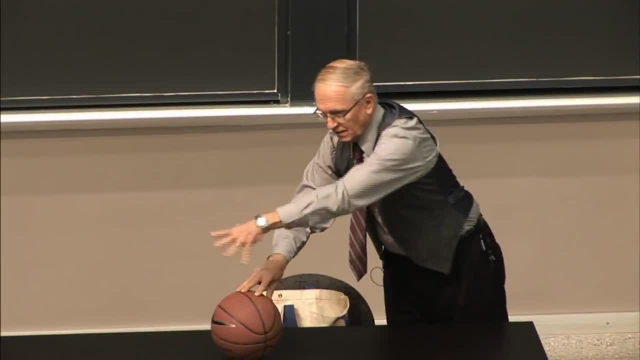 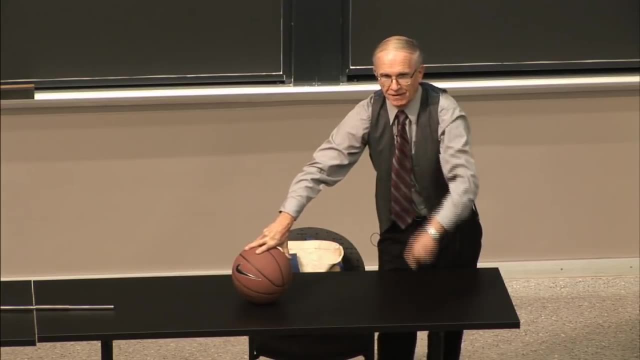 where that stripe is at any arbitrary place that it's gotten to on the plane, Name them. It seems to be moving to x. It seems to be moving to y in rotation. So In order to actually fully describe it, you've got to say where it is x and y. 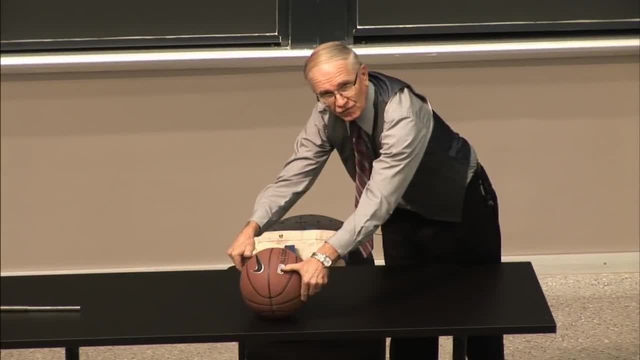 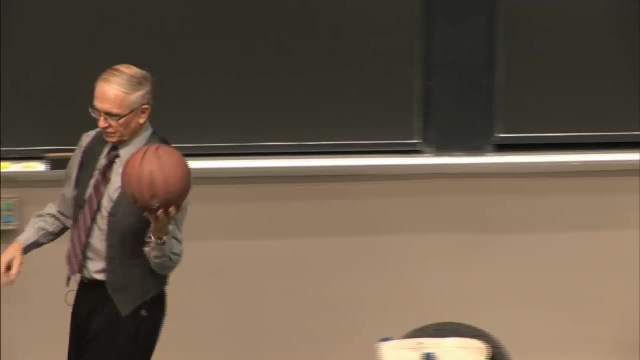 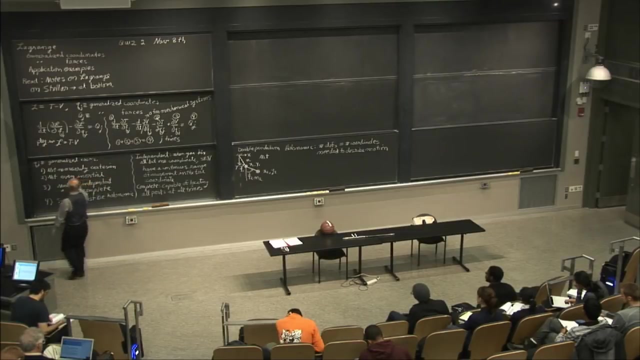 And you actually have to say some kind of theta and phi rotations that it's gone through, so that you know where this is OK. So this system is not holonomic And holonomic. it has to be holonomic in order to use Lagrange equations. 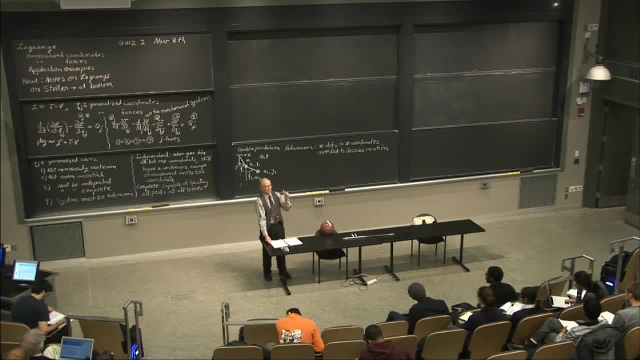 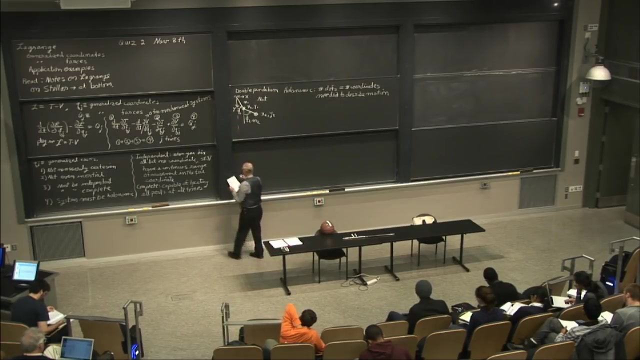 So when you go to do Lagrange problems, you need to test for it. your coordinates OK, Complete, independent and holonomic, And you get pretty good at it. So here's my Lagrange equations and I've itemized these. 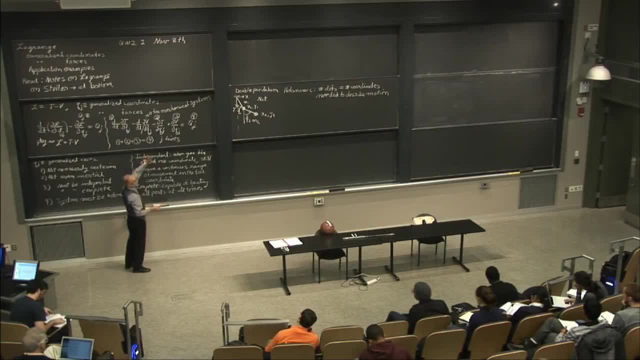 Four calculations you have to do. Call them 1,, 2,, 3, and 4.. And so what I want to write out is just to show you, just to get you to adapt, a systematic approach to doing Lagrange. So left-hand side. 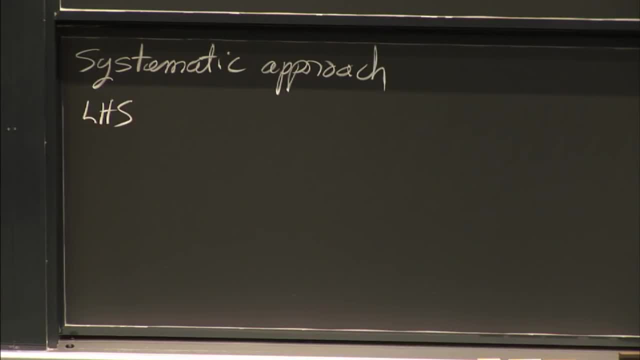 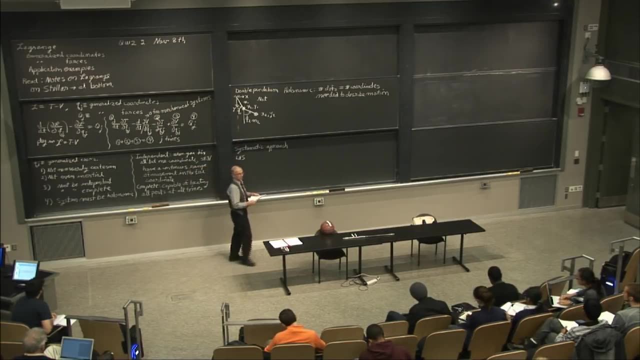 So the left-hand side of your equations of motion is everything with t and v. The right-hand side has these generalized forces that you have to deal with, And the generalized forces are the non-conservative forces in the system. OK, So this is going to get a little bit cookbooked. 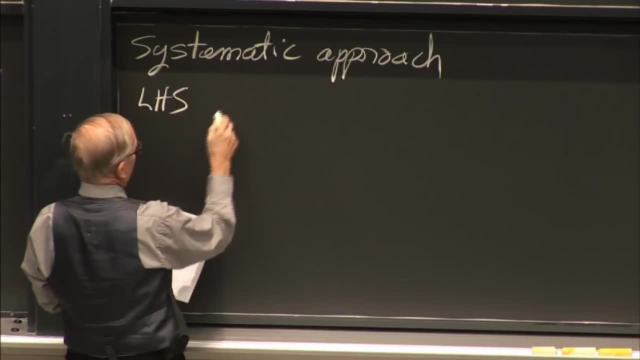 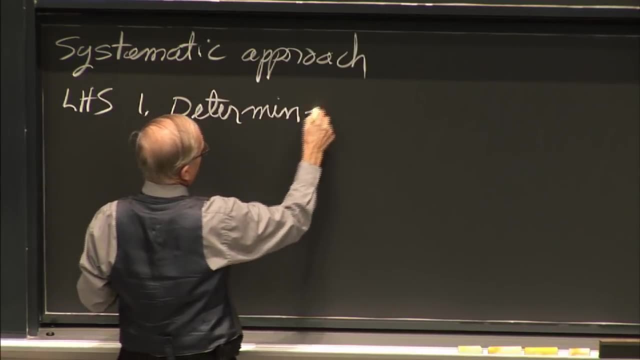 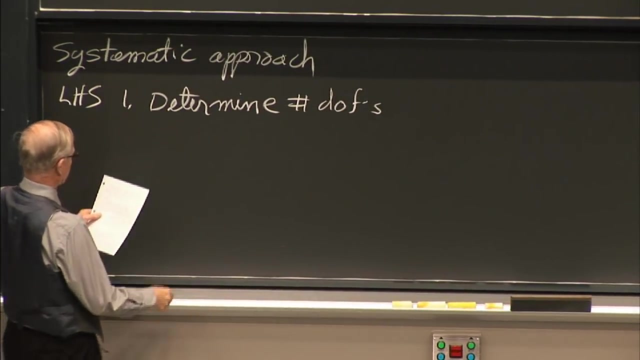 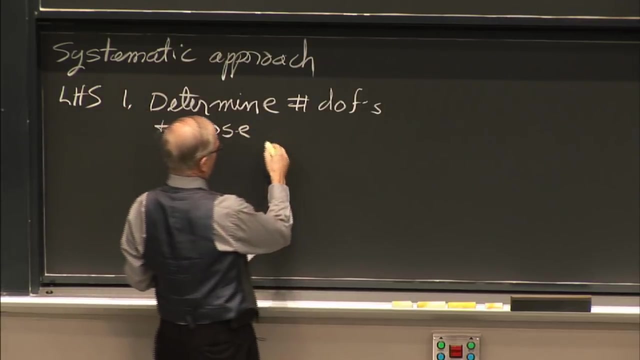 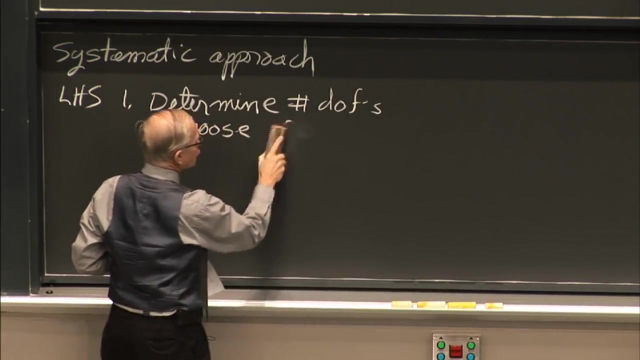 but it's, I think, appropriate for the moment here. So, step one: Determine the number of degrees of freedom that you need And choose your delta j's. Those are your, not deltas, excuse me, just qj's. Choose your coordinates. 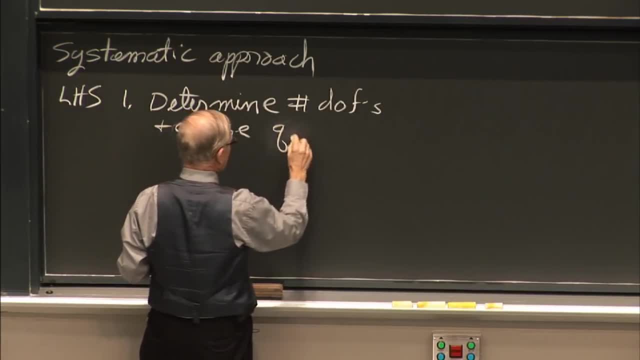 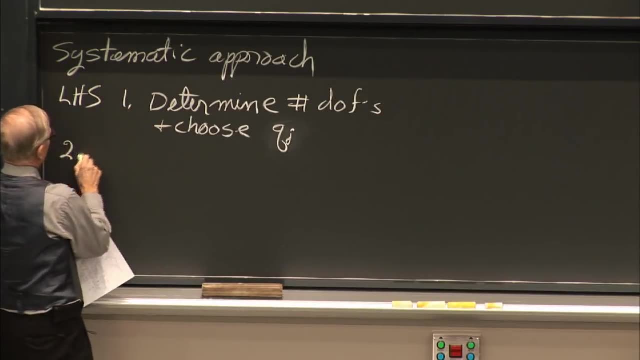 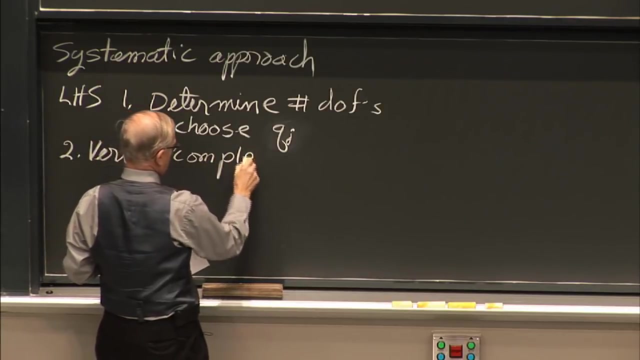 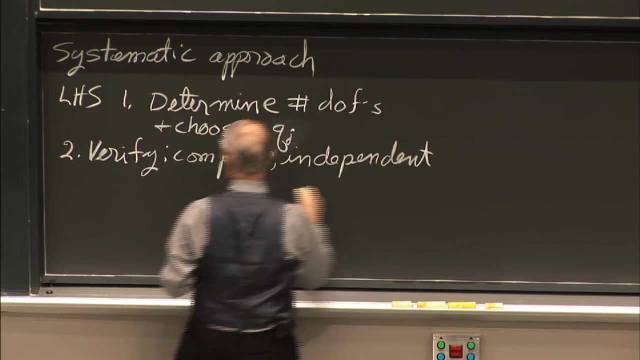 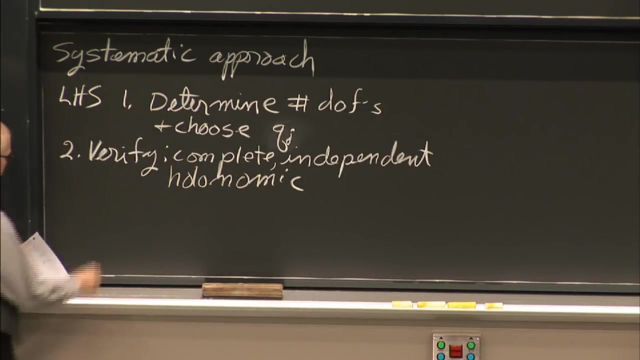 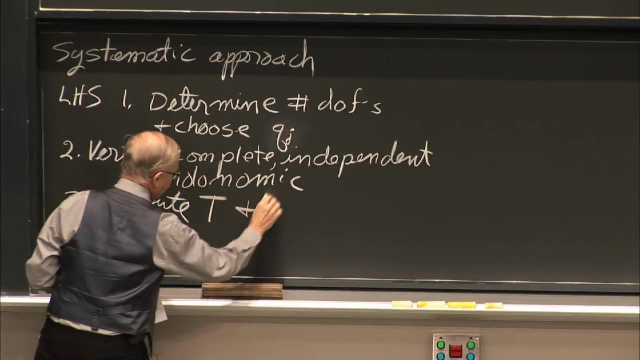 You find the number of degrees of freedom and choose the coordinates you're going to use. basically, Verify Complete, independent, holonomic Three Compute- t and v for every rigid body in the system. Compute your kinetic and potential energies. 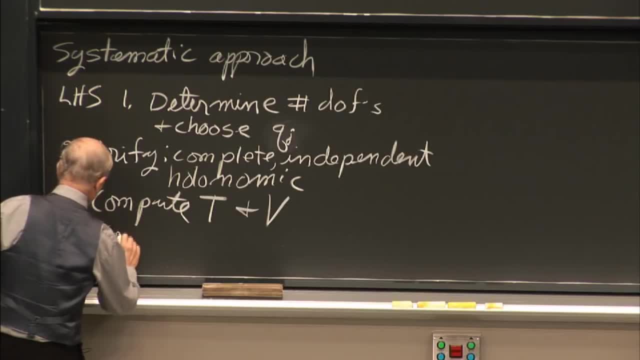 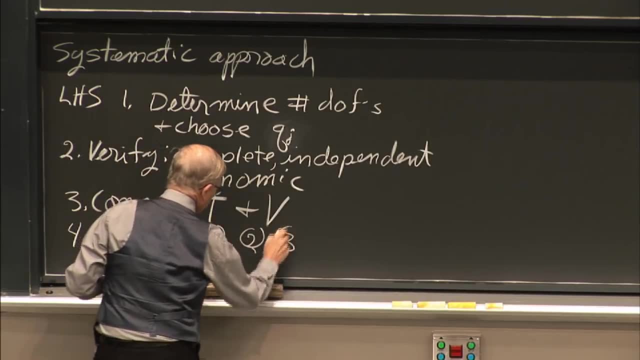 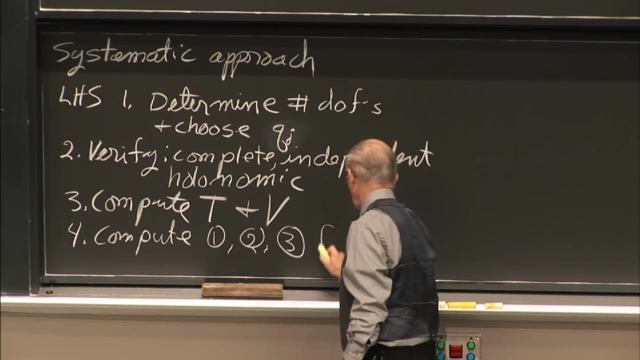 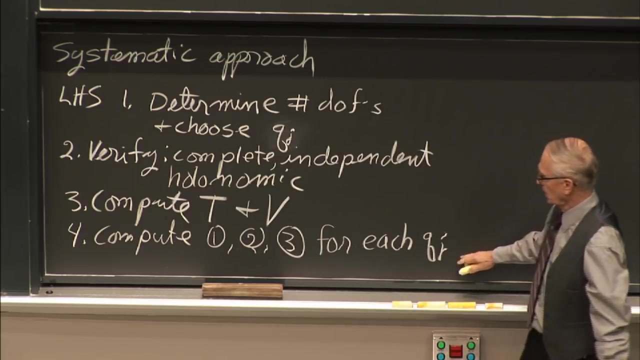 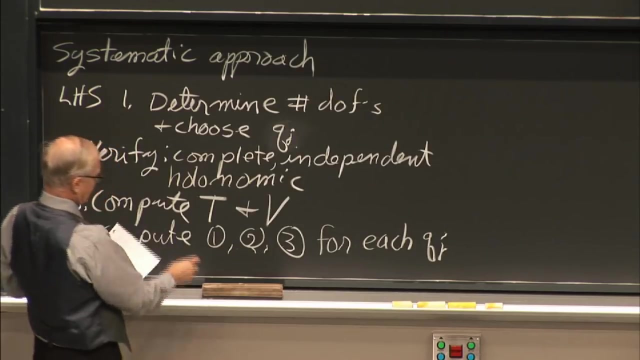 One, two, three for each qj. So for every coordinate you have you have to go through these computations: One, two, three, four for every coordinate. And this is your left-hand side. And if you don't have any external forces, 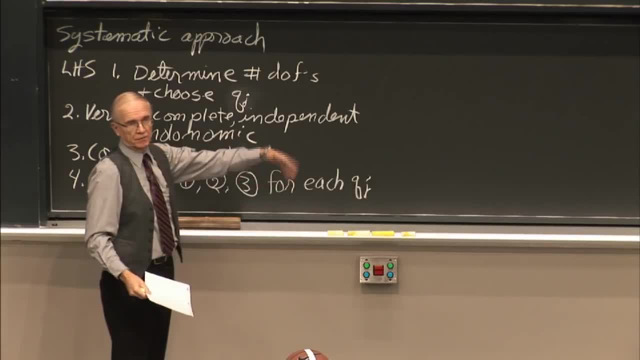 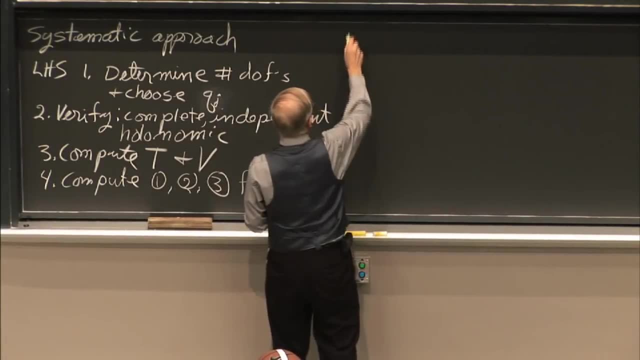 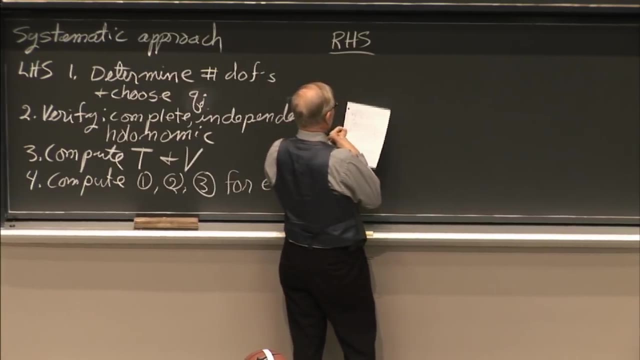 any non-conservative external forces, then 1 plus 2 plus 3 equals 0. But if you have non-conservative forces, then you have to compute the right-hand side. So the right-hand side, So for e to the power of t. 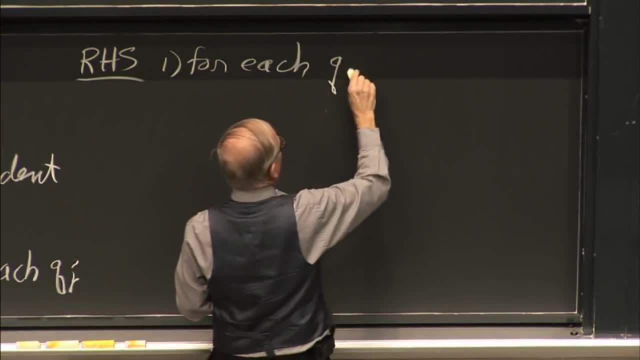 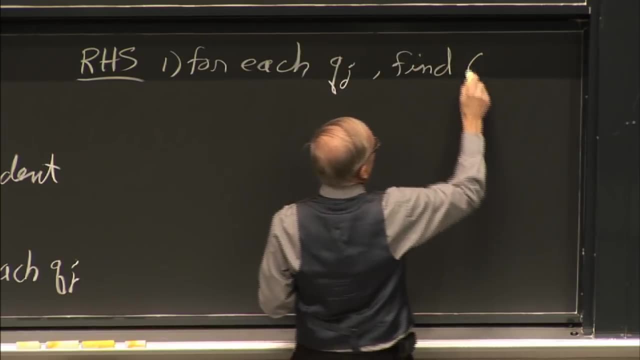 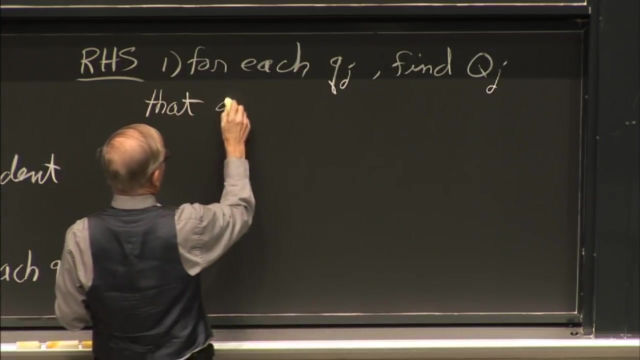 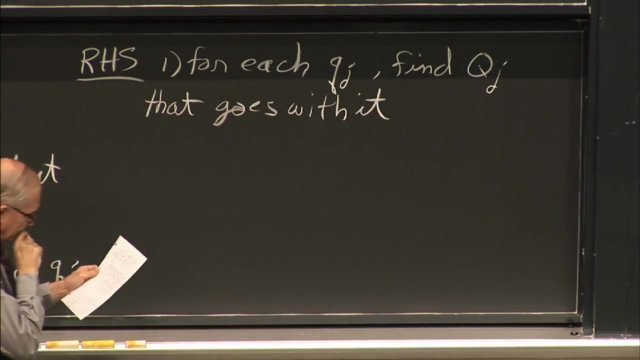 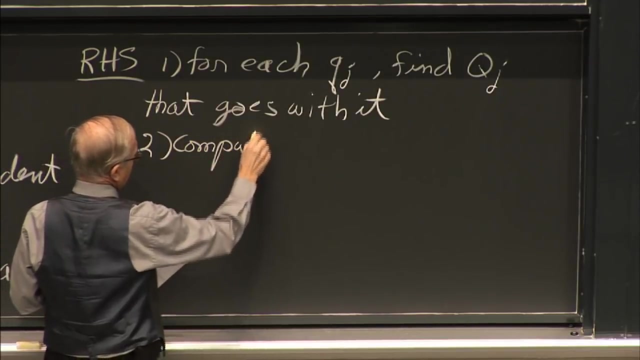 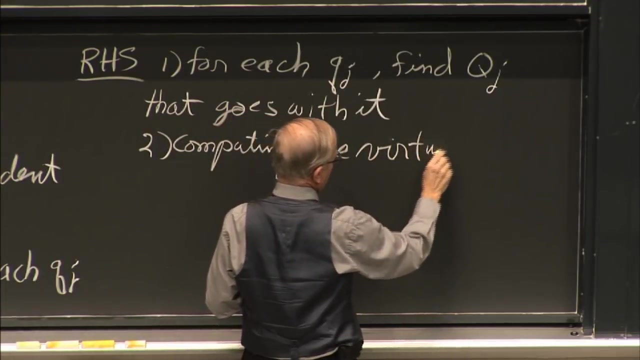 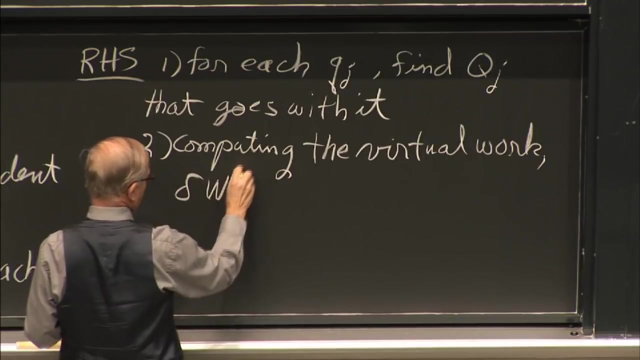 So for e to the power of t, So for e to the power of t. Each qj, each generalized coordinate, you need to find the generalized force that essentially goes with it, And you do this by computing The virtual work, delta w. I'll put the little nc up here. 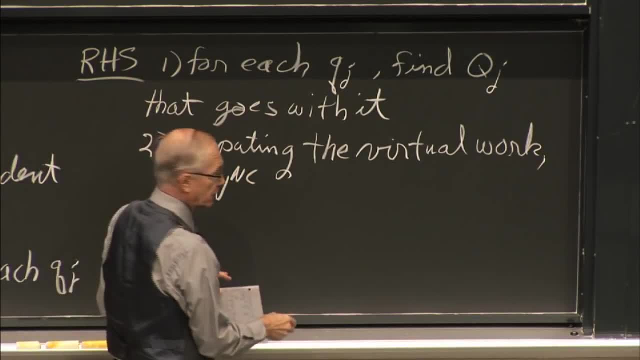 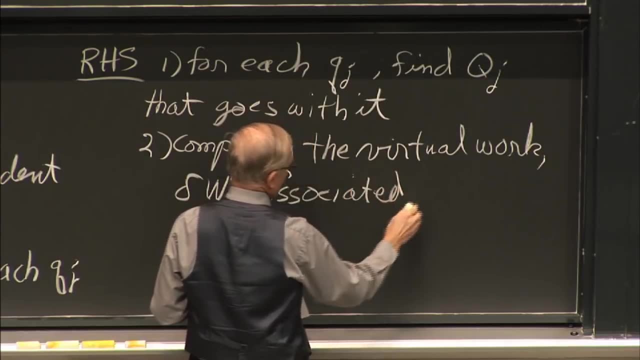 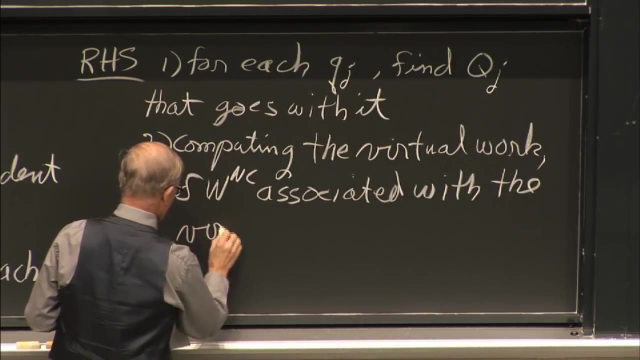 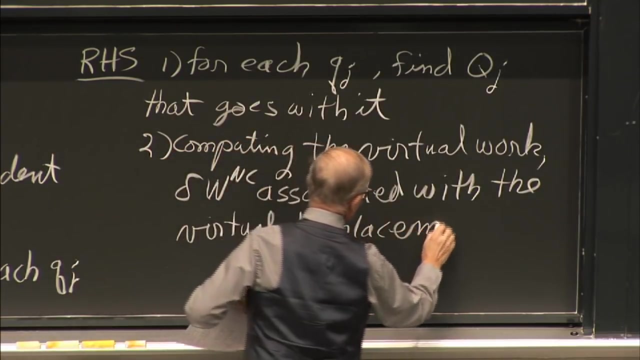 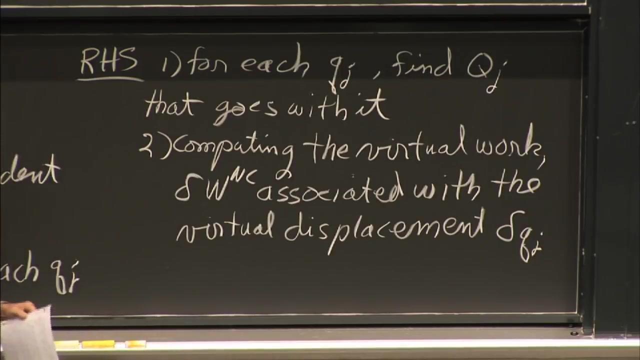 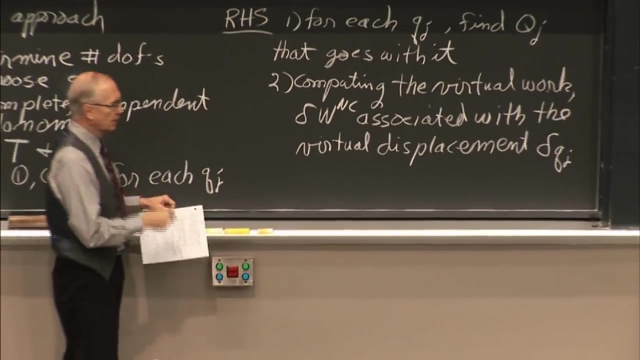 to remind you, these are for the non-conservative forces, The delta w associated With the virtual displacement delta qj. So for every generalized coordinate you have, you're going to try out this little delta of motion in that coordinate and figure out how much. 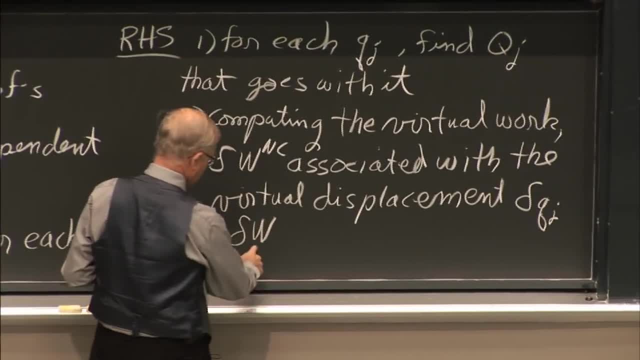 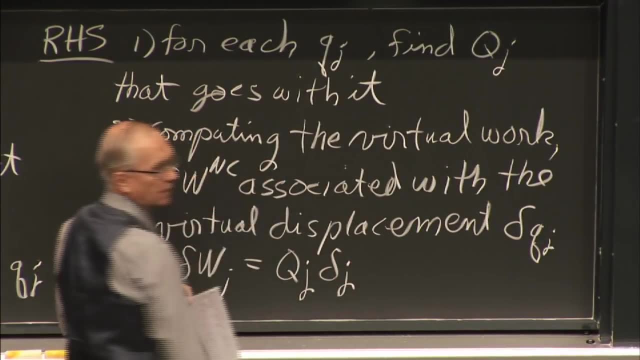 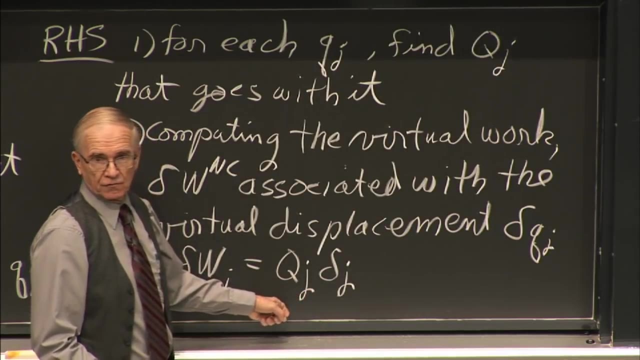 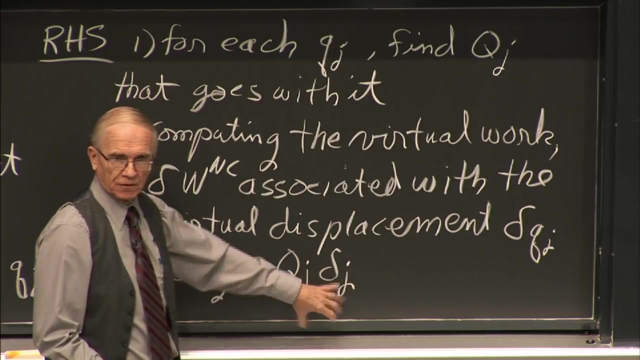 The virtual work you've done. So delta wj is going to be qj, delta j. This is the thing you're looking for And it's going to be a function of all those external non-conservative forces acting through a little virtual displacement. 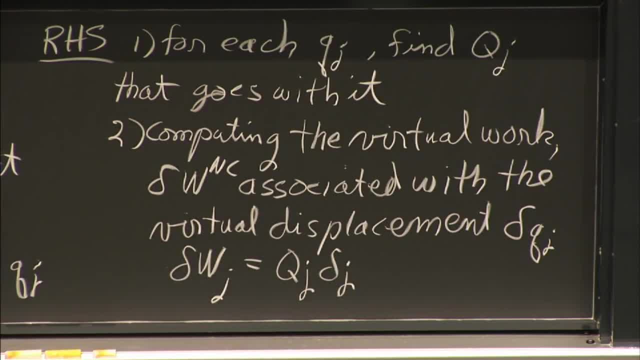 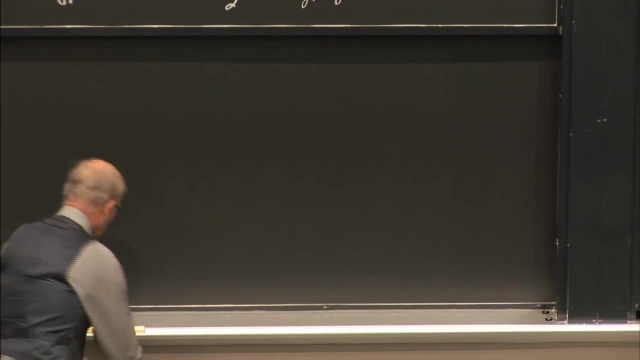 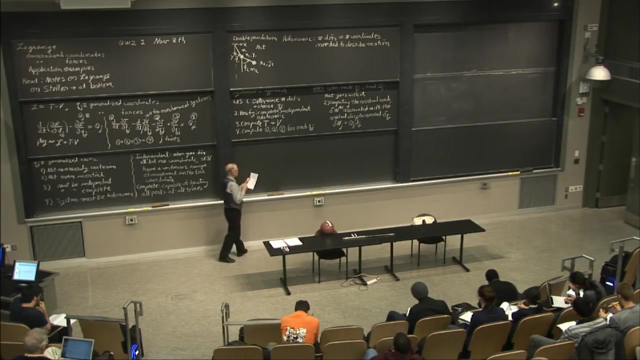 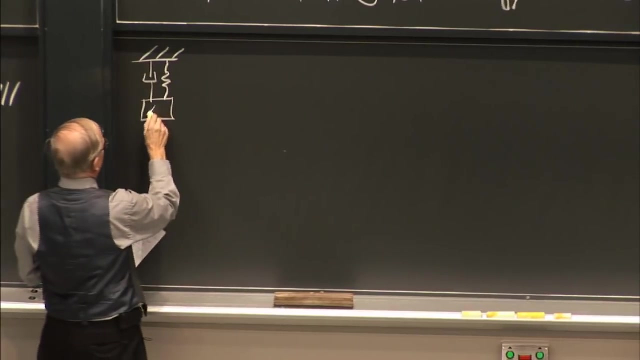 A little bit of work will be done. Mostly, I'm going to teach you how to do this by example. So let's quickly do a really simple, trivial system, Our mass spring Dashpot system. Single degree of freedom: m, k, b. 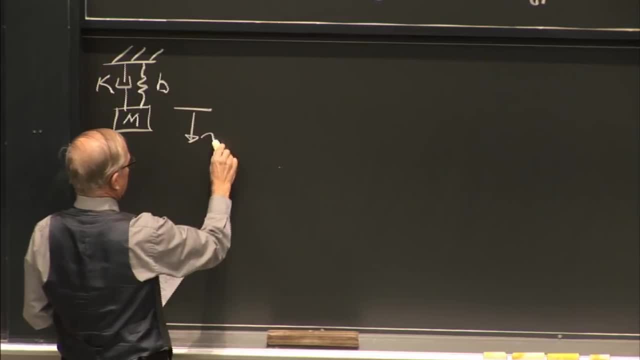 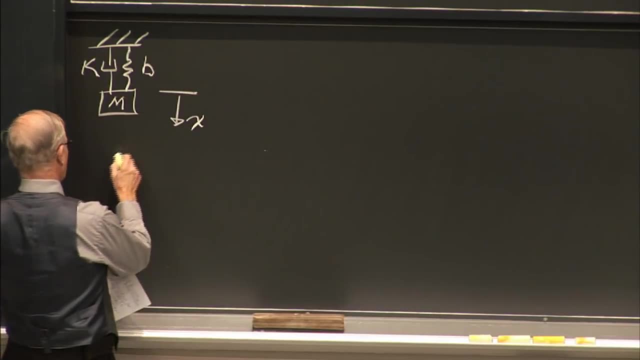 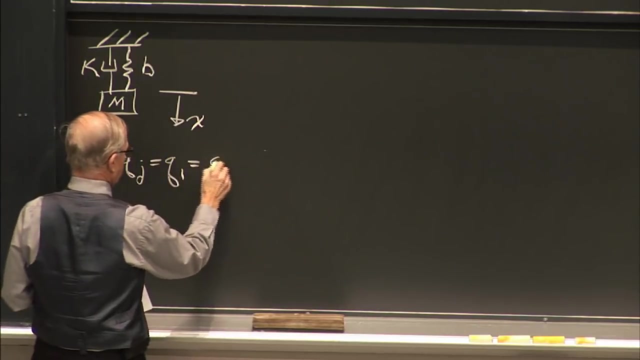 It's going to take one coordinate to describe the motion. x happens to be Cartesian. There'll be one generalized coordinate. So qj equals q1 equals qx. in this case, It's our x coordinate. Actually, Let's just call it x. 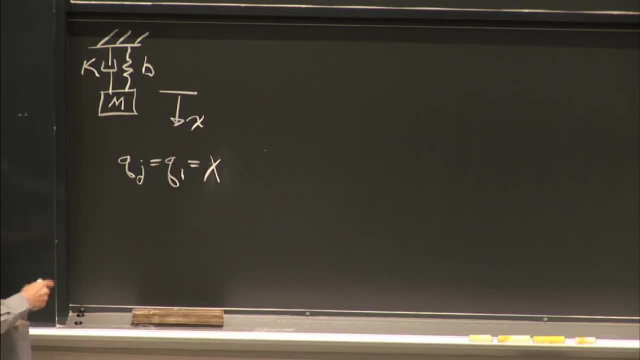 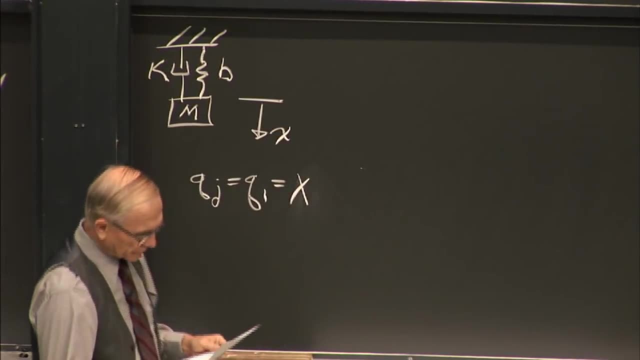 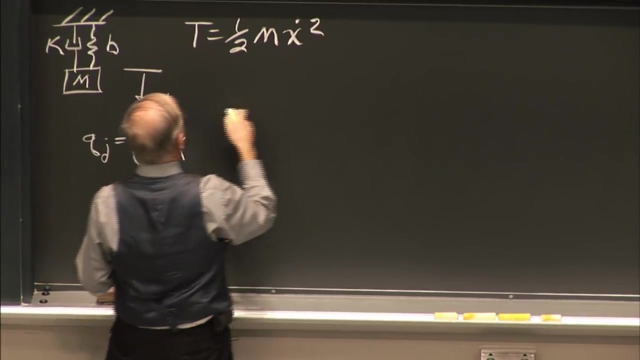 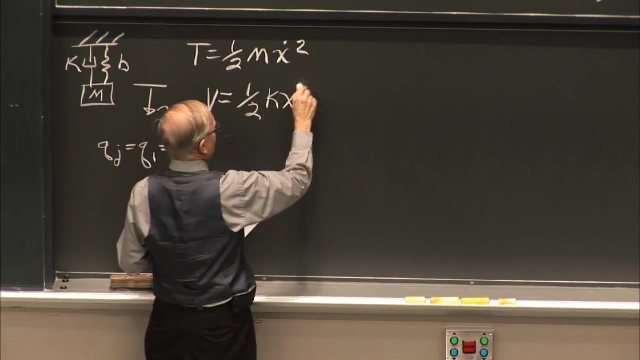 That's our generalized coordinate for this problem. Is it complete? Yep. Is it independent? Yes. Is it holonomic? No problem. We need t, 1 half m x dot squared, We need v And we have 1 half k x squared for the spring. 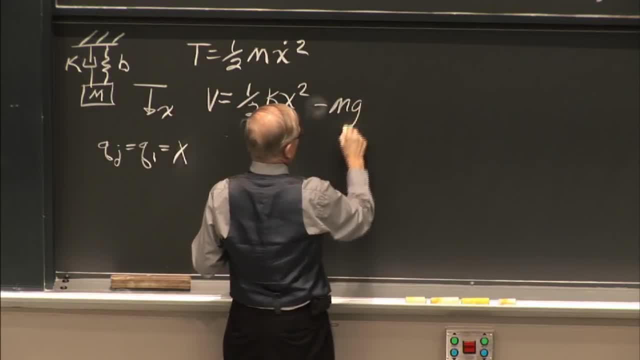 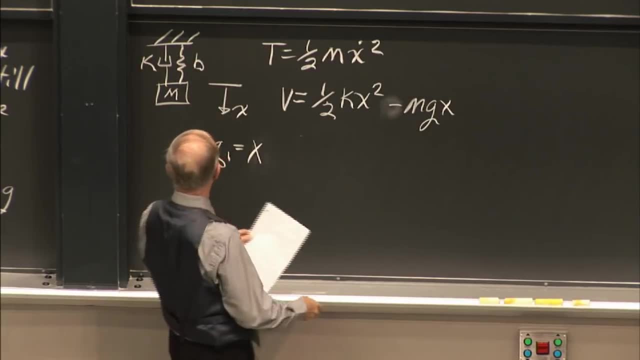 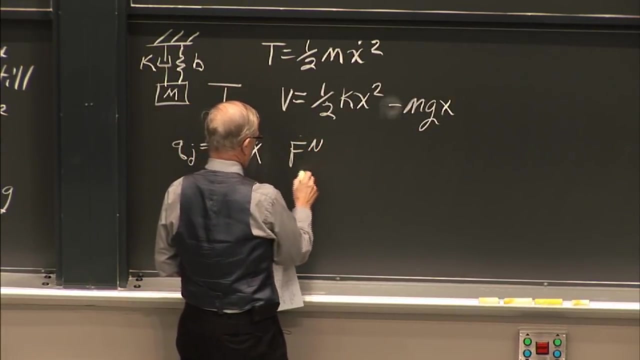 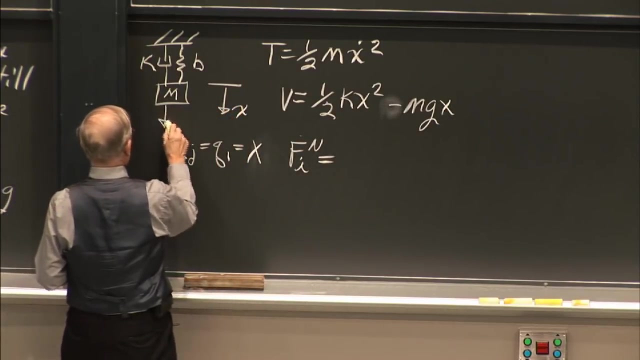 Minus m, g, x for the gravitational potential, energy. And now we can start And we have some external non-conservative forces. What are they? Fi non-conservative? And I think I'll better. I'm going to put an excitation on here too. 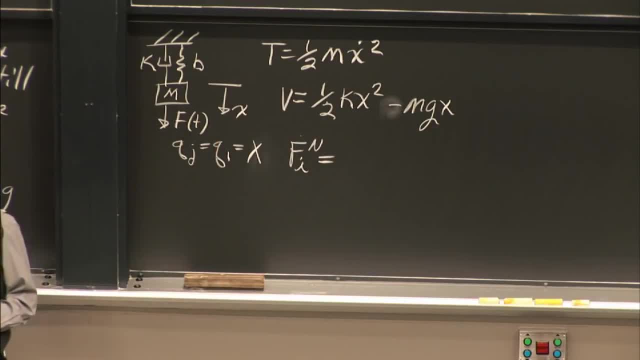 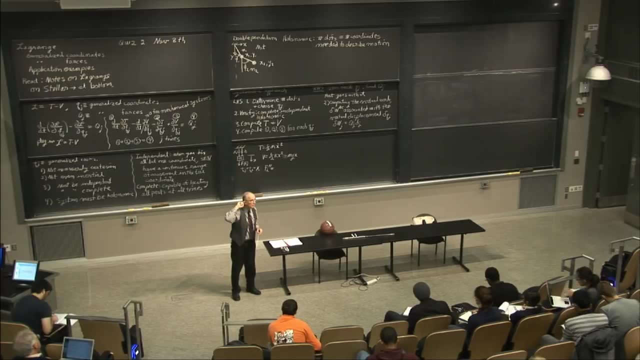 Some f of t, So what are they? I'm going to put an excitation on here too. Some f of t, So what are they? Some of the non-conservative forces. Jonathan Pardon, k x, dot, Not k, but my mistake. 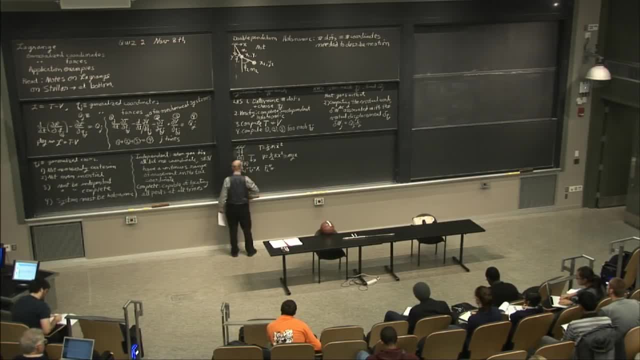 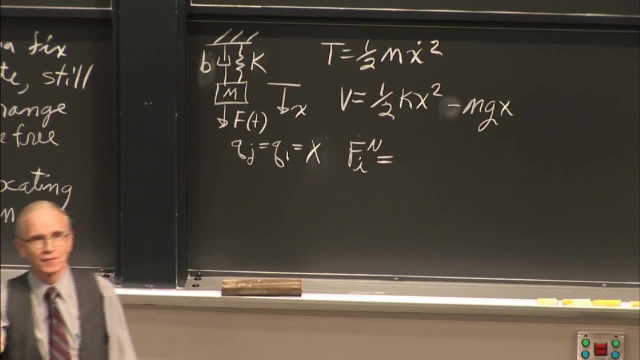 Sorry about that. You're correct. My brain is getting ahead of my writing here. That's normally b And this would be k. I'm not trying to really mess you up there. So what would that be? It would be b, x, dot, right. 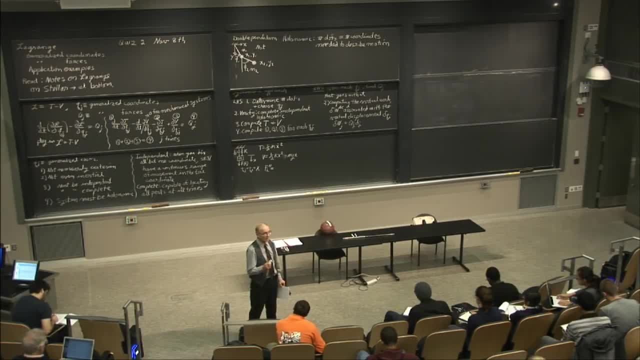 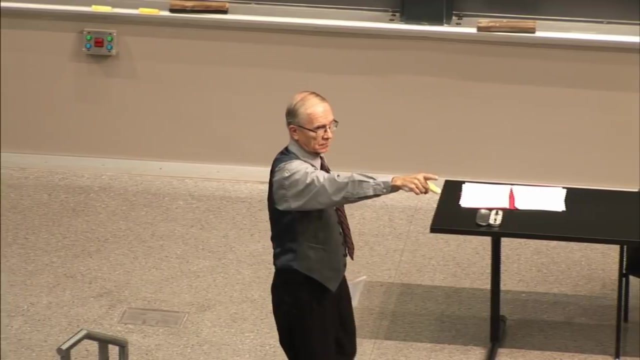 And is there anything else? Are there any other non-conservative forces? Non-conservative forces, Things that can put energy into or out of the system. So the damper can certainly extract energy. The force f. Yeah, the force f. 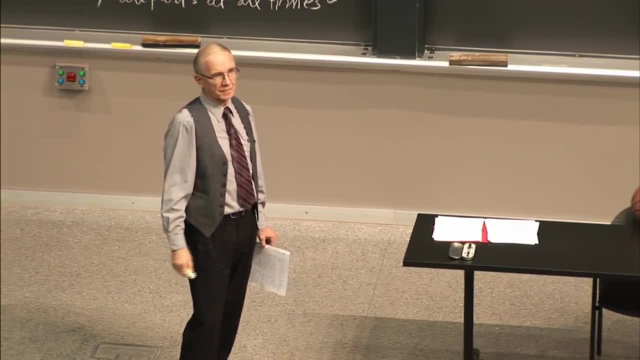 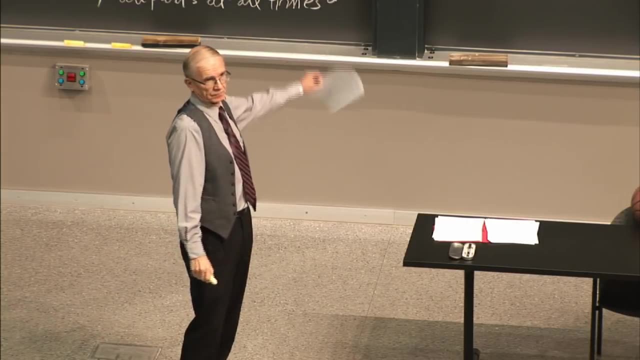 That external. it might be something that's making it vibrate or whatever, But it's an external force and it can do work on the system And it's not necessarily a potential. It's not a spring and it's not gravity. 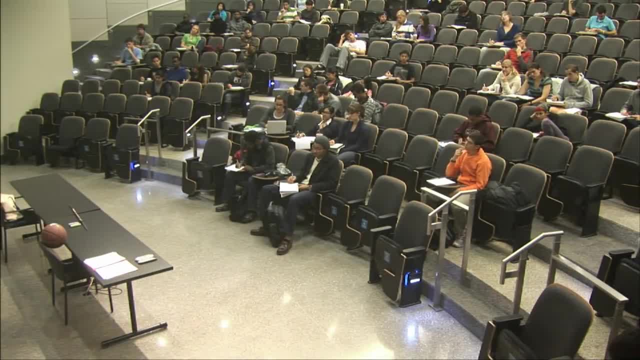 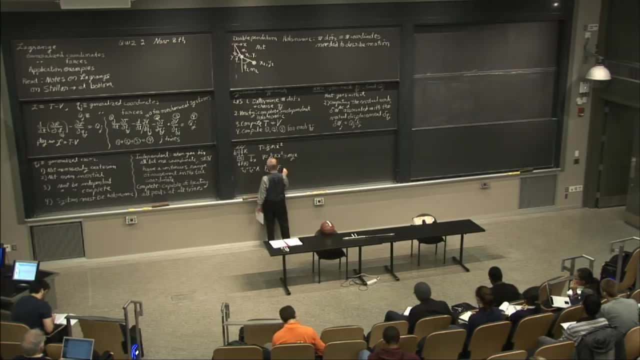 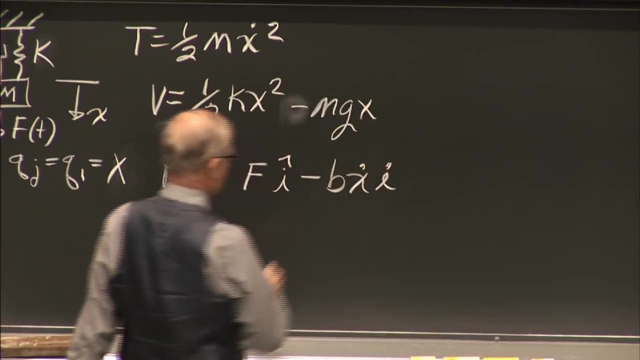 It's coming up and somebody's shaking it or something like that. So f is also non-conservative. So the non-conservative forces in this thing are f in the i direction and minus b, x dot in the i direction. And we could in our normal approach using Newton, 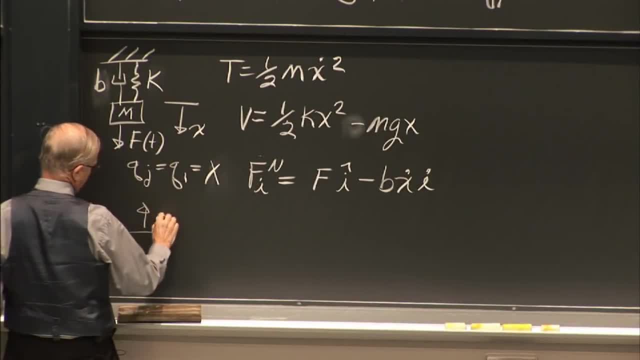 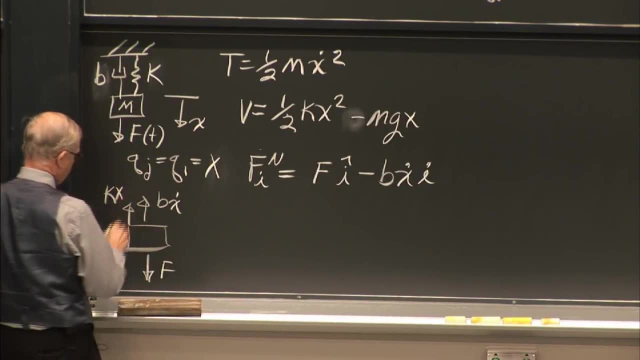 we'd draw a free body diagram And we'd identify a b x dot on it and an f on it, But we'd also have We'd have our k x on it. That would be what our free body diagram would look like. 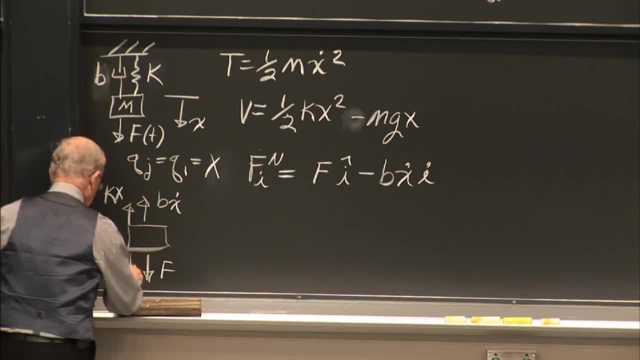 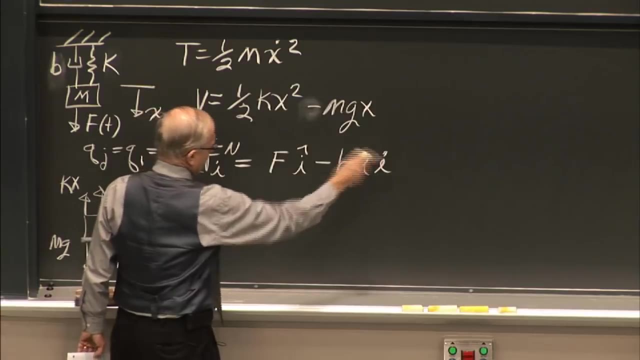 That's a conservative force. Oops, and we need an mg. So we have two conservative forces- k, x and mg- And we have two non-conservative forces- b, x, dot and f. So in this case, some of the non-conservative forces. 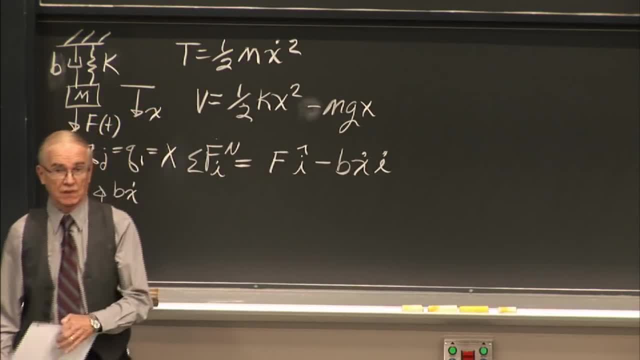 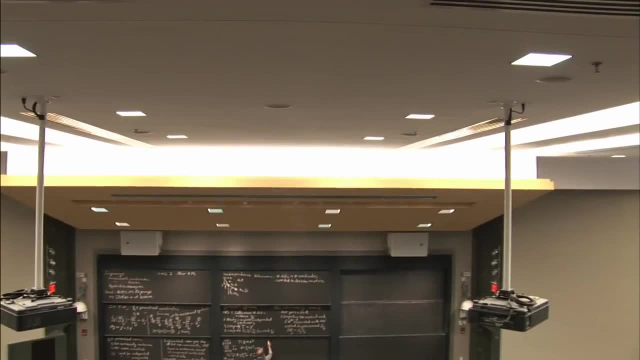 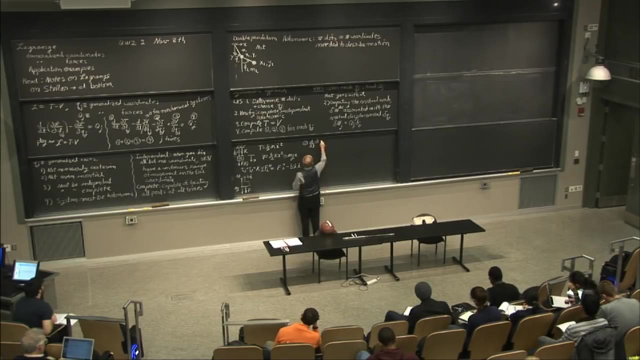 is f in the i direction, minus b, x in the i, x dot in the i direction. Ok, So, let's, So, let's do our calculus here. So 1d by dt of the partial of t, which is 1 half m x dot. 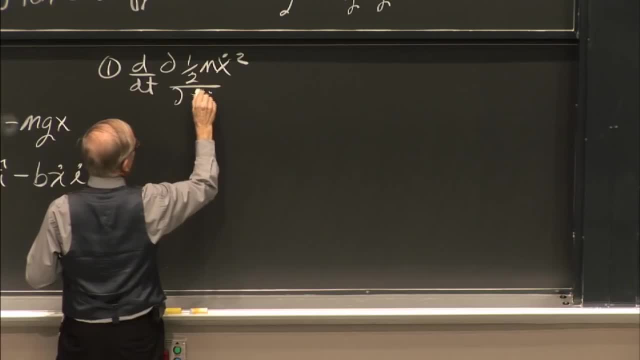 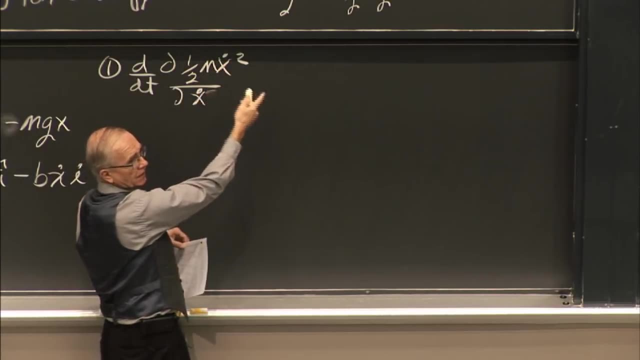 squared with respect to x dot. so that gives me the derivative of x dot. squared respect to x dot gives me 2m x dot. So this is d by dt, who was n plus nt to mx square, square, mx square. 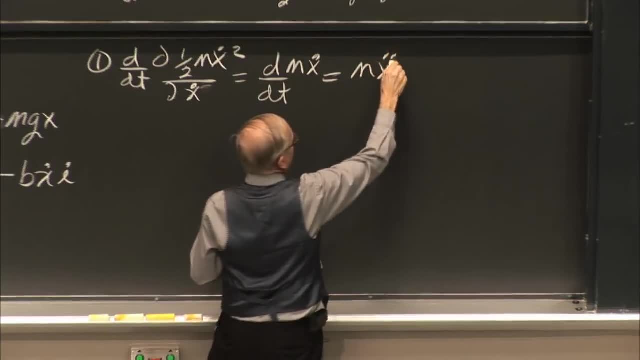 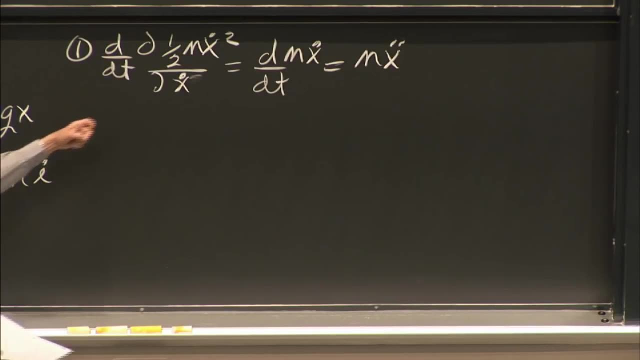 x dot. but that's m x double dot And, as you might expect, when you're trying to drive equation in motion, you're probably going to end up with an mx double dot in the result, and it always comes out of these d by dt expressions. 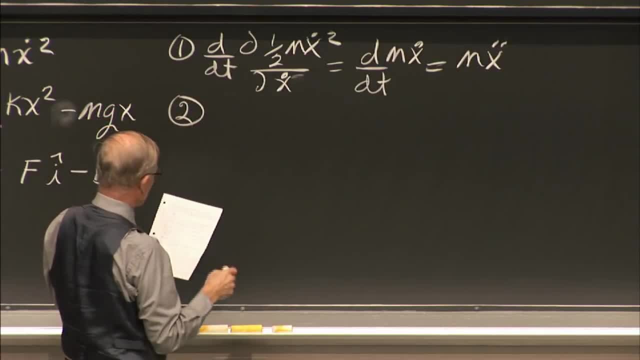 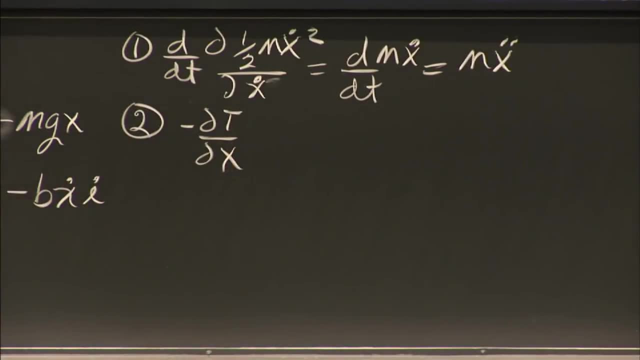 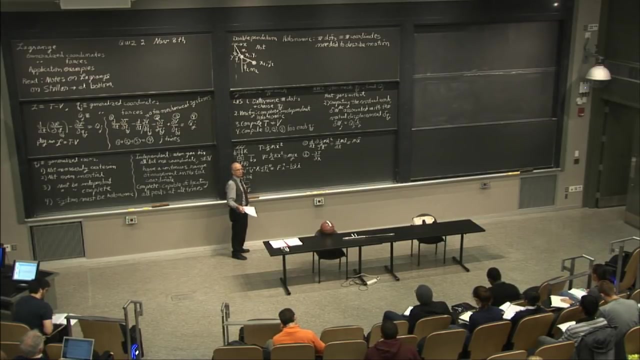 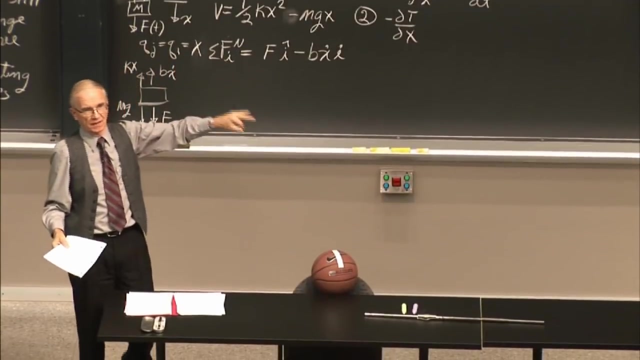 OK, so that's term one, Term two in this problem, minus t with respect to x. in this case, is t a function of x. It's 1 half m x dot squared. so is t a function of displacement x. It's a function of velocity in the x direction. 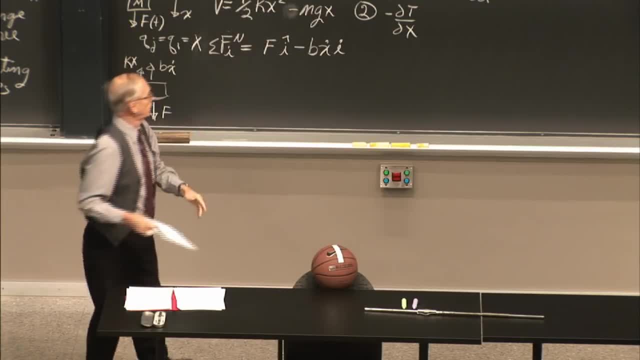 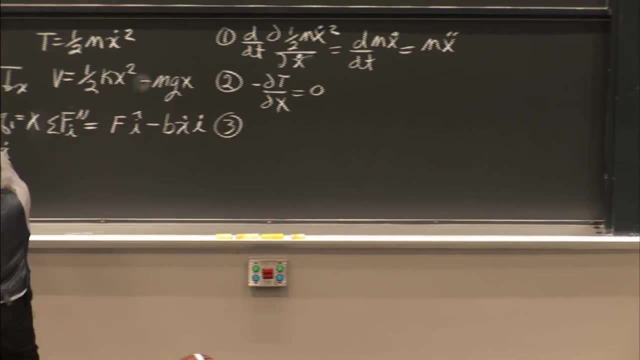 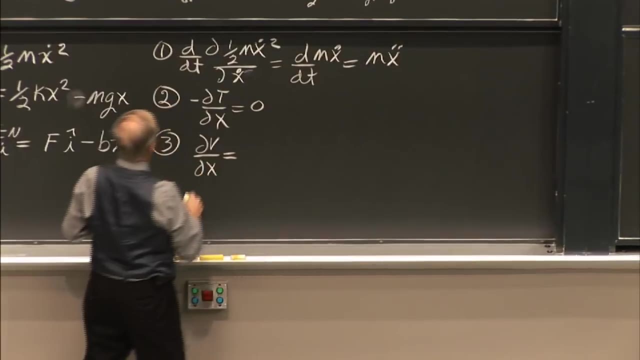 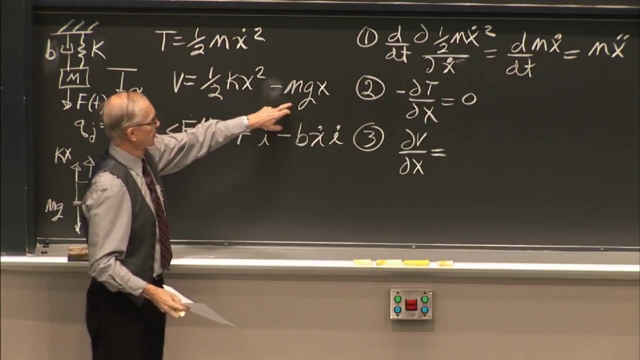 but is it a function of displacement? No, so this term is 0.. Three, our third term partial of v with respect to x. Well, where's v Half kx squared? the derivative of this is kx minus mg. 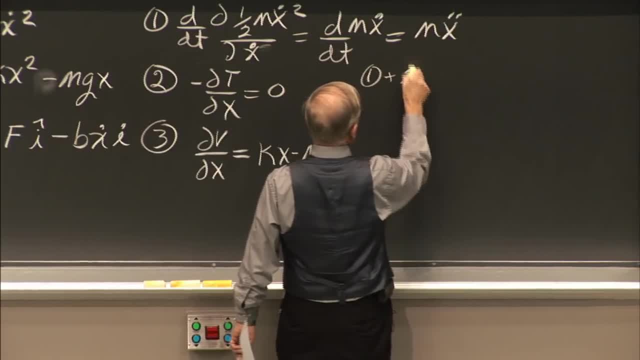 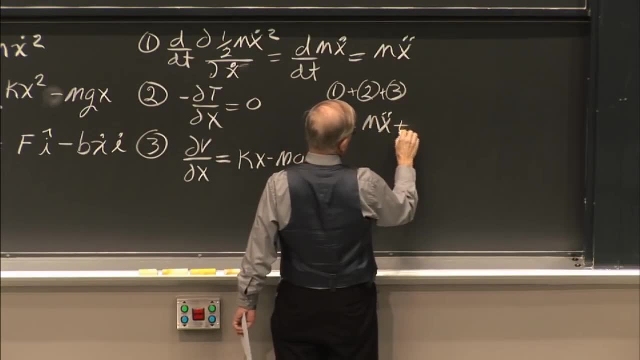 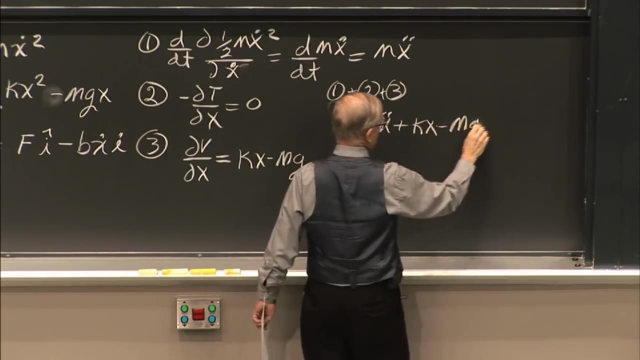 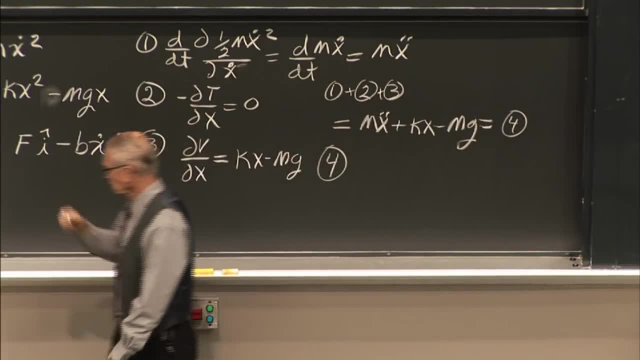 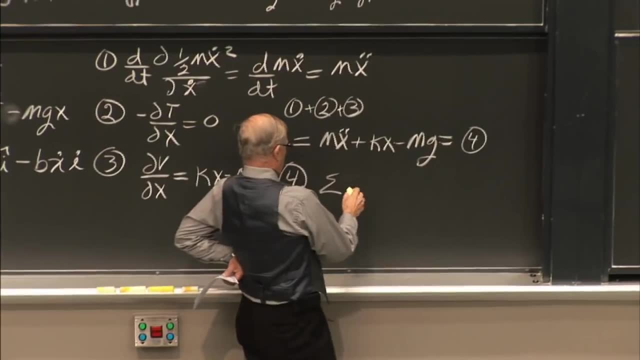 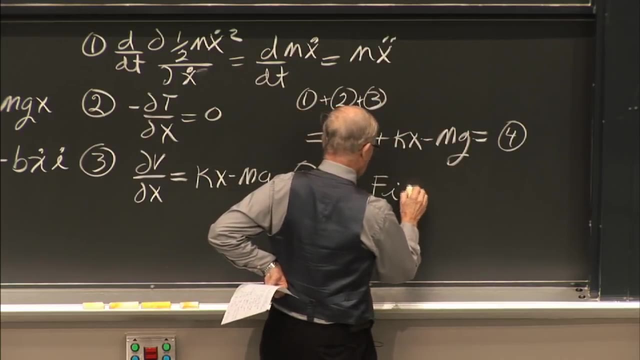 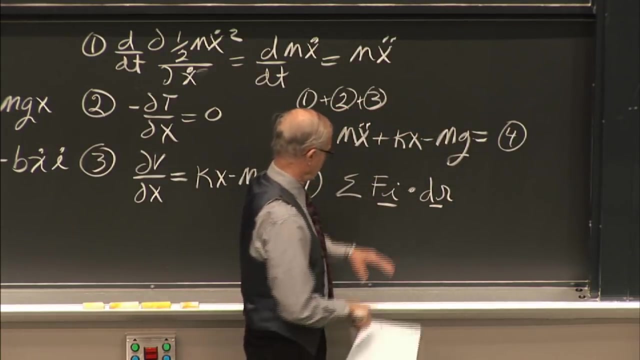 Now we need to do 4 for the right hand side, And 4 is really the summation of the fi's, the individual forces dotted with dr. These are both d, both vectors. dr is the movement. a little bit of work. 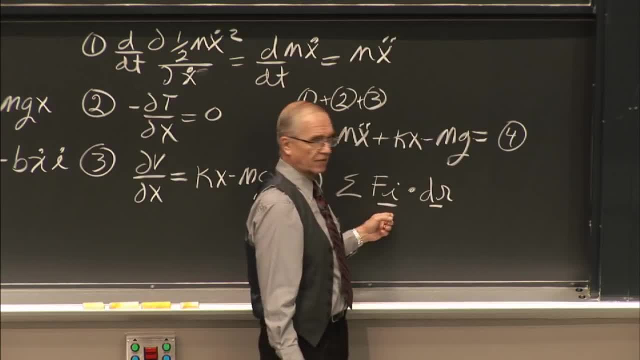 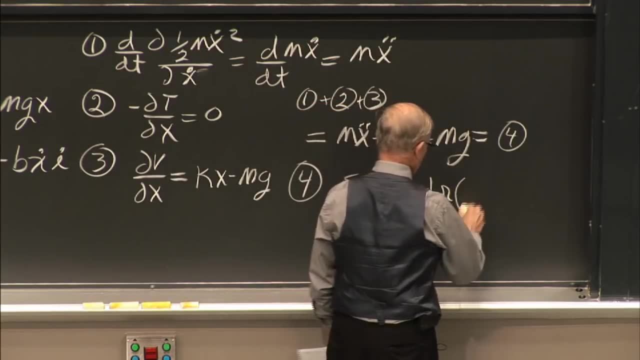 and it's going to be a delta quantity like delta. x and f are the applied forces And you need to sum these up. So this dr in general is going to be a function of the delta, j's the virtual displacements. 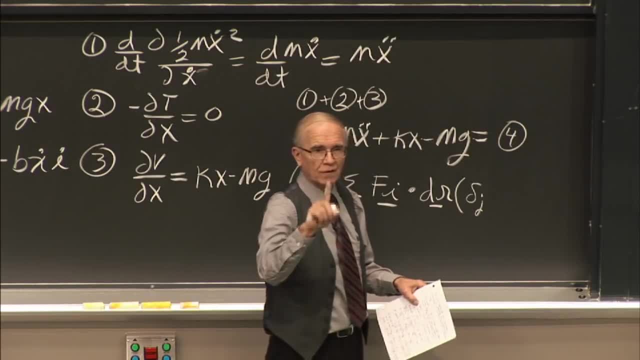 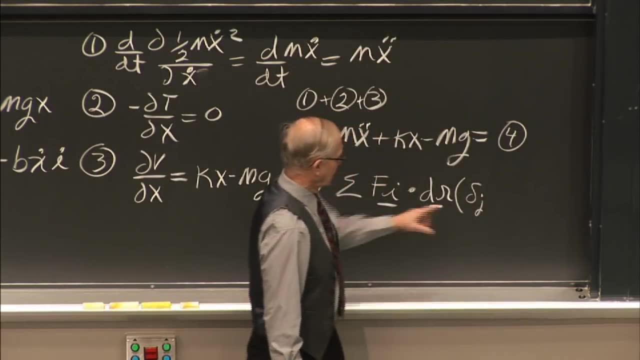 in all the possible degrees of freedom of the system. We do them one at a time. In this case we only have one, so it's trivial. But this could be delta 1,, 2,, 3,, 4. And each one of them might do some work. 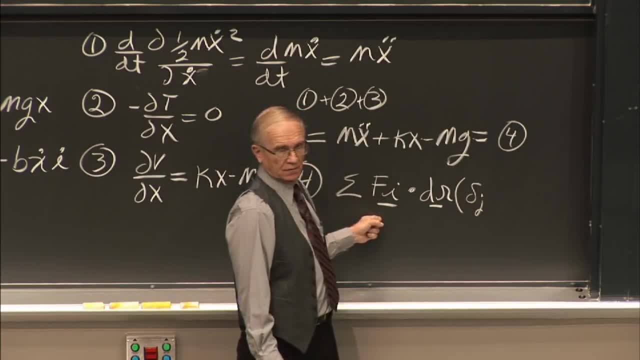 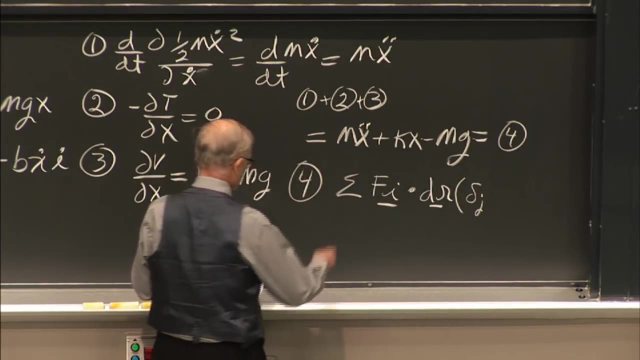 when f moves through it. But work is f, dot, the displacement. So it's the component of the force in the direction of the movement, the dot product, that gives you this little bit of virtual work. OK, so in this problem this is going. 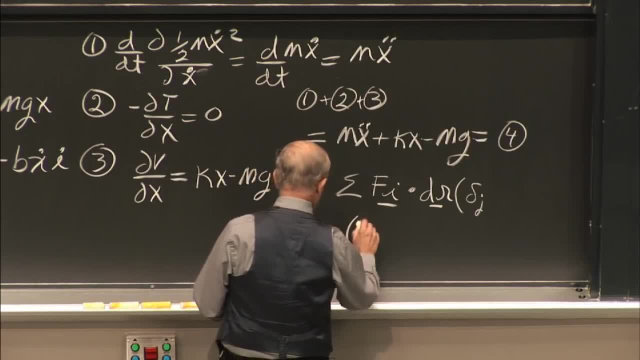 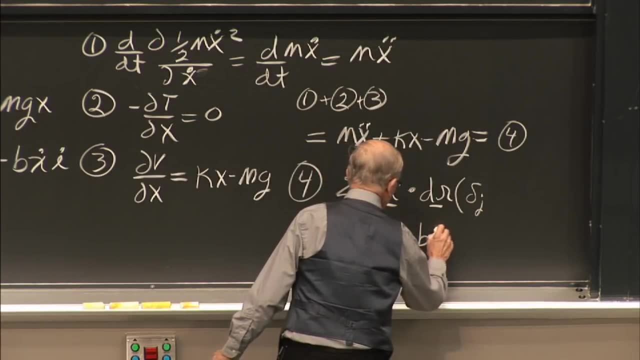 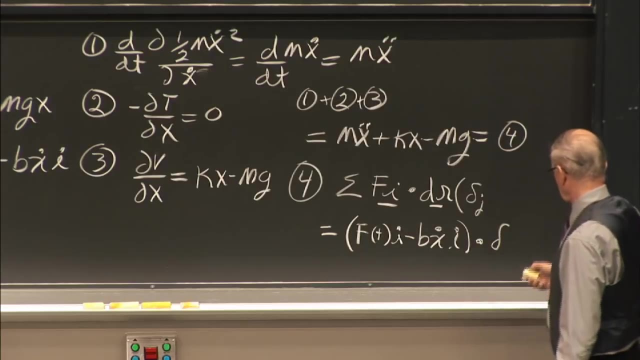 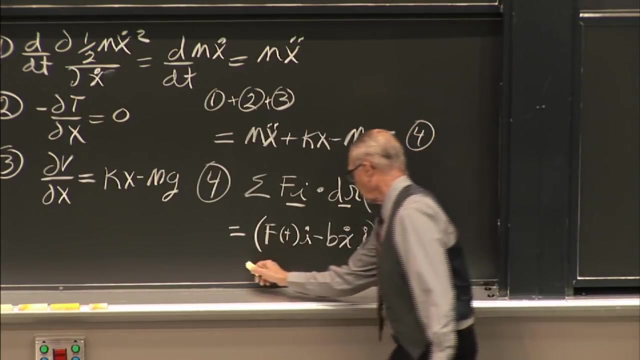 to be equal to. We actually have an f of t, some function of time in the i direction minus b x, dot in the i direction, dotted with delta x, which is our virtual displacement in our single generalized coordinate, And this whole thing is going to be equal to q x- delta x. 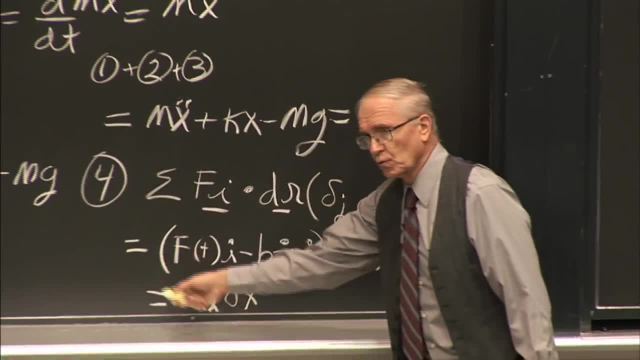 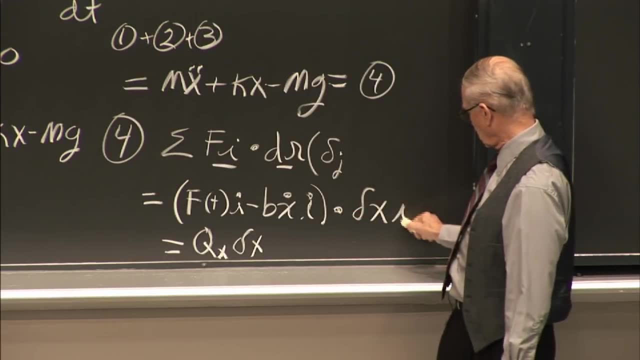 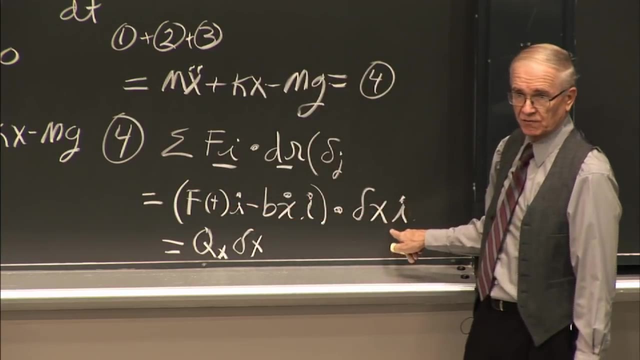 So you figure out the virtual work that's done. So if you do this dot product, this is also in the i hat direction. So i dot i, i dot i. you just get ones because the forces are in the same direction as the displacement. 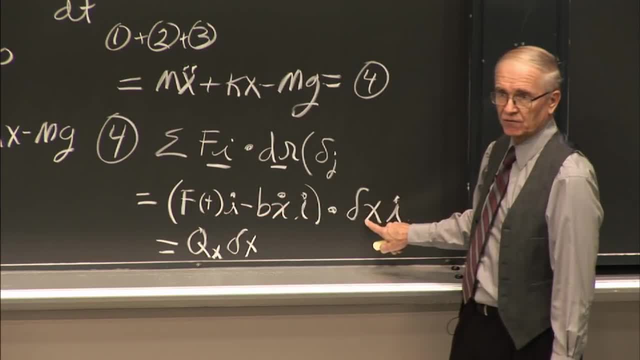 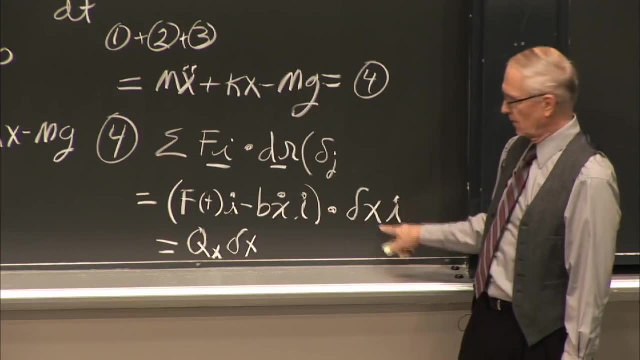 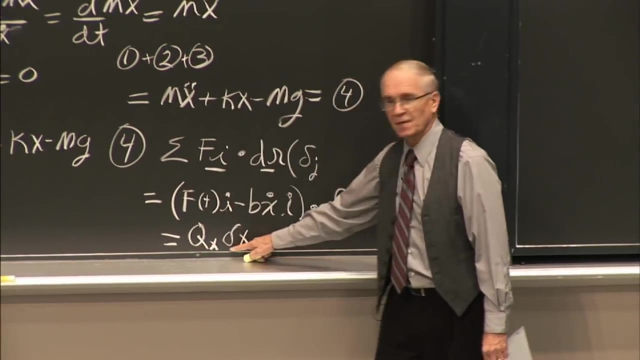 You're going to get an f of t delta x as one of the little bits of virtual work, And you'll get a minus b x dot delta x And that together, those two pieces added together, are the generalized force times delta x. 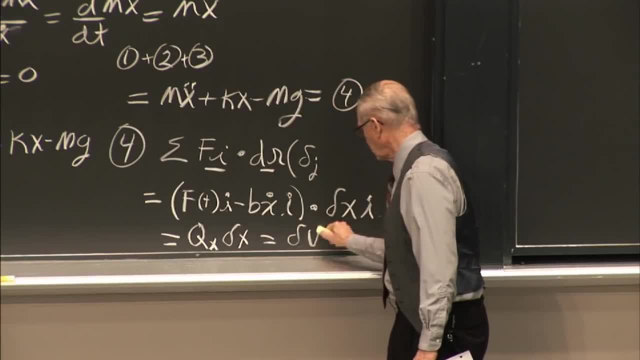 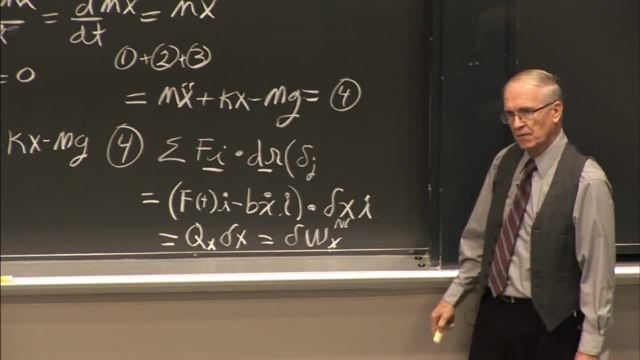 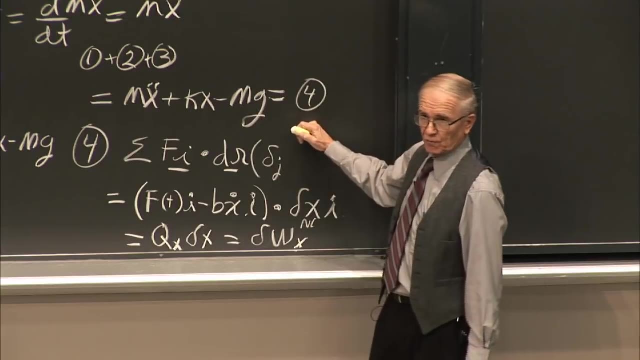 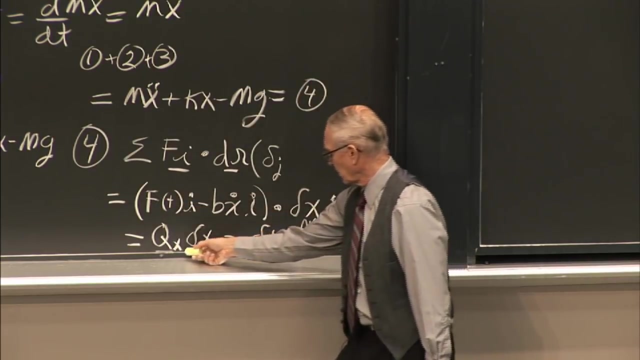 This total here gives you delta w- non-conservative, for in this case coordinate x. So we're trying to solve for what goes on the right-hand side. We need the qx. So we have here. you notice what'll happen. You'll cancel out the delta x's. that result. 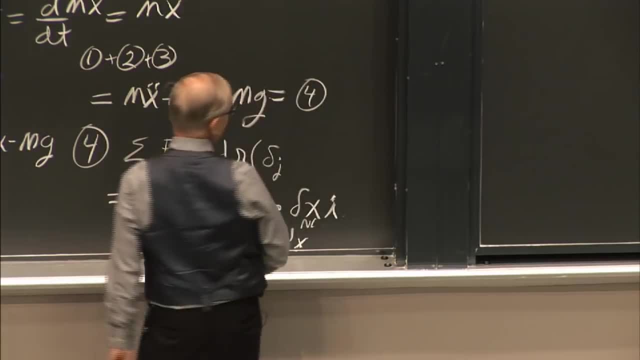 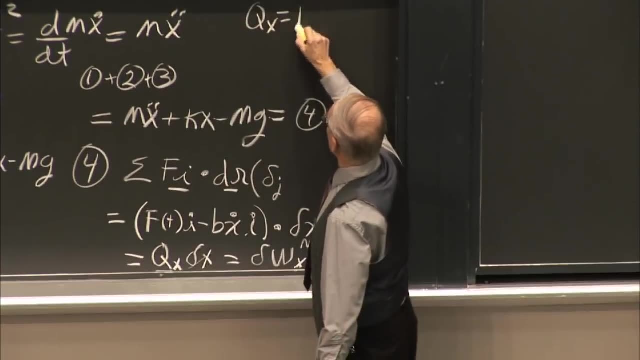 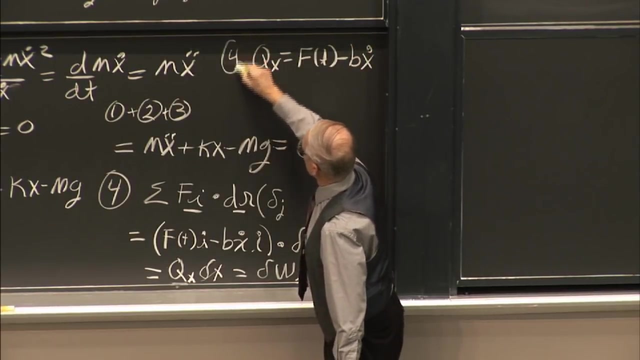 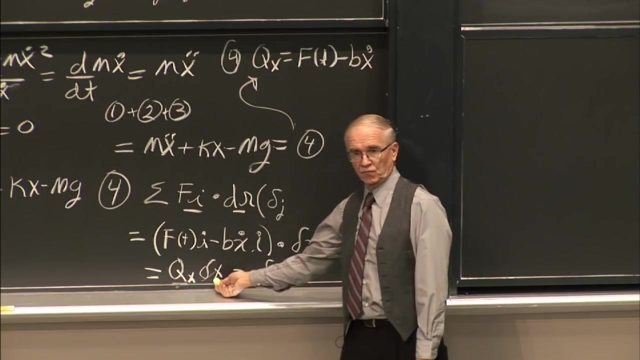 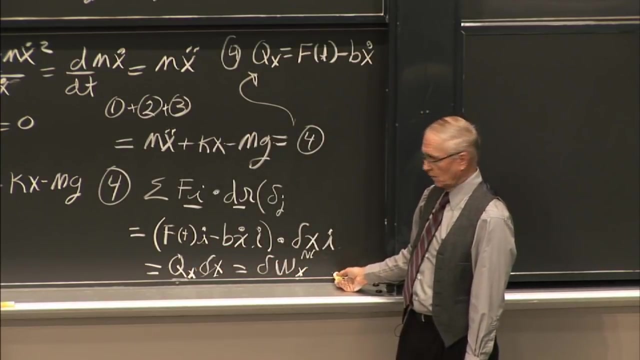 And in this case what you're left with is q: x equals f of t minus b x dot. So this is number four. So qx, delta x is the bit of virtual work that's done. What goes into our equation of motion is the qx part. 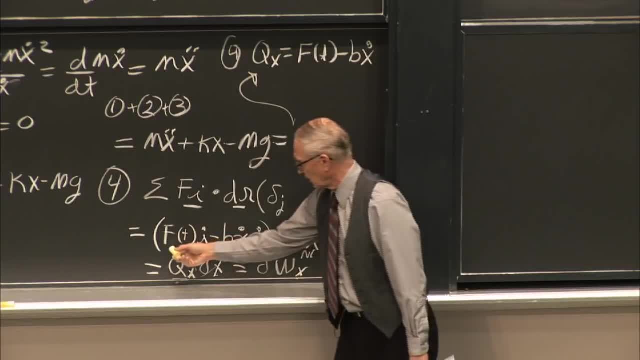 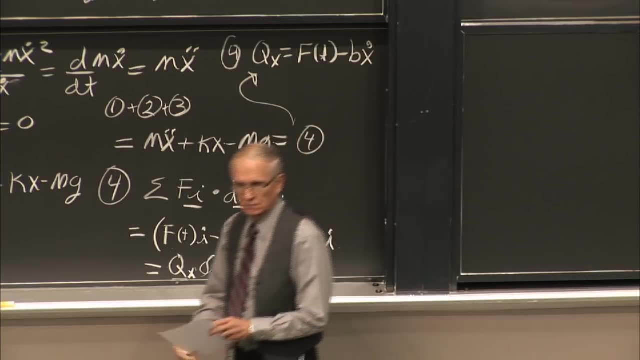 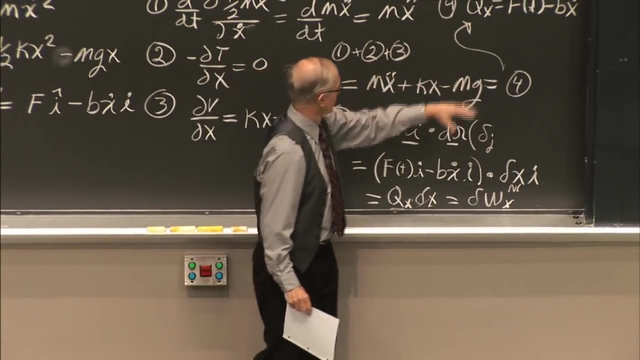 And we got it by computing the virtual work done by the applied external non-conservative forces as we imagine them going through delta x And we're done, And you have the complete equation of motion for a single degree of freedom system. You could rearrange it a little bit. 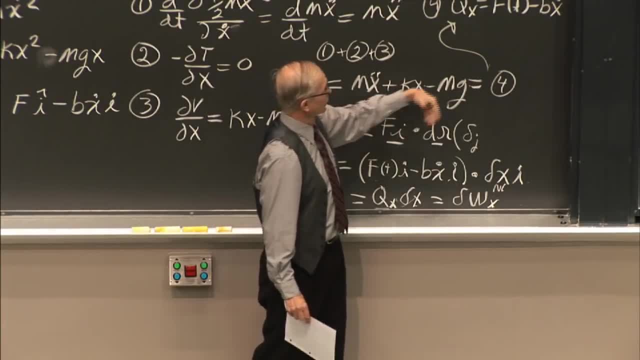 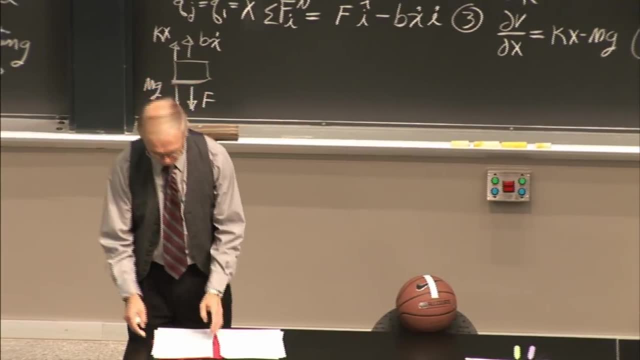 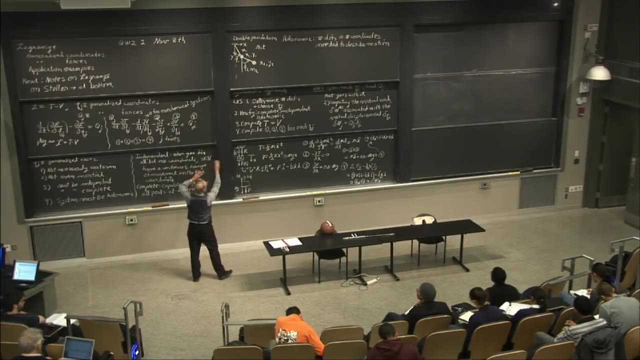 mx, double dot plus bx, dot plus kx equals mg plus f of t, if you will. So it's the same thing you would have gotten from using Newton in a trivial kind of example, but it helps define each of the steps, things that we said were required. 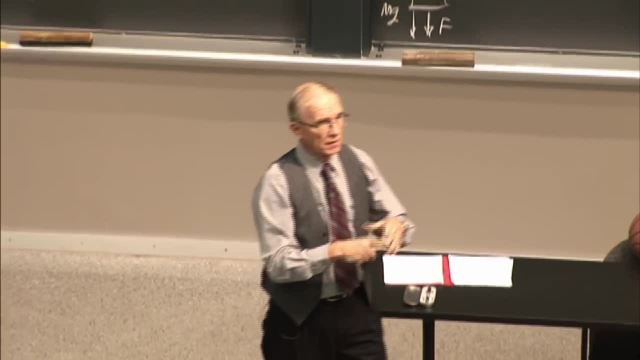 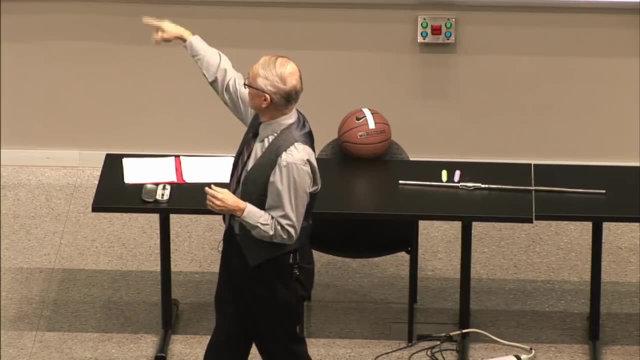 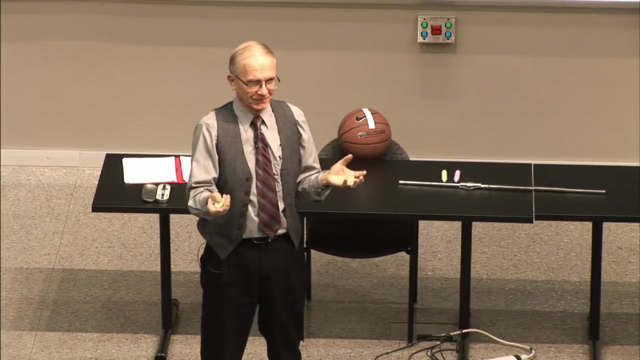 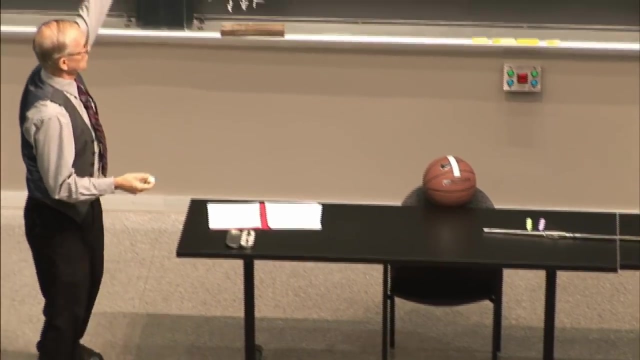 OK, so we're going to go from there to a much harder problem. So again, any issues or questions about definitions procedure. So when we start getting into multiple degrees of freedom, you need to set up a careful bookkeeping. So I just do this myself then. 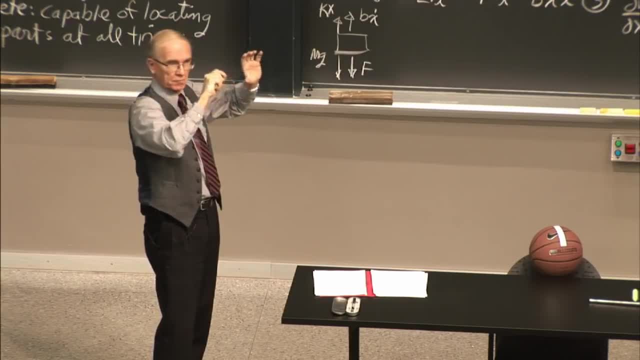 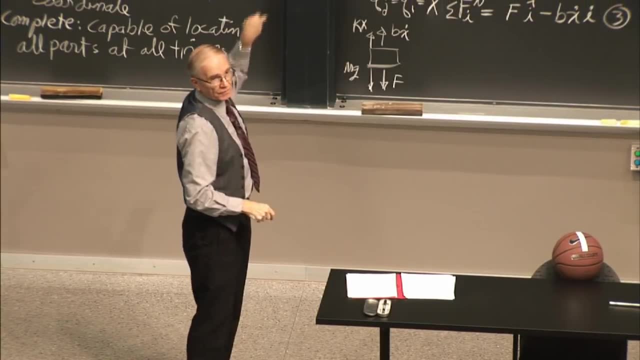 At the top of the page I identify coordinates. I write down t, write down v, Then I say OK, coordinate 1. 1,, 2, 3, 4. equation. Then I start with the coordinate 2, calculus for 1,, 2,, 3,. 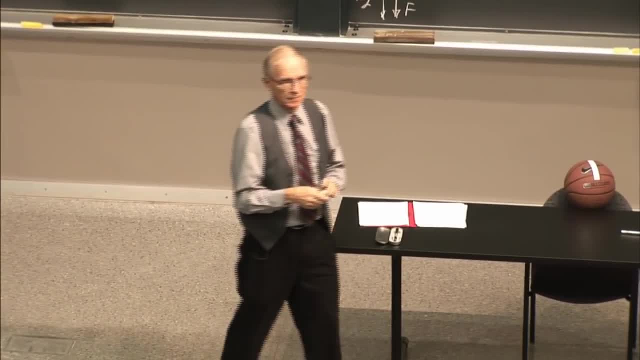 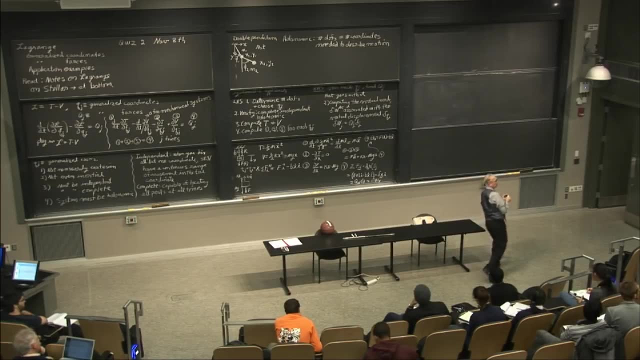 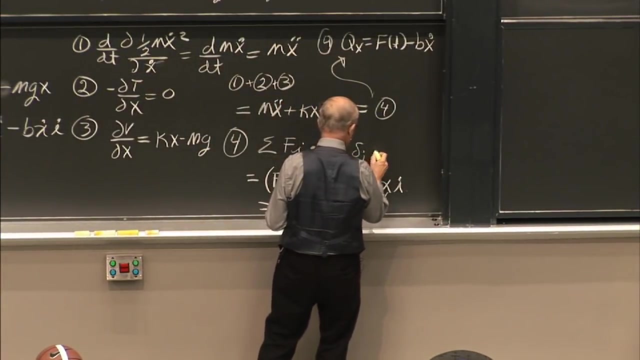 and 4, and so forth until you get to the end. OK, questions. Yeah, On the line with the four circles. what's that thing after the dr? It's like the delta parentheses and the j's. Oh, these are functions of the delta j's. 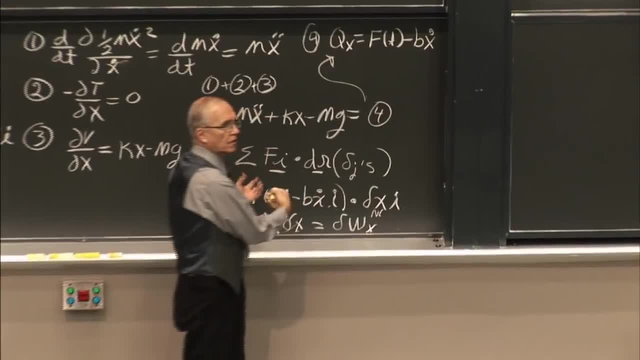 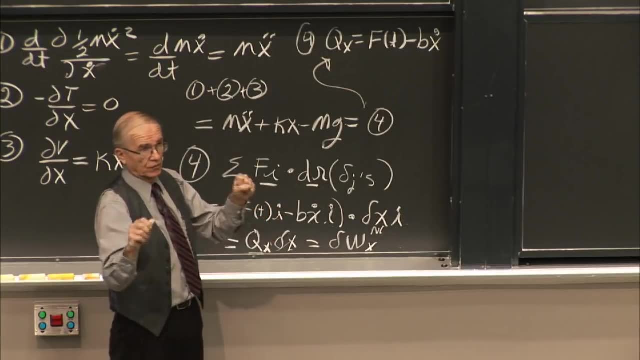 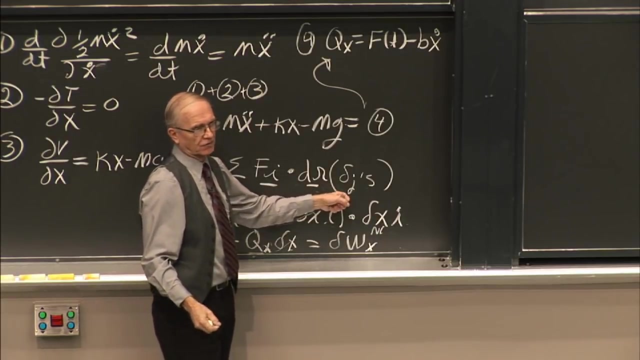 This, dr, where it comes from, the work that's being done in the virtual displacement around a dynamic equilibrium position for the system, is a little movement of the system, dr, And we express it. It's expressed in terms of a virtual displacement of the generalized coordinates of the system. 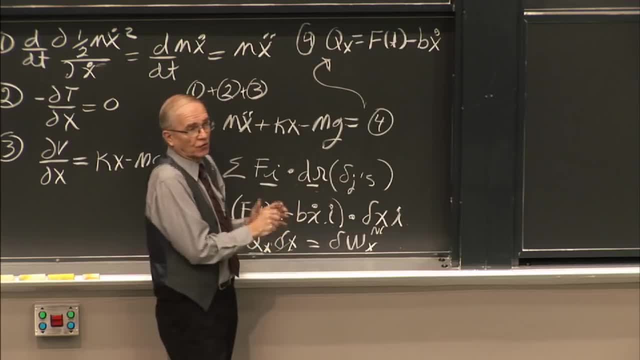 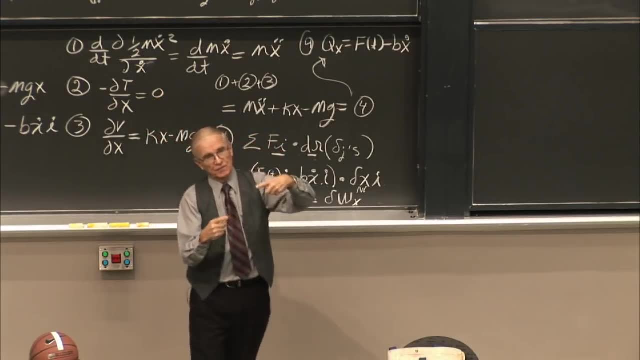 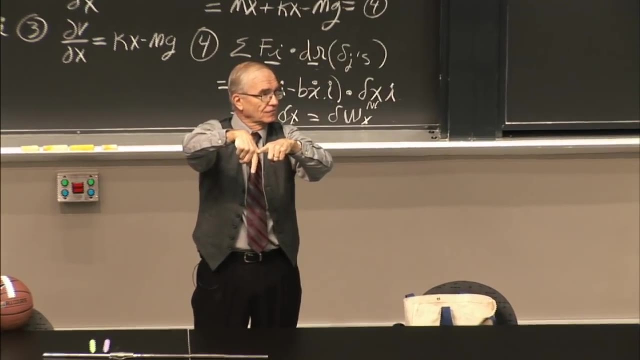 So where the dr comes from is going to be delta. In this case it's only delta x, And in the next problem we're going to do, the force in the problem is not in exactly the same direction as the delta x's and delta theta's and so forth. 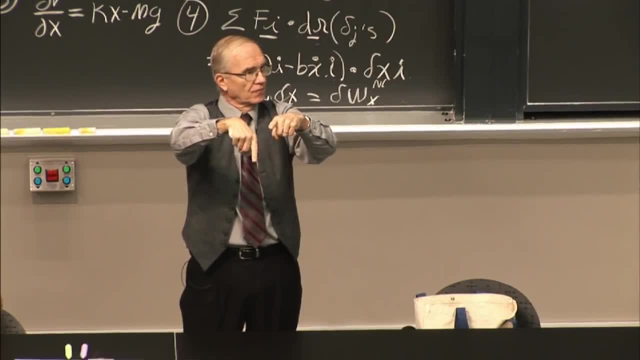 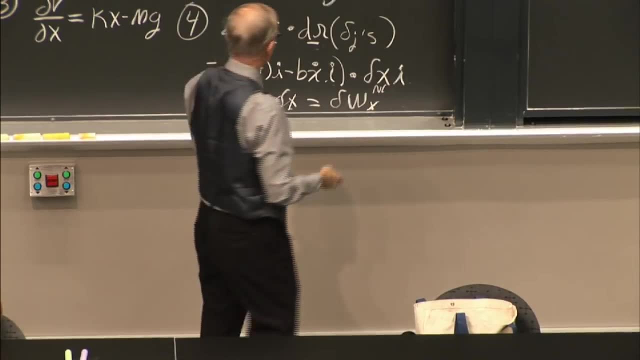 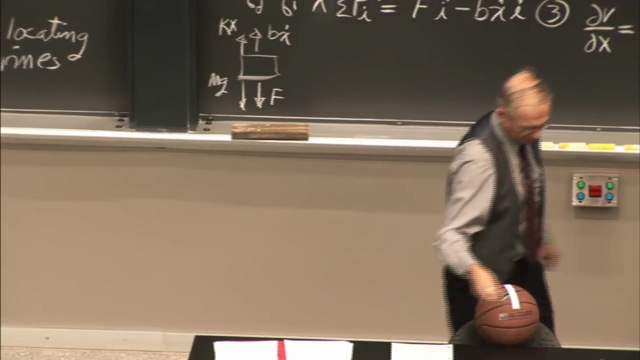 So when you do the dot product, only that component of the force that's in the direction of the virtual displacement does work And you account for that. So let's look into a more difficult problem. So the problem is this. I tried to. 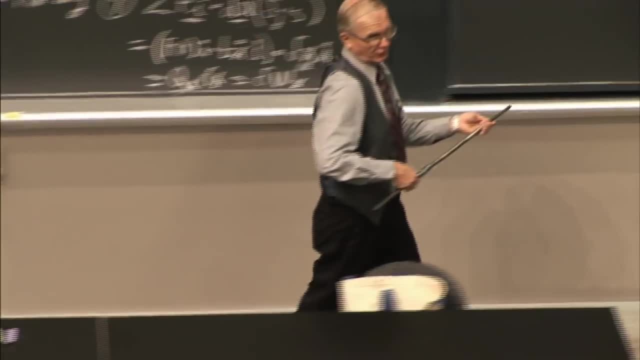 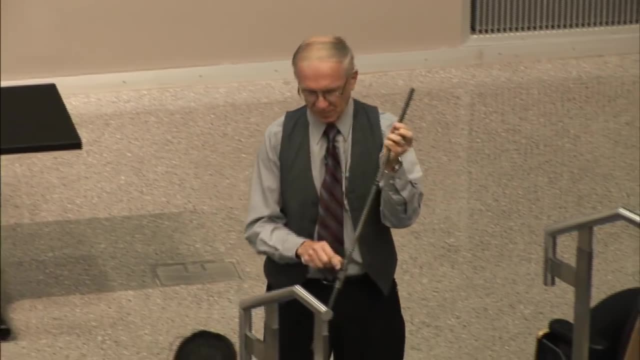 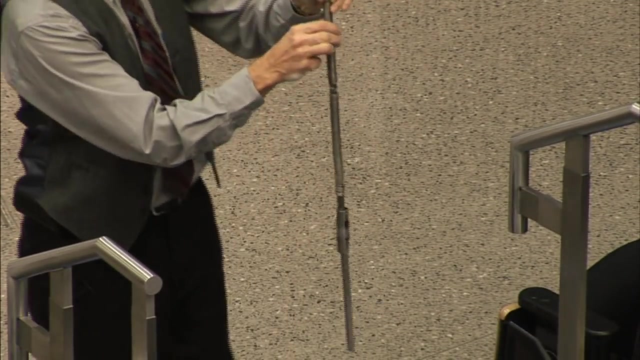 I tried to fix this up before I came to class And I didn't really quite have the parts and pieces I needed. But this is a piece of steel pipe here, It's a sleeve on the outside of this rod And I've got a spring that's on the outside connected. 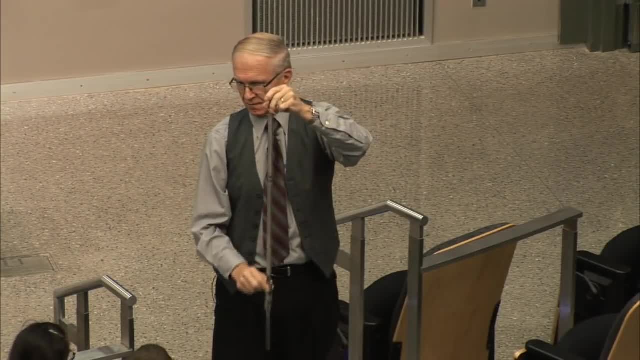 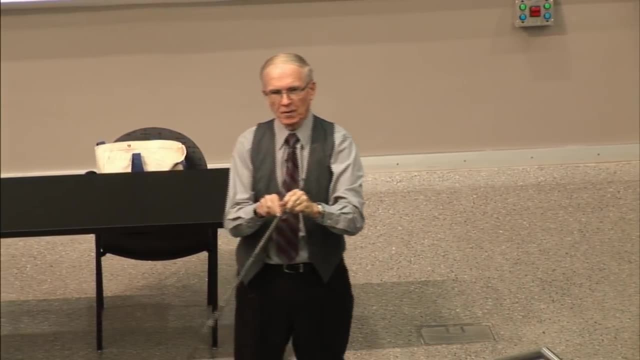 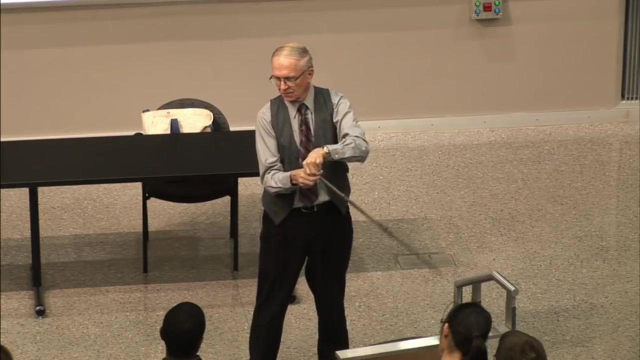 to this piece, And so we can do this, OK, And it's also, though, a pendulum, So the system I really want to look at is this system. So if this swings back and forth, the thing slides up and down. 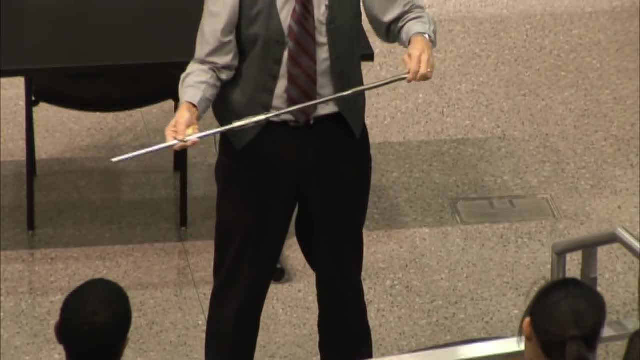 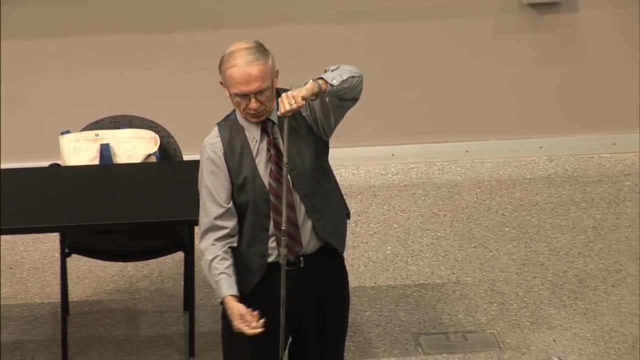 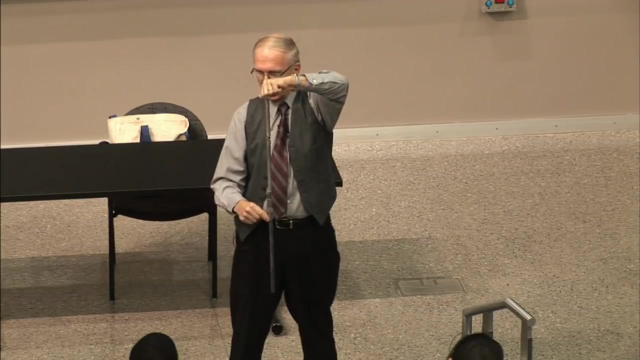 So this has multiple sources of kinetic energy, multiple forms of potential energy. OK, And I'll. For the purpose of the problem, I'm going to say that there's a force that's always horizontal, acting on this mass, pushing this system back and forth. 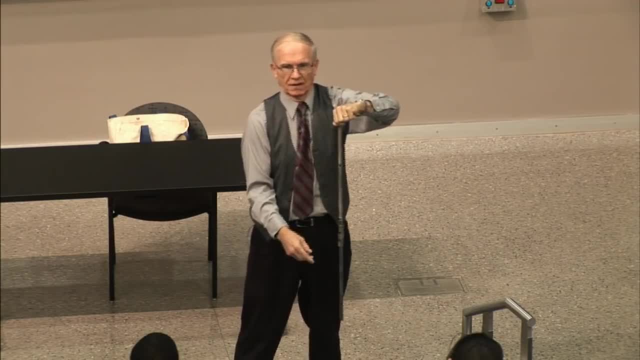 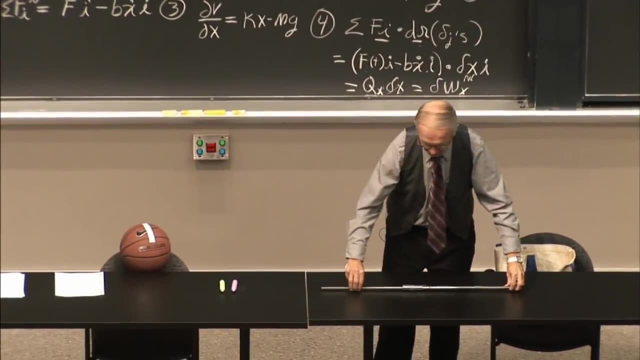 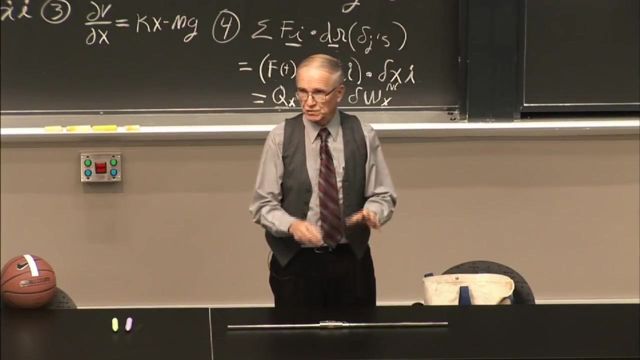 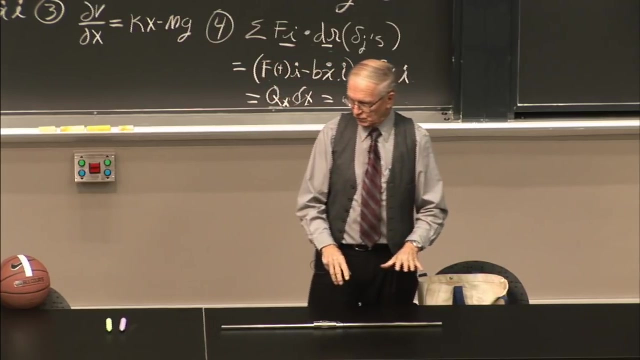 Some f, cosine, omega t, always horizontal, And I want to drive the equations of motion of the system. So is it a planar motion problem? All right, How many rigid bodies involved? Two, OK, So there's two rigid bodies. 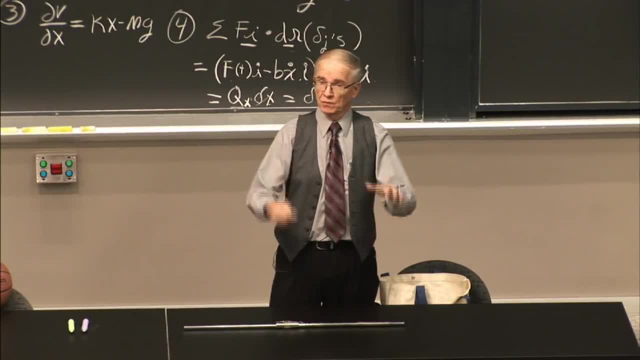 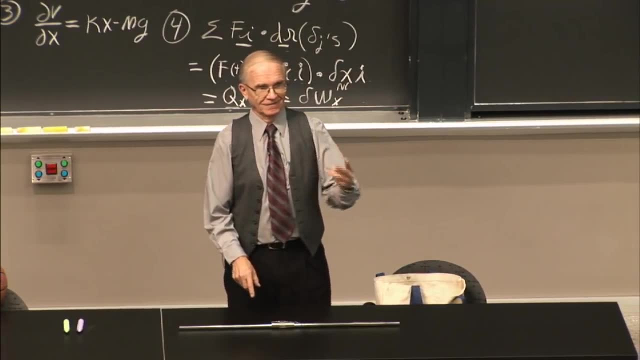 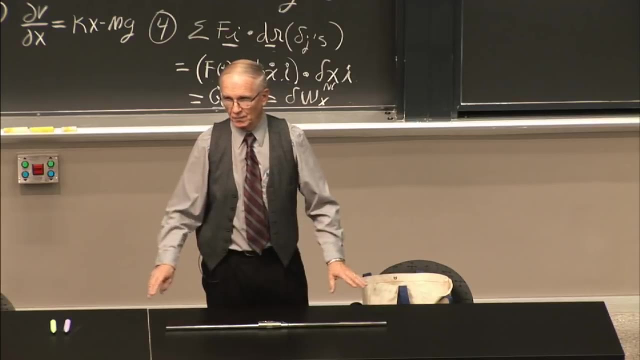 Each could have possibly six degrees of freedom. But when you say it's planar motion, you're actually immediately confining each rigid body to three. Each rigid body can move x and y and rotate in z. So when you straight out and out say this is planar motion, 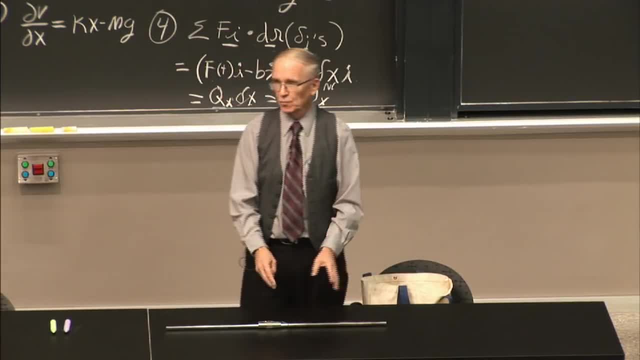 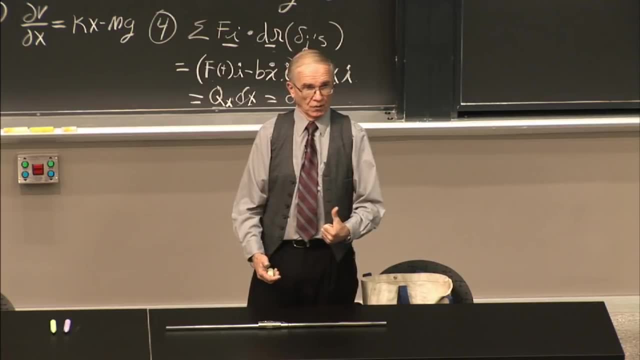 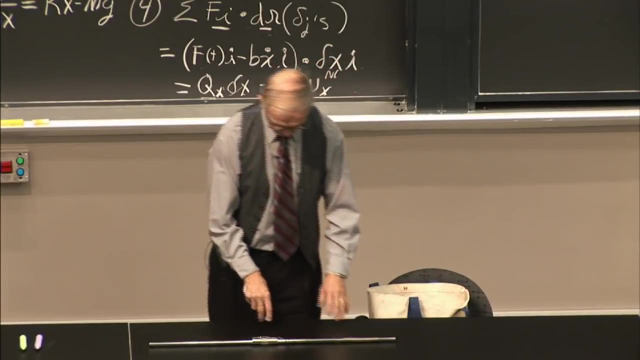 you've just said, each rigid body has max three. So this has a maximum of six possible Right? No, the other three disappear too. There's no z deflection and no rotation in the x or y. OK, So we have a possible maximum six. 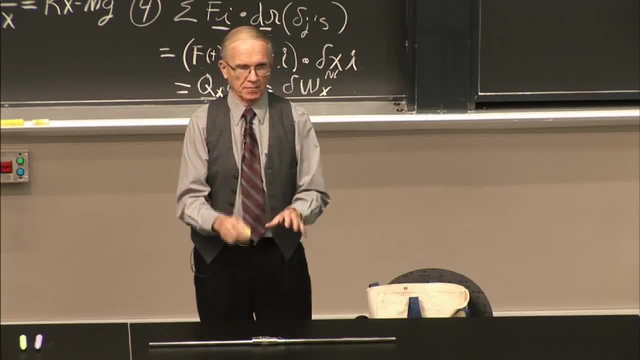 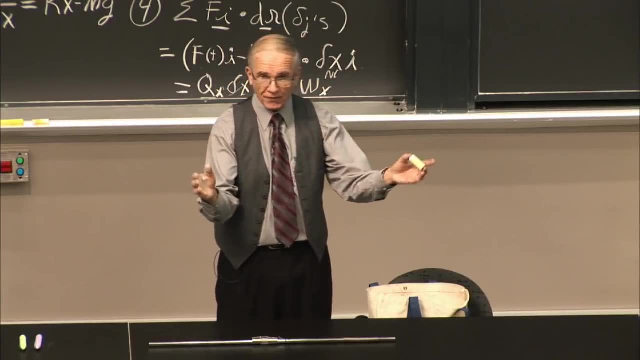 How many degrees of freedom does this problem have? How many coordinates will we need to completely describe the motion of the system? So come up, So think about that, Talk to a neighbor, Decide on the coordinates that we need to use for this. 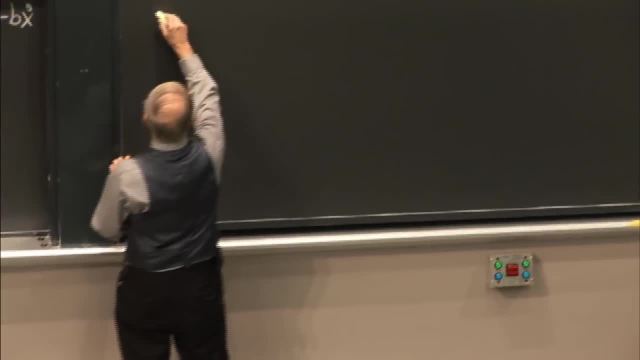 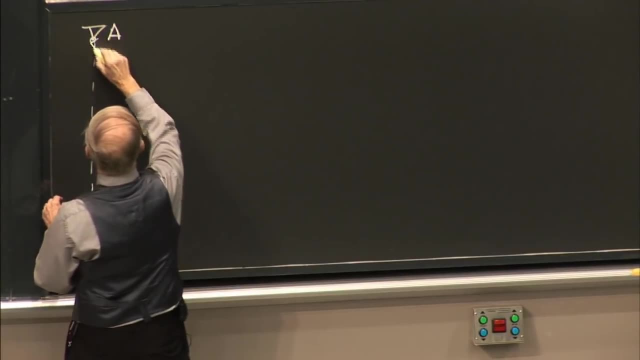 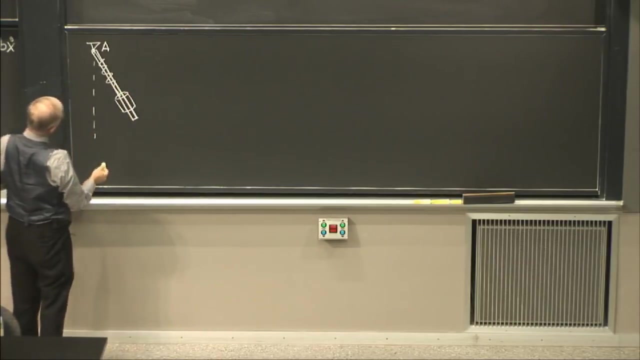 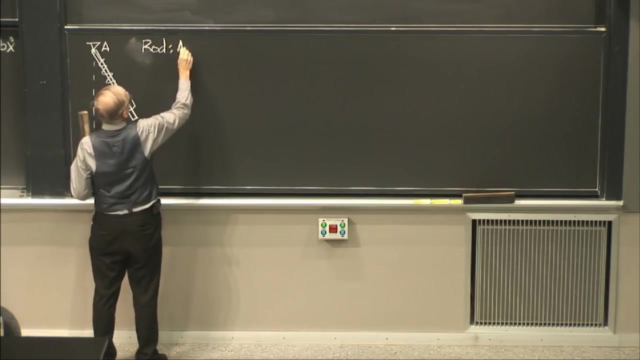 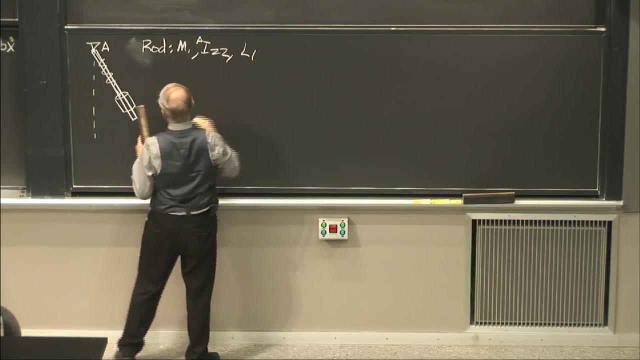 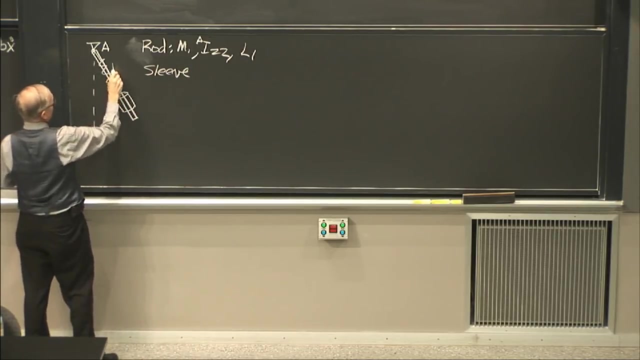 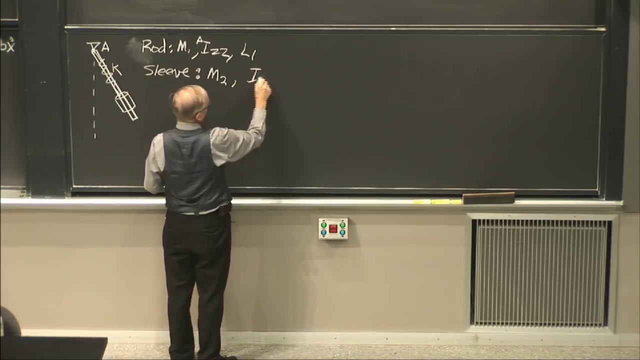 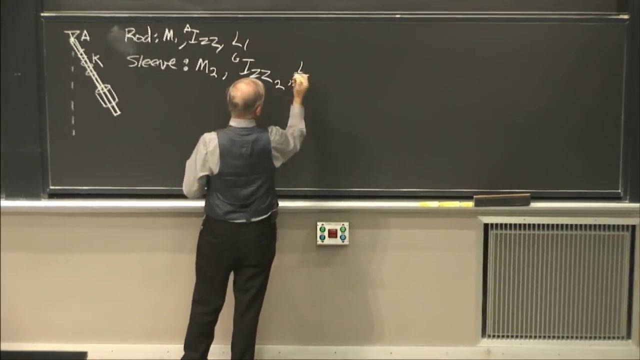 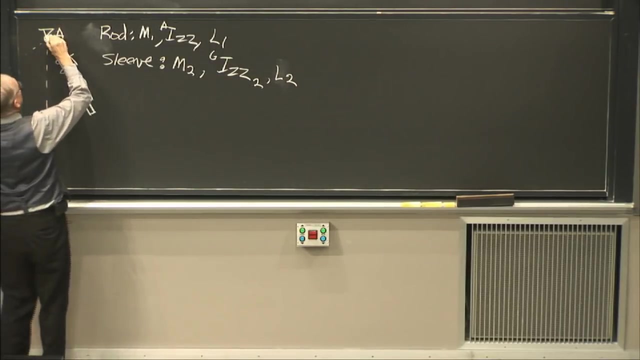 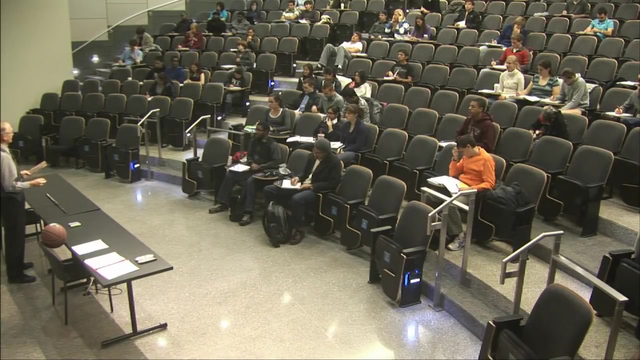 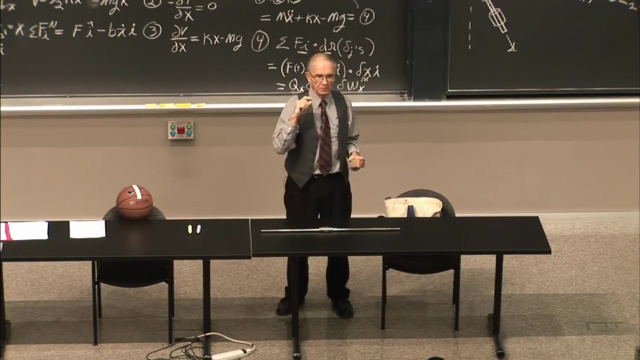 While I'm drawing it. OK, OK, OK, OK, OK, OK, What do you decide? How many? 2. 2. All right, what would you recommend? What would you choose? Pardon The angle and the top bar down the middle. 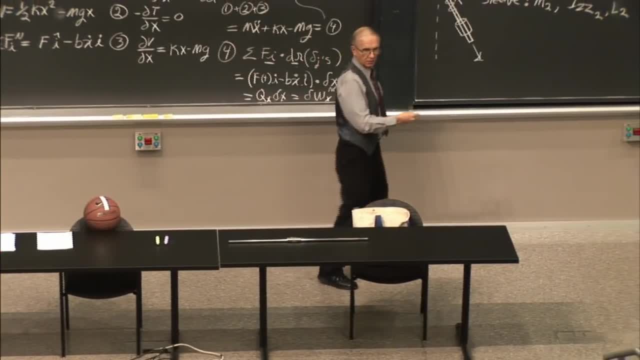 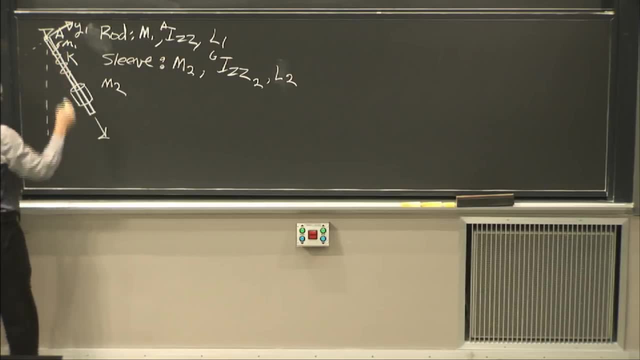 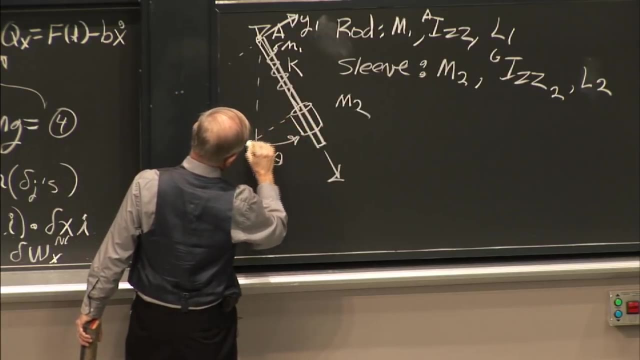 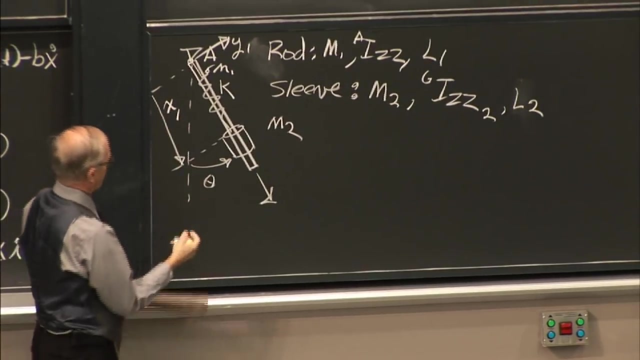 An angle and a deflection of what I'm calling m2 here. OK, So this is m2, the rod is m1, and he's suggesting an angle, theta and a deflection which I'll call x1.. And I've attached to this bar the rod I'm calling it. 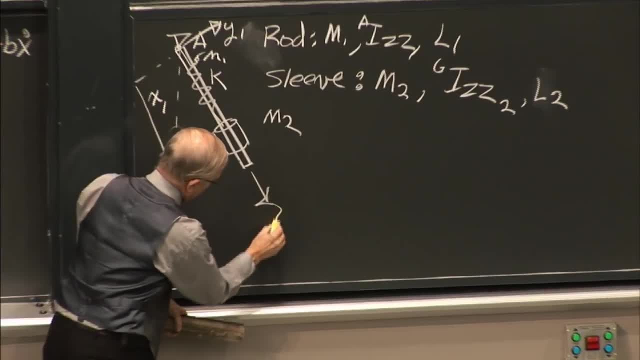 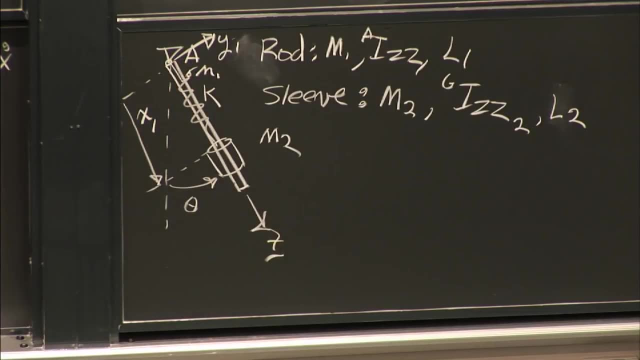 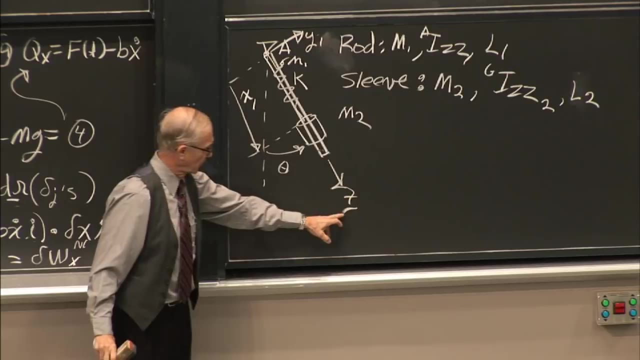 a rotating coordinate system- x1, y1, about point A. So A x1, y1 is my rotating coordinate system attached to this rod. So I'm going to locate the position of this by some value: x1, measured from point A. 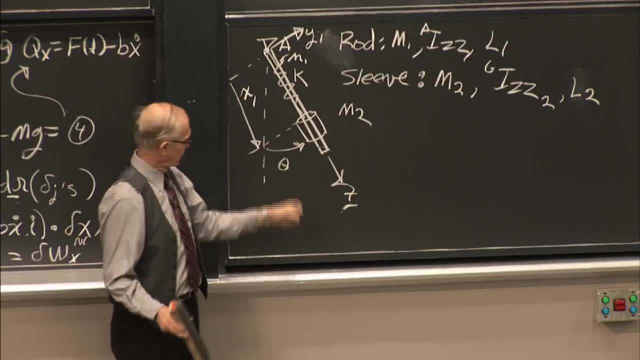 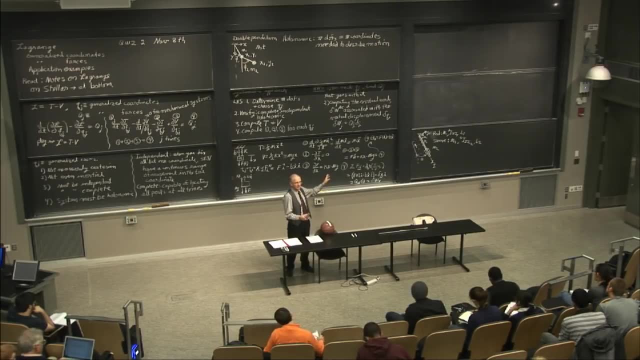 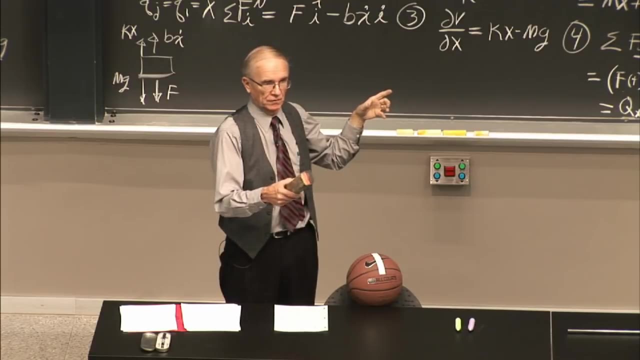 And Locate the position of the rod itself by an angle. theta Good, Is it complete? So if you freeze one, do you still have that complete? Again, did you describe the motion at any possible position? Those two things, yes. 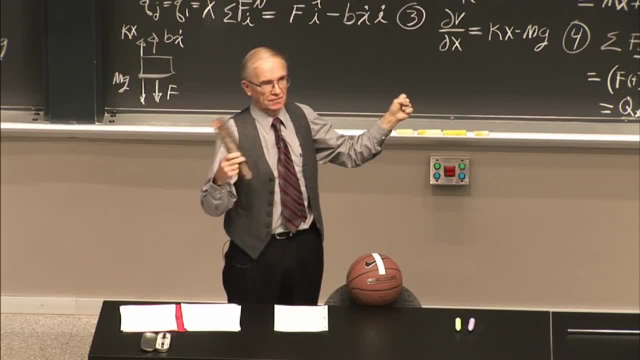 Is it independent? If you freeze x, can theta still move. If you freeze theta, can the x still move. OK, Is it whole and only Right. 2 equals. You know, If we need 2, we got 2.. 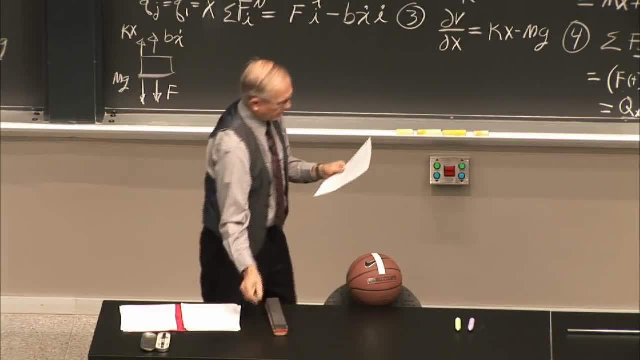 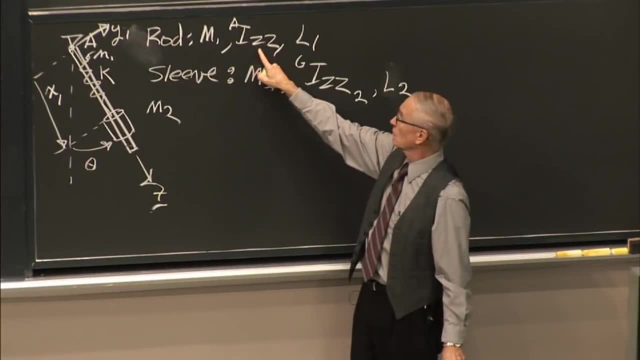 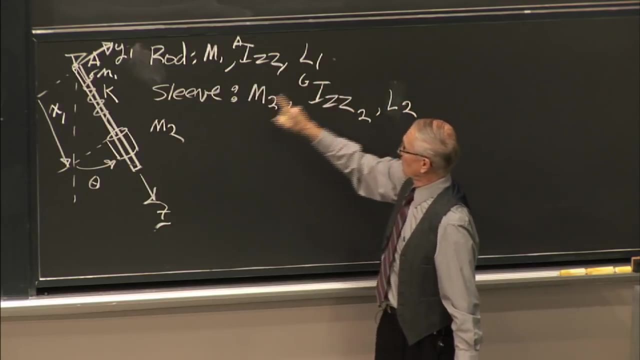 And they're independent and complete Good. So now the harder work starts. So I'm going to give us the mass of the rod, the mass moment of inertia of the rod about the z-axis. but with respect to A, The length of the rod is l1.. 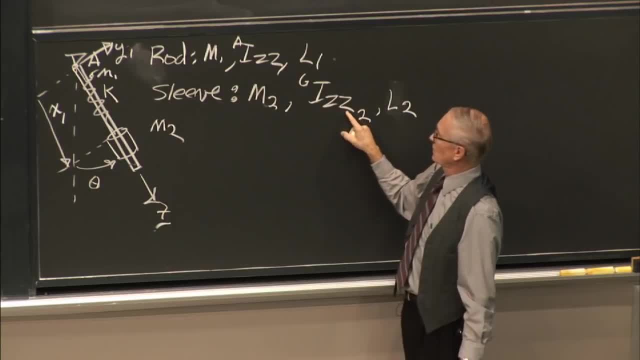 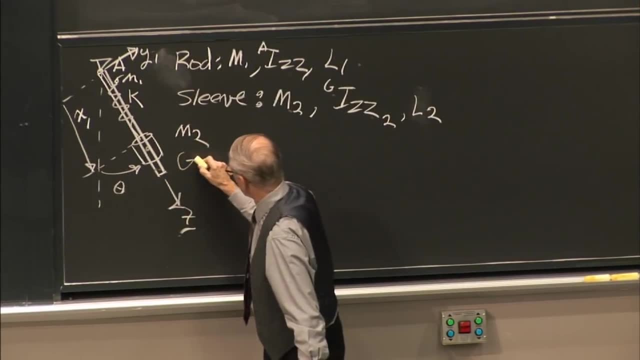 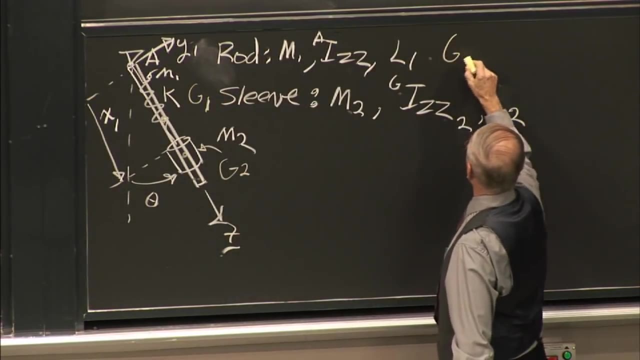 The sleeve mass m2, Izz with respect to its g, So it has a g. There's also- I better call it- g2.. That's the g of the sleeve. There's also a g1, a center of mass for the rod. 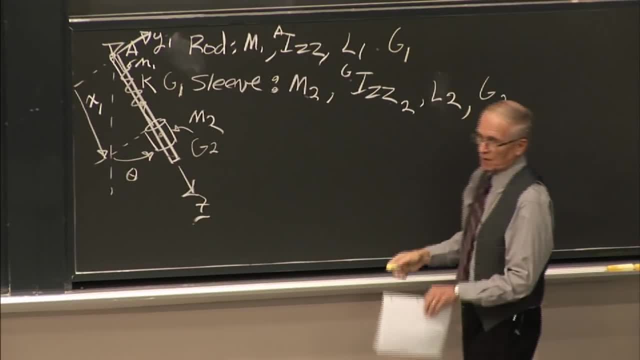 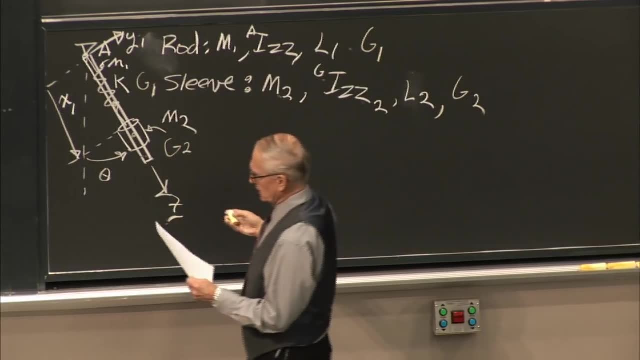 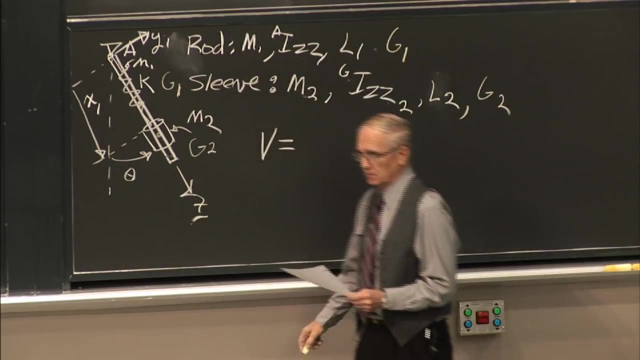 and a center of mass for the sleeve. Those are properties that we'll need to know And I'll give them to you, OK, So we need to come up with expressions for potential energy and kinetic energy. So this problem, the potential energy, is a little messy. 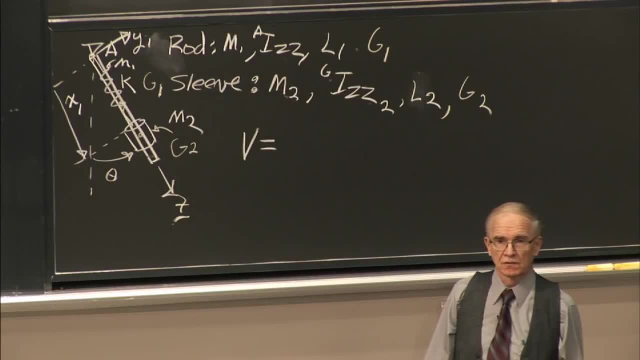 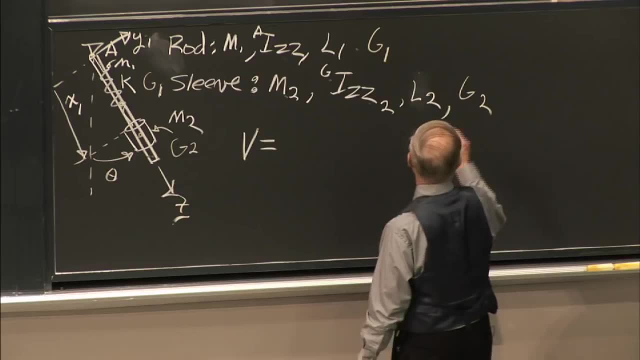 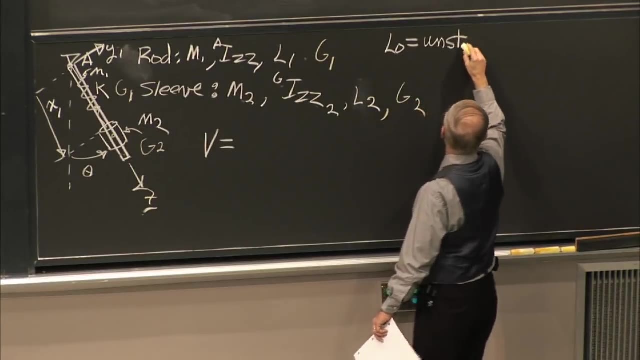 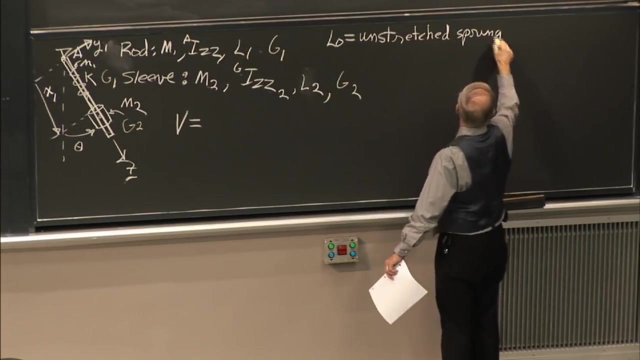 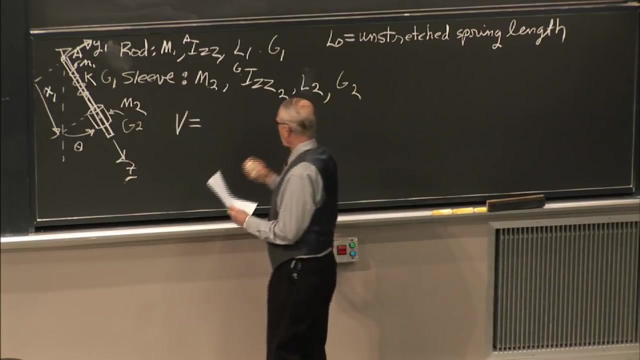 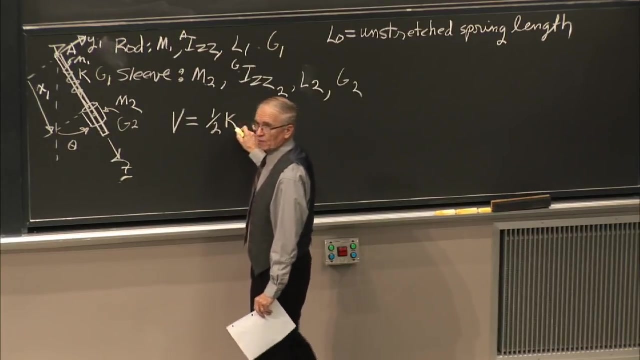 Because you have to pick references. You have to account for the unstretched length of the spring. So l0 is the unstretched spring length. OK, We know that also. So I propose that the potential energy look like 1 half for the spring anyway, 1 half the amount. 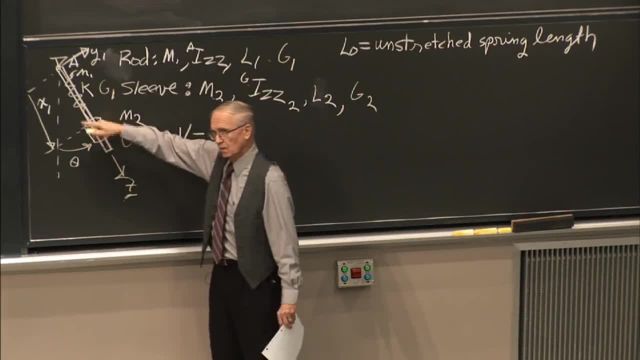 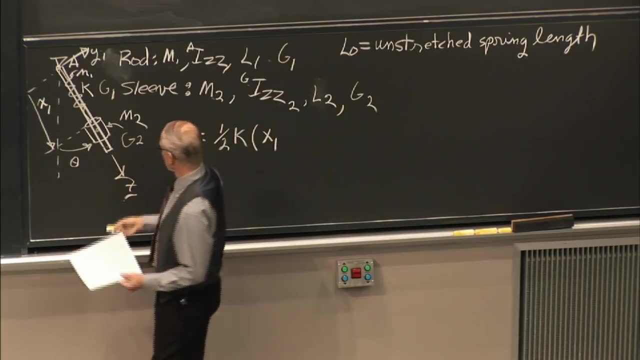 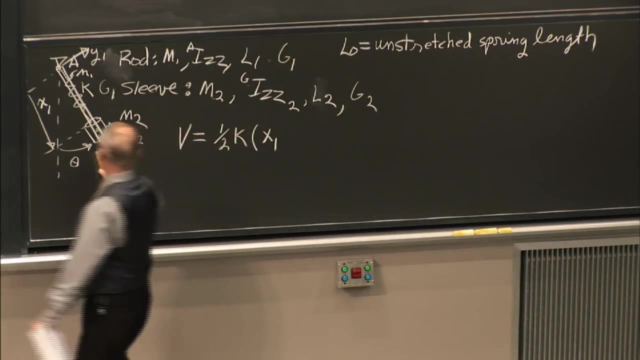 that it stretches in a movement, x1.. The amount that it stretches then should be whatever that x1 position is And that x1 position. I drew it slightly incorrectly. I'm going to use x1.. I'm going to locate the center of mass, which. 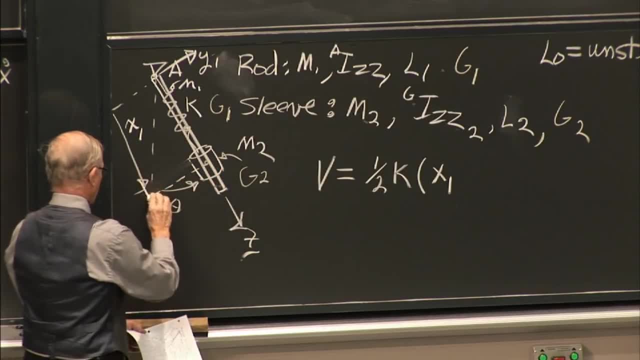 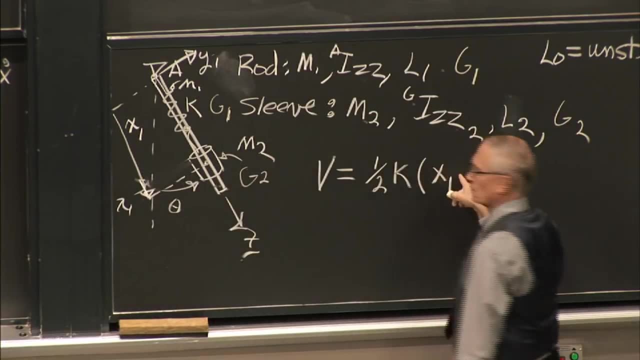 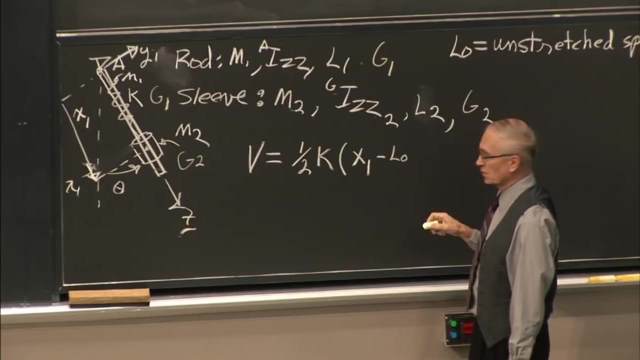 is always a good practice. So here's the center of mass. So my x1 goes to the center of mass. That's x1.. So that's the total distance And from that we need to subtract l0, the unstretched length of the spring. 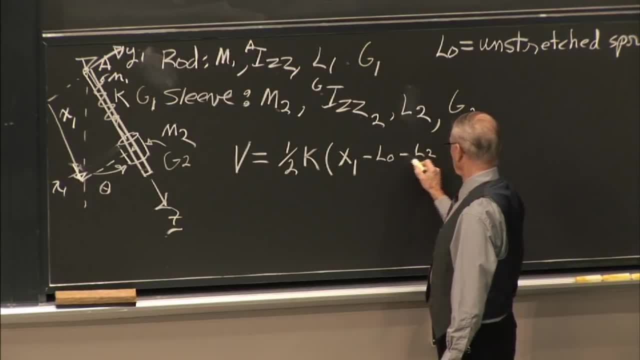 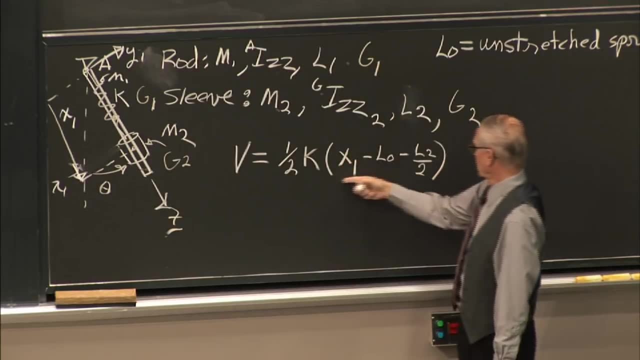 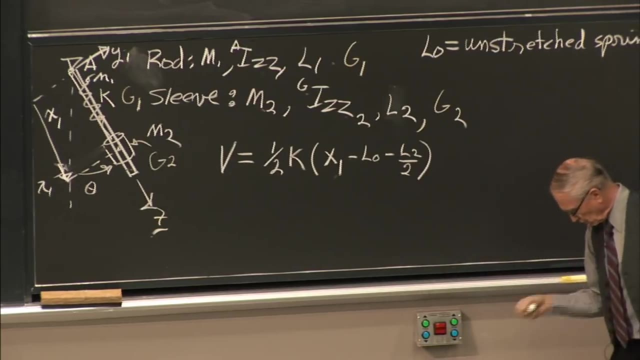 And we need to subtract half the length of the body because that's that extra bit here. OK, So this is the amount that the string is actually stretched when you go through a motion, when the coordinate is x1.. And you've got to square that. 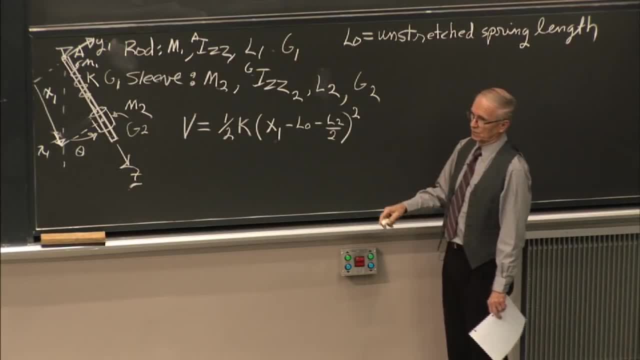 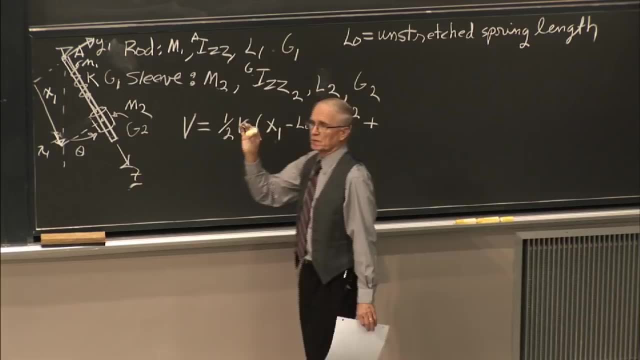 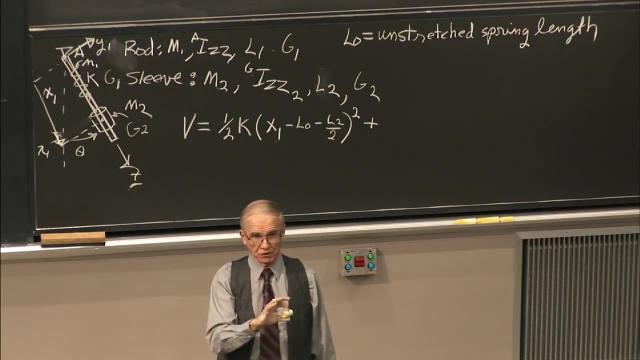 And that would be the potential energy stored in the spring. Then we've got to do the same thing for the potential energy. We have two sources of potential energy due to gravity, And they are two objects, right, Two objects, Two objects. 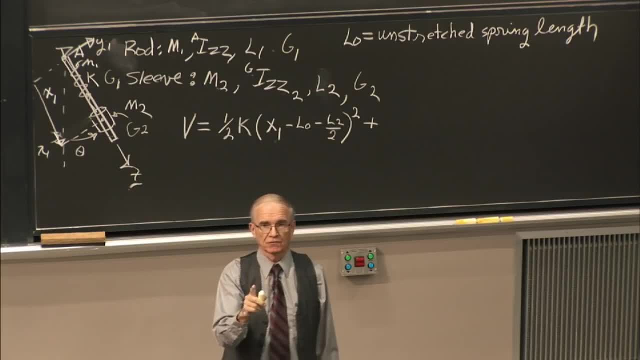 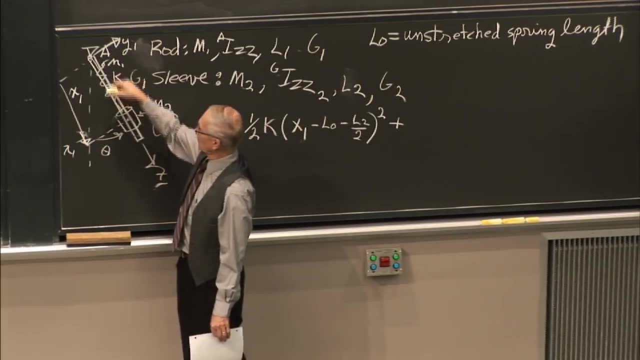 Two potential energies. So why don't you take a minute and tell me the potential energy associated with the rod? So the rod has a center of mass And the center of mass it's a pendulum basically. So it's the same as all the pendulum problems. 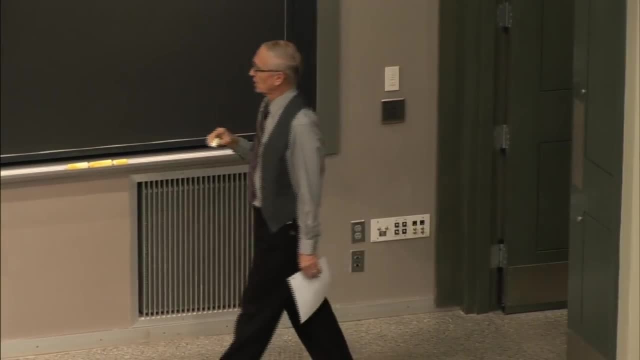 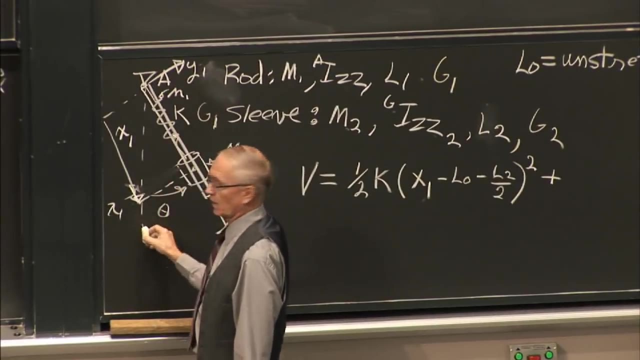 you've ever seen, And I would recommend that we use as our reference position its equilibrium position hanging straight down. And I'll tell you in advance: I'm going to use the unstretched length, I'm going to use the unstretched spring position this time. 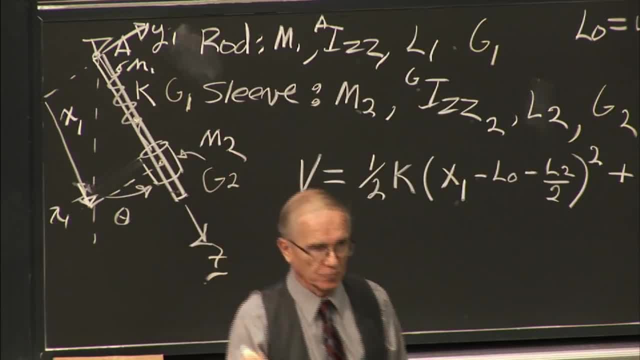 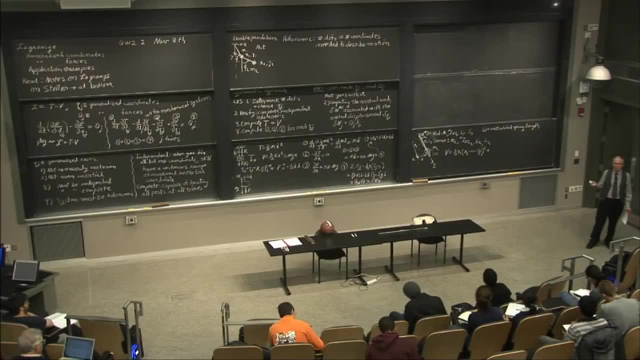 I'll just stay with that. That's where it's going to start from. That's my reference for potential energy. But does the unstretched spring position have anything to do with the potential energy of the rod? No, OK, So its reference position is just hanging straight down. 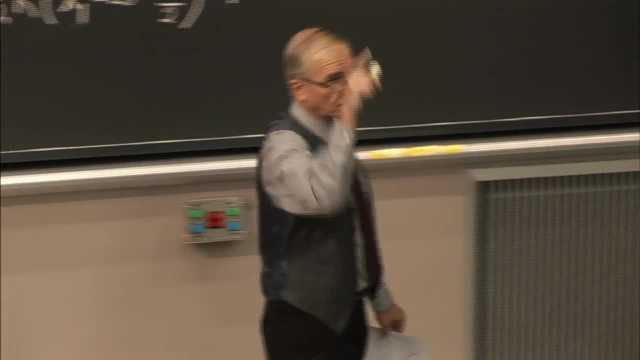 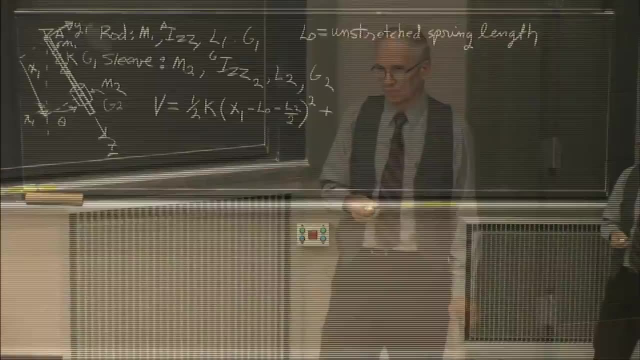 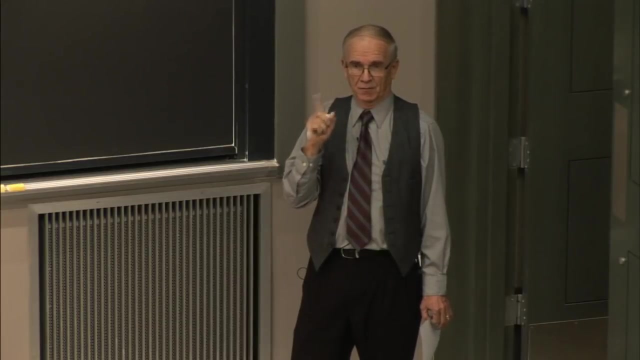 So figure it out. What's the giving a potential energy expression for just the rod part? Think about that. So I'm going to remind you about something about potential energy. Potential energy: one of the requirements about it is the change of potential energy from one position. 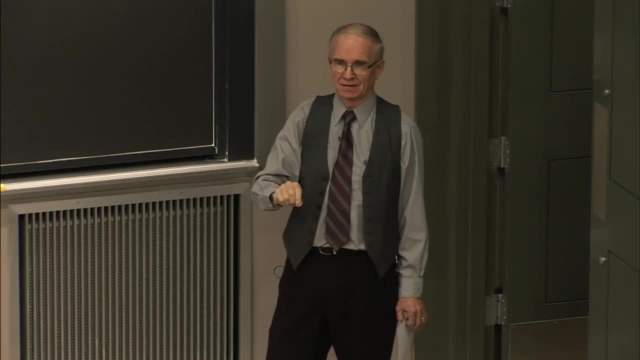 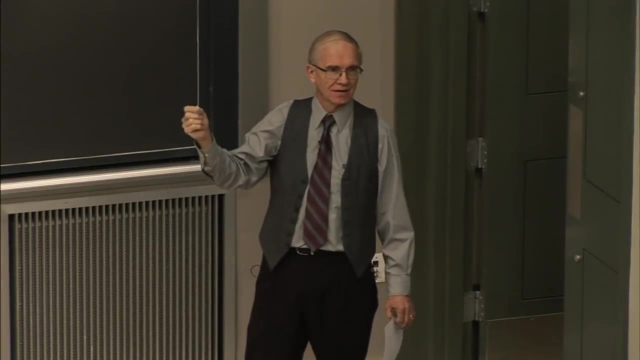 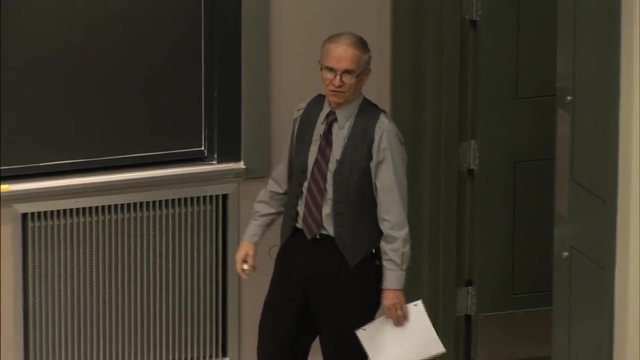 to another is path independent. So you don't actually ever have to do the integral of minus mg dot dr. You don't have to do the integral, You just have to account for the change in height between its starting end position and its some other position. 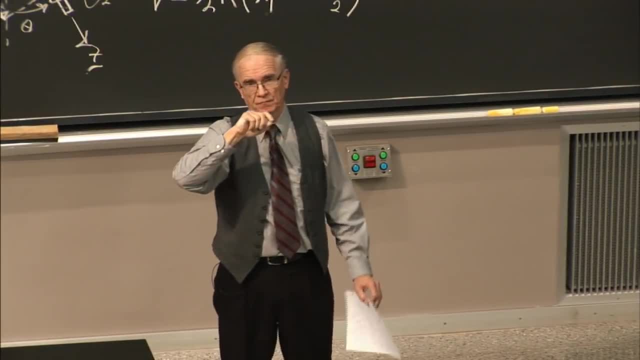 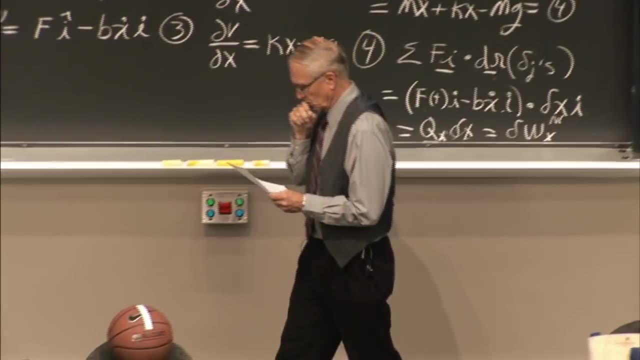 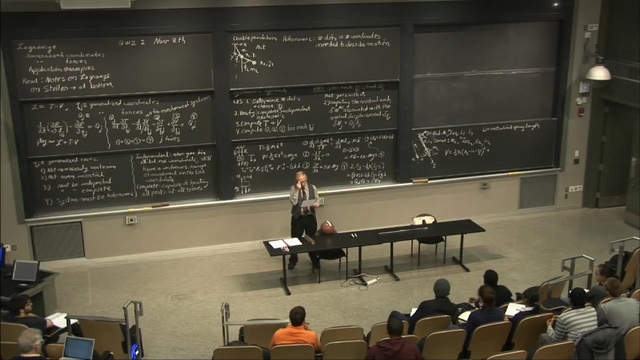 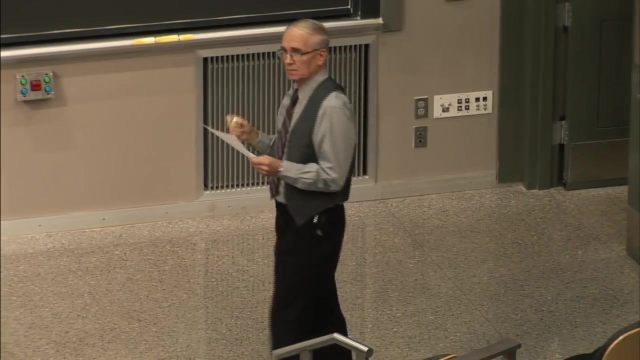 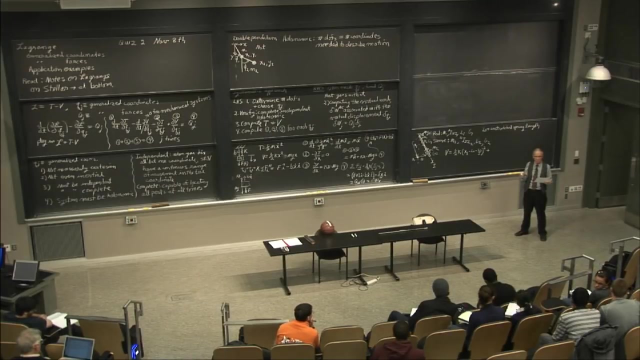 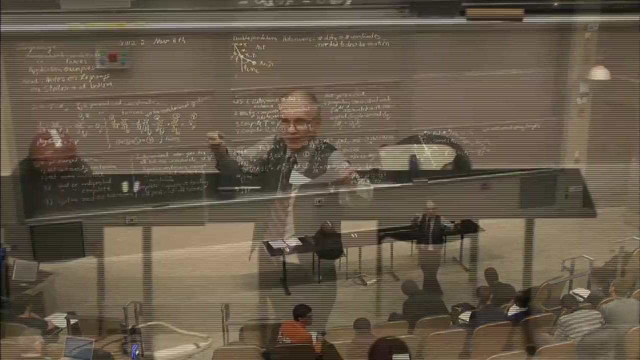 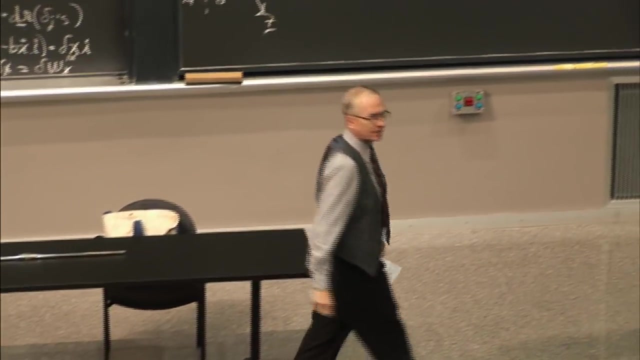 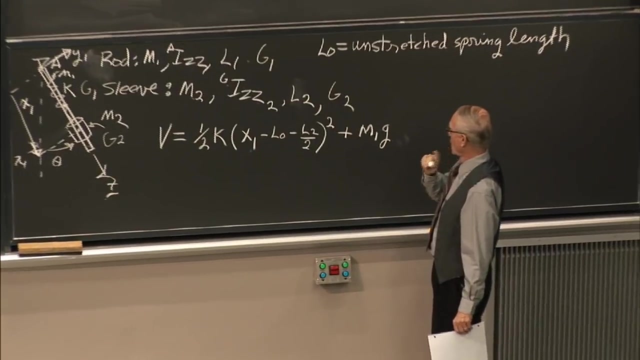 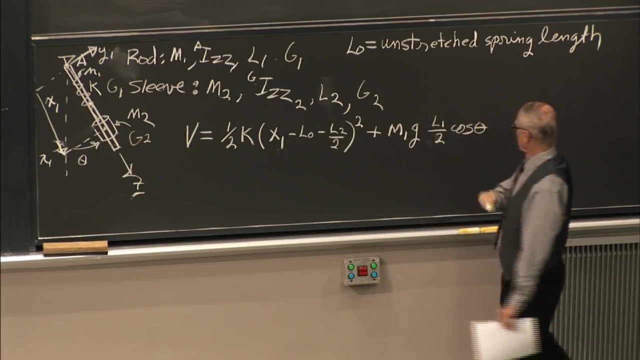 Spend a minute or two thinking about that. Work it out. You got a question. OK, So you have a suggestion for me, ladies. Yeah, Huh, It would be m1g times l1 over 2.. OK, Anybody want to make an improvement on that? 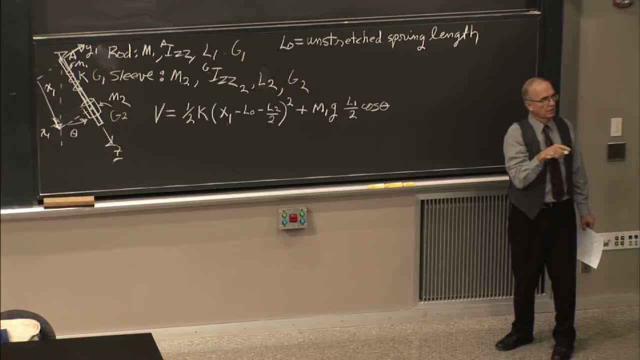 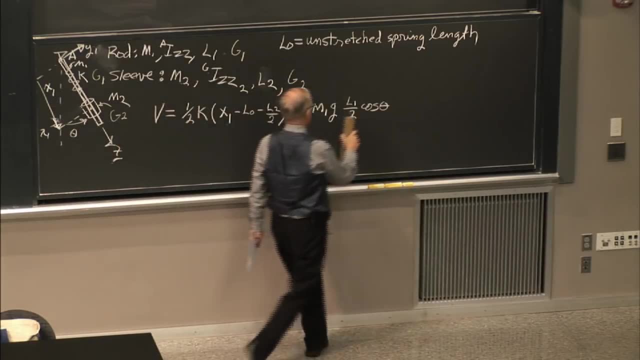 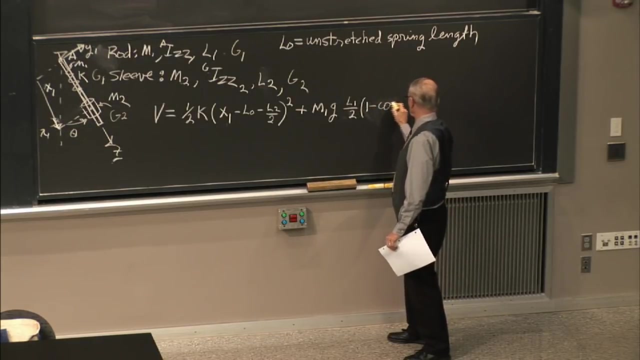 Or do they like it? Improvement: 1 minus cosine Cosine theta. So let's put that up and let's figure out if we need that. So it could be because we have a bid for cosine theta and 1 minus cosine theta. 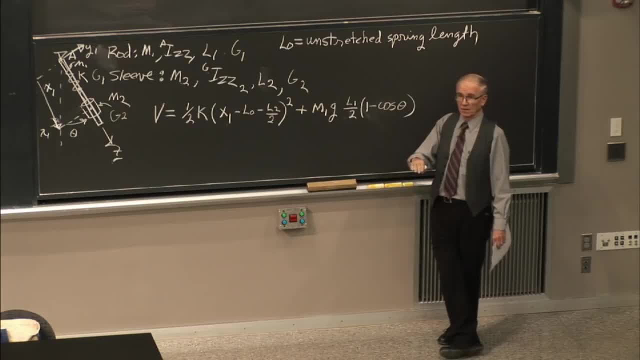 So you need to have a potential energy at the reference and you need to have a potential energy at the final point, And the difference between the two is a change in potential energy here. OK, So the reference potential energy is mg over 2.. 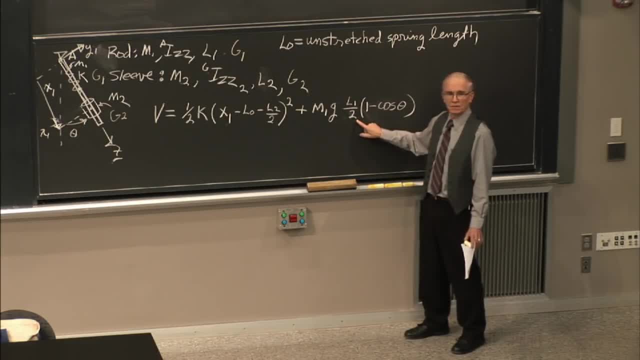 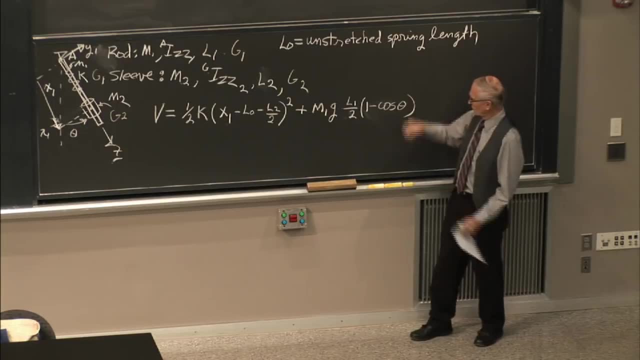 OK, Yeah, So it's going to be l1 over 2 when it hangs straight down And then when it moves up to this other position, the l1 over 2 times. this is delta h. This is the change in height that it goes through. 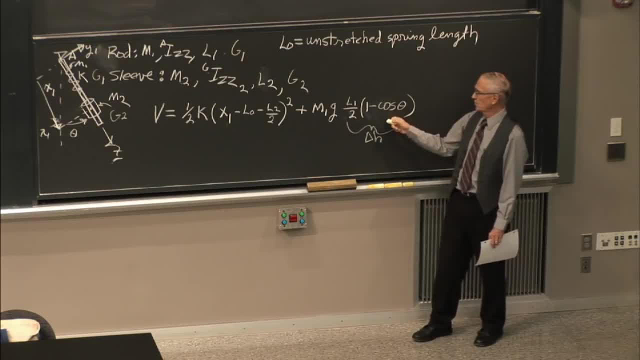 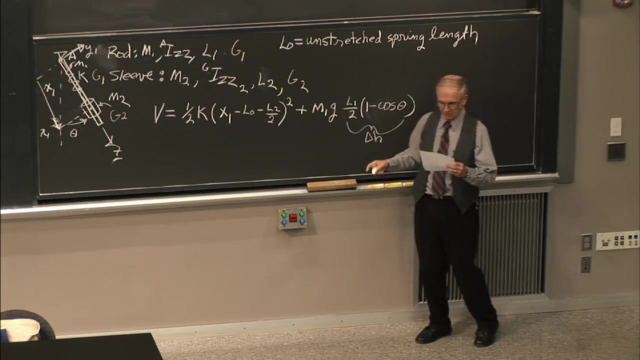 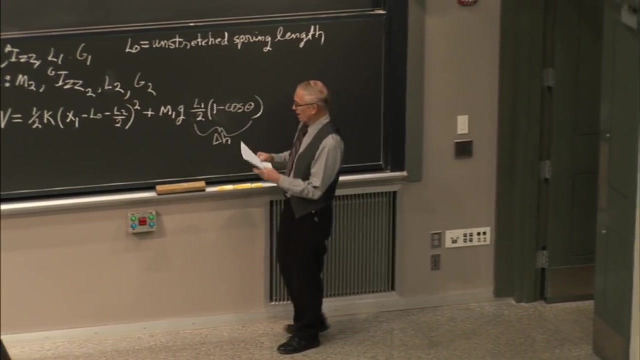 So you need the 1 minus, right? And why is it? and do we have the signs, right? Yeah, OK, So now we need another term and I'll write this one down. We need a little. this one's a little messier. 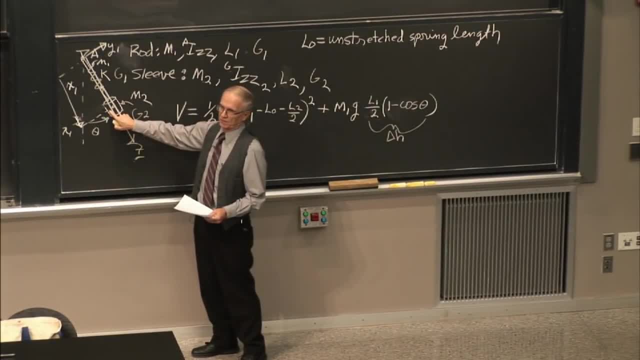 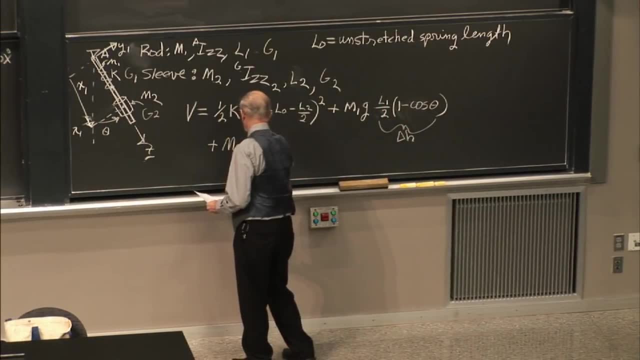 We need a potential energy term due to gravity for the sleeve, And that's going to mimic this. You're going to have a term here plus m2g And that's going to mimic this. You're going to have a term here plus m2g. 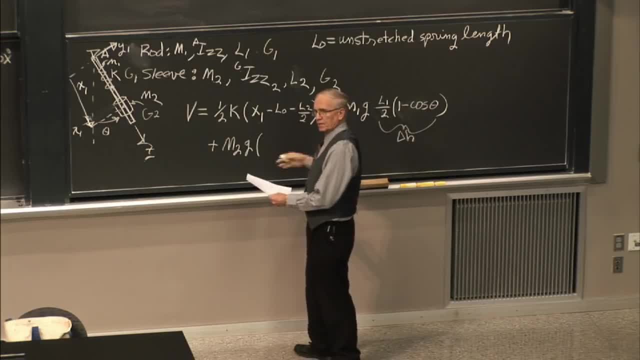 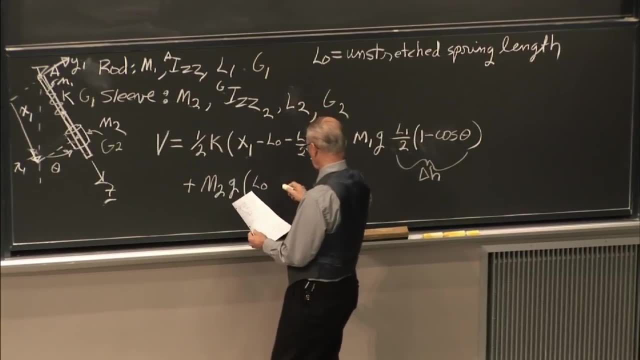 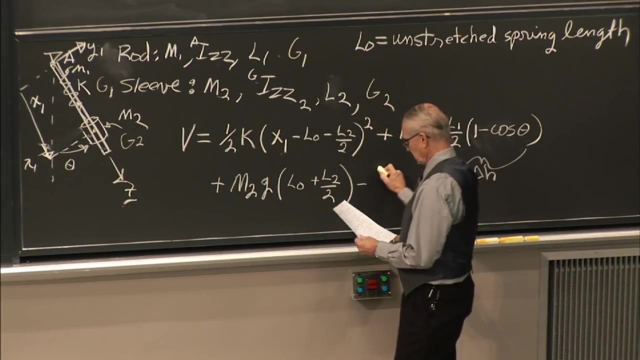 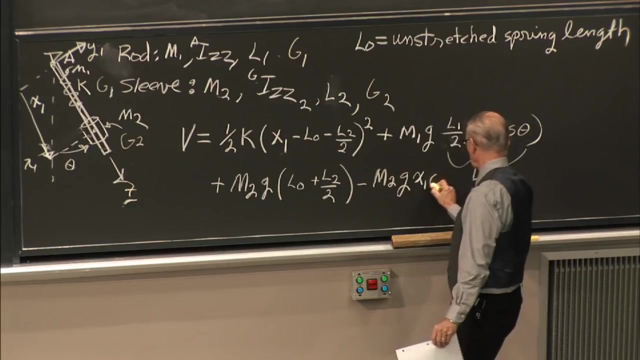 And its reference. I'm just going to do it as a reference amount minus the final amount. The reference will be at the initial location of its center of mass, which is l0 plus l2 over 2 minus m2g x1 cosine theta. 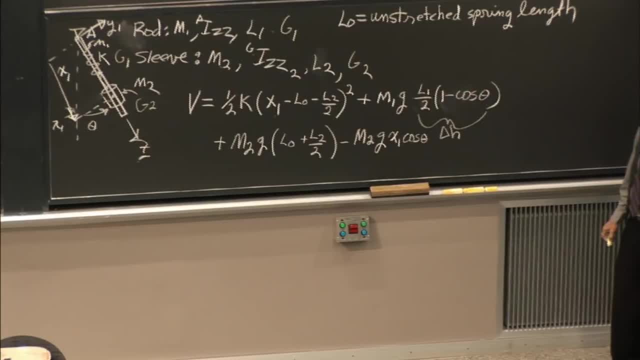 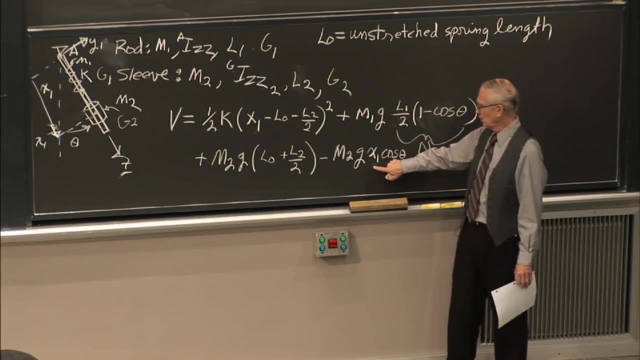 And then we'll calculate it, Because this one gets a little messier. because you've got this thing, It can move up and down the sleeve And if that moves you've lost your reference. So you can't do this as a concise little term like this. 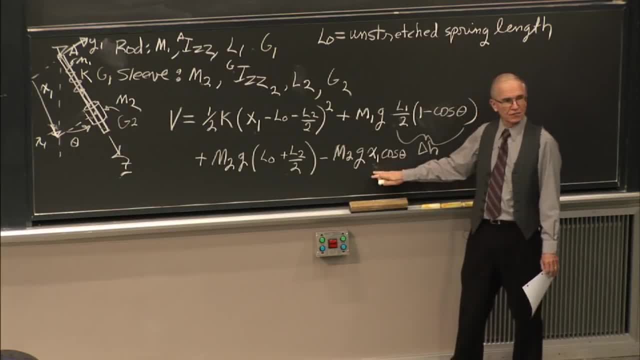 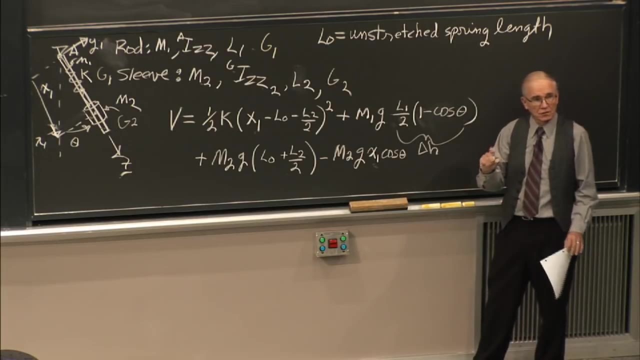 You have to separate out the reference. and then this is the final And the l0 plus l2,. this quantity here is the starting height, This x1 cosine theta, It is the finishing height And the difference between the two gives you the change in the potential energy. 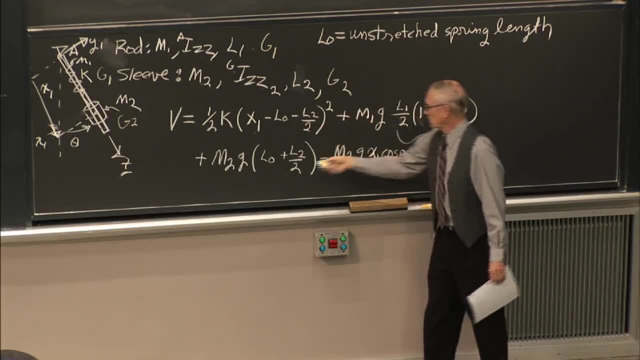 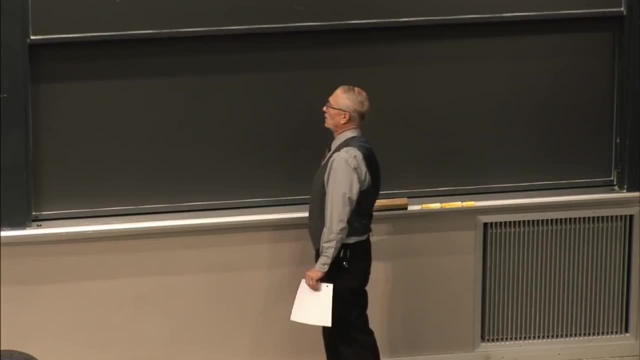 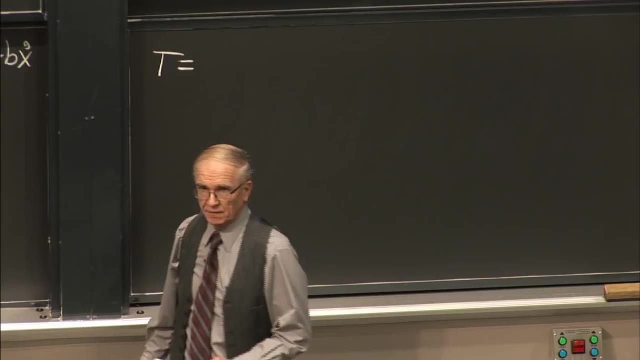 So this is your potential energy expression. This plus this plus these. All right, So what about t? We've got to be able to write it. Kinetic energy is generally easier. You've got to count for all the parts and pieces. 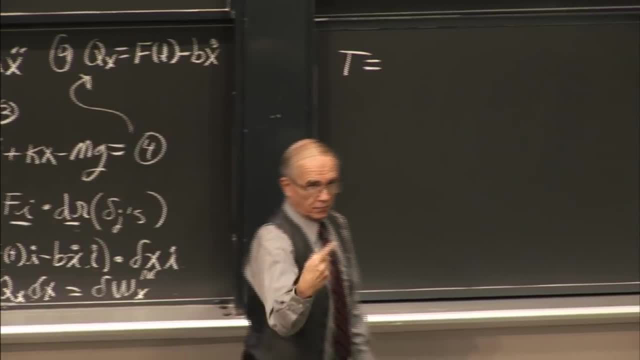 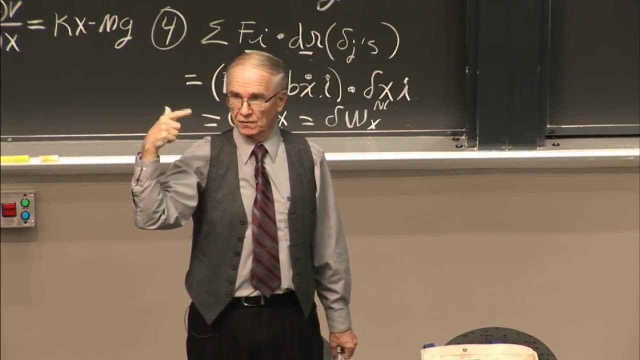 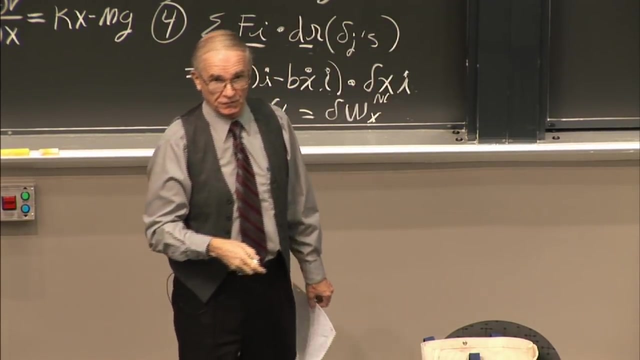 We have two chunks and we're going to have rotational kinetic energy associated with the rod, Rotational kinetic energy associated with the sleeve, But also some translational kinetic energy associated with the sleeve right, And I'll write these terms down: 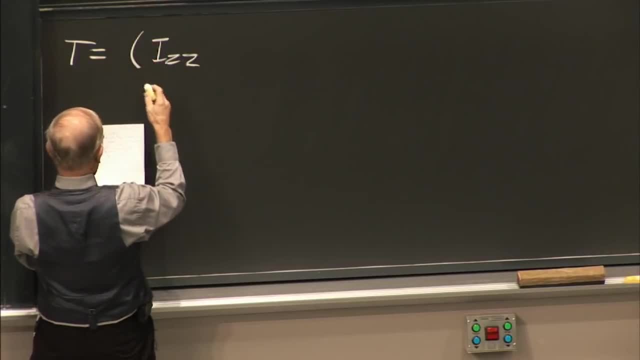 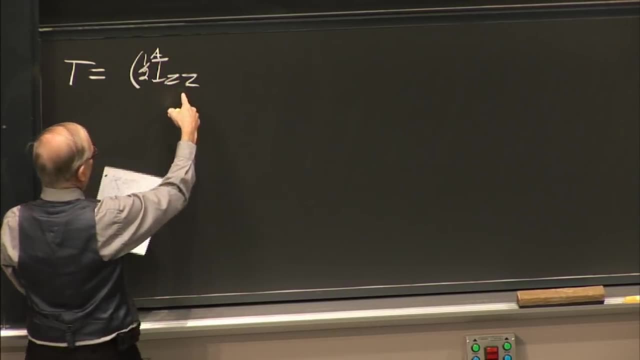 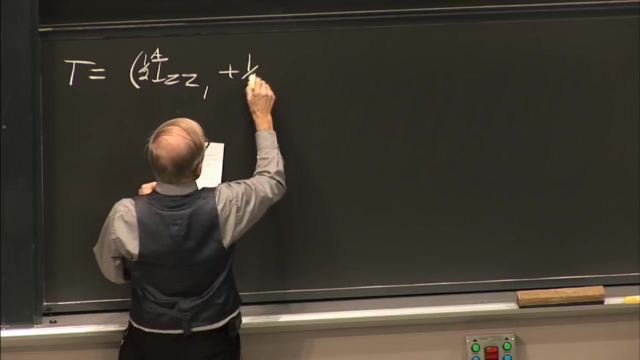 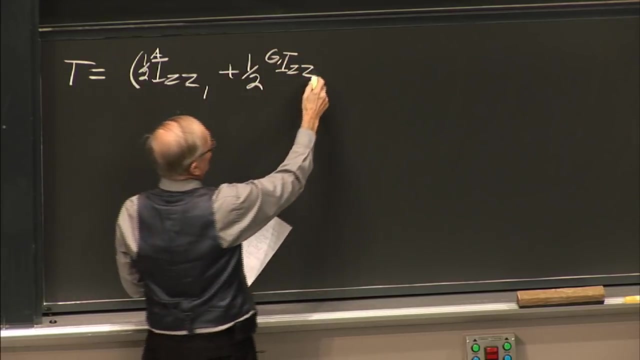 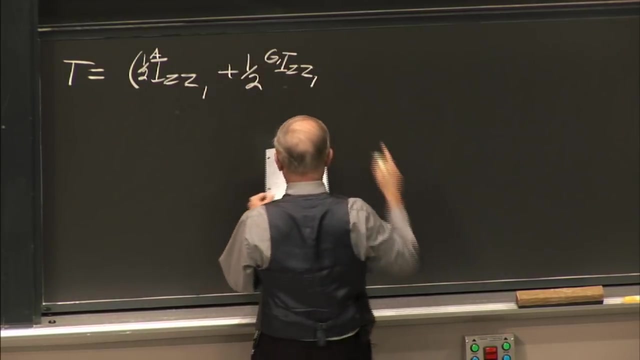 And I've made the problem go a little faster here. 1 half Izz about A, That's the first, That's the rod, Plus 1 half Izz for the sleeve about g, And we'll discuss why the difference here. 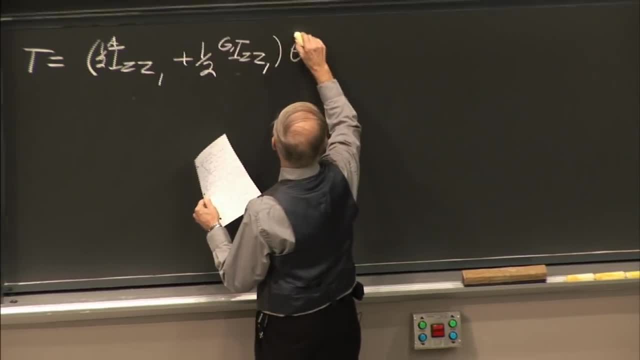 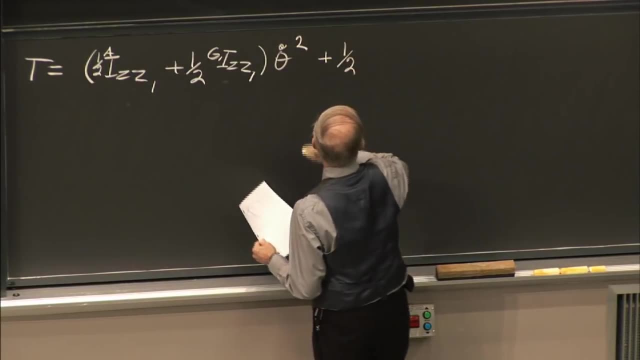 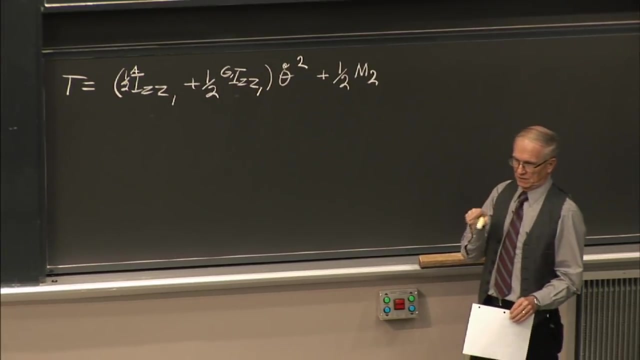 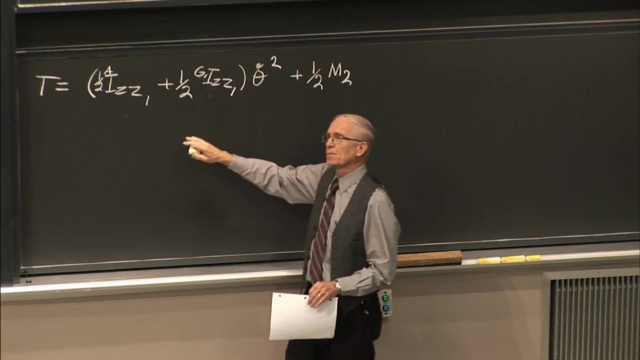 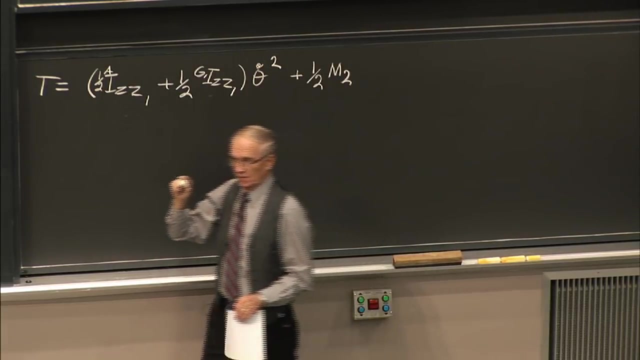 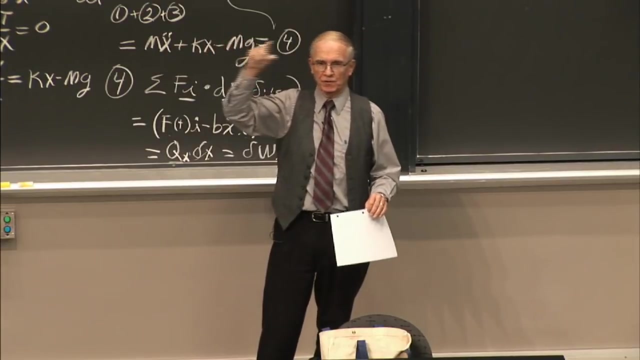 And that's theta dot squared Kinetic energy. that comes from translation of the center of mass. Because I'm broken up, I've accounted for it. Let me start over. This system is pinned about A And the rod is just simply pinned at A. And the last lecture I put up. 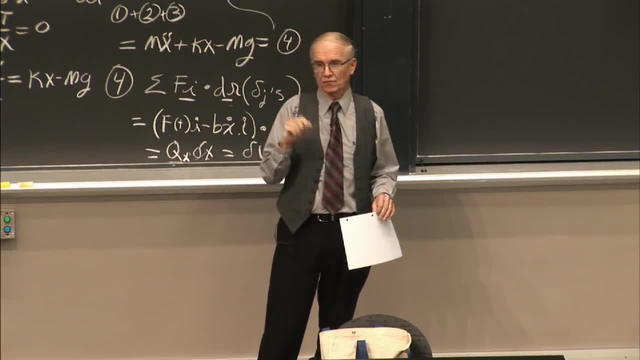 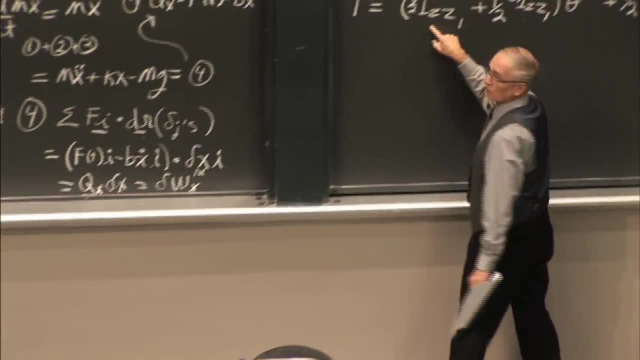 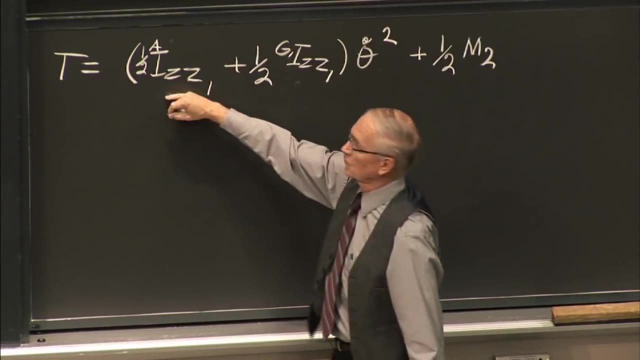 these different conditions, simplifications. You can account for something about a fixed pin by computing mass. moment of inertia about A. It's basically a parallel axis theorem. argument Times 1, half times that times theta dot squared. So this gives you all of the kinetic energy in one. 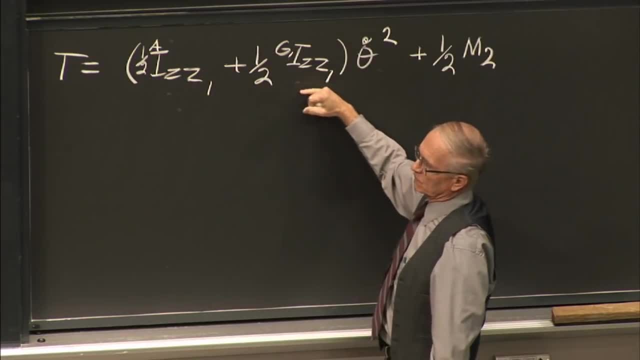 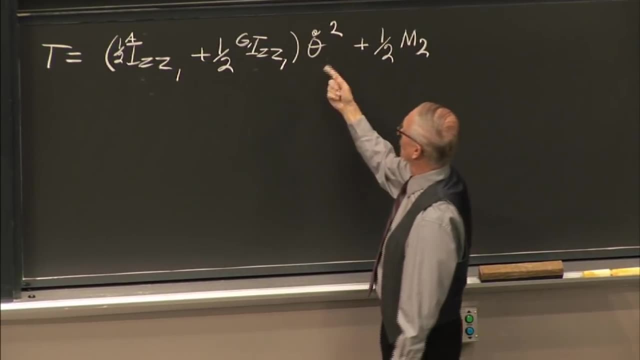 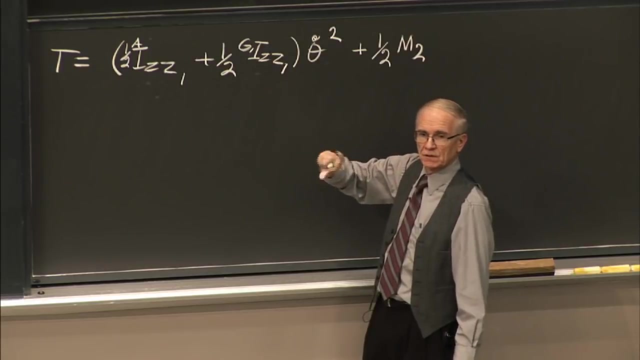 go with the rod, But for the sliding mass, because its position is changing, you can't do that. You have to account for the two components of its kinetic energy separately. This accounts for rotation about g, even though g is moving. That accounts for that energy. 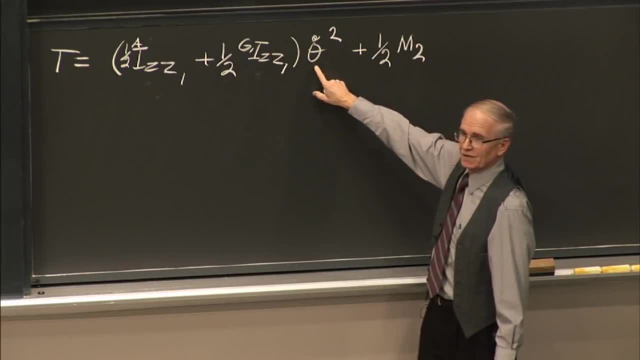 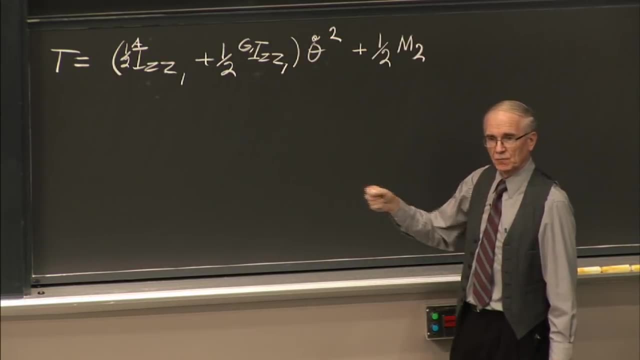 This accounts for, because it's only a function of theta dot. It's not a function of that position x. This term is going to account for, then, the kinetic energy associated with the movement of the center of mass. So we need a, v, g, 2.. 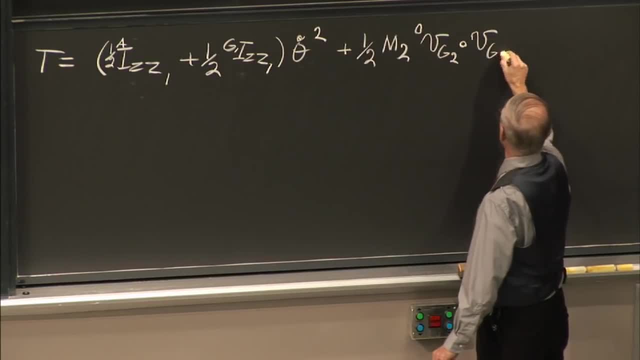 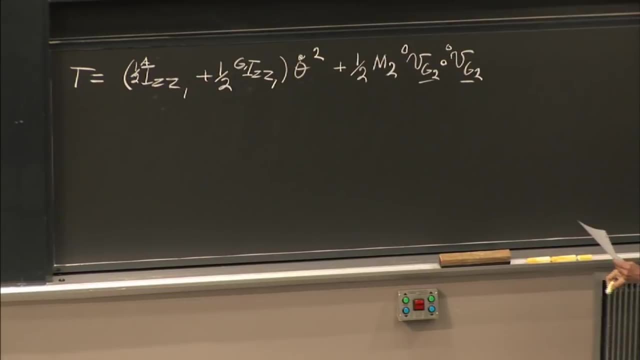 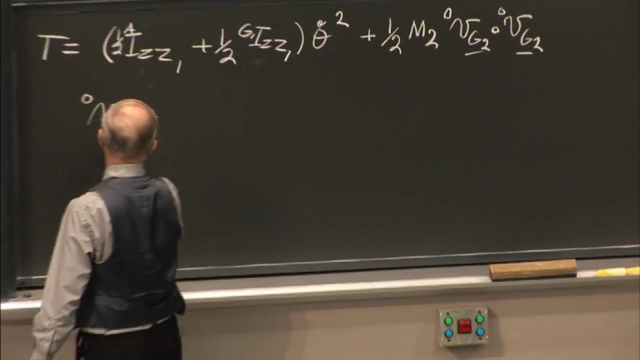 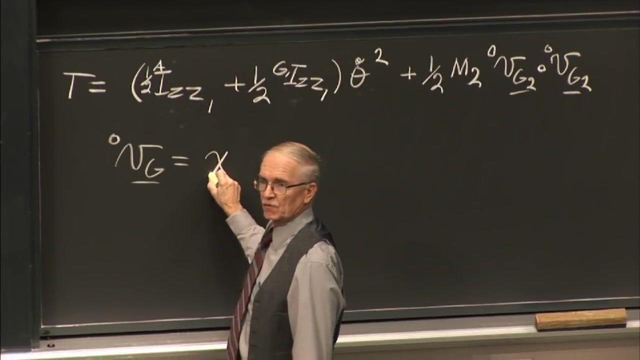 In the inertial frame, dot v g 2,, these being vectors. And does that get everything? I think that does. So v g o is it certainly has a component that is at speed sliding up and down the rod right. 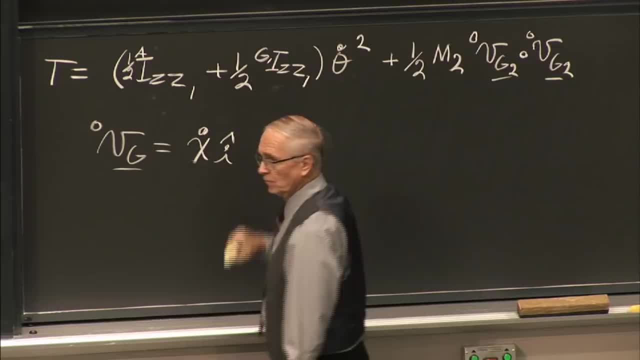 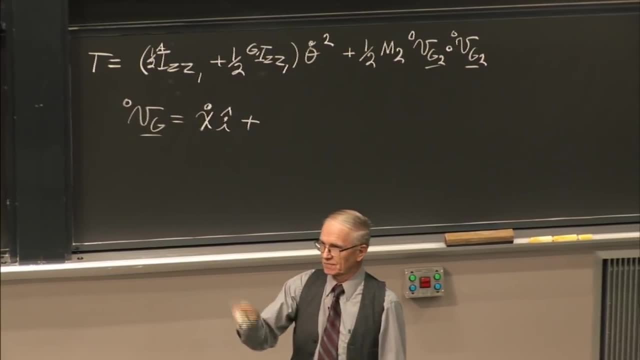 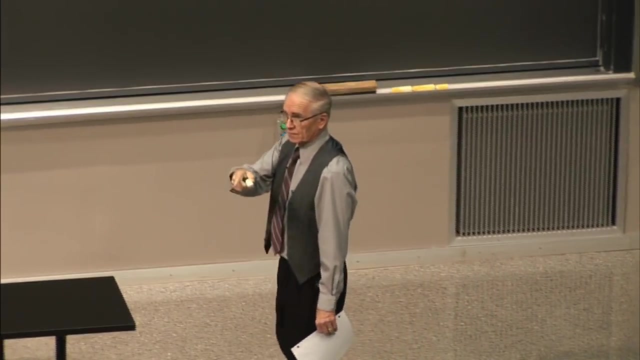 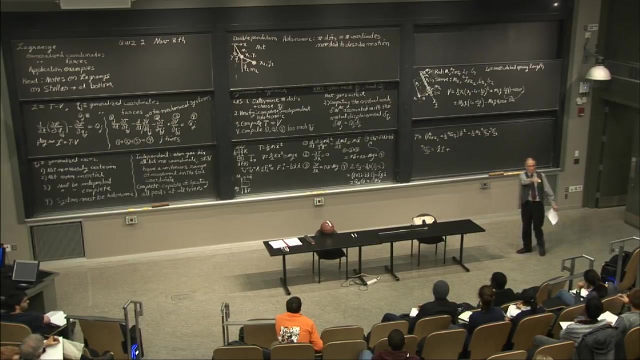 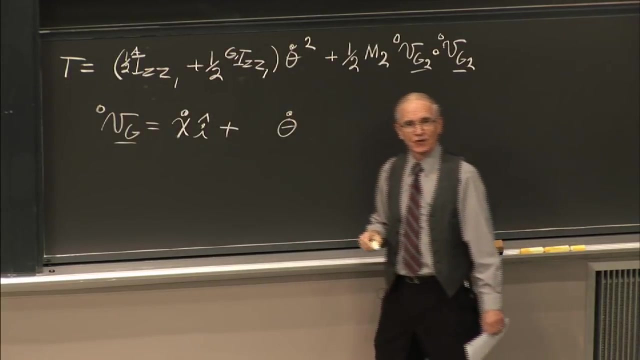 And that's in the i hat direction. But it has another component. due to what? Can you tell me what it is? It's contribution to its speed, due to its rotation. It's got a theta dot. yep, It needs an r right. 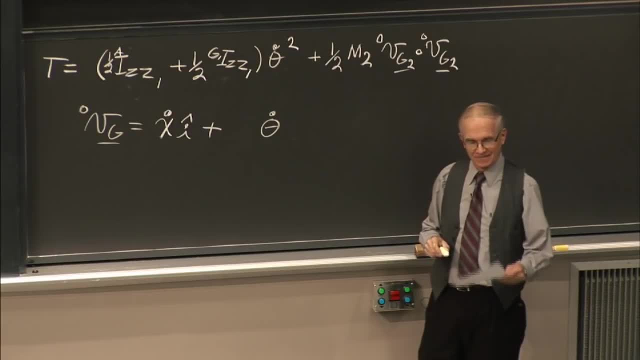 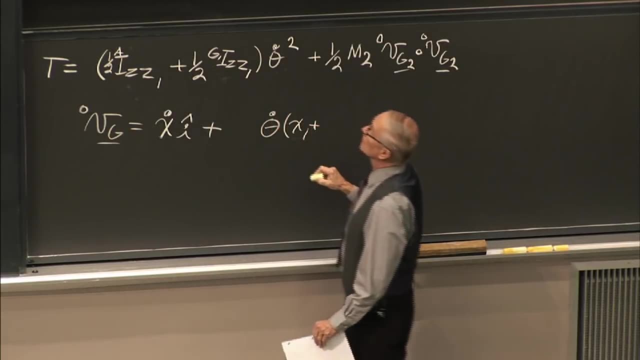 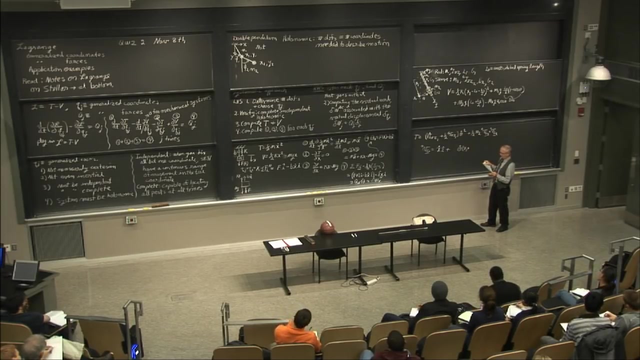 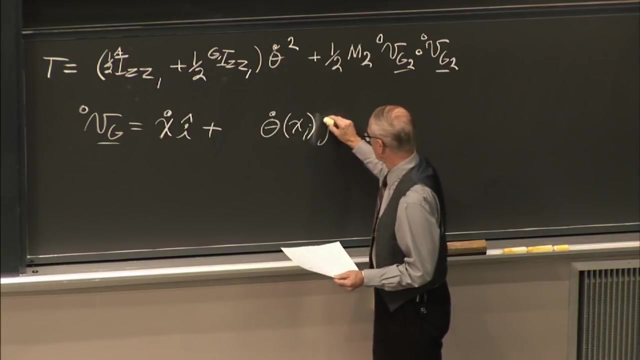 Yeah, so this would be an x1 plus. no, actually I made x1 go right to the, so just x1. theta dot. In what direction? Yeah, so j hat here right The moving. it's actually that's. 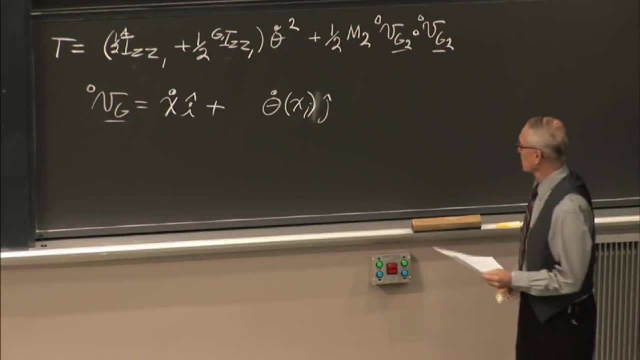 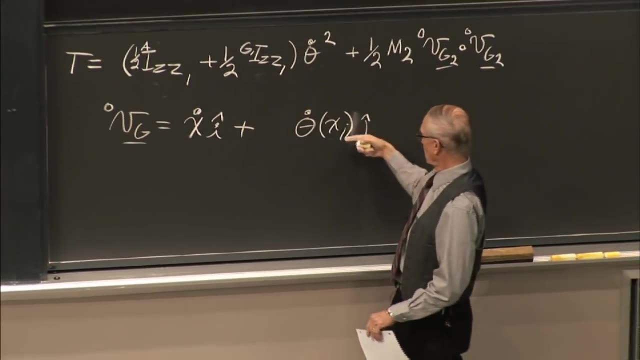 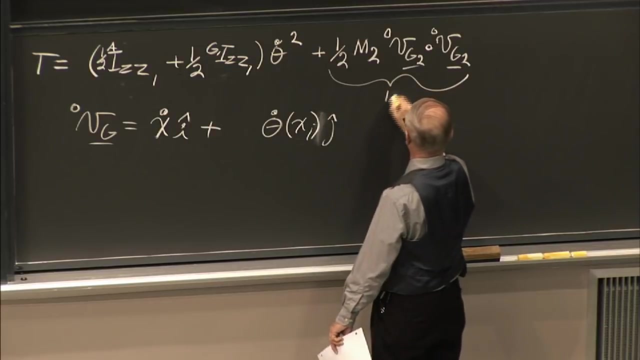 the moving coordinate system unit vector. It's in the y direction And so we do the dot product. You get this times itself: i dot i and j dot j. You get that. this quantity here is 1 half m2 x dot squared. 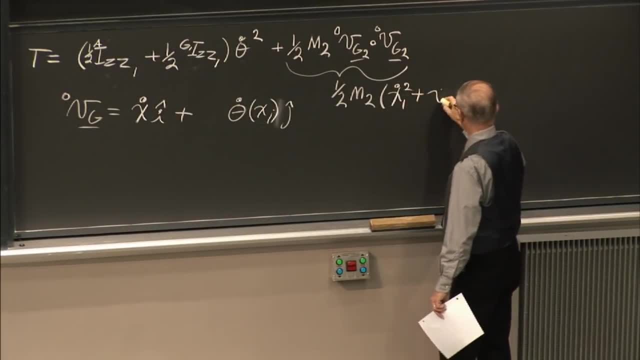 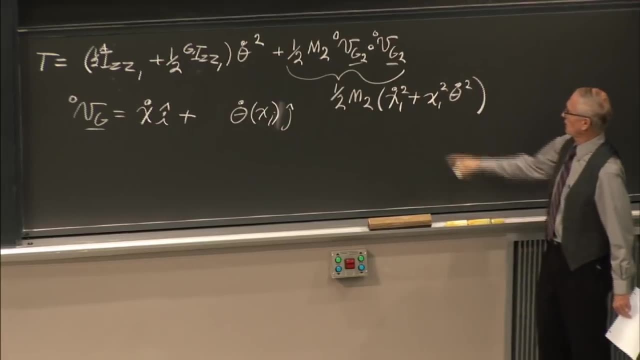 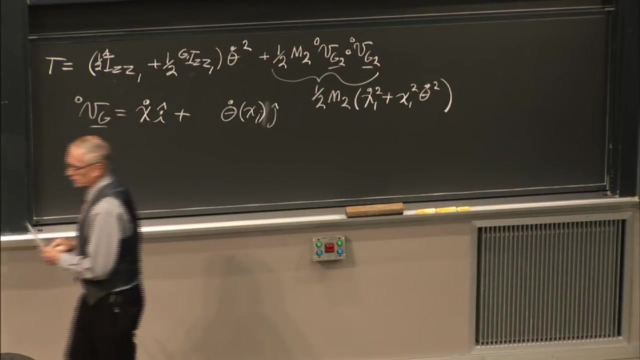 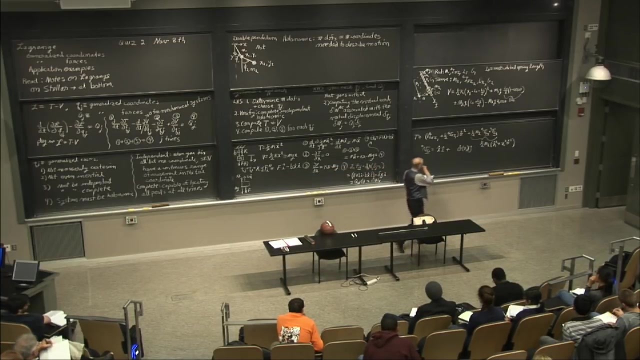 plus x, it's an x1, I guess x1 squared, theta dot squared, That's the kinetic energy of counting for the velocity of the center of mass. So now we have an entire kinetic energy expression. So now we have how many coordinates? 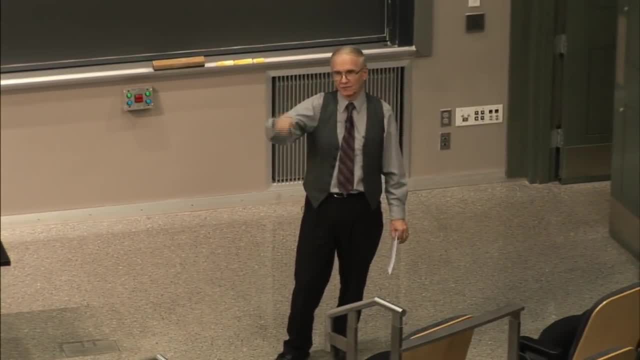 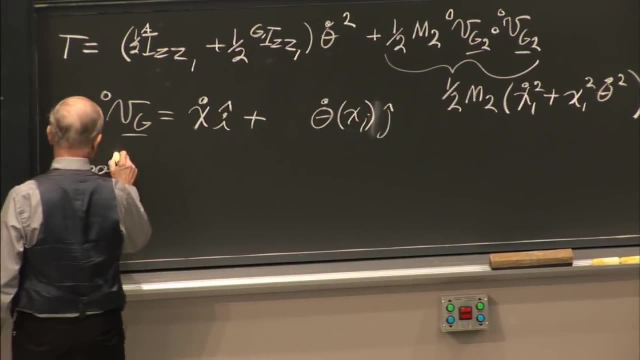 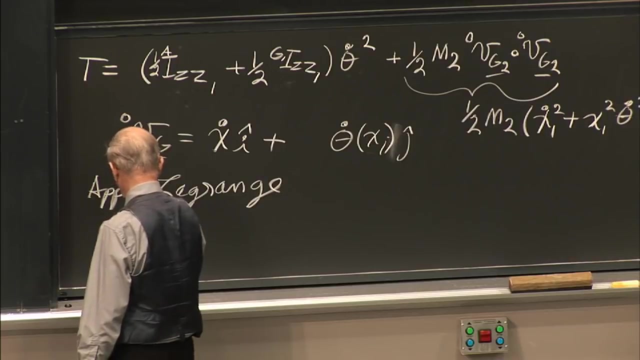 Two right. How many times do we have to turn the crank and go through the Lagrangian system? You've got to go through it twice. So let's apply, Let's apply Lagrange here and we'll just do number one first. 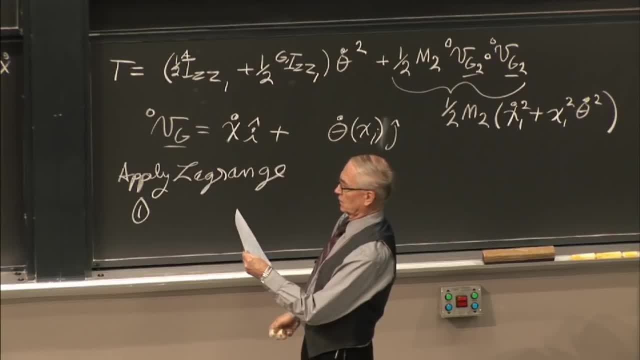 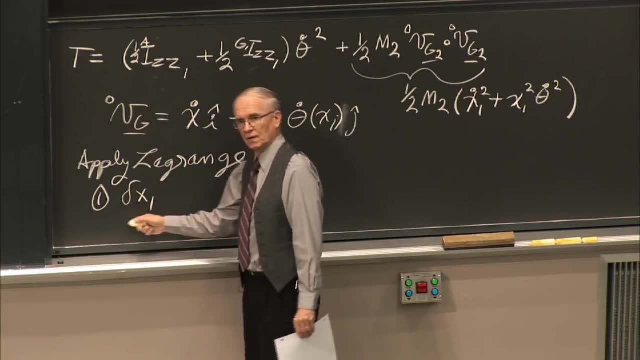 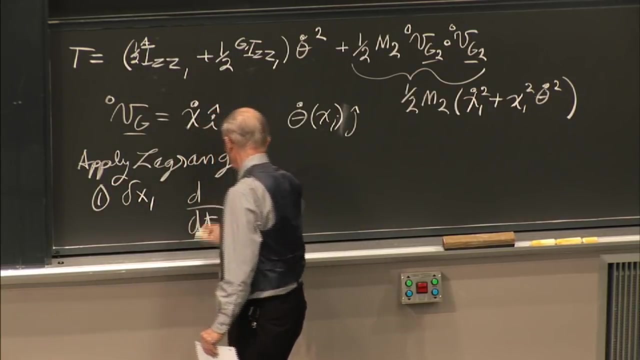 And let's see which one do I have on my paper. first, I guess we'll do the x1 equation. This is delta x1. So this is generalized coordinate x1. And we need to do term one, which is then d by dt. 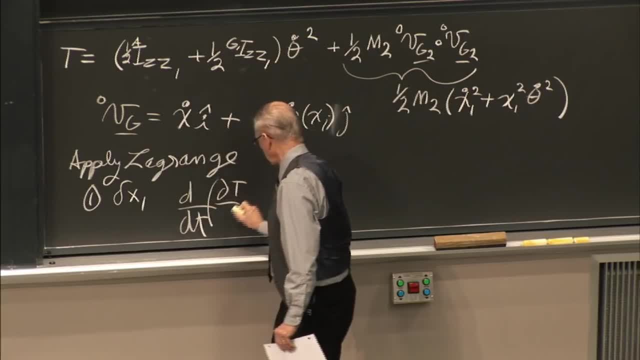 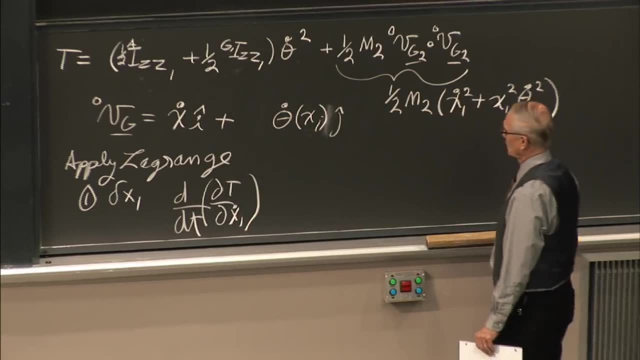 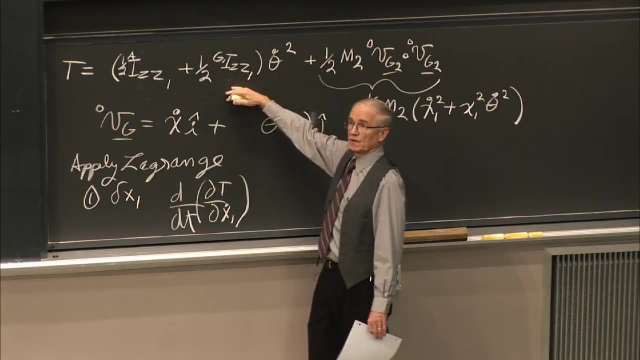 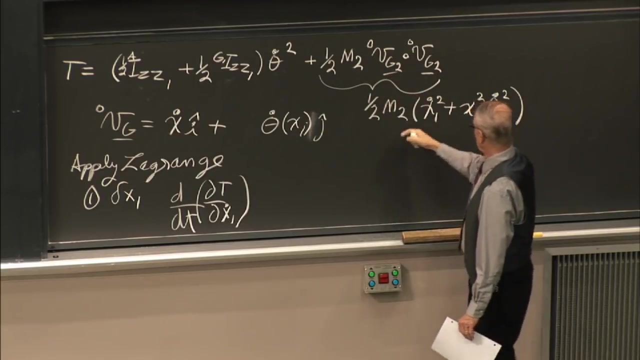 of Partial of t with respect to x1 dot. So we look at this and say, well, is this term a function of x? Nothing, You get nothing from there. Is this term a function of x? Yeah, it's down here. 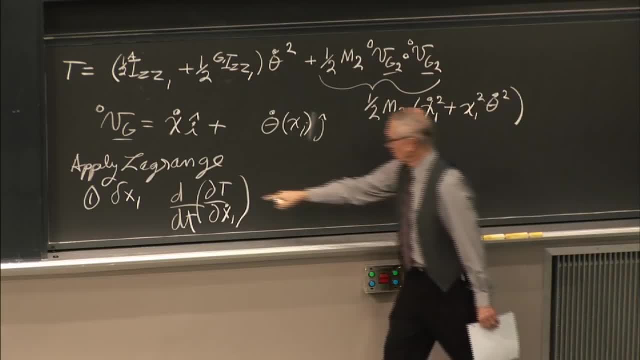 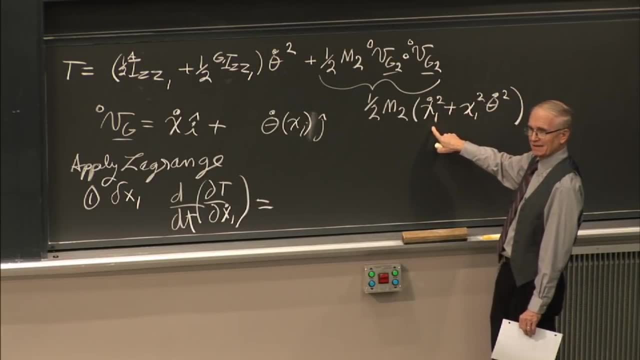 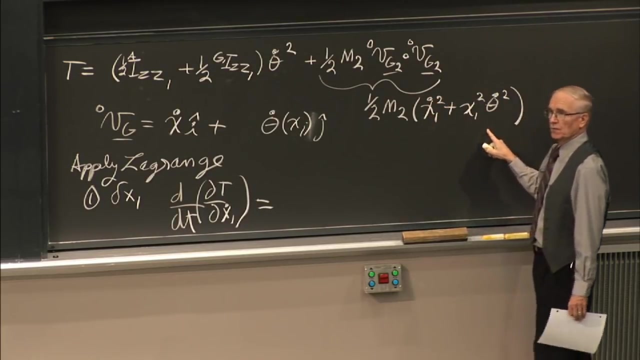 So we only have to take the derivative of this. We have to do that job. OK, So the derivative of this with respect to x dot. you get a 2x dot here. Do you get anything from here when you do this with the derivative with respect to x dot? 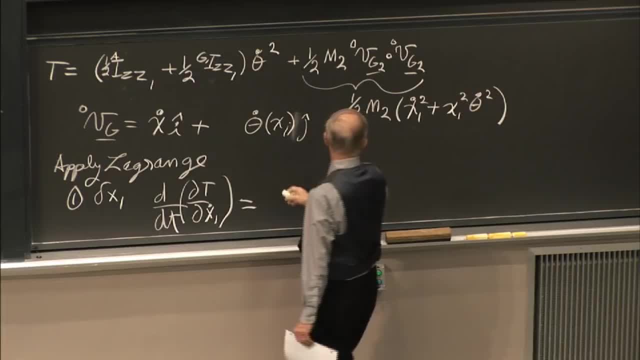 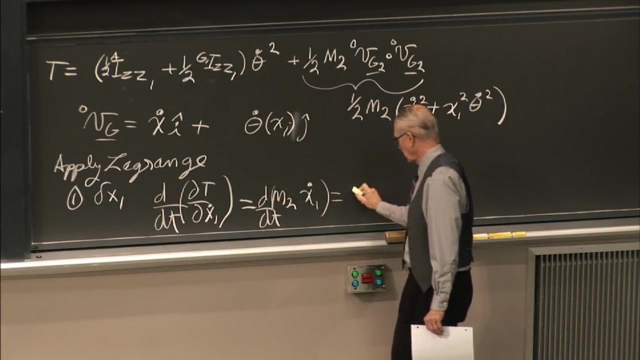 You only get a contribution from here. The 2 cancels that, And so this should look like m2 x1, dot, but d by dt, And I won't do this. I'll do this in two steps here, so you see what happens. 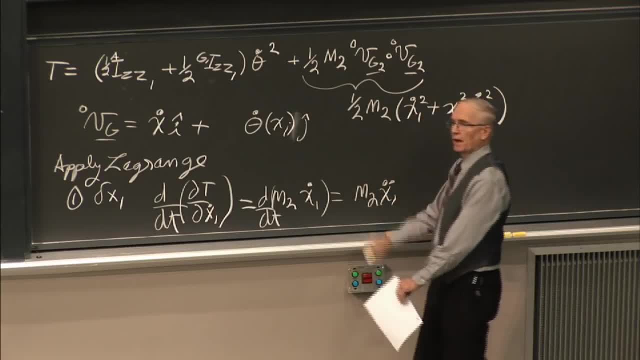 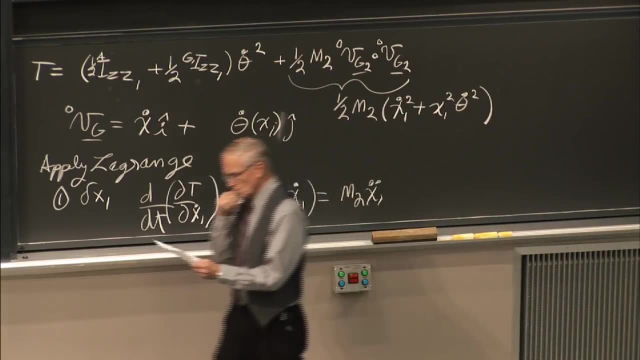 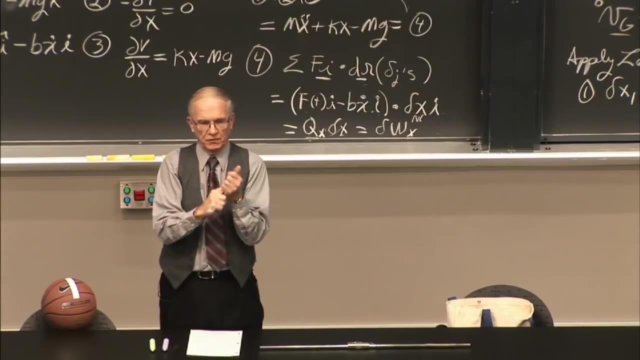 You get an m2 x1 double dot out of that. OK, So we've gotten the first piece of this. We've got a couple to go. But I want you to know a lot about Newton's laws And you know a lot about calculating equations of motion. 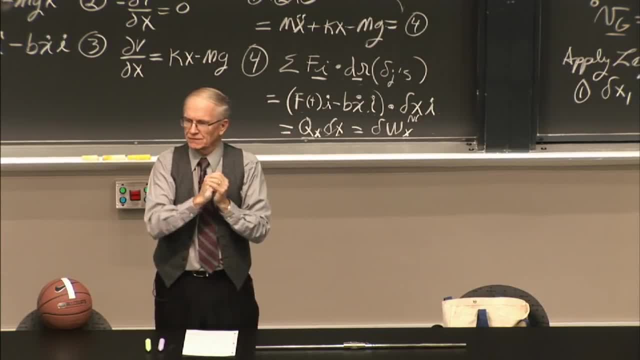 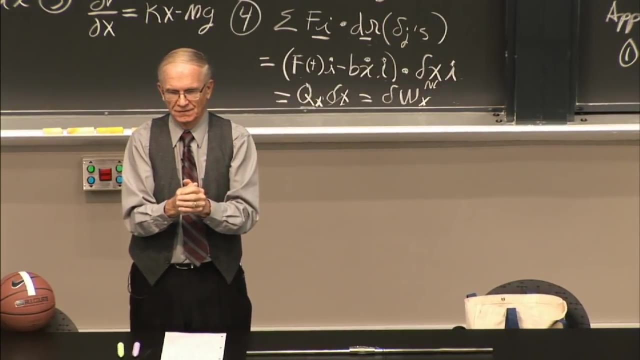 now We're using sum of torques and all that stuff, right. So this is just something moving. It has circular motion, It has translational motion. What other accelerations had better appear in this equation of motion, And which equation are we getting? 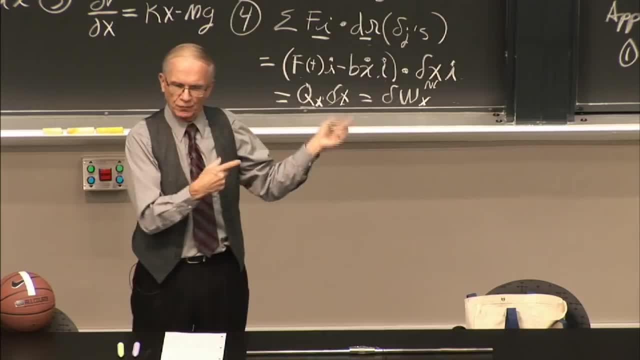 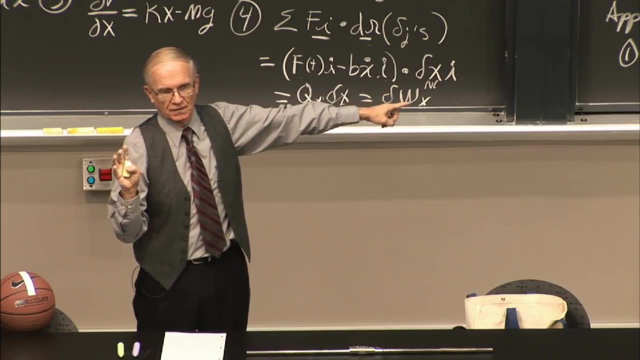 And there's going to be two equations And they have sort of physical significance to it. What equation does this begin to look like Just physically? What movement is being accounted for here? Looks like translation in the x direction. It's this thing sliding. 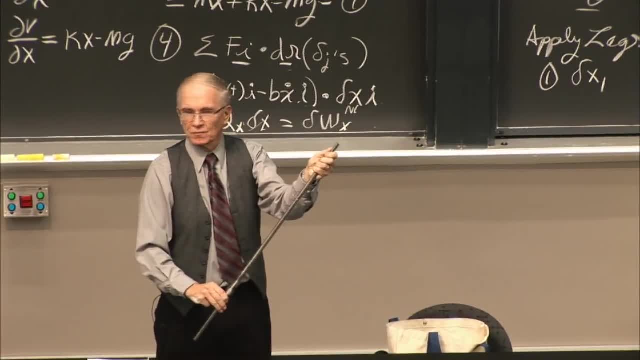 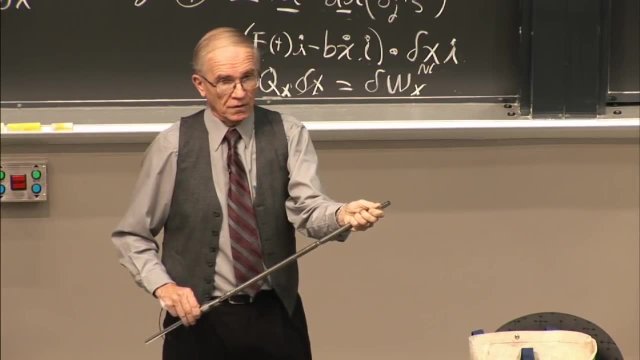 It's this part of the motion sliding up and down. You're writing an equation of motion And mx double dot has units of what Torque Force. So this is a force equation. This is just f equals, ma is what this is going to show us. 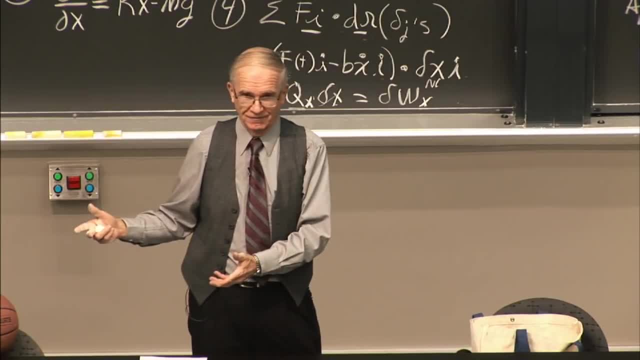 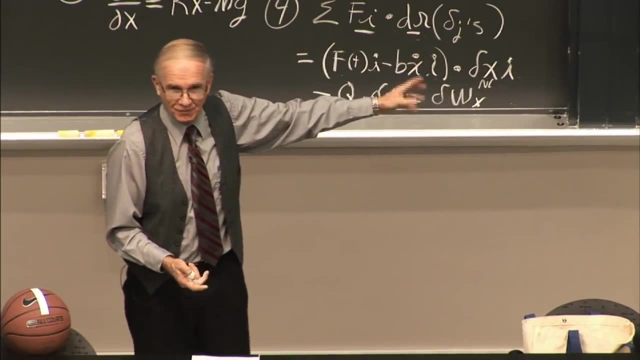 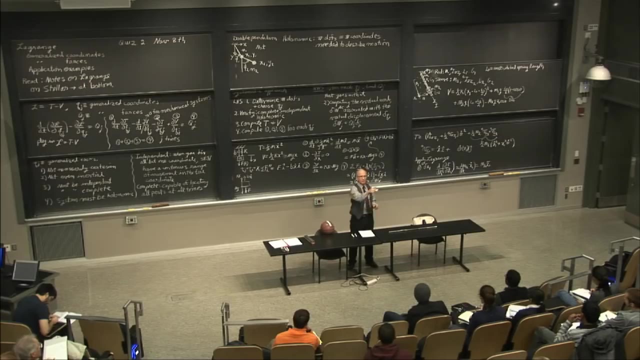 Remember, the direct method has to give you the same answer as Lagrange. So we're getting a force equation. It's describing mx double dot. What other acceleration terms do you expect to appear in this? from what you know, A centripetal term. 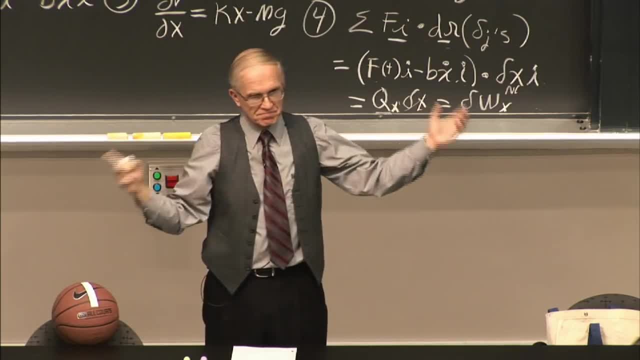 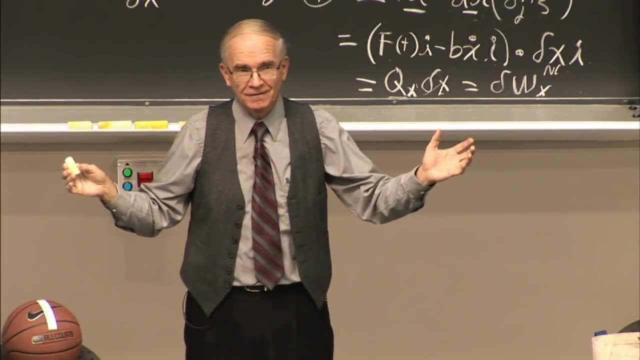 You believe there ought to be a centripetal term in this answer? Why? Because it's got circular motion involved, for sure. Any others? Is there any Coriolis in this? In this direction, Which direction are we working in? 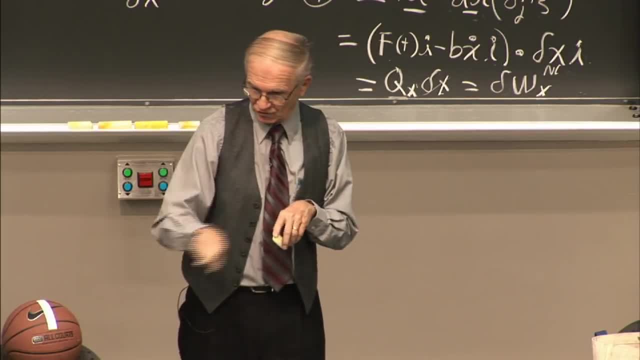 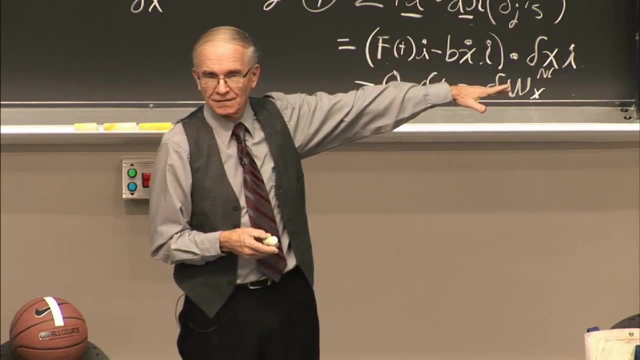 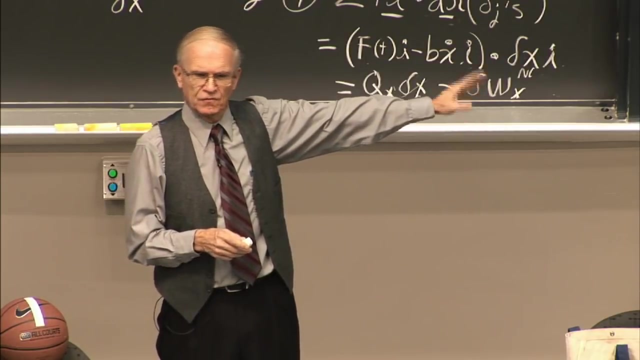 Is there Coriolis acceleration in the x direction. By the way, these equations, do we have any ijk's in here? These are pure scalar equations, No vector, no unit vectors involved. Did this equation only describe motion in the x? 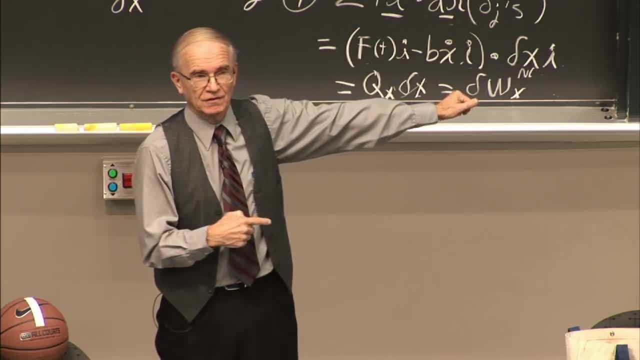 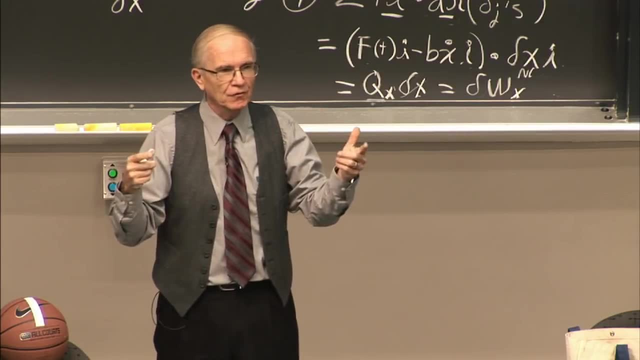 So will there be a Coriolis force in this acceleration, in this problem? Will there be an Eulerian acceleration? No, There's no Eulerian acceleration in this equation of motion. The reason I'm going through this is I want you to start developing your own intuition about 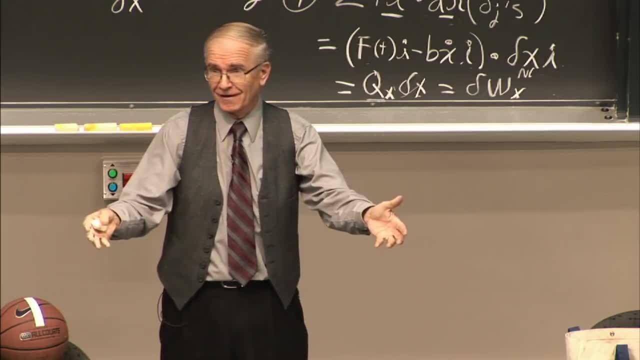 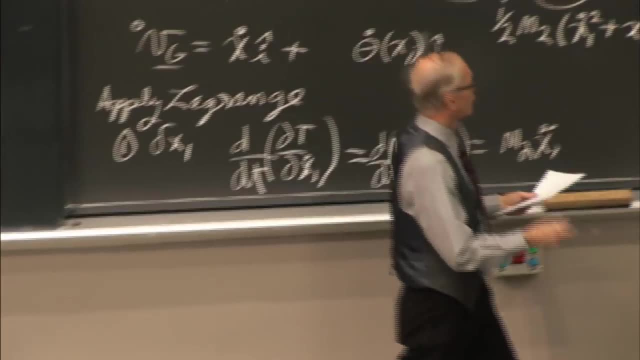 whether or not, when you get it at the end it's got everything it ought to have and doesn't have stuff it shouldn't have. OK, So you're forecasting that we better get a centripetal term. Well, let's see what happens. 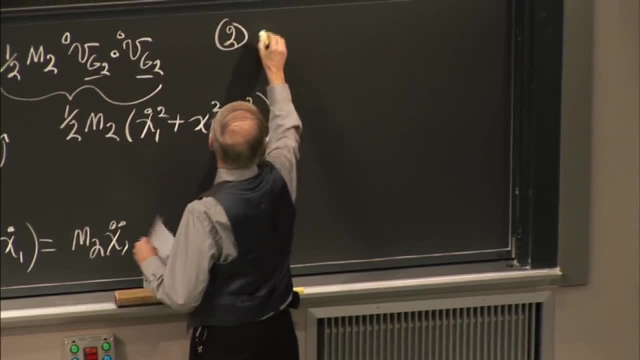 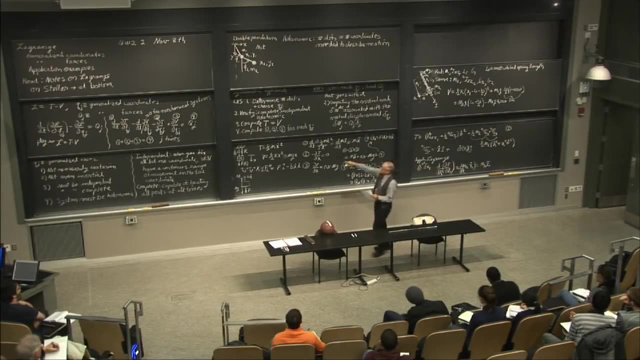 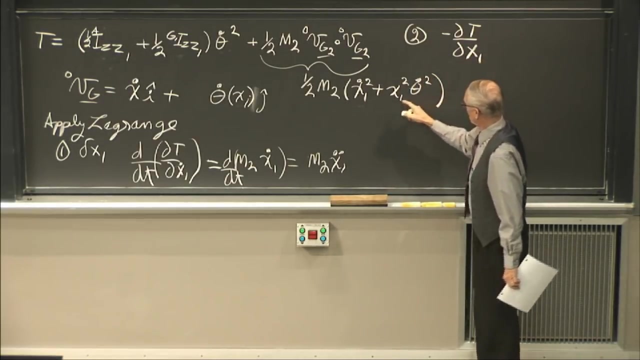 So that was number one. Number two: here is our dt by minus the derivative with respect to x in this case. So we go here: x1 we've been calling it. Is this a function of x, this piece? Nope, it's x dot. 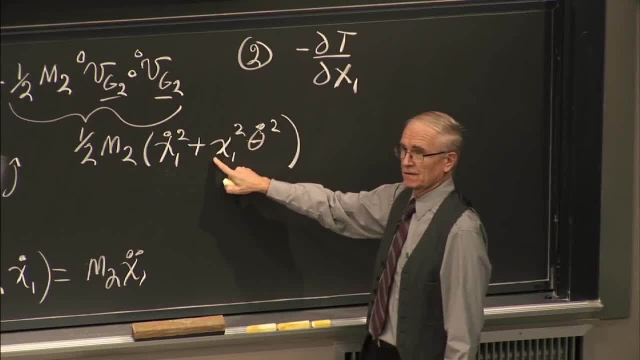 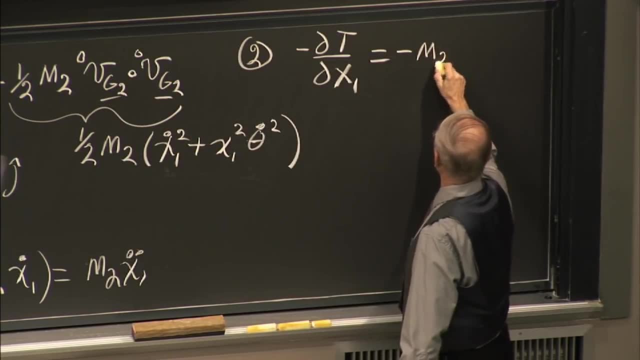 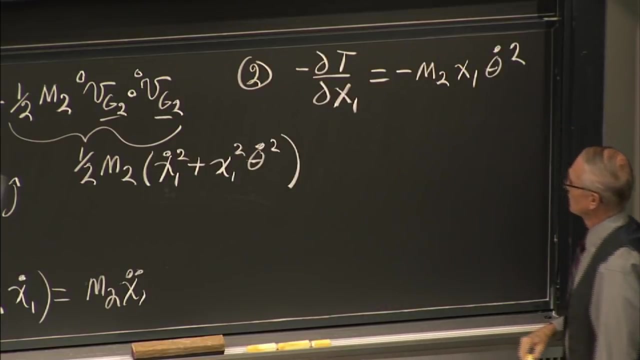 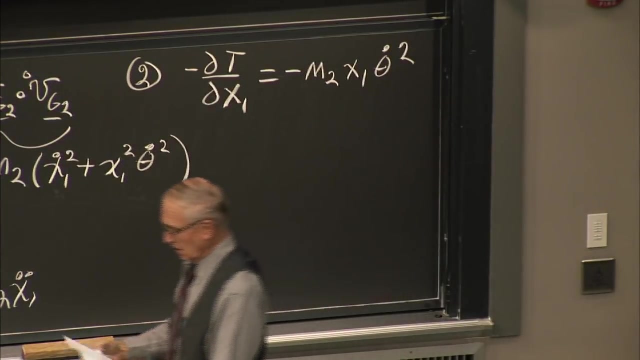 How about this one? Right, Take this derivative. you get 2x. So this fellow is going to give us minus m2.. So x1 theta dot squared, What's that look like? There it is. There's your centripetal term that you're expecting to get. 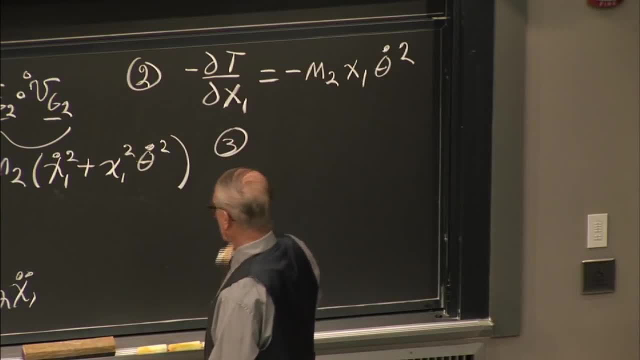 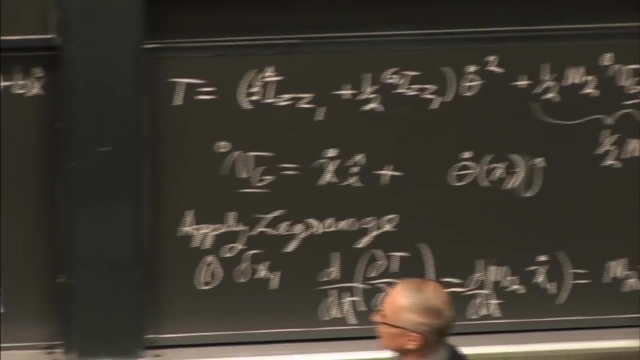 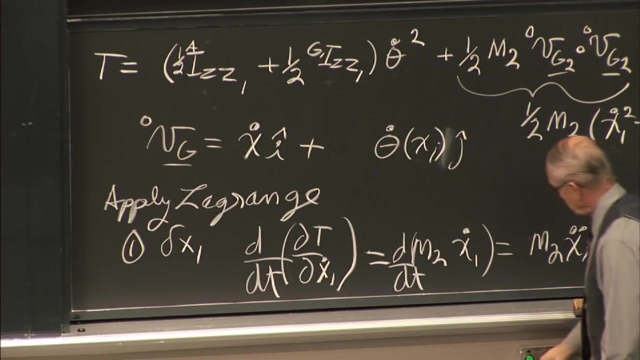 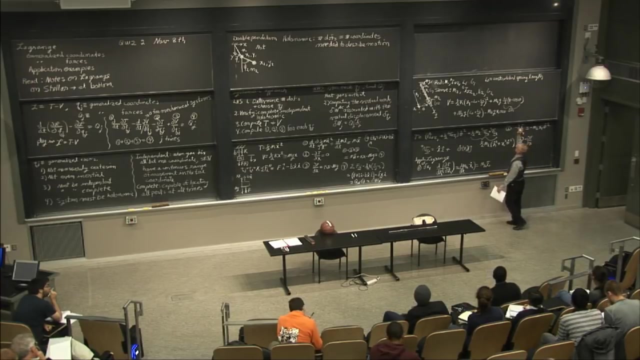 And step three is plus partial of v with respect to x, This case with respect to x. And where's our potential energy expression? Well, it's up here, And where are the x dependencies in it? There is no x in that term and no x in that term. 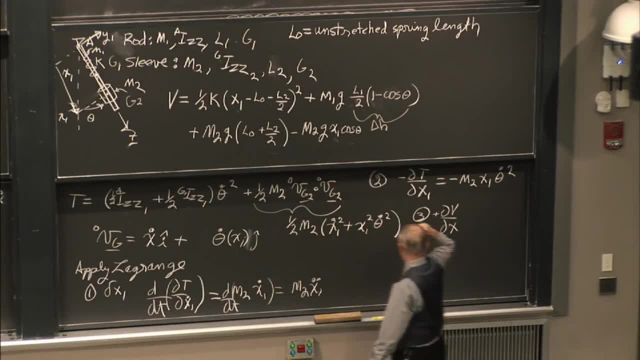 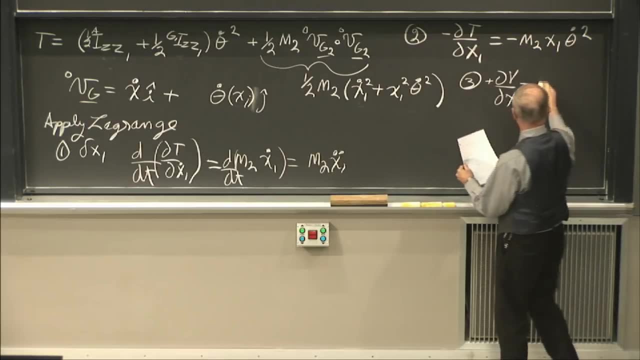 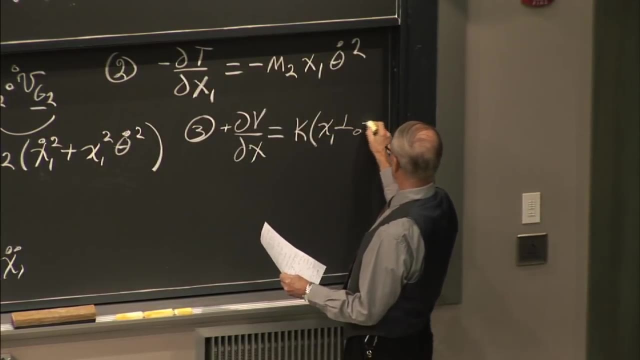 But we have x's in both of these other terms. So when we grind through this, I'll write down what we come up with. We get certainly a spring term Kx1 minus x2.. OK, That's it. Minus L0, minus L2 over 2.. 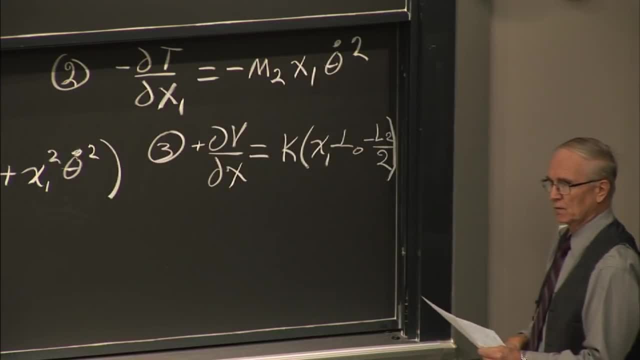 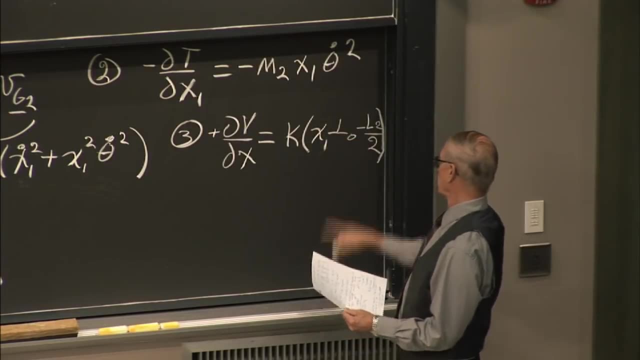 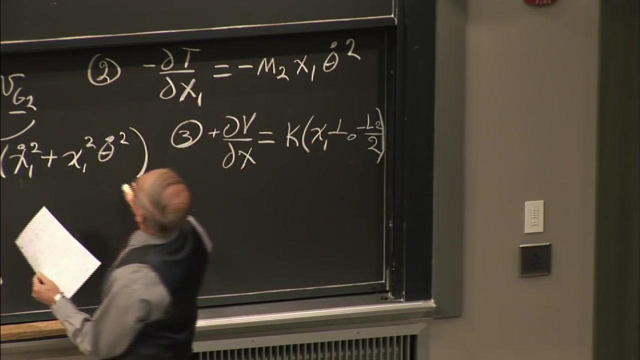 So that's the spring piece. when you take the derivative, The 2 cancels the half And the derivative of the parts inside just gives you 1.. So that's the first piece of the potential energy expression, And the second piece is only going to come from here. 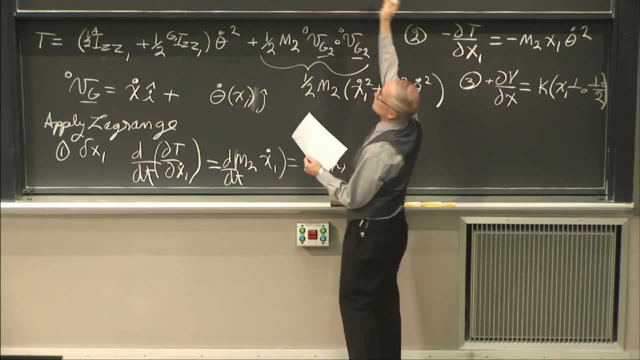 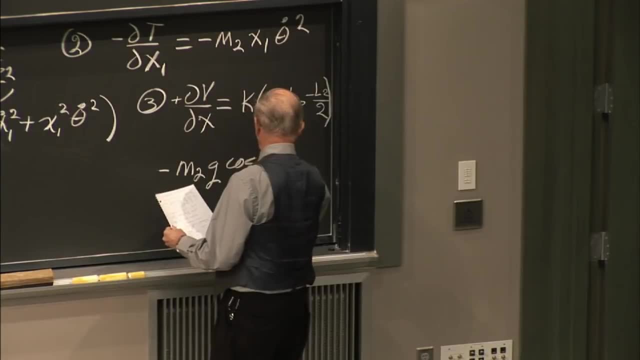 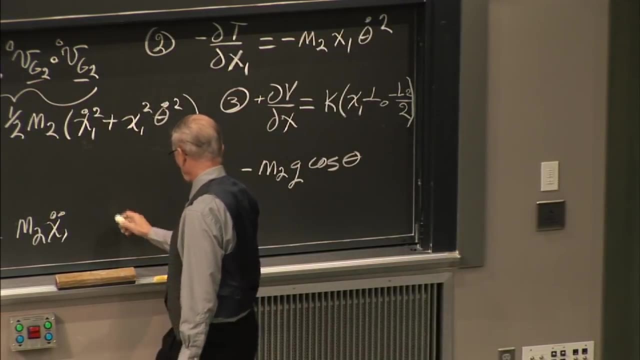 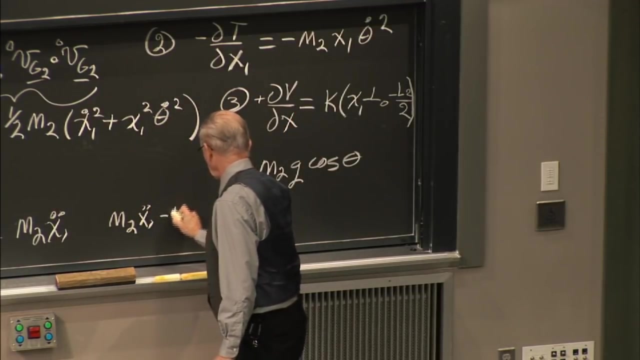 The derivative of this with respect to x1 is just m2g cosen. OK, OK, Cosen theta minus, And you add those bits together, you end up with m2 x1, double dot minus m2, x1, theta dot squared plus k. 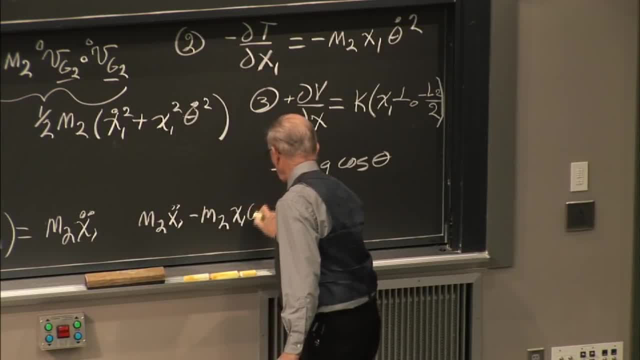 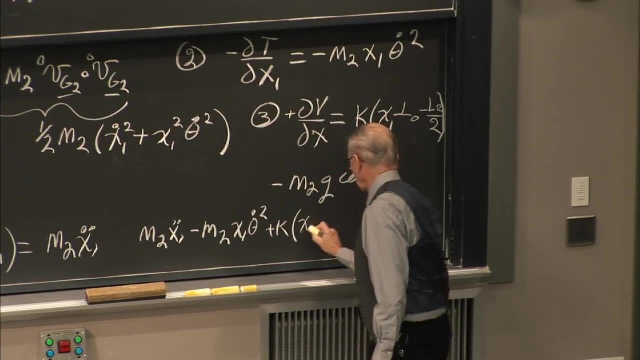 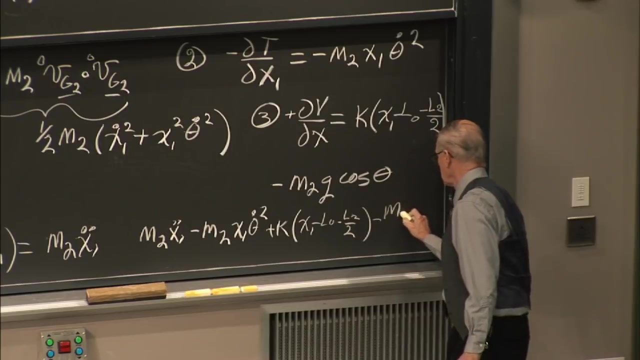 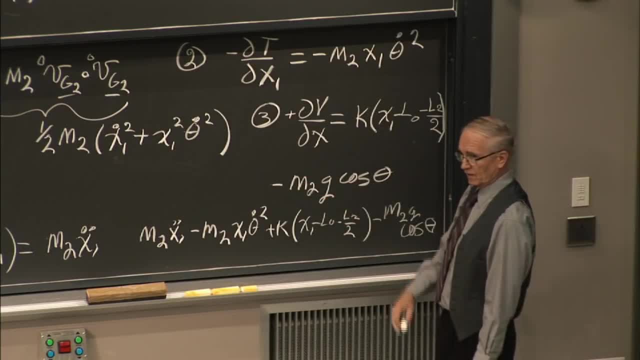 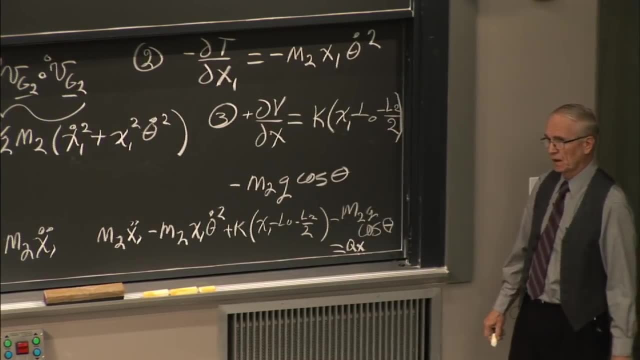 So those are the three terms, one plus two plus three, that go on the left-hand side And they're going to equal my q x. that I find. But I still now have to find what the generalized force is in the x direction. 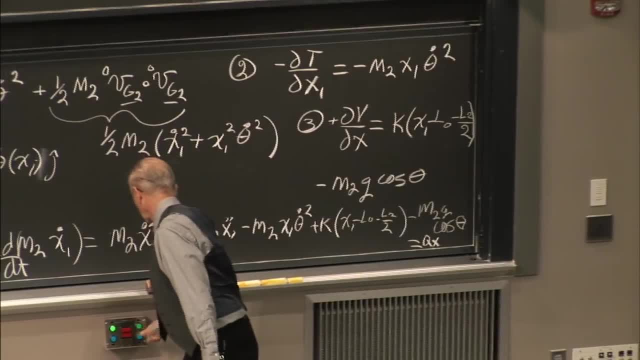 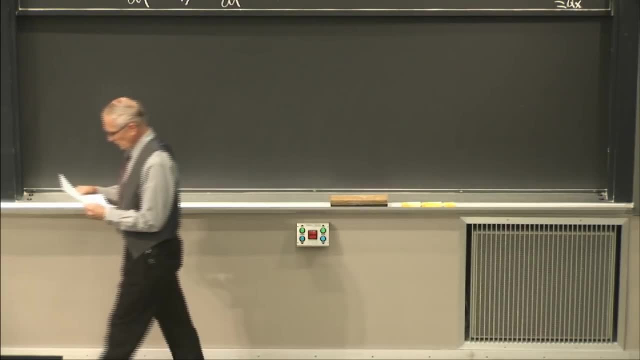 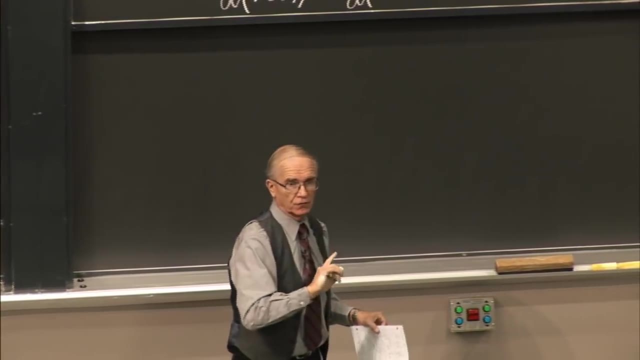 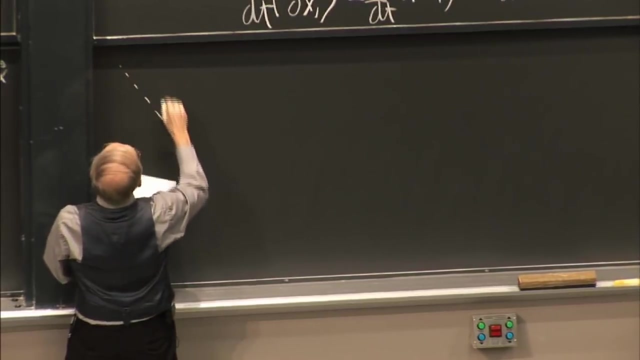 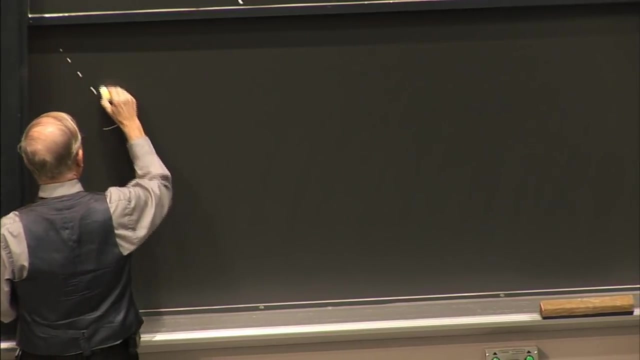 OK, OK. So all that's left to do for this problem is to find q sub x, the generalized force that goes on the right-hand side. So now let's draw a little diagram here of my system And at the end of the sleeve. so here's my sleeve. 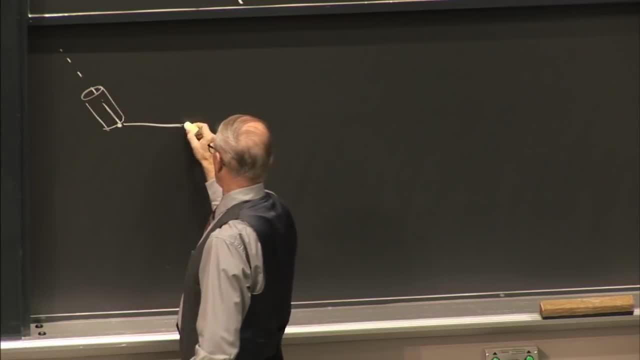 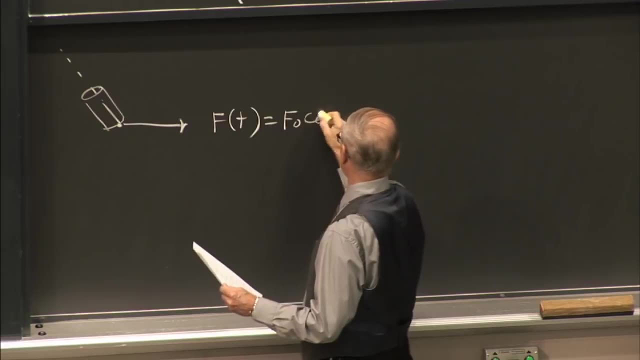 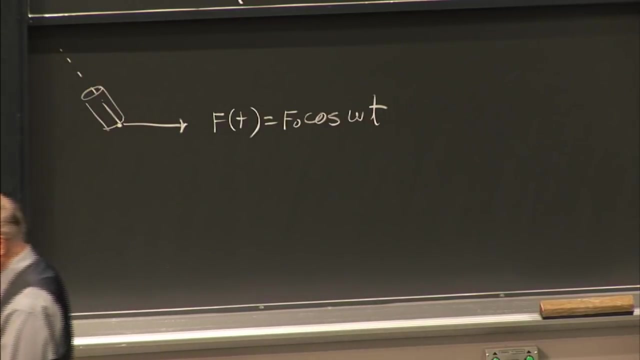 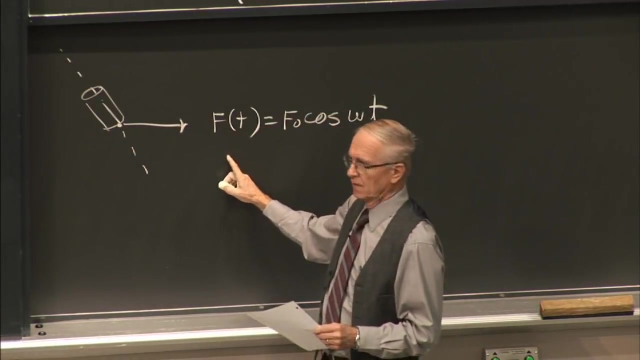 I've applied this force. This is f of t. Maybe it's some f0 cosine, omega t. It's an oscillatory force. external force Make it vibrate And I need to know the virtual world. I need to get the work done making that force go. 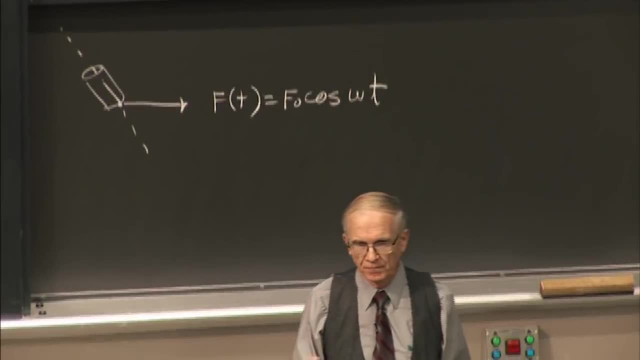 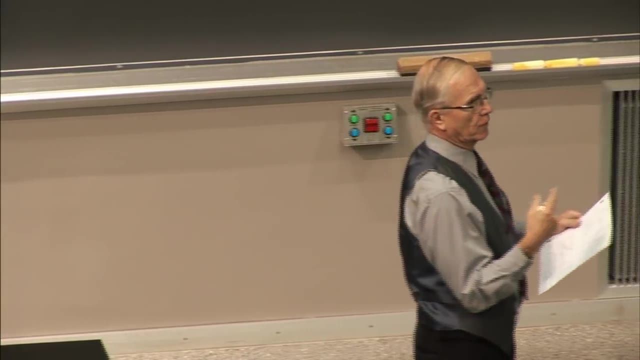 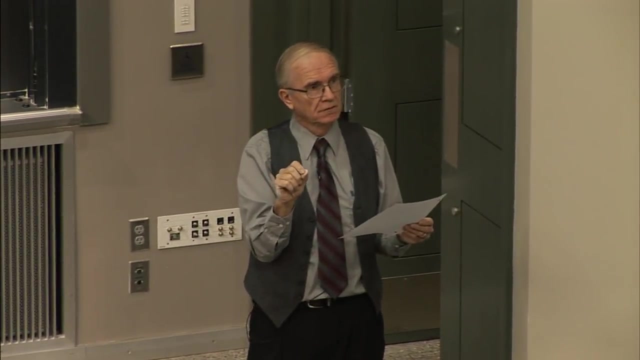 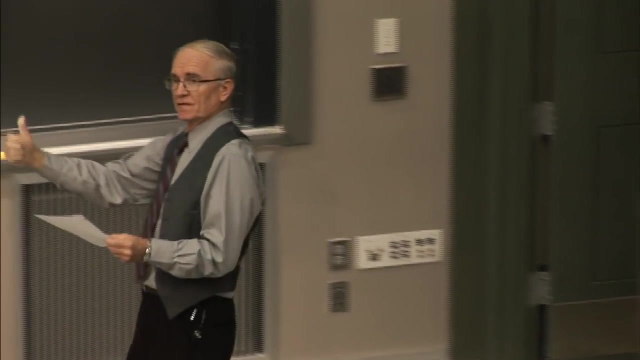 through a displacement. in what direction? So this equation is the x1 equation, right, And so the virtual displacement I'm talking about is delta x1. And the amount of work that it does is delta x1 times the component of this force, that's. 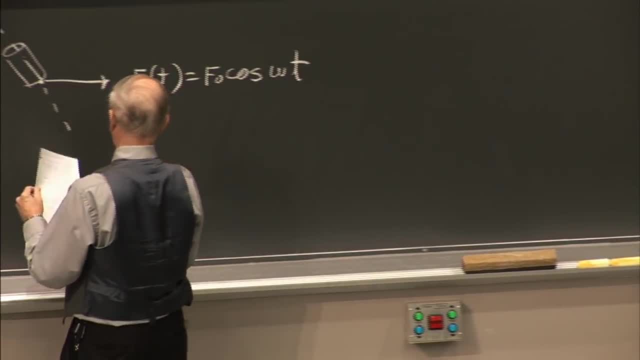 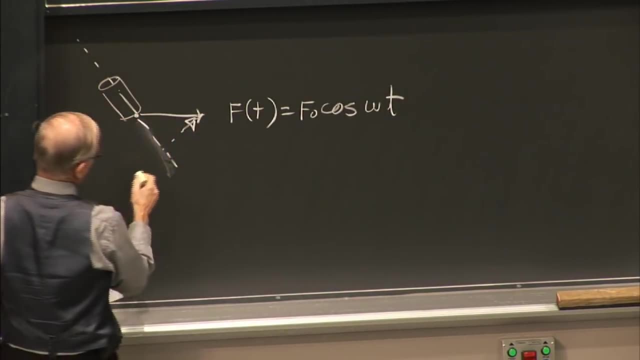 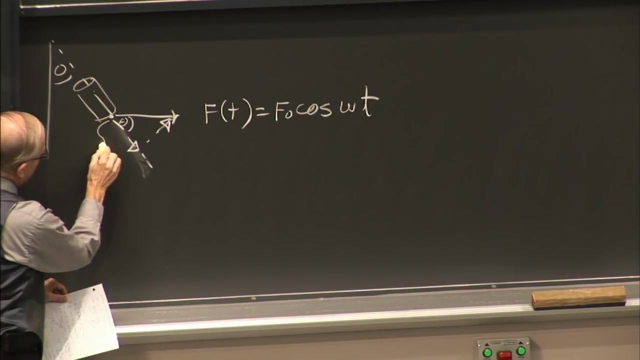 in its direction. So I'm going to take this force and break it up into two components. This is my theta. This is also theta. So this will be f0.. This is f0.. This is f0.. This is f0.. 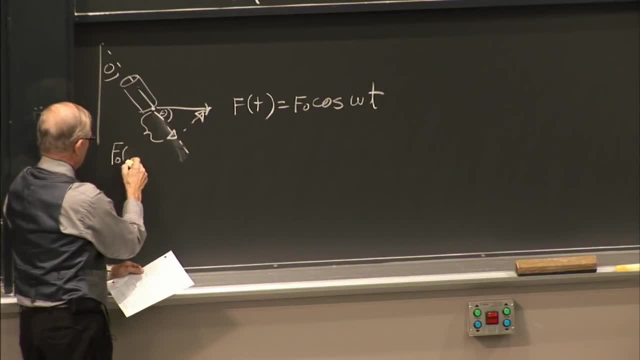 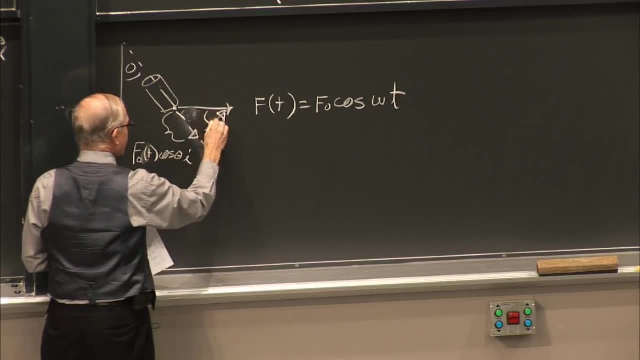 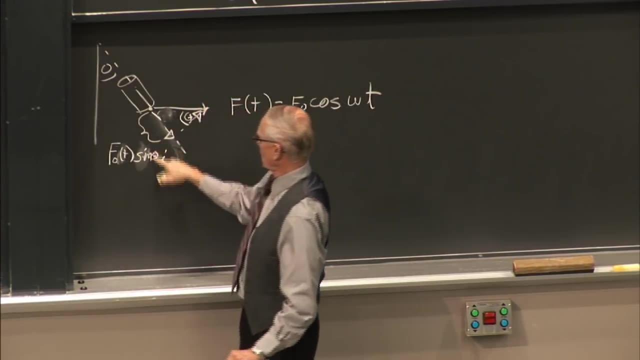 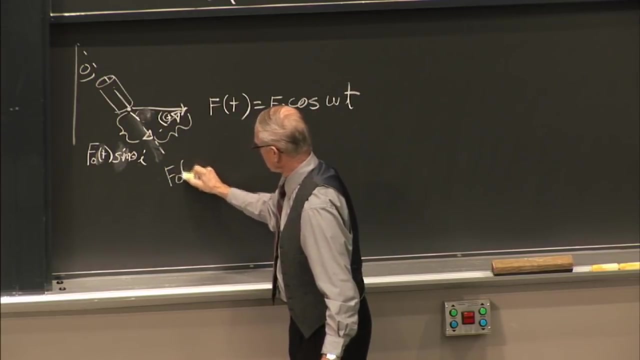 No, Hey, I got this wrong. I drew this wrong. I'm sorry. This is theta. This is going to be sine. This side is sine theta in the i direction And this piece, This is f0 of t, cosine theta in the j. 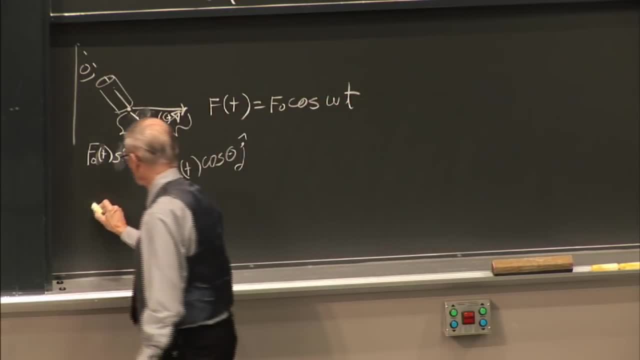 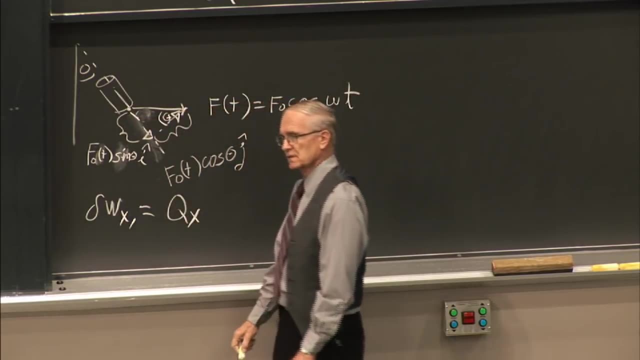 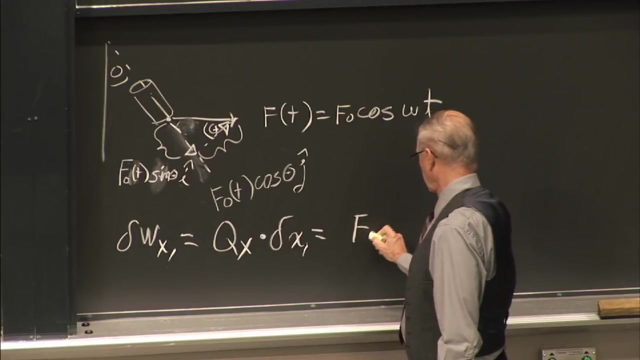 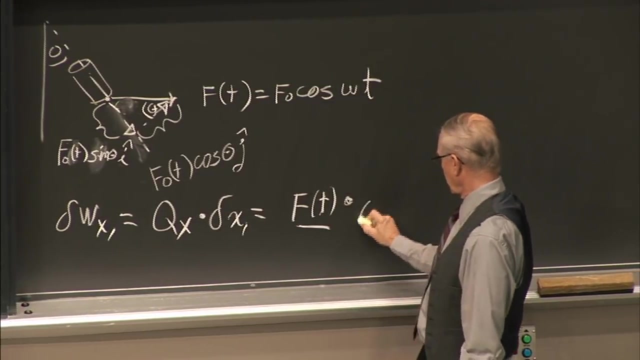 So I break it up in two parts. And the virtual work associated with x1 is the thing I'm looking for: qx dotted with delta, x1.. And that is f of t, here A vector dotted with dr, my little displacement. 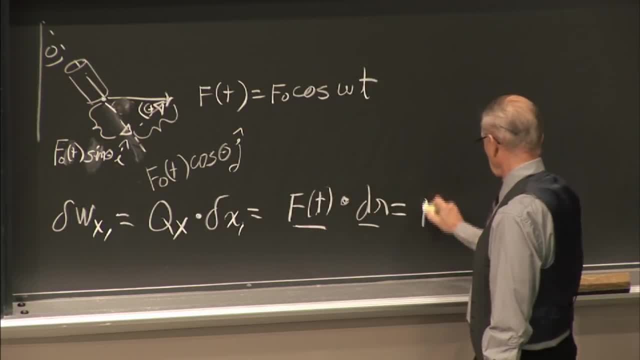 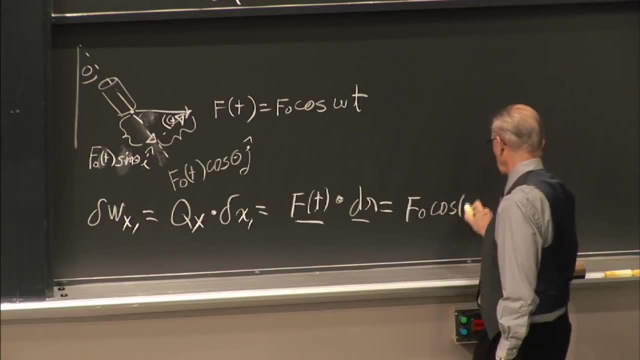 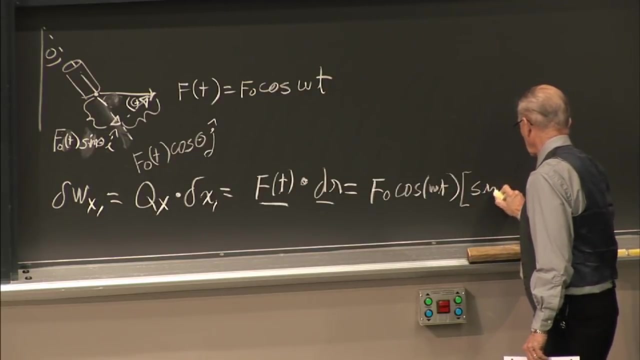 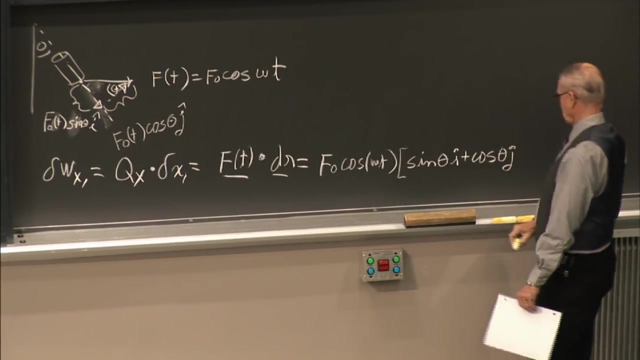 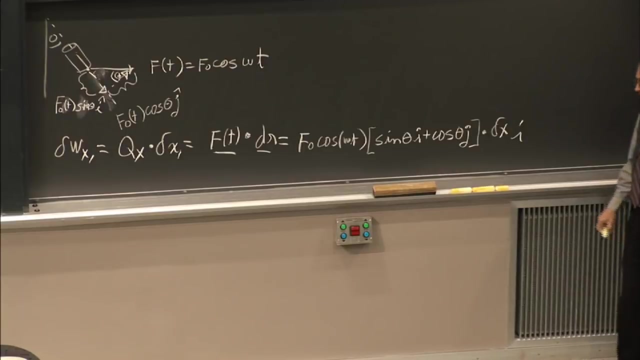 But in this case this then all works out to be f0 cosine omega t, And it has sine theta i plus cos theta j. OK, OK, Theta j components dotted with delta x in the i. So you're only going to get i. dot j gives you 0.. 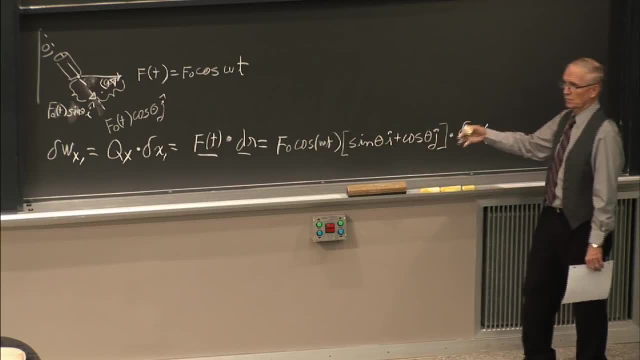 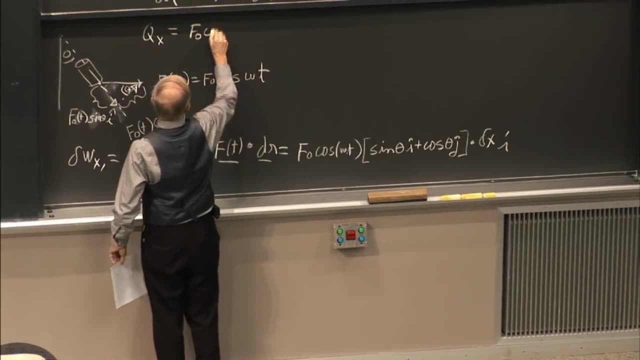 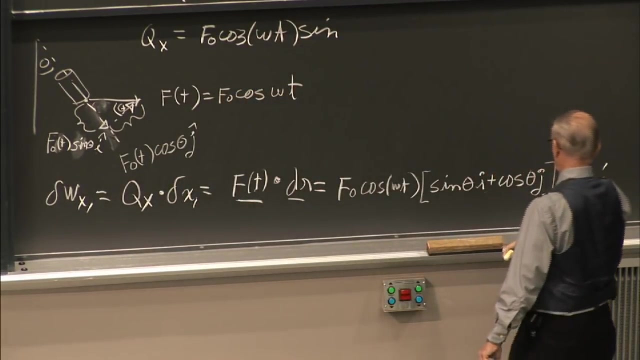 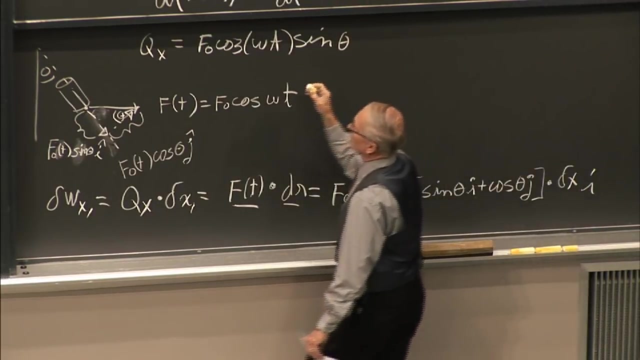 i dot, i gives you 1.. So you're going to get one piece out of this. It says then that qx equals f0, cosine, omega t, sine, Theta, Theta, Theta. And to start with, you have a delta x here and a delta x here. 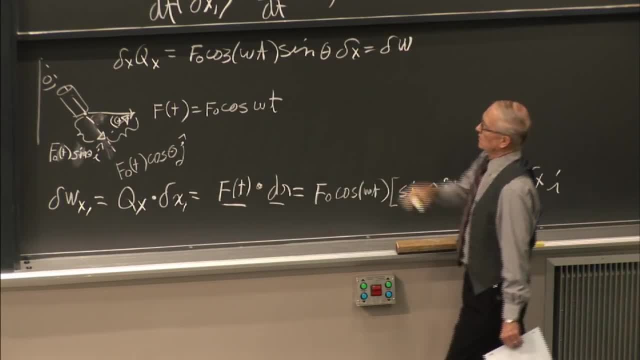 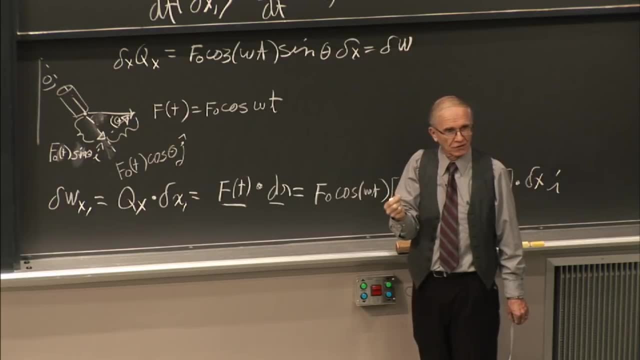 And that gives you the delta virtual work. Then to solve, to find you need. I need. personally, when I do these problems, I think in terms of that little virtual deflection And I actually figure out what's the virtual work done. 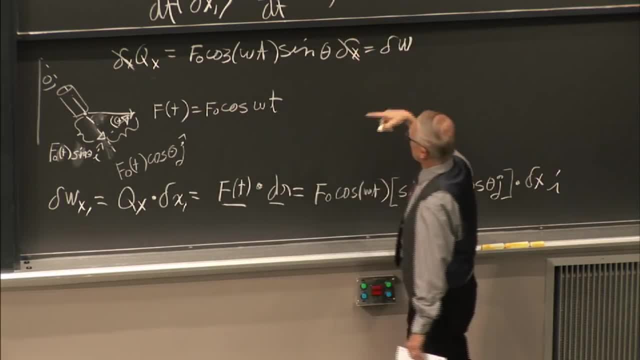 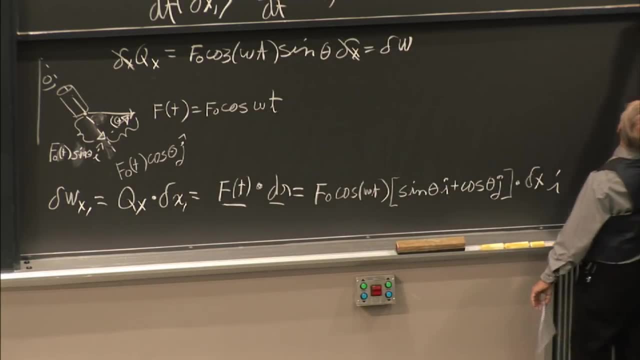 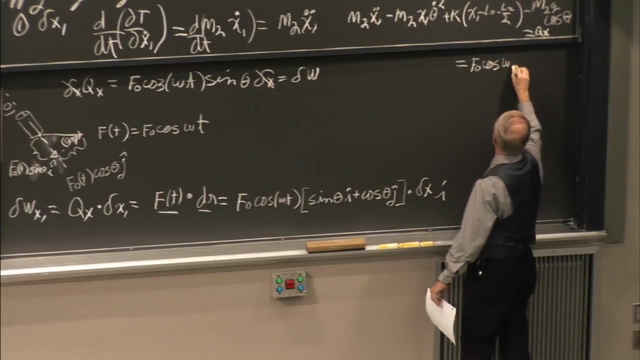 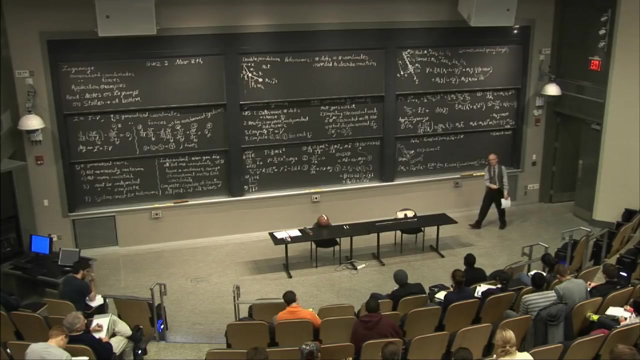 And then at the end I take this out, And this is that. This is the qx that I'm looking for. So my final equation of motion says this: equals f0, cosine, omega t sine theta, And that's your equation of motion in the x1 direction. 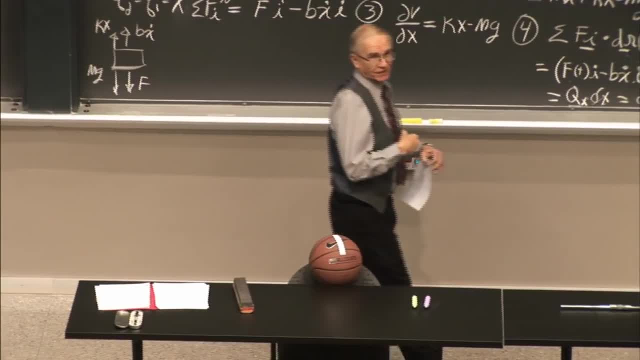 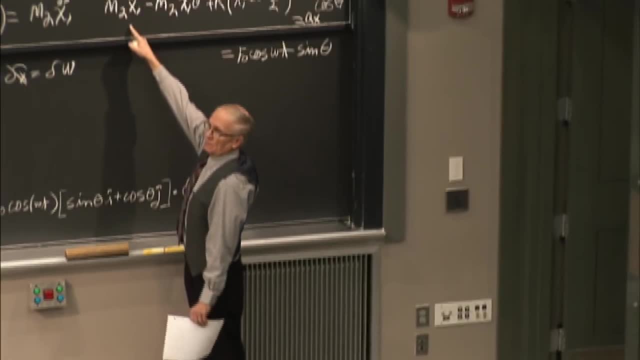 So when you finish one of these, you need to ask yourself: does this make sense? Does this jive with my understanding of Newtonian physics? Better have a linear acceleration term, because that's what it's doing. You have another acceleration term in the same direction. 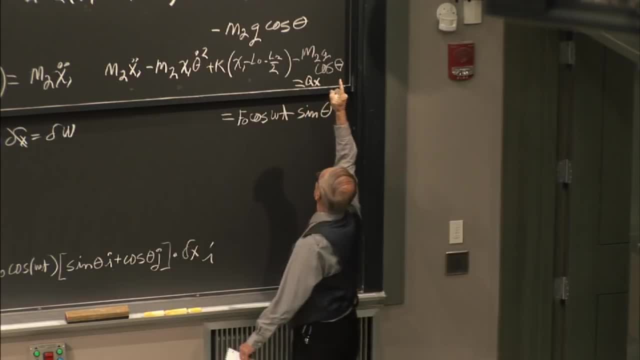 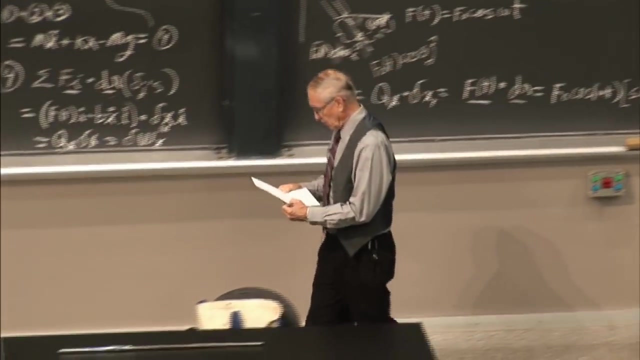 due to centripetal, a spring force, for sure, and a component of gravity in the direction of motion up and down the slide equal to any external forces in that direction. So it makes pretty good sense. OK, Now also another test you can do. 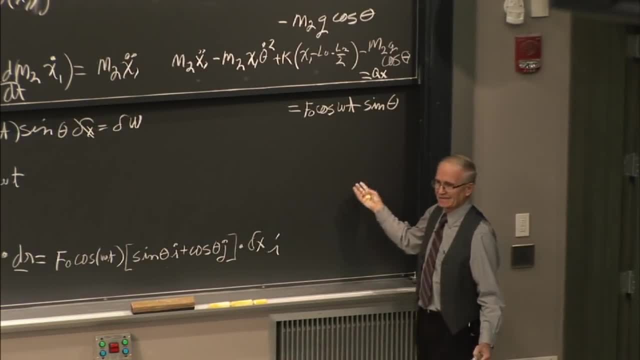 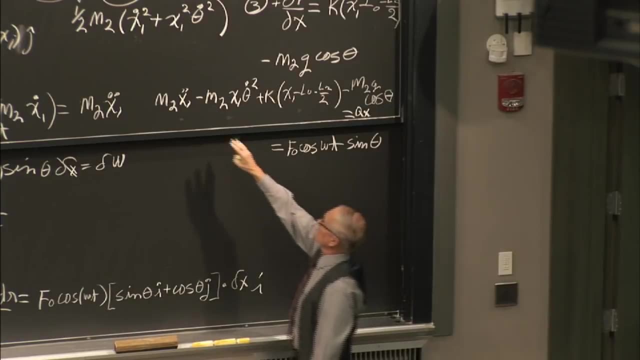 is: does it satisfy the laws of statics? That's another check you can perform. Does this thing at static equilibrium tell the truth? At static equilibrium, all time, derivatives are 0.. So this would be 0.. This would be 0.. 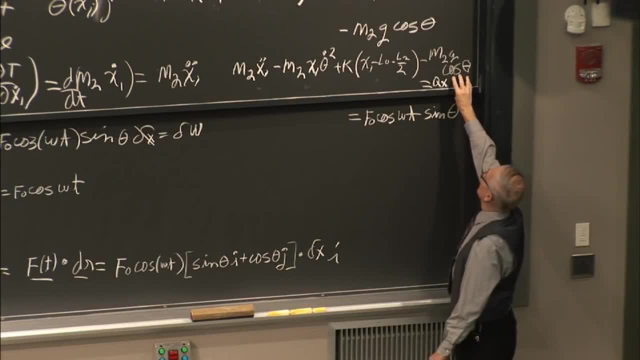 You know, at static equilibrium it hangs down. So cosine theta is 1.. Static: you don't have any time-dependent forces. That's 0.. So the static part of this says that. you know it's 0.. It's 0.. 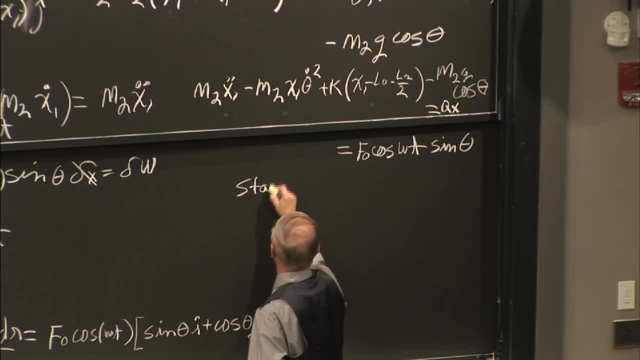 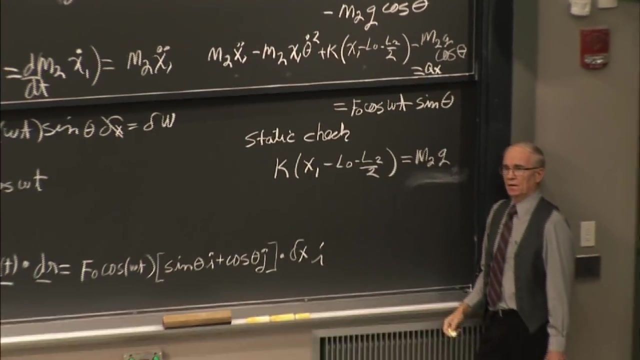 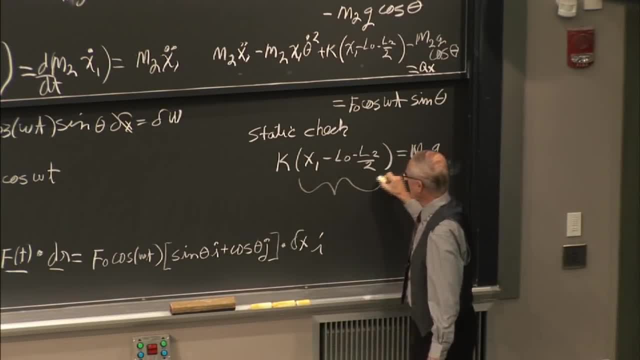 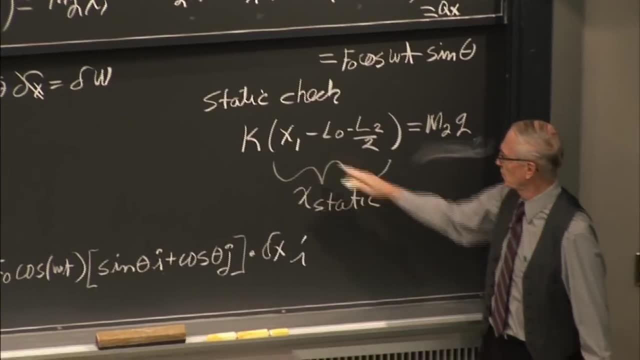 And you could figure out, then this must be k times something. This is the x, This is the amount that the spring stretches. the static stretch of the spring, so that it's equal to the spring, has an equal opposite force to the weight of the thing: m2g. 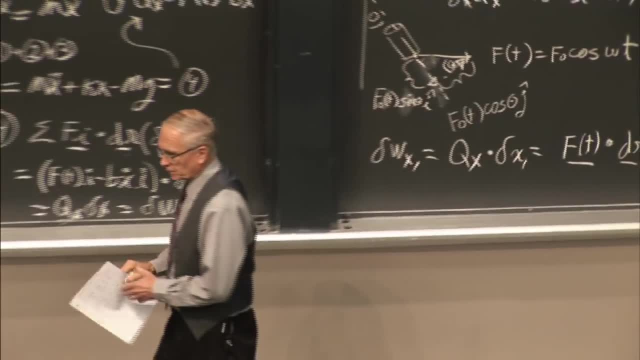 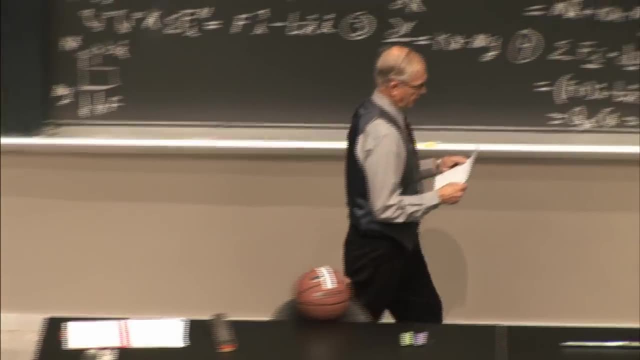 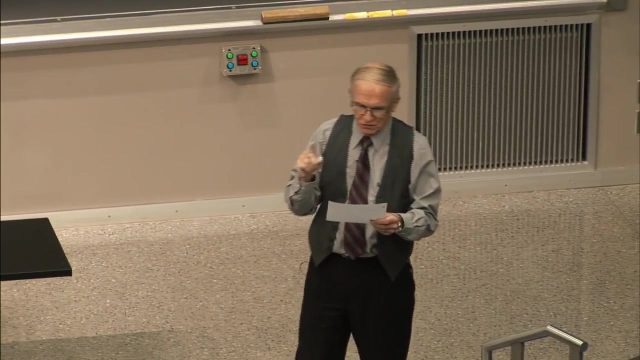 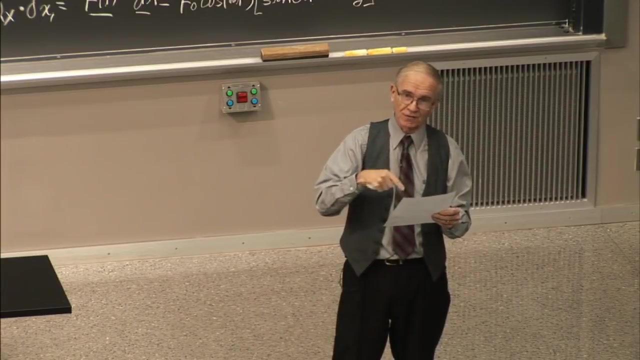 So that's another check you can do when doing the problems. OK, so I want you I'll write up the other one. We have one more equation to go right. Got to do all the derivatives with respect to theta, So you take a minute to decide how many acceleration terms. 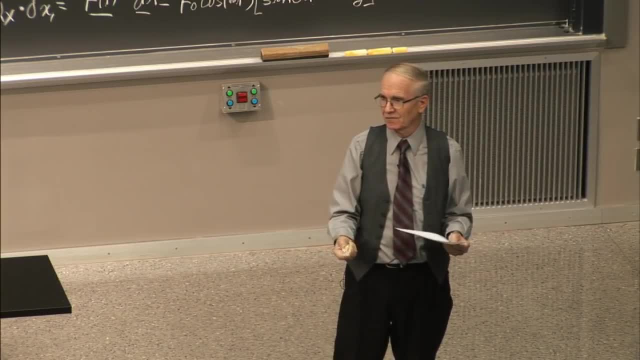 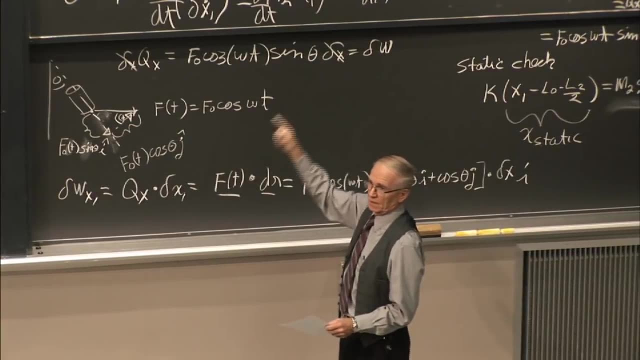 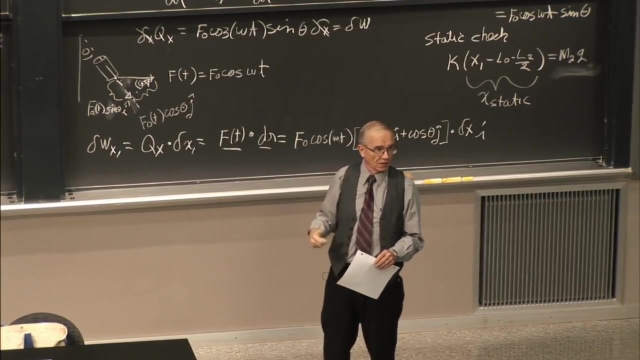 and what acceleration terms do you expect to see come out of this second equation of motion? Because now we're talking about which motion- Swinging motion- And what's its direction? In Newtonian sense it would have a vector direction. It's in what we call j here. 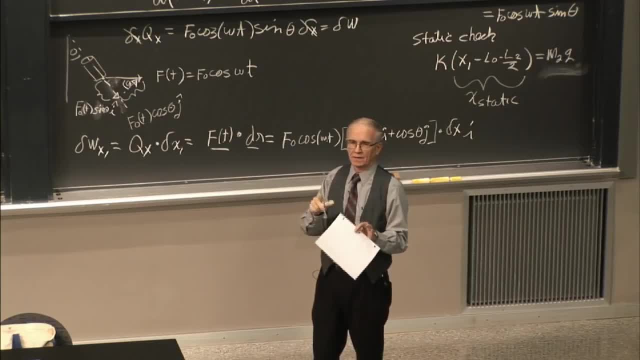 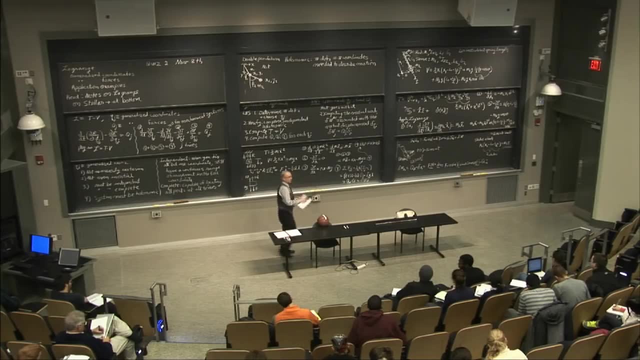 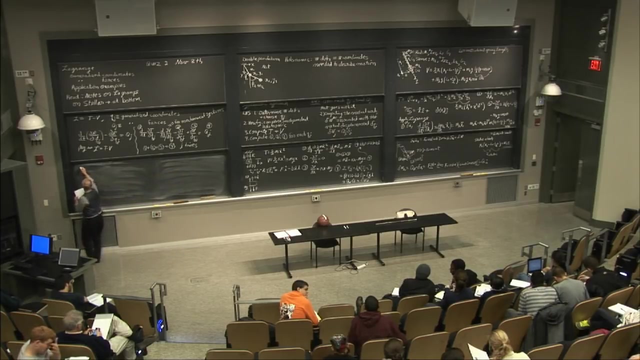 OK, so you're about to get the j equation: What, What, What terms do you expect to find in it? Talk to your neighbors and sort this out. Basically, tell me what the answer is going to be. What is the expression for u? what is the expression for v? 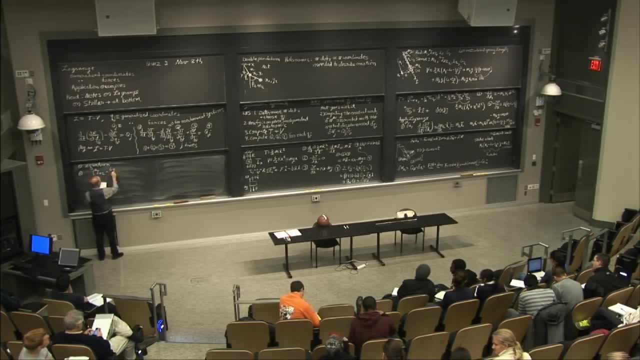 So you want it to be. What's the expression for u? What's the expression for v? What's the expression for v? So that's what we're going to use for the next section of this. What do you think? What? 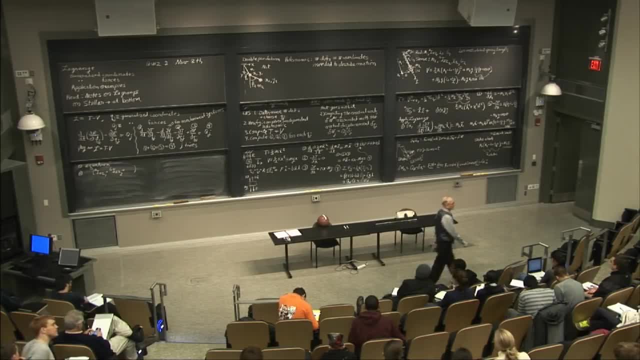 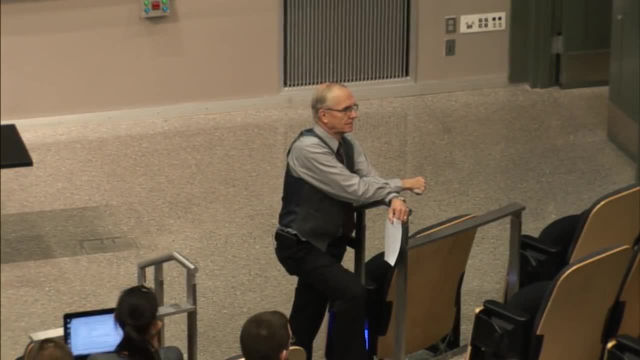 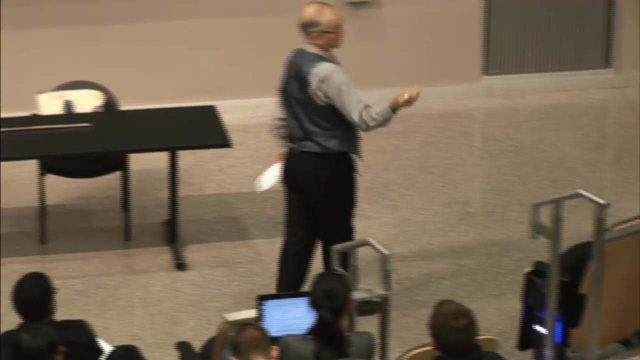 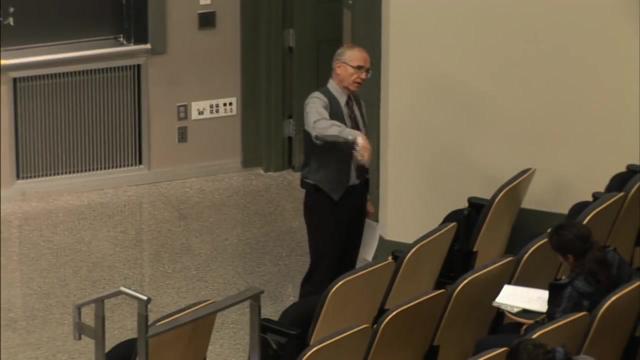 What are we going to get? We were debating about whether or not it was going to be like speeding up in the theta path. So it is a pendulum, just a weird pendulum. So is there? does the theta change speed? Sure, 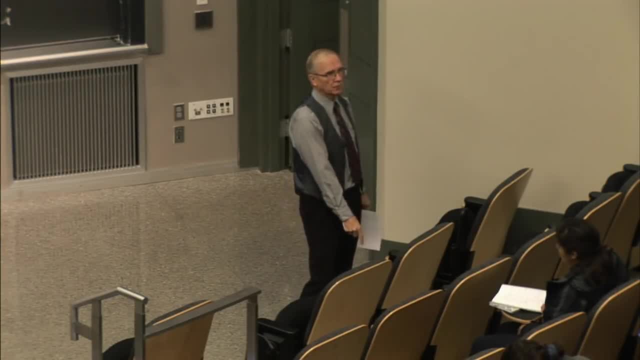 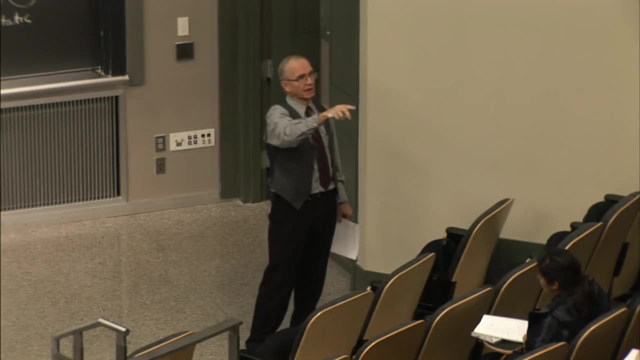 When it gets up at the top of its swing, it's 0.. All the way down, it's maximum speed. So what terms does that imply that you're going to get That, Coriolis? Well, maybe, maybe not. 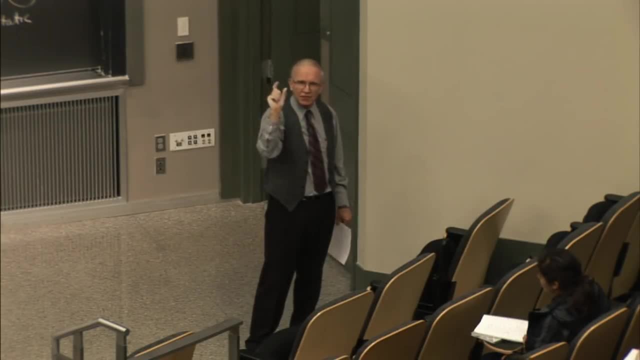 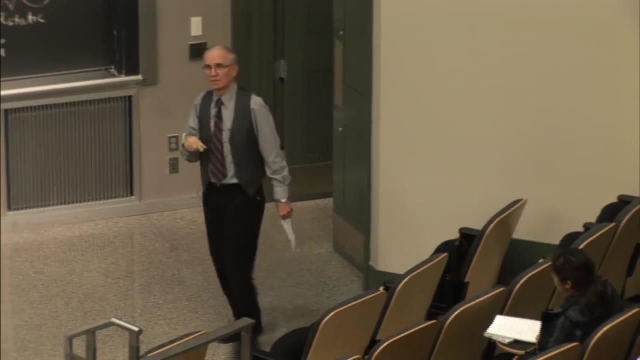 Yeah, Eulerian, You're going to get an Eulerian, which means you've got a theta double dot term. You're expecting a theta double dot term to show up. OK, What else Will you get? a Coriolis term. 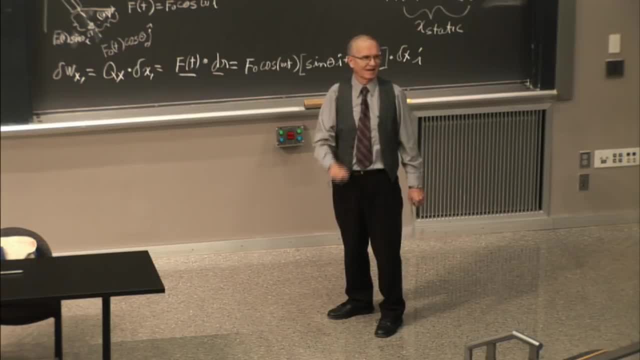 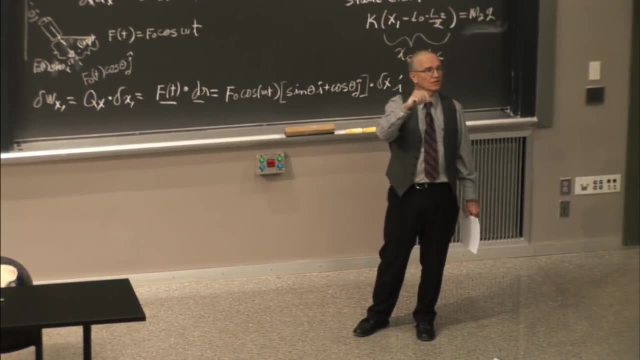 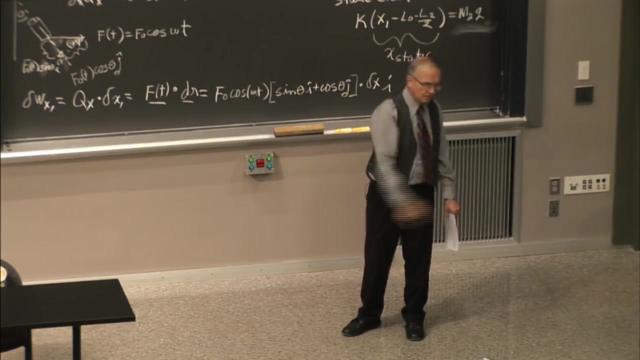 Do you expect a Coriolis term, Something that looks like x dot, theta dot. Yeah, The thing is sliding up and down the sleeve. It has a non-zero value of x dot Any time you've got things moving radially while something is swinging in a circle. 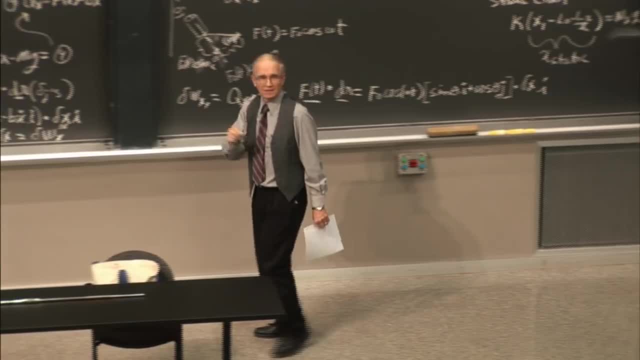 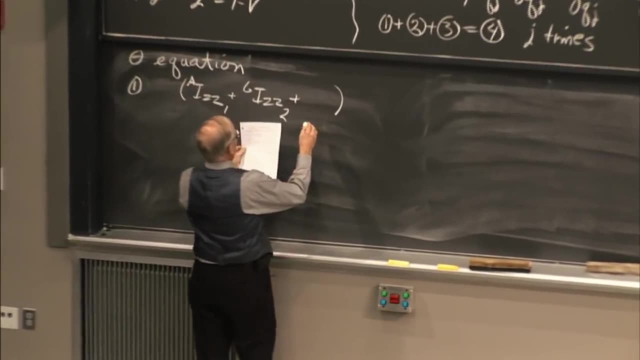 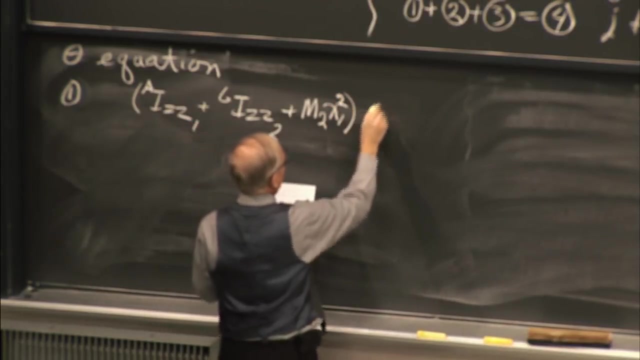 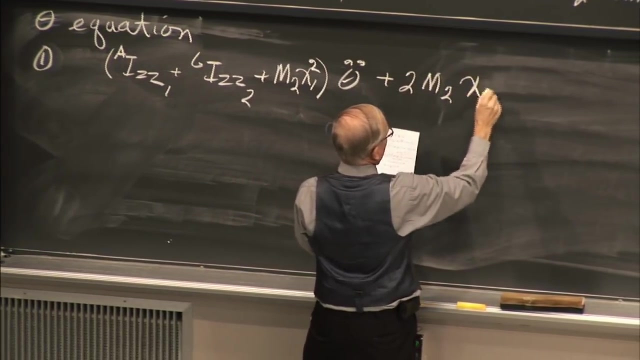 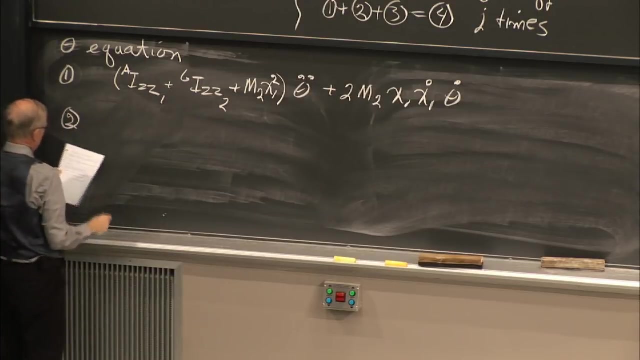 you will get Coriolis forces. It means the angular momentum of that thing is changing and it takes forces to make that happen. So here's what this answer looks like. The answer looks like That's the one term. The two piece gives you 0.. 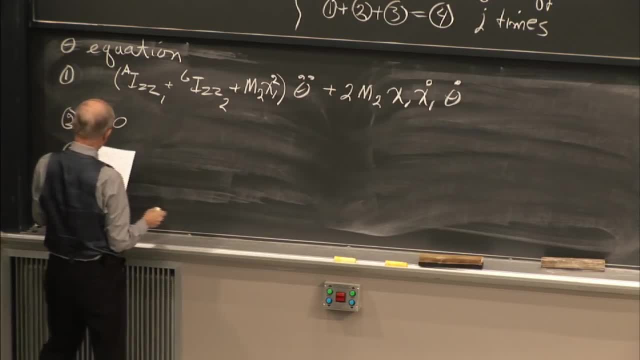 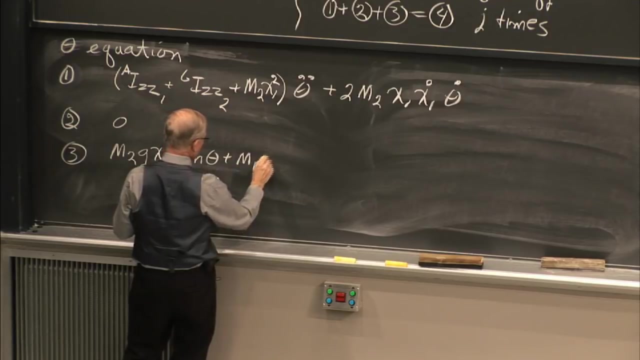 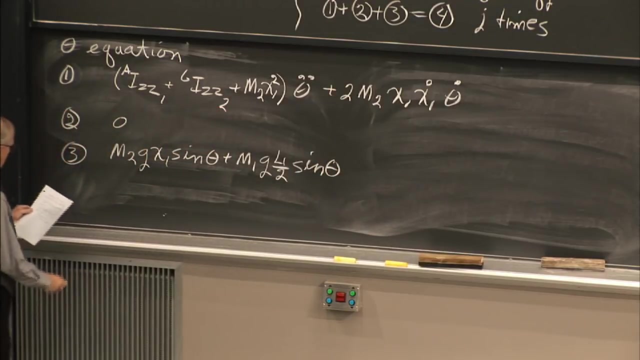 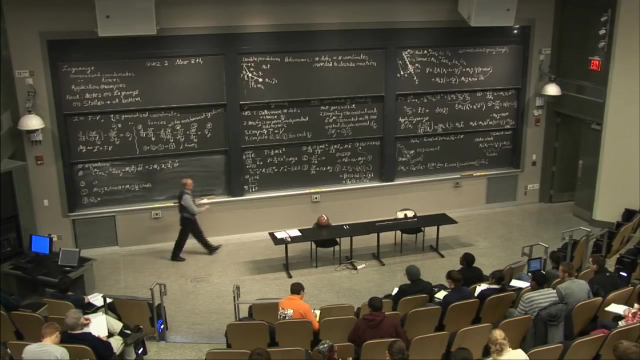 It's not a function of x. in the three piece, The potential energy piece gives you m2 g x1 sine theta, plus m1 g l1 over 2 sine theta, And the fourth piece, the q theta. well, that's just going to be the virtual work done. 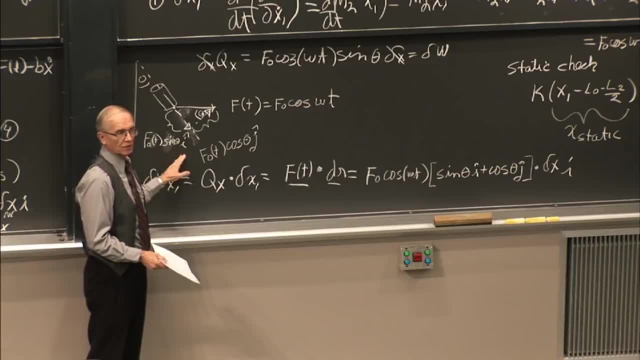 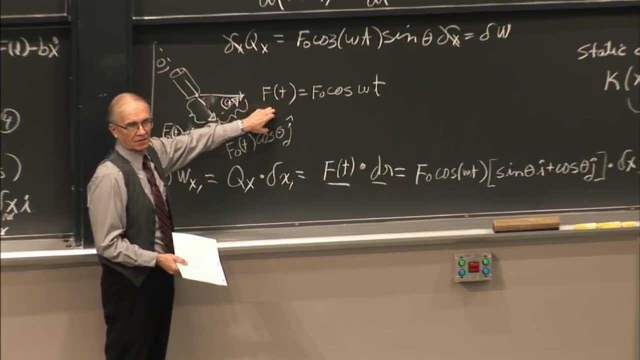 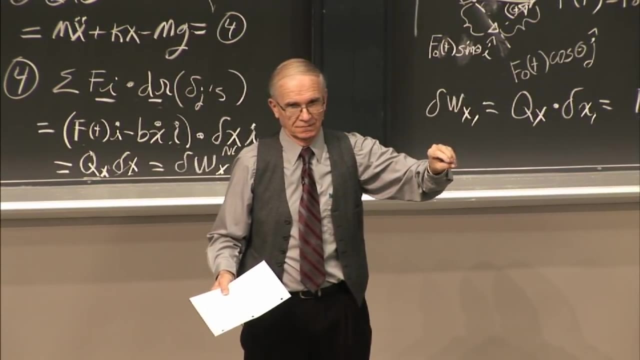 There's a tricky bit to this one. Now, there's virtual work, but which direction? So we have an f dot, a dr. The only f we have is this: What's the dr? What direction is it? This is the theta coordinate. 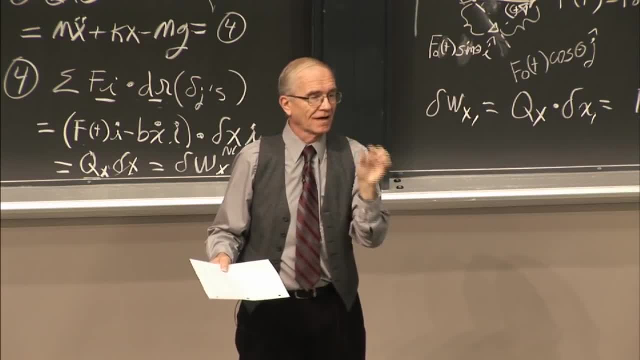 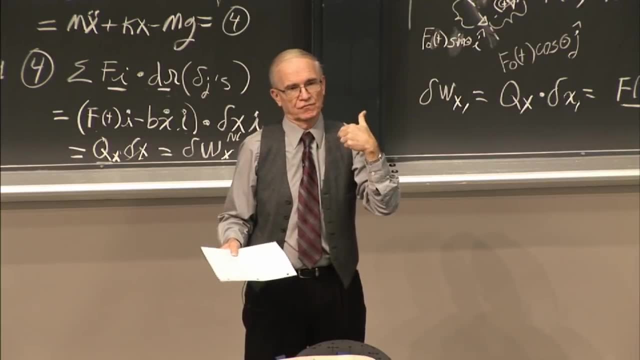 What direction does that give you displacements? f, dot, dr. dr is a displacement, not an angle. To get the work done you've got to move a force through a distance. So the distance first of all is in what direction when theta moves? 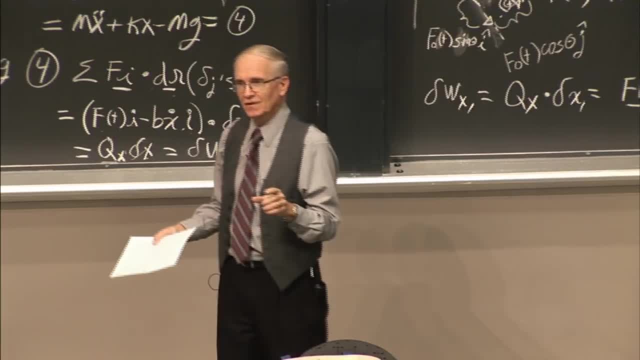 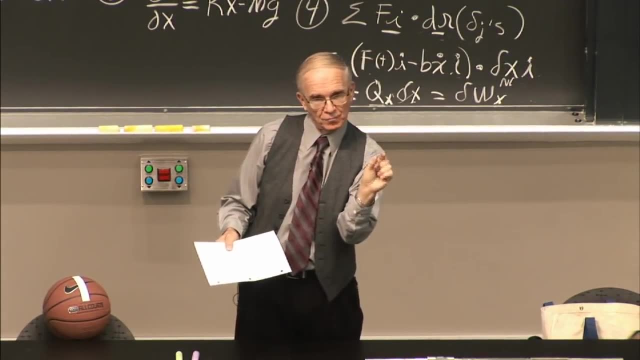 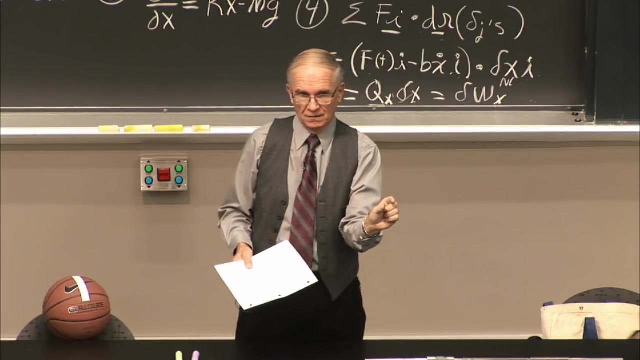 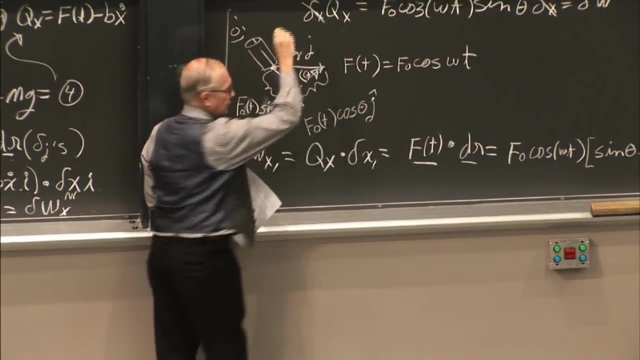 j a little. j hat right. And how much? if now, if you get a virtual deflection of delta theta, what's the virtual displacement? You get a virtual change in angle, delta theta, but is that the virtual displacement? What's the displacement of this point here in the j direction? 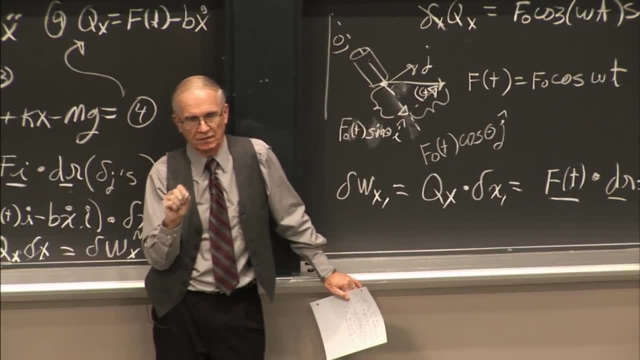 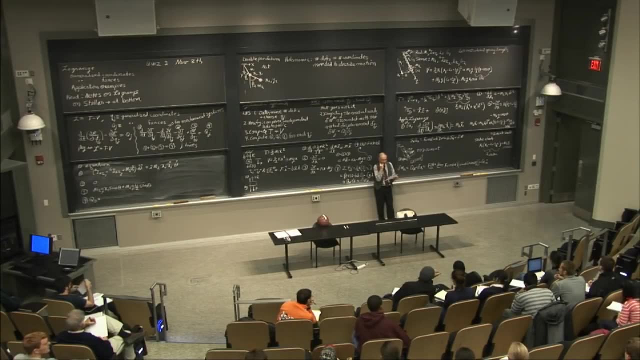 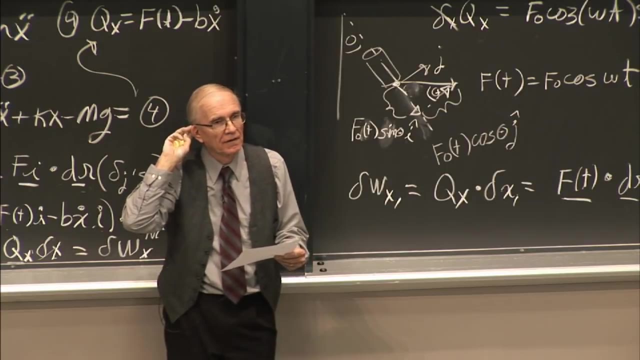 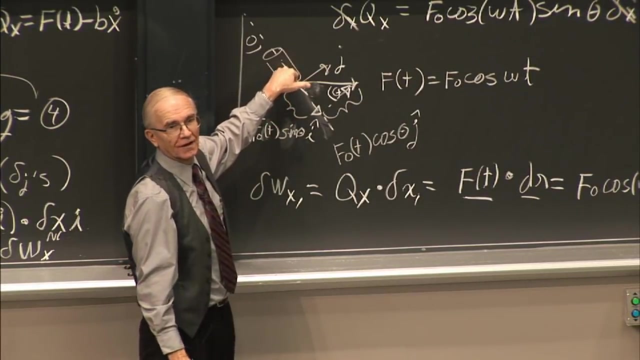 given a virtual displacement: delta theta. Think that out Can't quite hear you. x1, delta theta. x1 delta theta will give you the motion, the displacement, the displacement at the center of mass, in that direction. x1 comes from here to here. 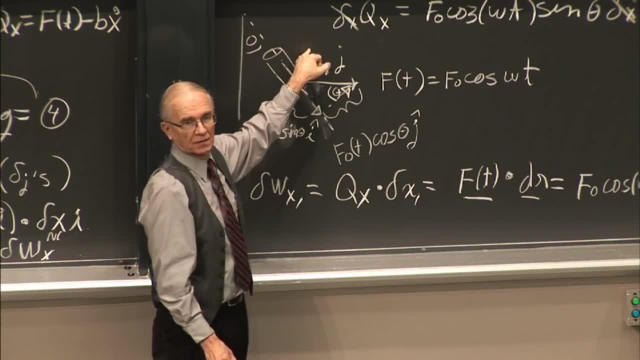 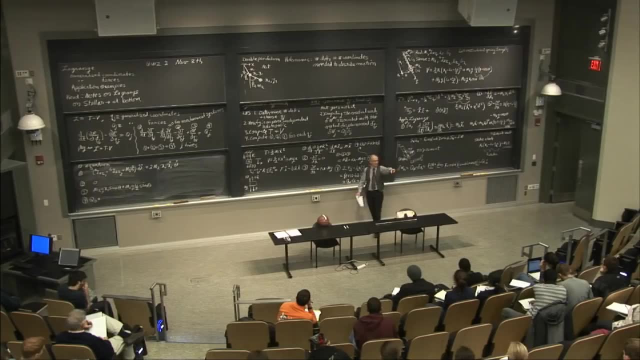 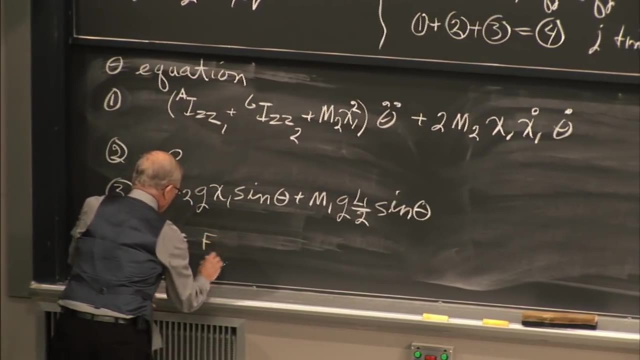 So x1, delta, theta will give you a little displacement in that direction. But is that the displacement we care about? We need the displacement here. So you're close, So we're going to get some force dot a displacement. dr j hat. 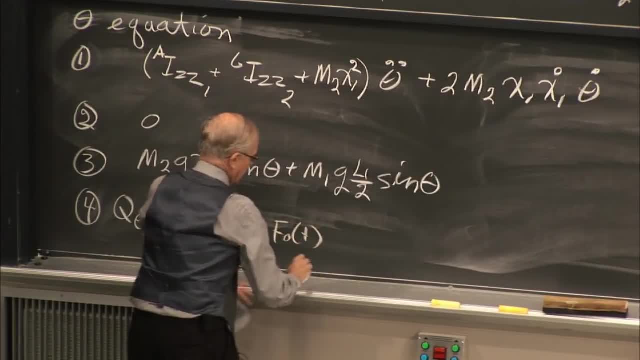 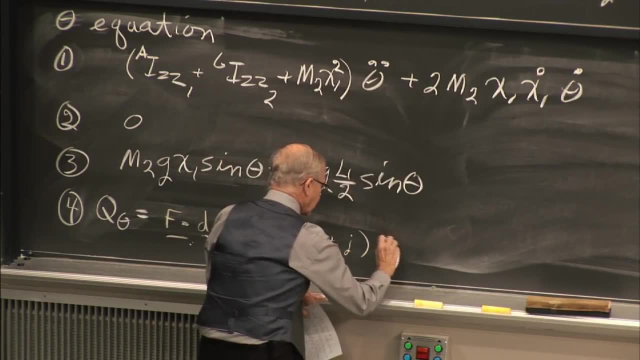 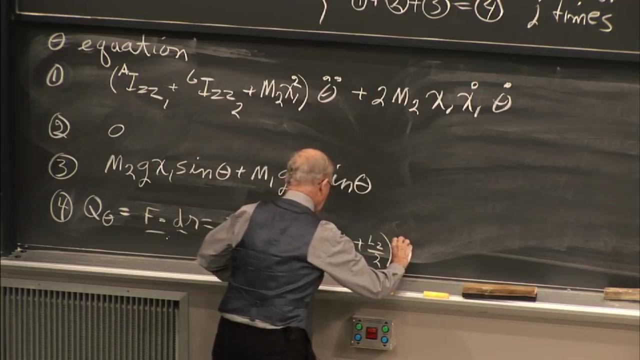 And that's going to be our force. this guy with its i and j components. i and j terms, But this term out here is x1 plus l2 over 2 to get to the n, And it's in the j direction. 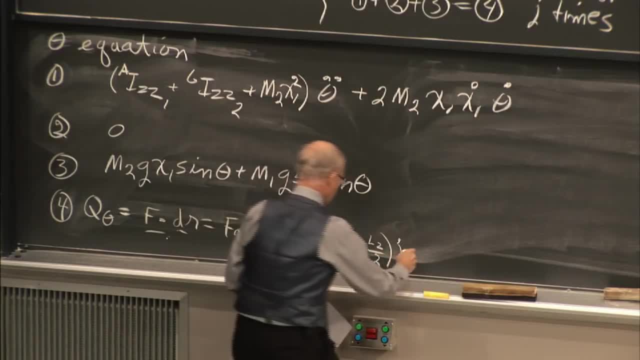 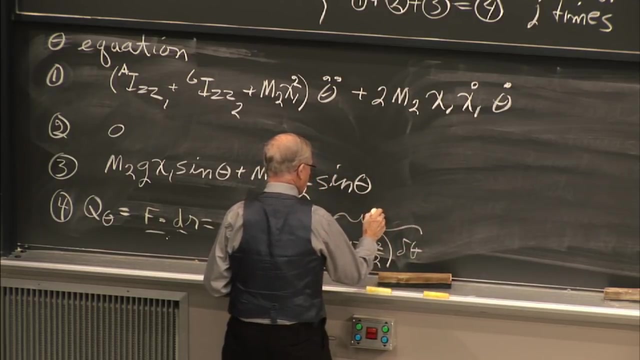 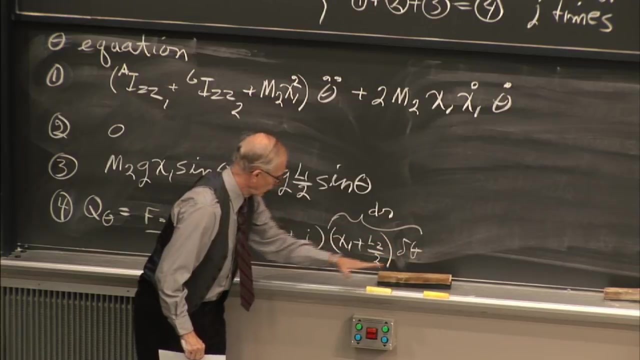 So it's a length times a and you need the delta, this quantity, And you need a delta, Delta, theta, Delta, theta- This is the term, This is the dr for this system. An angle, a virtual deflection in angle times, a moment arm. 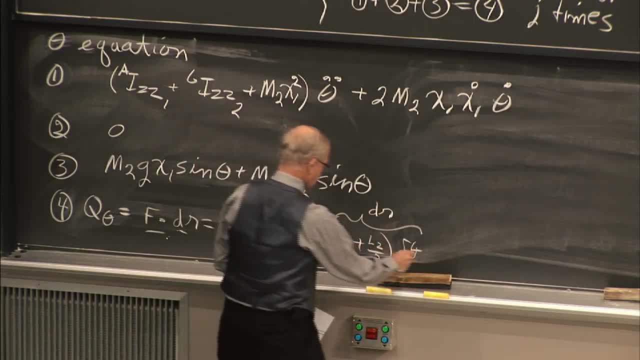 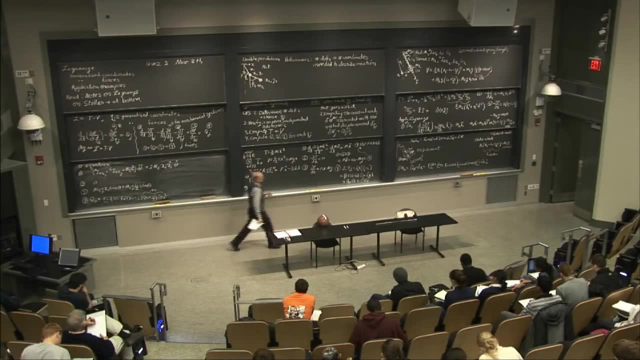 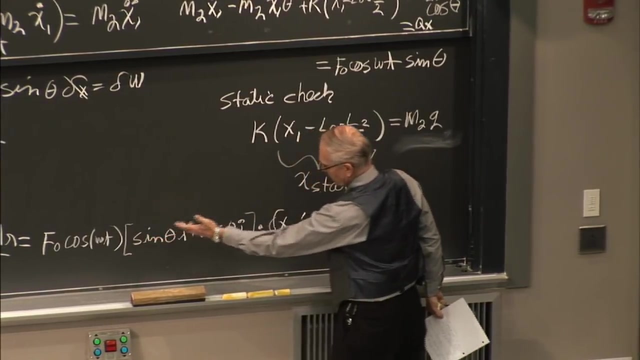 gives you a distance. It's in the j hat direction, dotted with the same force, breaking the force up into its i and j components. It had a sine theta i Cos theta j. So this is going to give me a f cosine, omega t cos theta j dot. 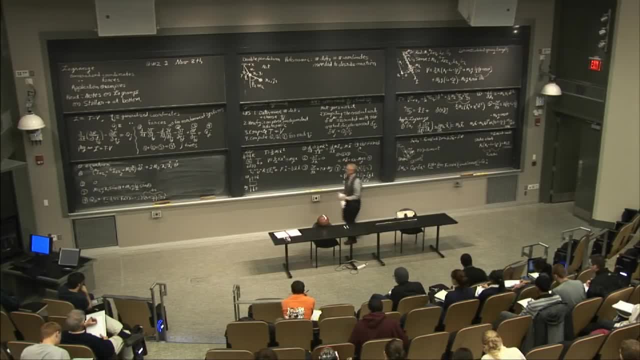 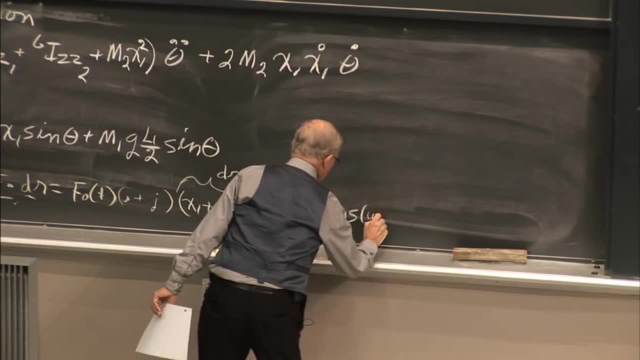 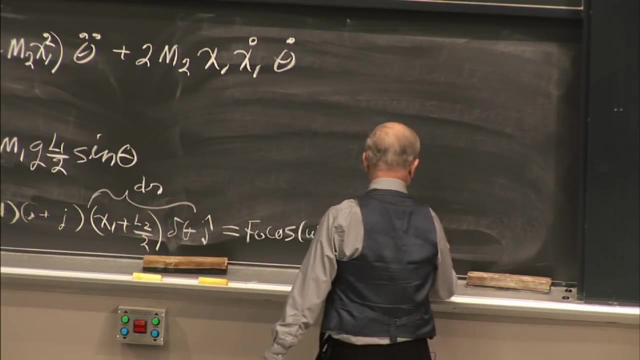 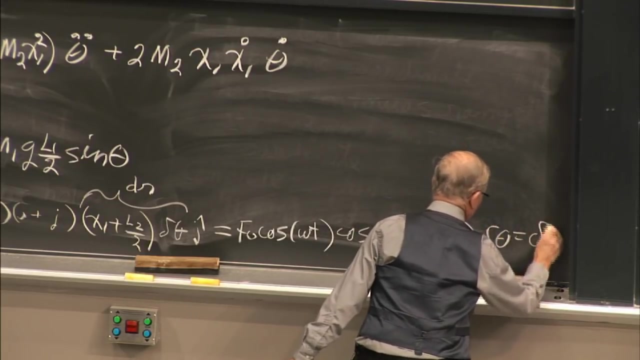 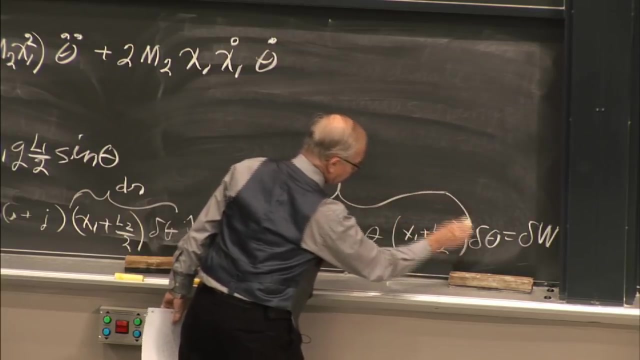 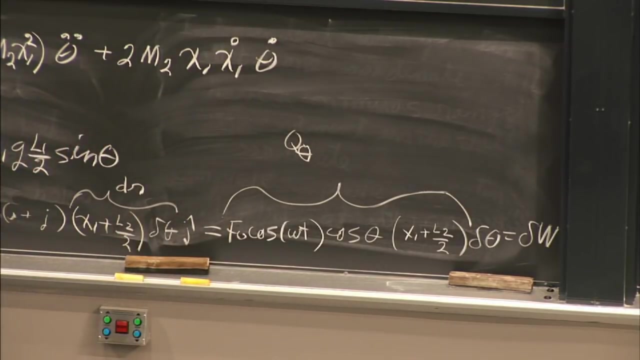 j, f0, cosine, omega t, cos theta x1 plus l2 over 2 delta theta, That is the delta w, That's the work, And the virtual or the generalized force q theta is this part of it. So this plus this plus this equals: 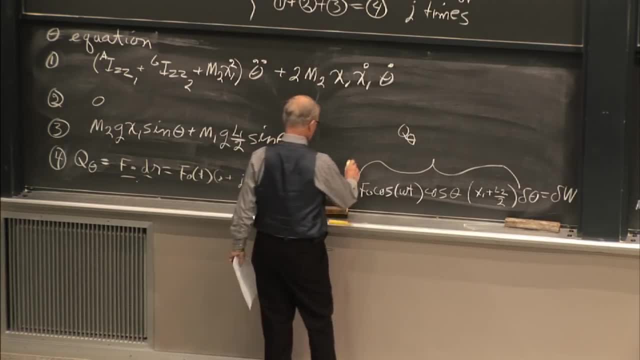 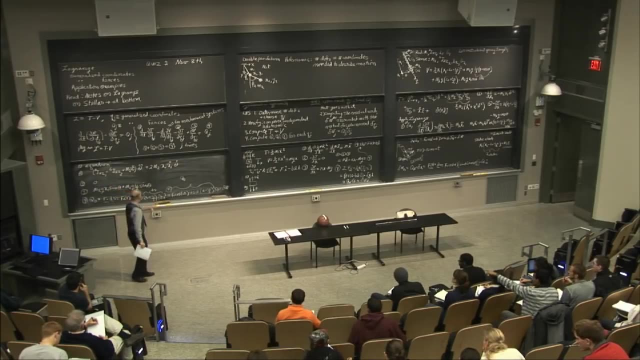 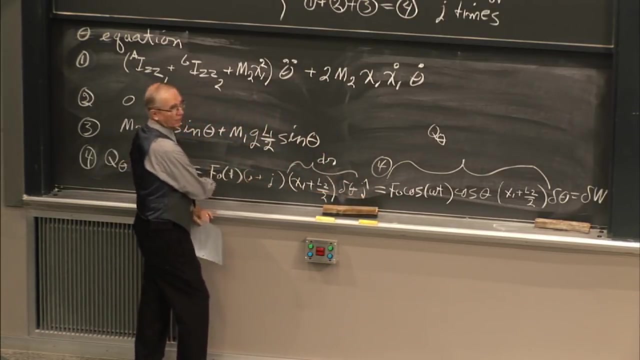 that on the right-hand side. So this is part four, And so this, let's just look at it. Yeah, So f of t, I didn't want to write it all out- This thing breaks into an i and a j piece. 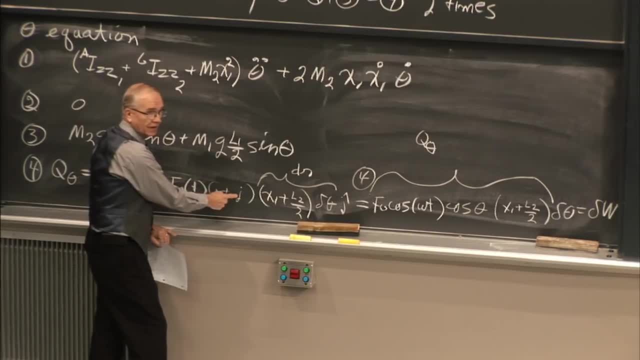 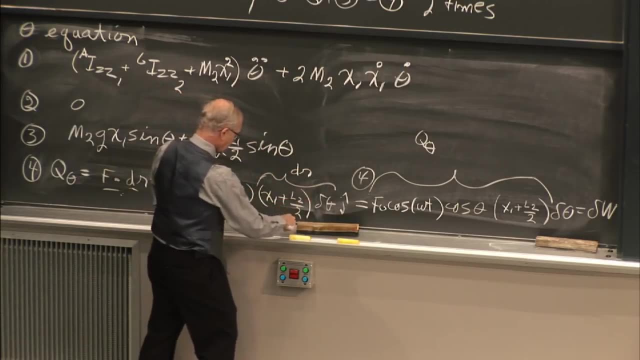 which is written over there. This is the sine theta i, cos theta j term which I pulled out, which I brought back from over there, And we dot it with the dr that we care about, which is x1,. this length times that angle in the j direction. 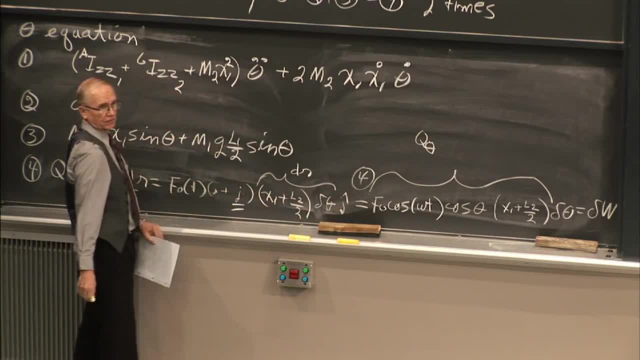 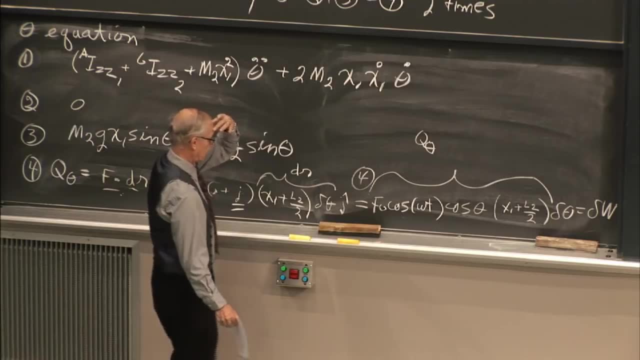 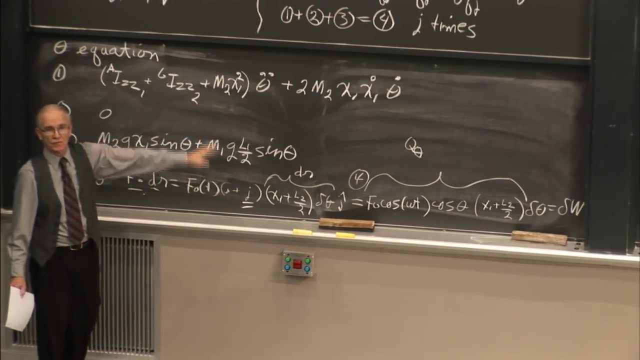 So j dot, we only pick up the j piece of this, And that gives us this cosine, theta term. OK, Let's look quickly. This is a rotational thing. It has units of. is it force? Is this an equation, a force equation? 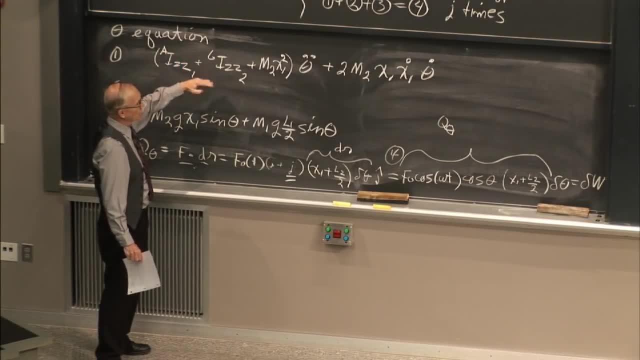 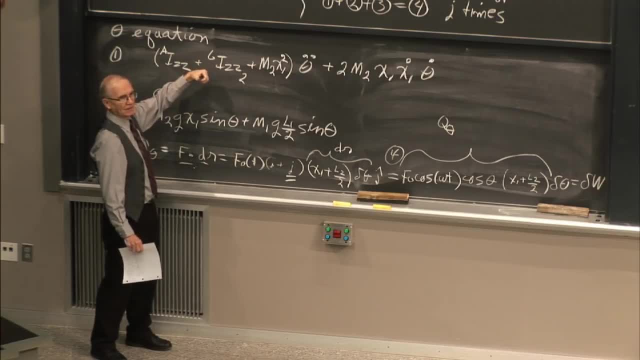 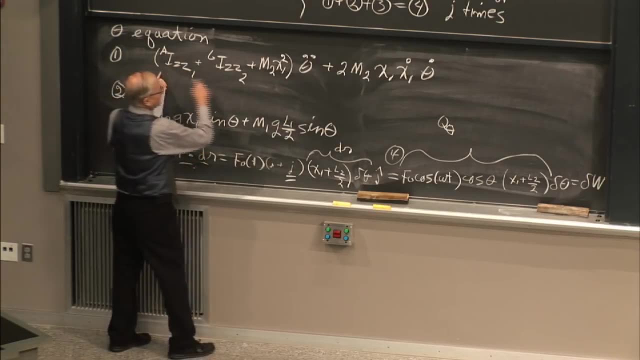 This is the total mass moment of inertia, Izz with respect to a for this system, such that the Eulerian acceleration, the torque it takes to make that happen, is the sum of the mass moment of inertia of the rod plus the mass moment of inertia of g plus m2 x1 squared. 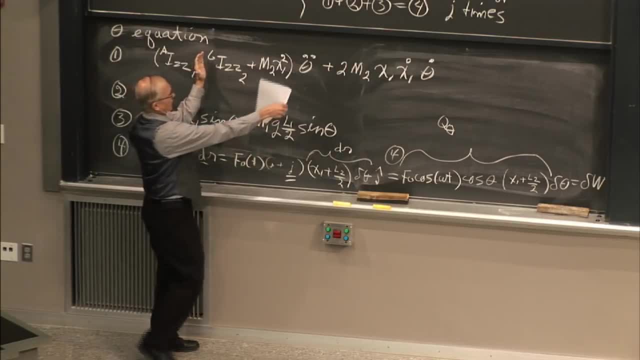 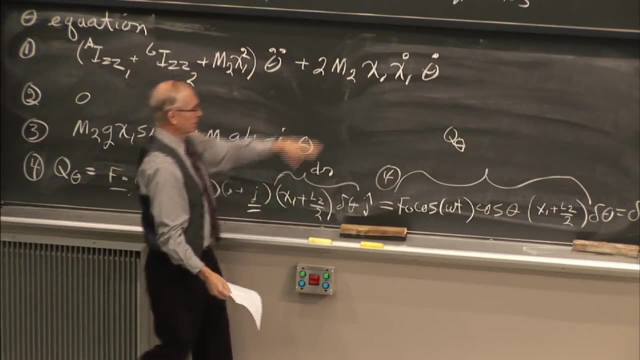 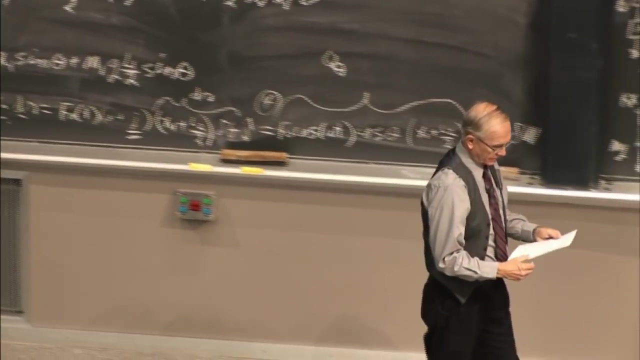 which looks a lot like the parallel axis theorem. This is Izz a for the moving mass. There's your Coriolis term And here's your potential terms, And there's your external force. OK, Talk more about these things in recitation.